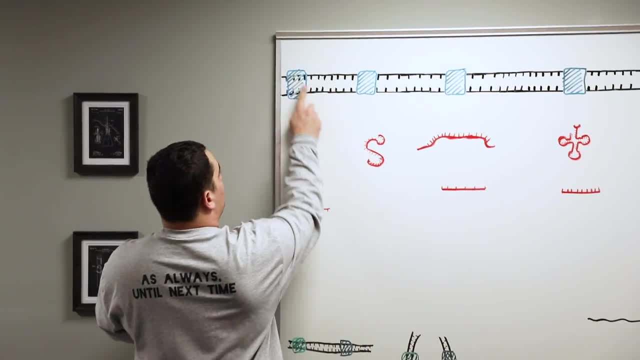 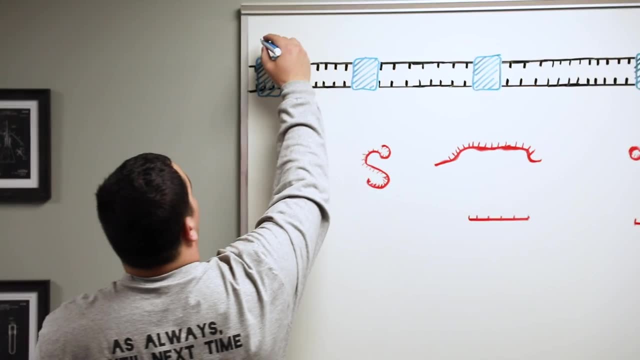 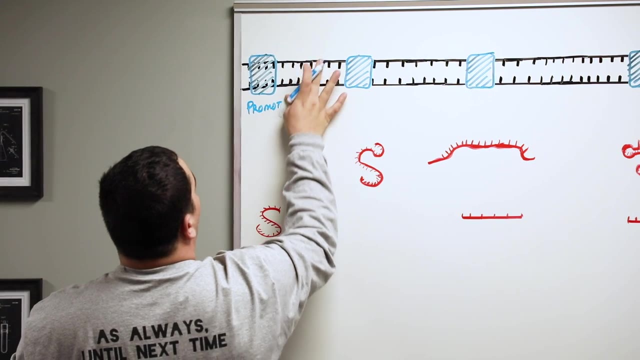 strand here, right, We have this DNA strand. On this DNA strand, we have these blue portions that I've highlighted here as a box with some lines in it. This, right here, for right now, I want you to know, is what's called a promoter. So this is called a promoter region. Now, a promoter region. 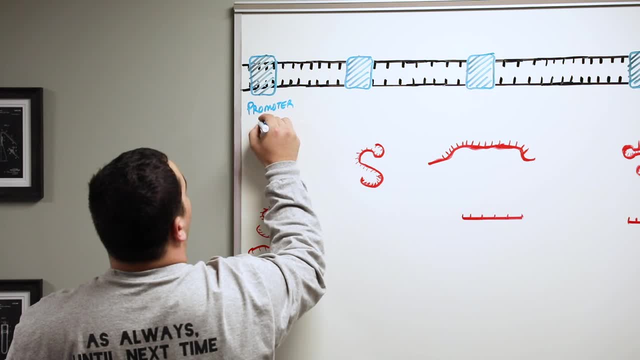 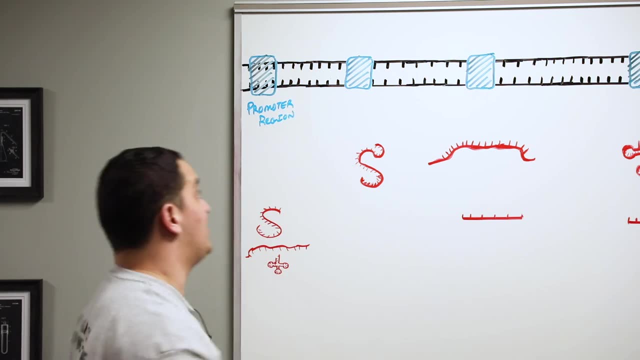 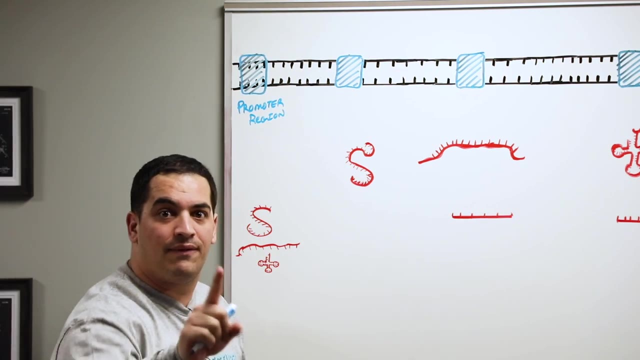 is a particular nucleotide sequence within the DNA, and what it does is it allows for particular proteins, like RNA, polymerases and transcription factors, to bind onto the DNA and then start moving through the DNA, taking the DNA and making RNA. So that's the first thing you 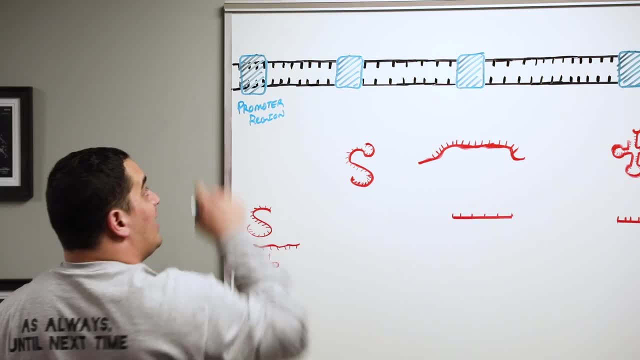 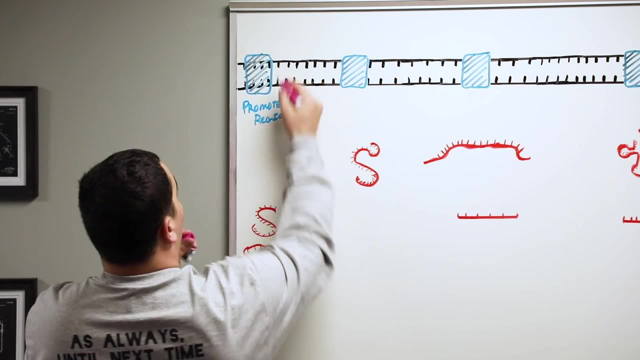 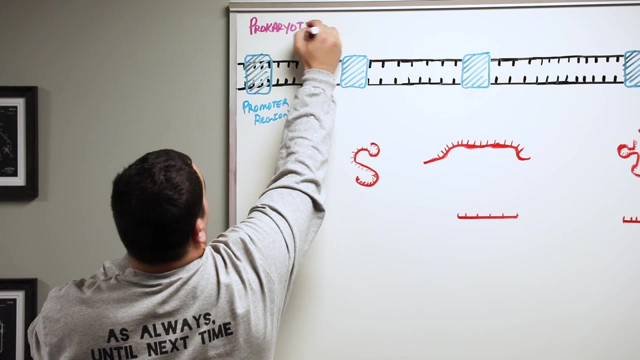 need to know is within the DNA there's a particular nucleotide sequence- we'll talk about a little bit later- called a promoter region, And that's the first thing that we need to identify. Let's say that we take this particularly for prokaryotic cells. So, prokaryotic cells. 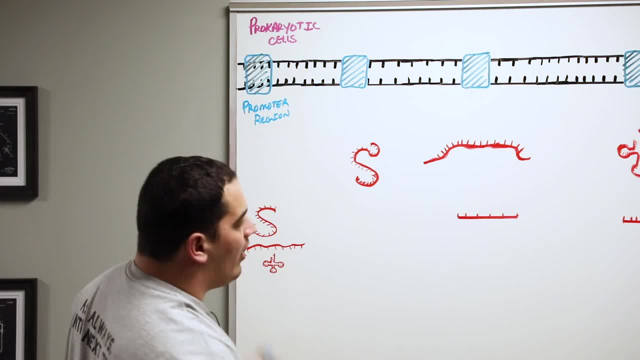 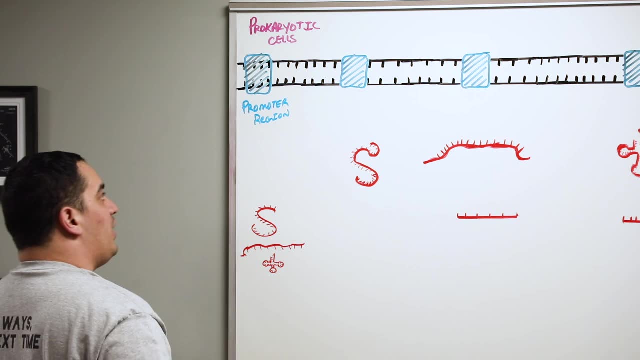 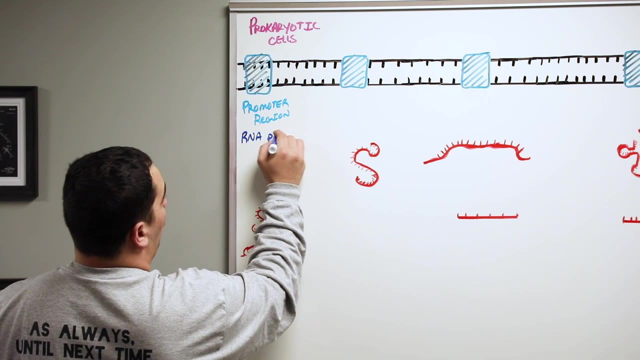 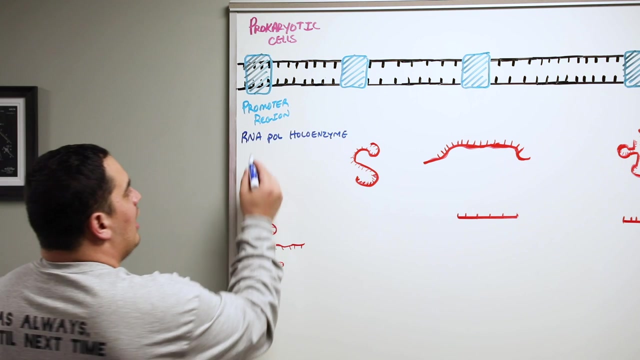 just say like a bacterial cell. okay, Prokaryotic cells use a very particular type of enzyme. What is that enzyme? It's called a RNA polymerase holoenzyme. Okay, so it's called an RNA. we're going to put pol polymerase holoenzyme. Now, that's a lot of stuff. Let me explain. 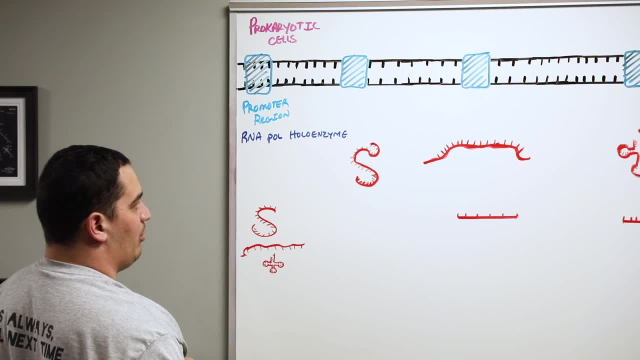 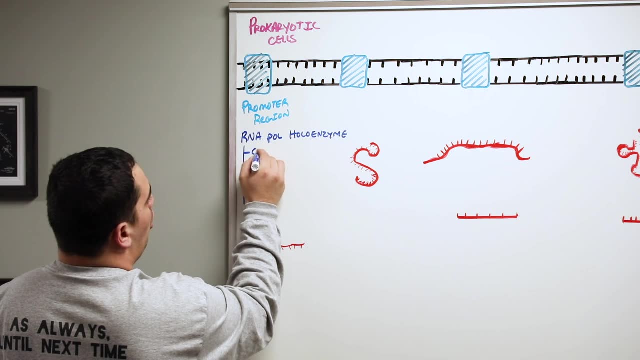 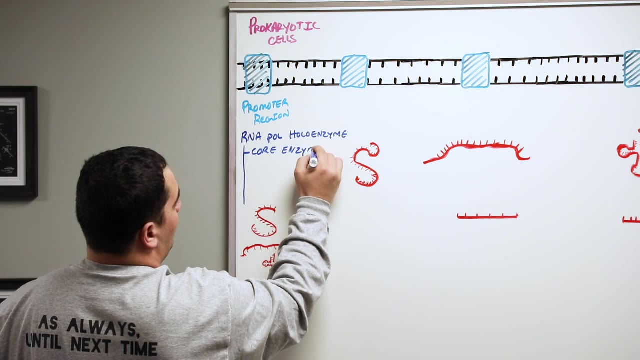 what this is and I'll show you the structure of it, a basic structure of what the RNA polymerase holoenzyme is. It's made up of two things. One of the components of this enzyme is called the core enzyme, And the core enzyme for this RNA polymerase holoenzyme consists of multiple subunits that 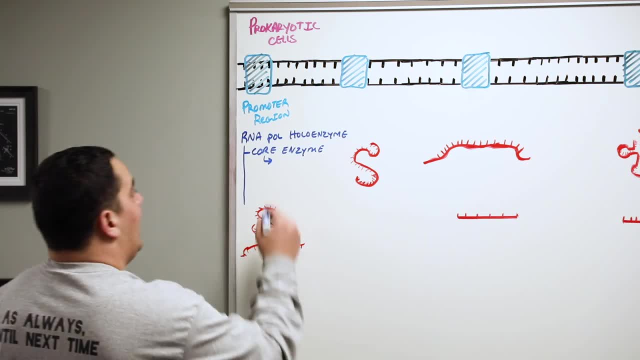 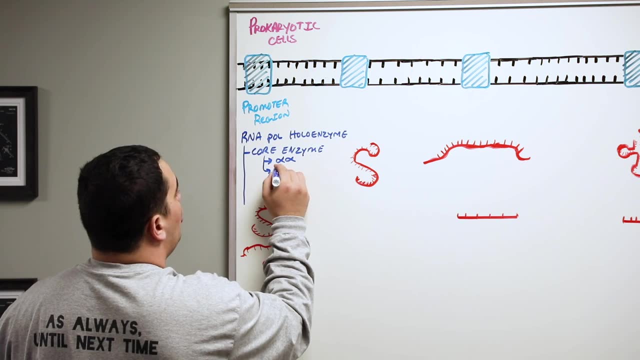 they just love to ask you on your USMLEs and other exams. And these are. they contain two alpha units- okay, two alpha chains, proteins. It contains two beta units. technically we say beta and beta prime. So this is the answer to your question. You really want to be specific? 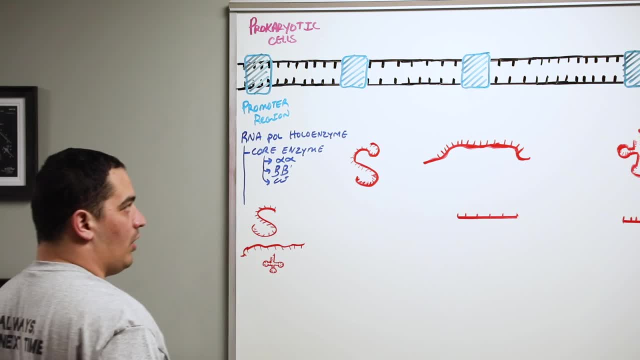 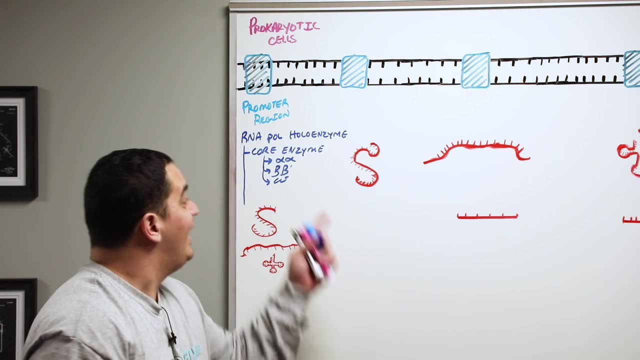 And then one more which is called an omega unit. Okay, so these are the primary components of the core enzyme which makes up RNA polymerase. What's important to remember is that these are what are going to really read the DNA and make RNA. 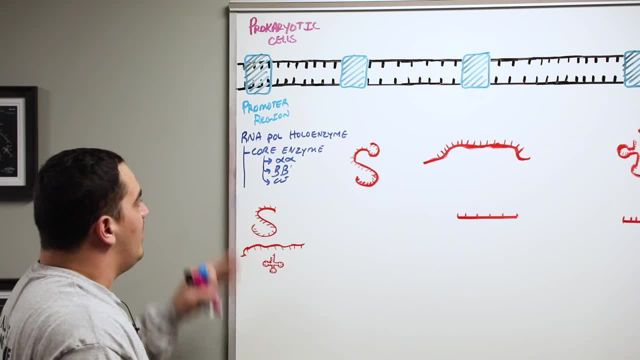 That portion of the enzyme reads the DNA and makes RNA. The next component of the RNA polymerase holoenzyme outside is the portion that we need in order to bind to the DNA, to the promoter region. Without it, we won't be able to allow for. 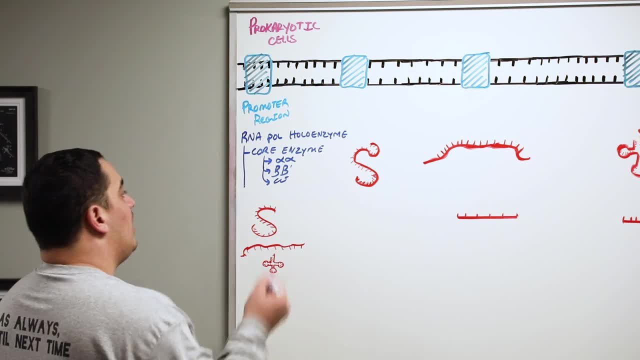 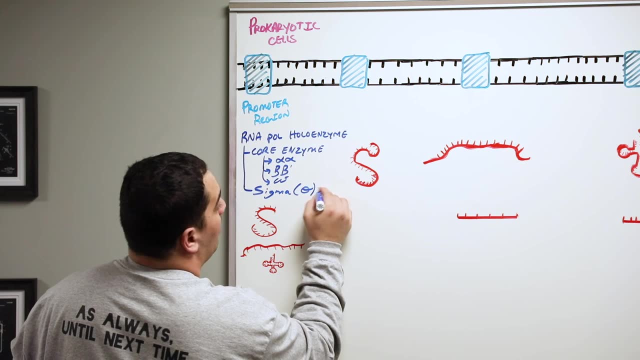 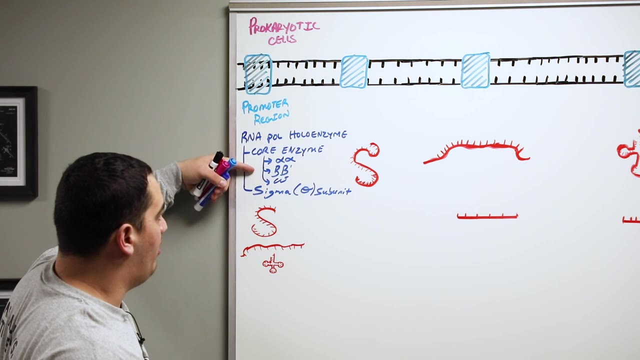 this RNA polymerase to bind to the DNA and transcribe it. This is called the sigma right or you can represent it like this: subunit or factor, if you will. okay, These two components: the core enzyme, which is made up of the 2-alpha, the beta and the beta prime, and the omega subunit. 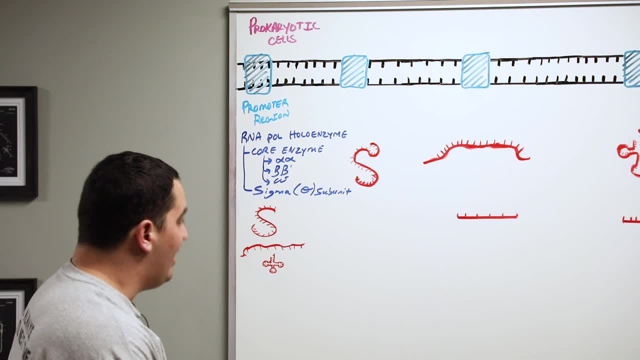 as well as the sigma subunit, make up the entire RNA polymerase. Now let me show you, for example here. Let's say I represent the core enzyme as just this kind of blue circle with lines in it, and then we'll represent the sigma subunit as kind of like a pink circle with some lines in it. 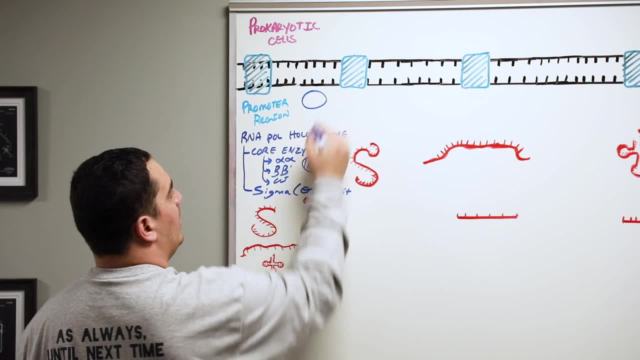 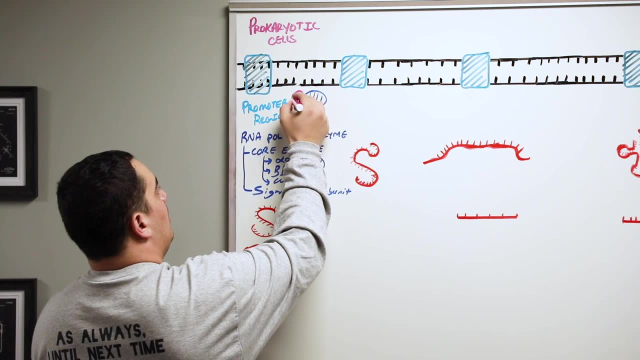 right. So let's imagine here we have that core enzyme, which we're going to represent like this, and then the other component of it, which is the sigma subunit, which we'll represent like this. That sigma subunit will then bind to the promoter region. 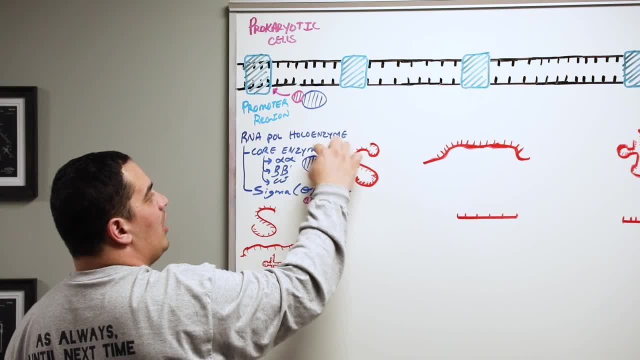 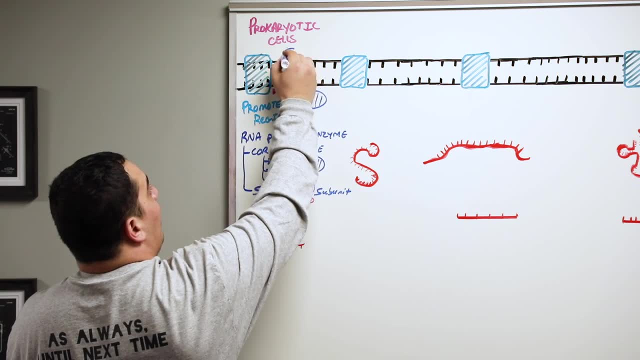 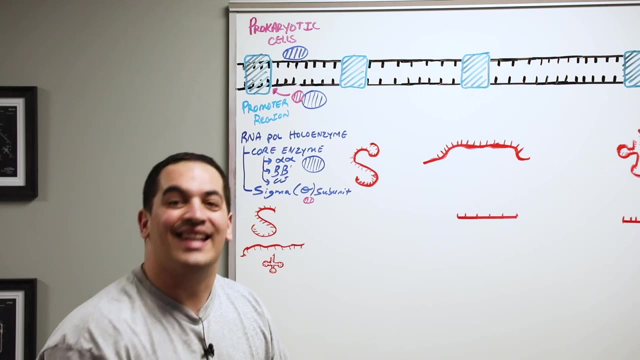 Once it binds to the promoter region, then this core enzyme of the RNA polymerase will then release away from the sigma subunit and it'll start moving down this DNA. and as it moves down the DNA, it'll read the DNA from 3 to 5 and synthesize an RNA strand from that which we'll talk about more. 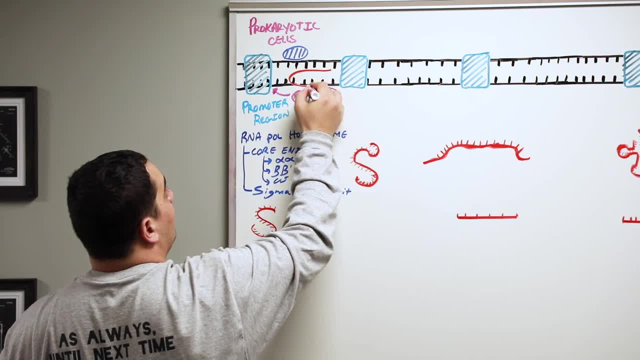 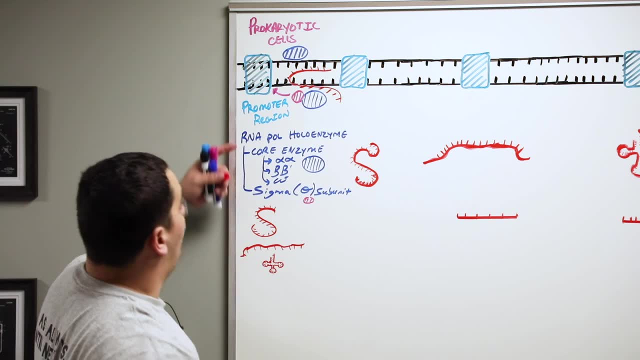 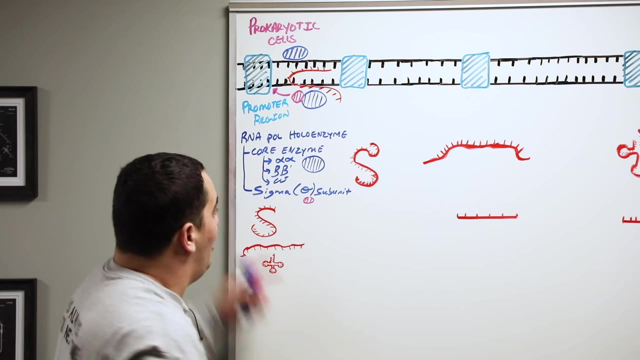 detail later from 5 to 3, so it'll read the DNA and make RNA. this RNA that we make from in prokaryotic cells with the RNA polymerase holoenzyme is very different from eukaryotic cells. in prokaryotic cells, that mRNA that we made 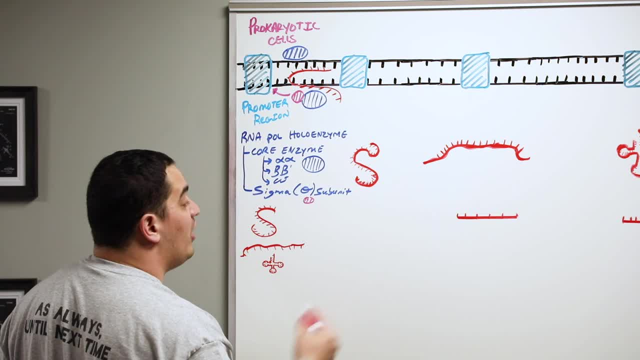 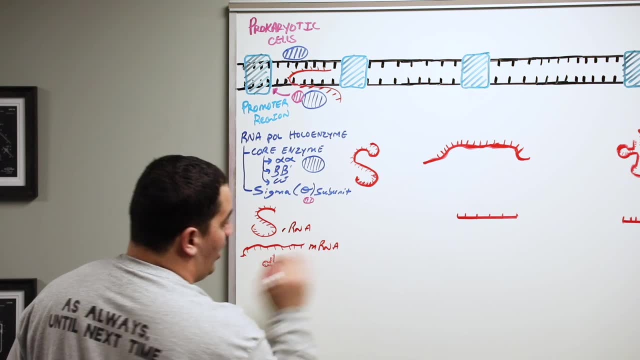 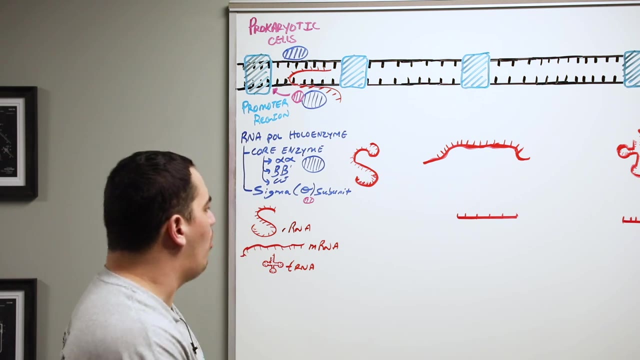 from this one RNA polymerase holoenzyme can make all the RNA we need, whether that be our RNA within the prokaryotic cell, whether that be mRNA within the prokaryotic cell or tRNA within the prokaryotic cells. so that's very important big thing. I really need you guys. 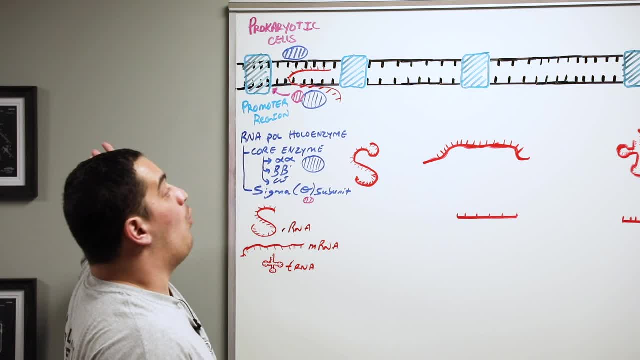 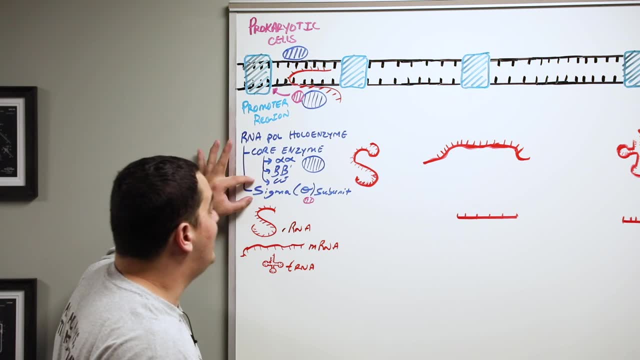 to take away from, that is prokaryotic cells. they use one RNA polymerase, which is called a holoenzyme, made up of two components: a core enzyme made of these subunits and a sigma subunit. the core is what reads the DNA, makes the RNA the. 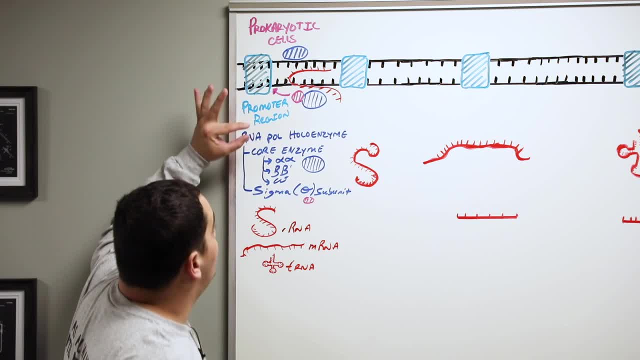 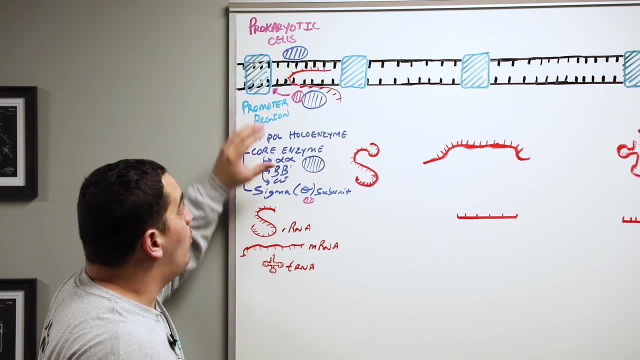 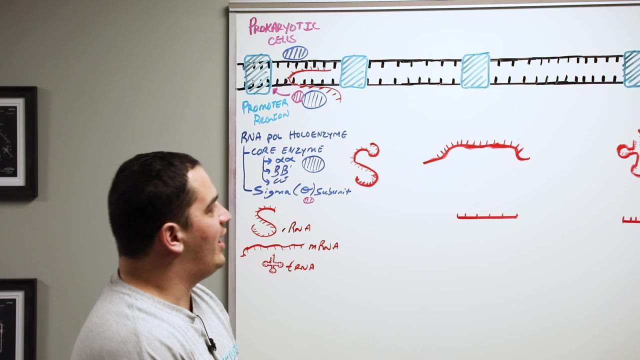 sigma subunit is what binds the RNA polymerase to the promoter region, enabling it to transcribe the DNA. okay, and whenever you make RNA within a prokaryotic cell from this RNA polymerase, it makes all the RNAs that are in that prokaryotic cell and eukaryotic cells. it's a little bit. 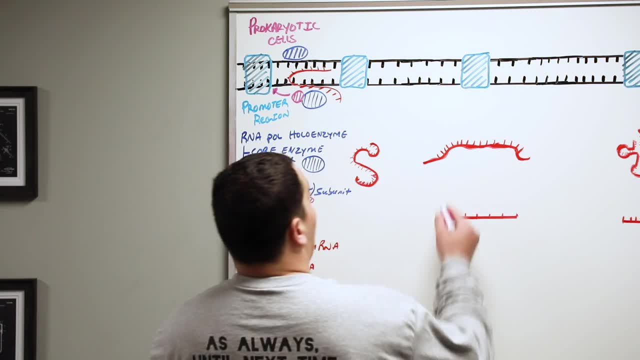 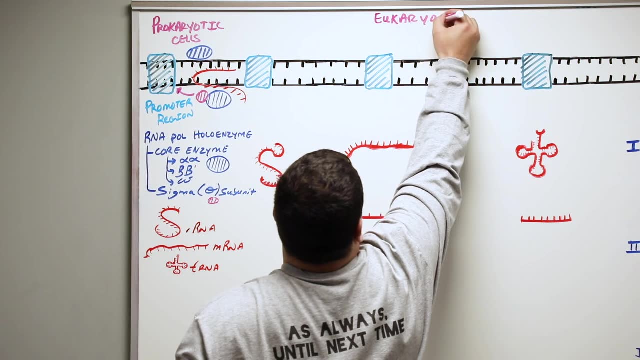 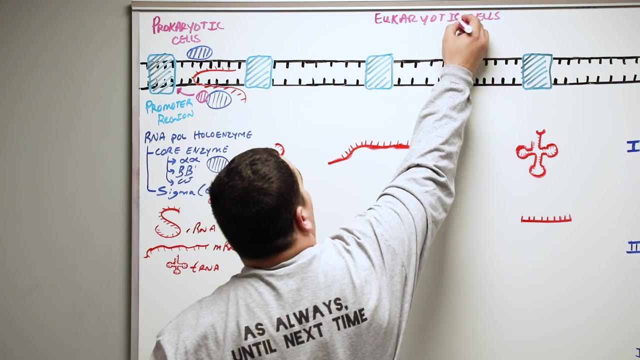 different, so let's talk about that. let's say, here we have three promoter regions that I want us to focus on, and this is all within eukaryotic cells and eukaryotic cells. we need two different things in order to allow for transcription to occur. 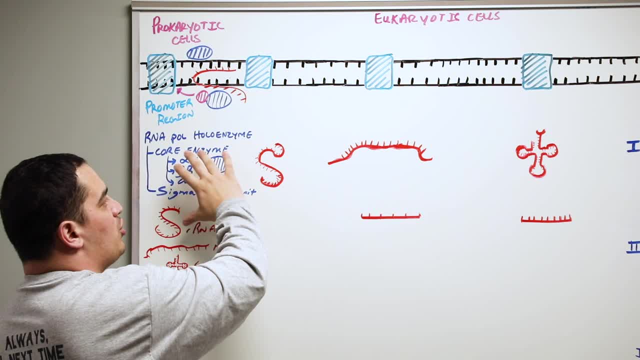 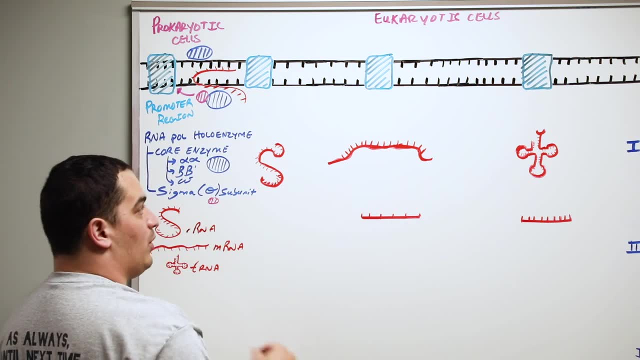 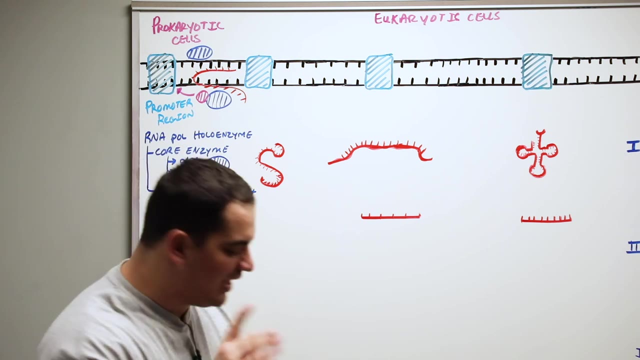 and this portion here, right, and this portion of prokaryotic cells. we only need one enzyme and which had two different components. within eukaryotic cells, each process requires a particular enzyme, an RNA polymerase and a transcription factor. let's, let's kind of write that down. so let's say that we take this first. 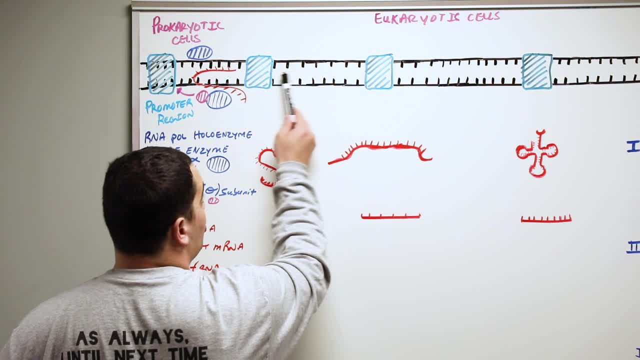 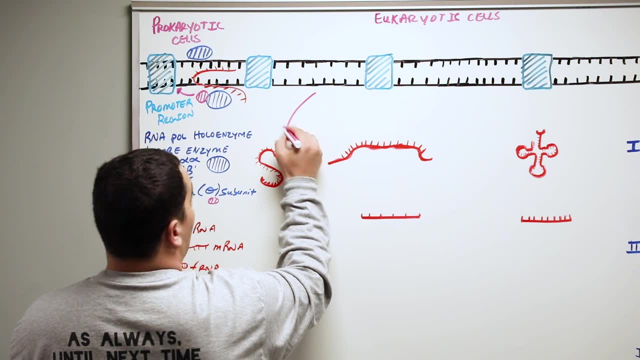 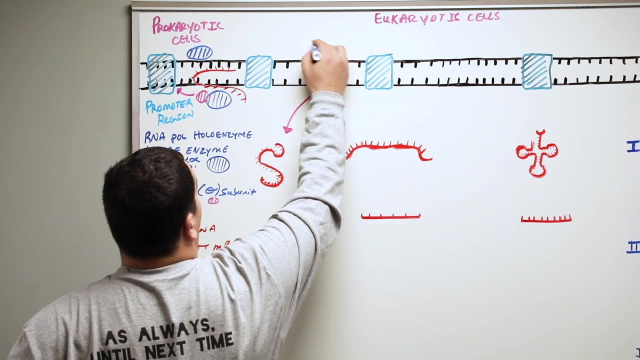 promoter. we want to read this gene, this portion of the DNA, and make RNA, and this is the RNA that we're actually going to synthesize right here. okay, from this gene, a particular enzyme. let's represent this in blue, since we've been kind of doing blue here. there's going to be a particular 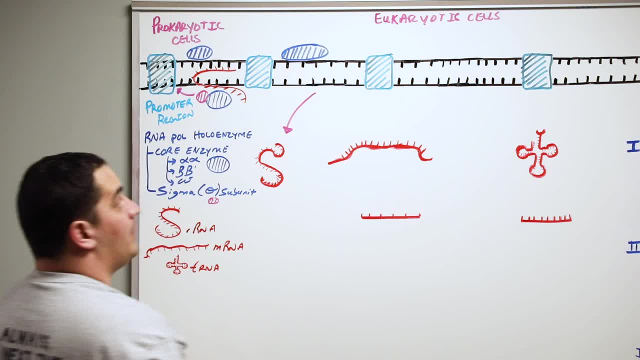 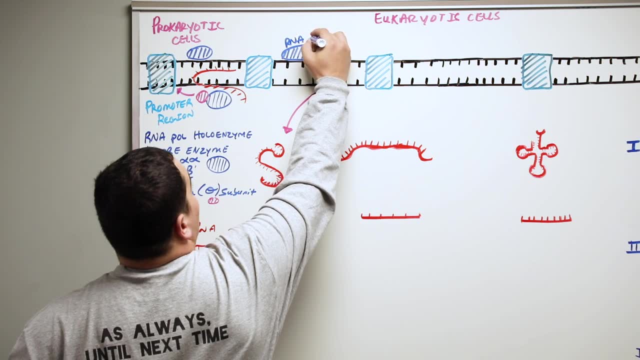 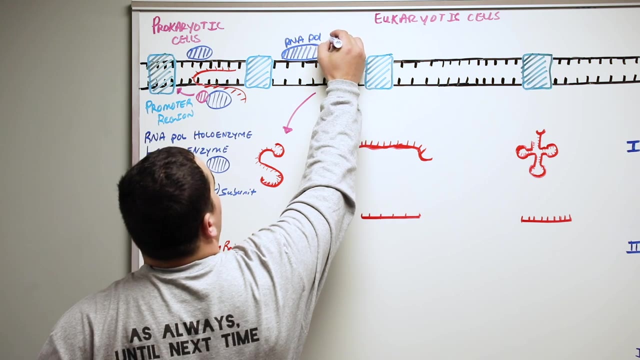 enzyme which is going to read this DNA, okay, and make this RNA. there's a particular enzyme. what is that enzyme called? it's called RNA polymerase, but this is the first promoter within the eukaryotic cells that we're talking about, right? so let's call it RNA polymerase 1. RNA polymerase 1 will read: 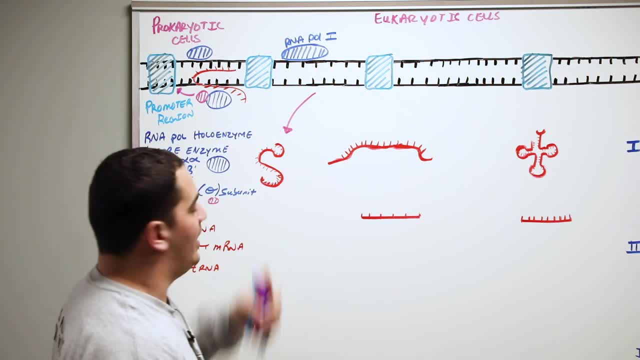 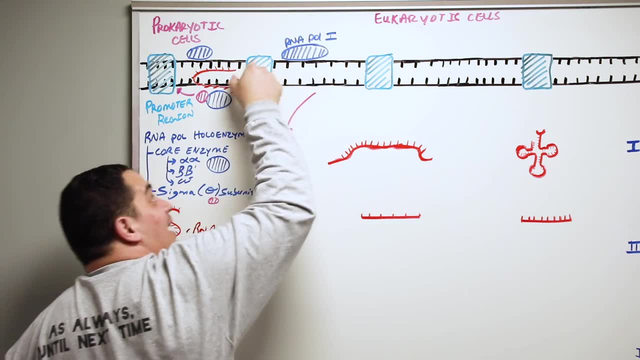 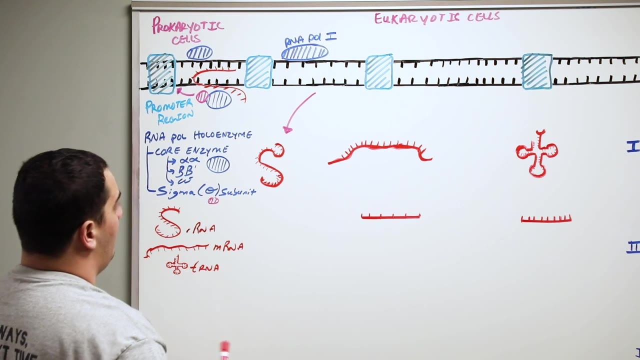 the DNA and make a particular type of RNA. but in order for it to do this, it needs a special protein that can bind to the promoter region, which allows for the RNA polymerase to bind to the DNA and read the DNA. what is that particular protein? that protein, let's represent it here and let's do green. there's a. 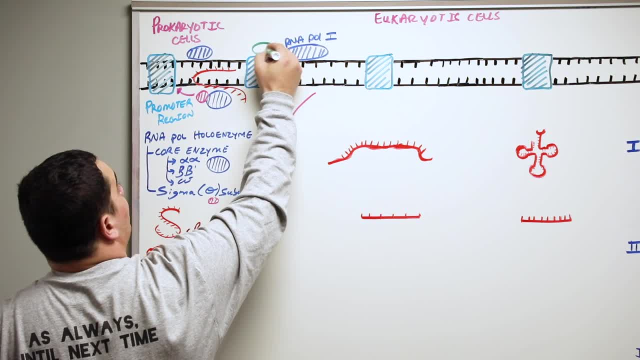 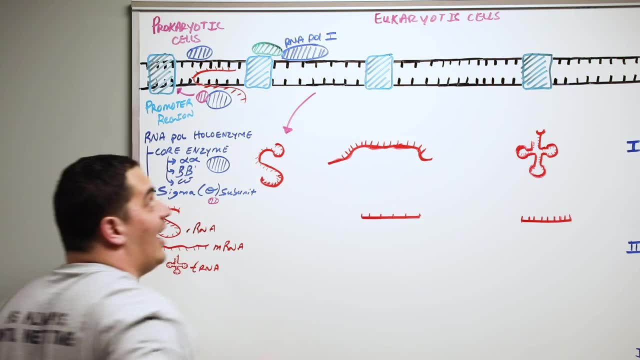 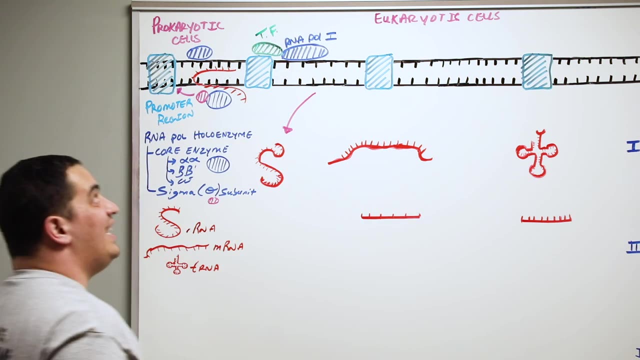 particular protein which will bind here to the RNA polymerase and to the promoter and allow the RNA polymerase to bind to the DNA and start moving down, reading the DNA and making this RNA. what is this called? this is called a transcription factor, TF, and there's 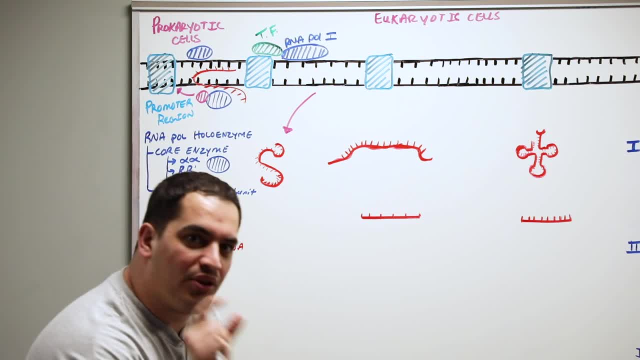 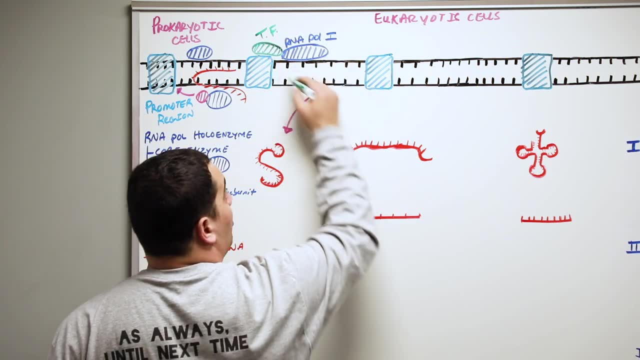 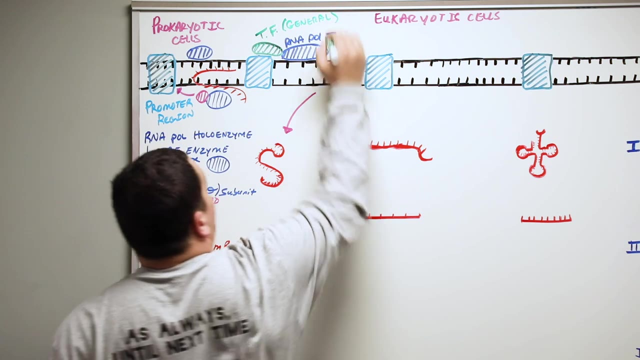 many different types of transcription factors. the particular thing that I need you to remember for right now is that we call these transcription factors which are utilized by RNA polymerases within eukaryotic cells. we call these general transcription factors. we'll talk about very specific types with an RNA. 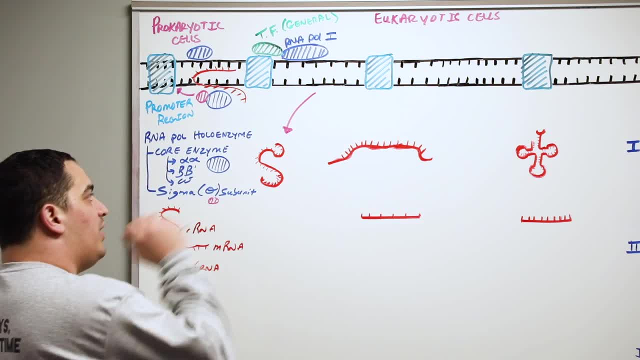 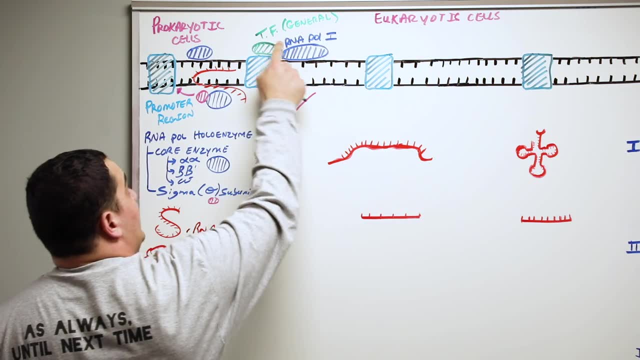 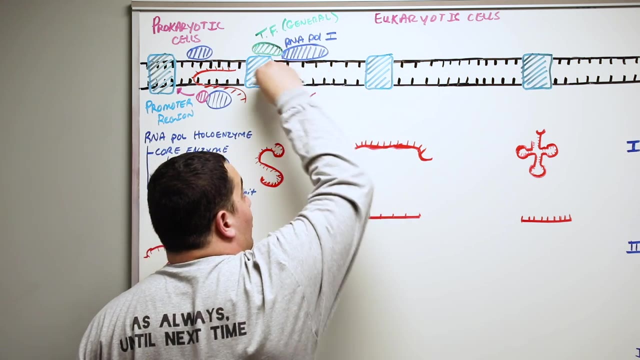 polymerase type 2 a little bit later, but for right now, two things I need: in order for this RNA polymerase to be able to read the DNA and make this RNA, RNA polymerase 1 needs a general transcription factor to bind to the promoter, allowing the RNA polymerase 1 to then bind into the DNA. 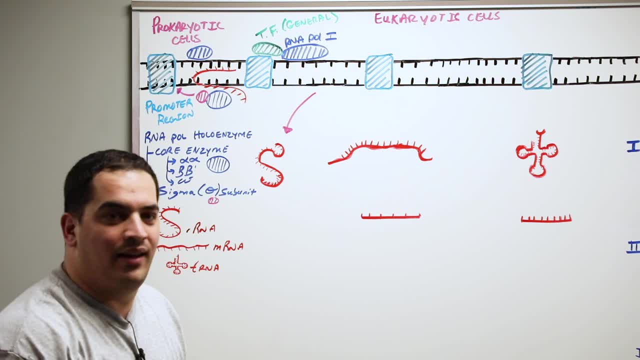 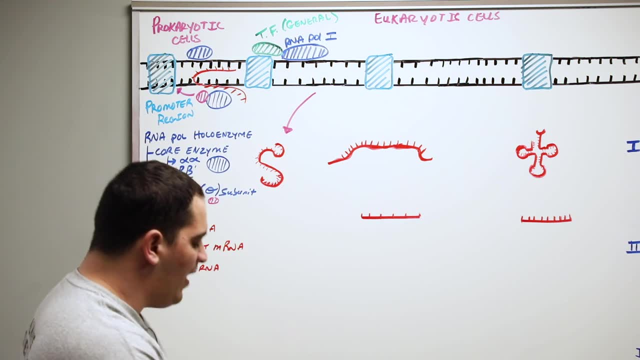 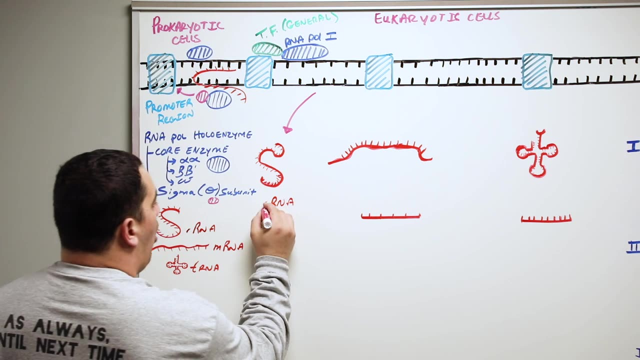 read it and make RNA. what type of RNA does it make? I have all the RNAs within prokaryotic cells from one RNA polymerase, but RNA polymerase 1 makes a very particular type of RNA and this is called our RNA. now, our RNA is very 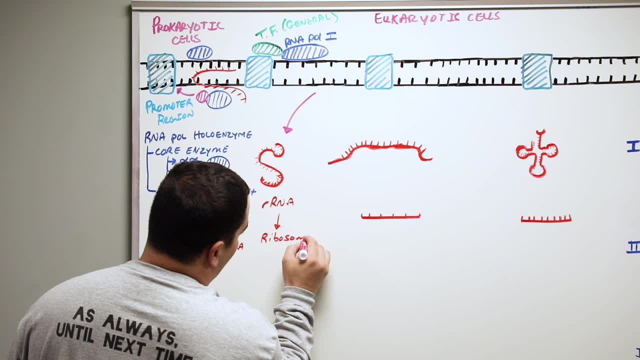 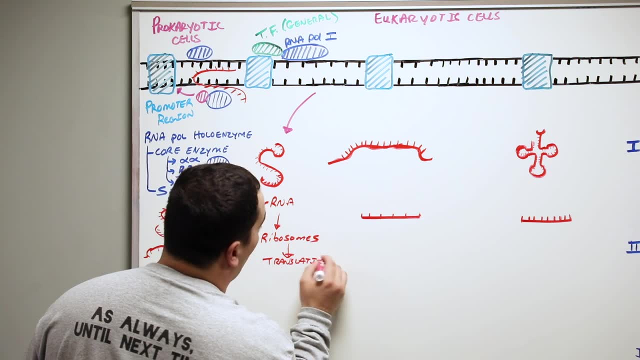 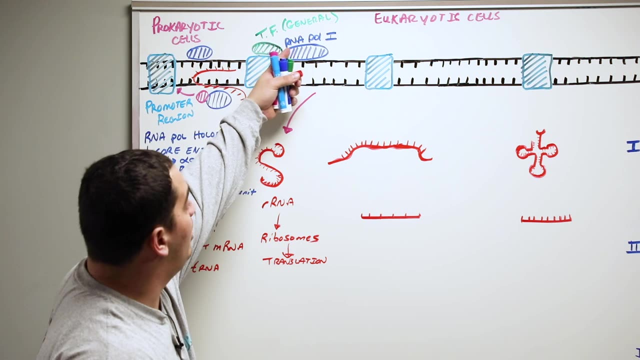 important because this is incorporated into what's called ribosomes. ribosomes and ribosomes are utilized in the translation process, where we take mRNA and from that make proteins. so we'll talk about this later in another video, but for right now, first thing I need, you knows, RNA polymerase 1 with transcription. 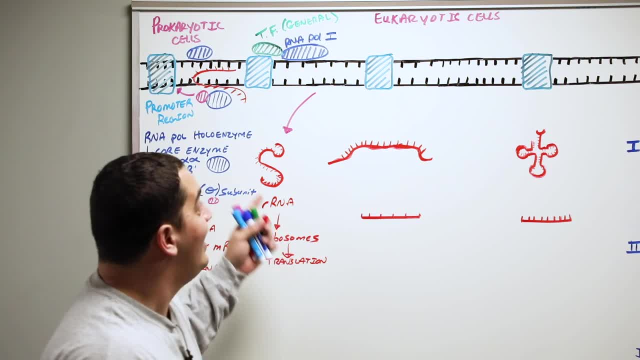 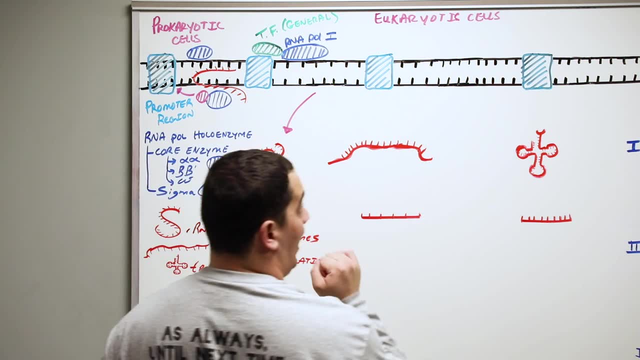 factors reads the DNA and makes RNA polymerase 1, our RNA. now that makes everything else pretty easy from this point. here's another promoter region of a particular sequence of DNA right within a eukaryotic cell. so this is the second promoter region. another enzyme binds. 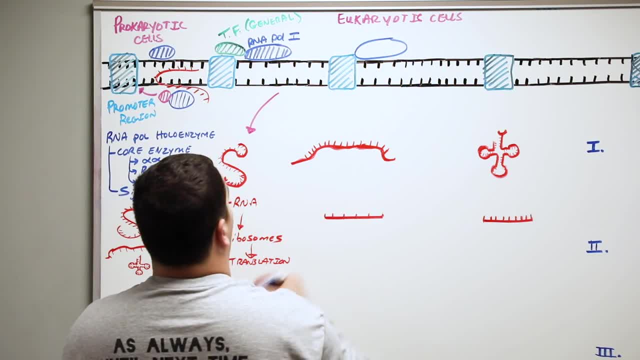 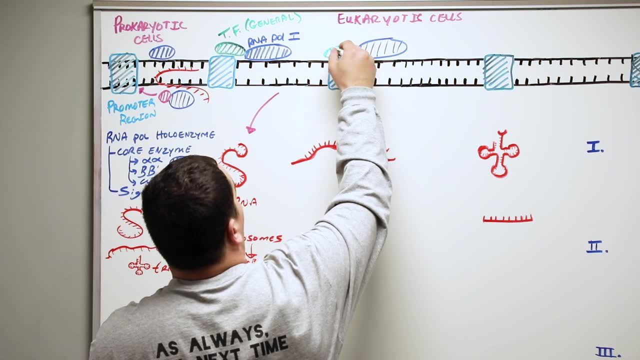 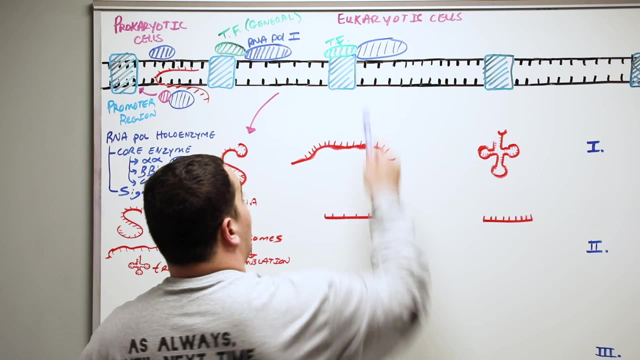 another RNA polymerase, and not only just that one RNA polymerase here, but we also need a set of general transcription factors to bind to this promoter region. so general transcription factors we need to bind to the promoter region, enabling this RNA polymerase to bind to the DNA, read it and then make what Make these particular? 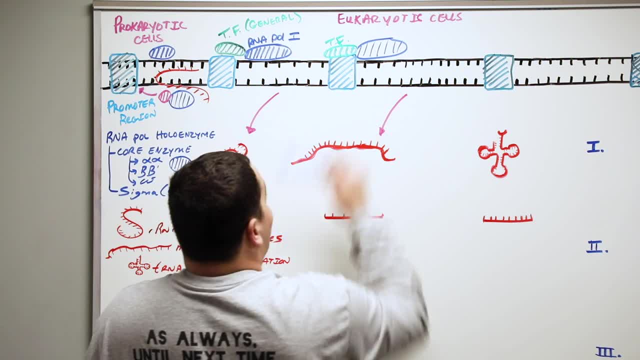 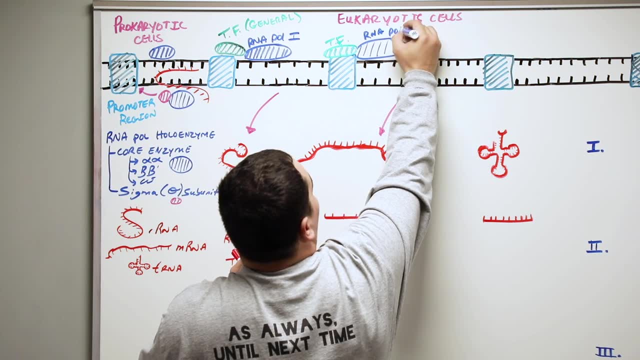 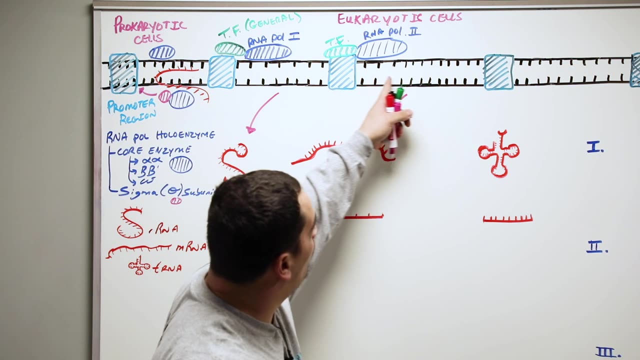 types of RNA we have here. This is well. this was the first promoter, this was the second one. alright, so we're gonna call this RNA polymerase 2.. RNA polymerase 2 will bind to this promoter via the transcription factor, read the DNA and make RNA. What kind of RNA is it going to be? 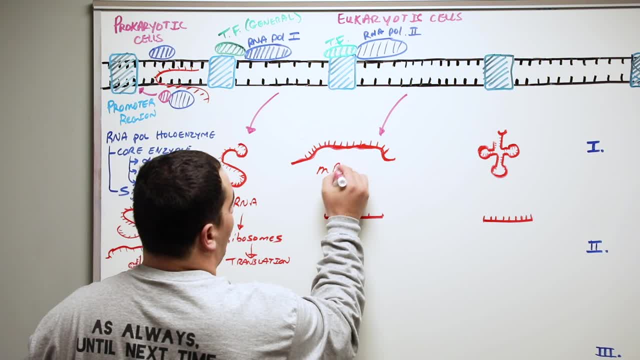 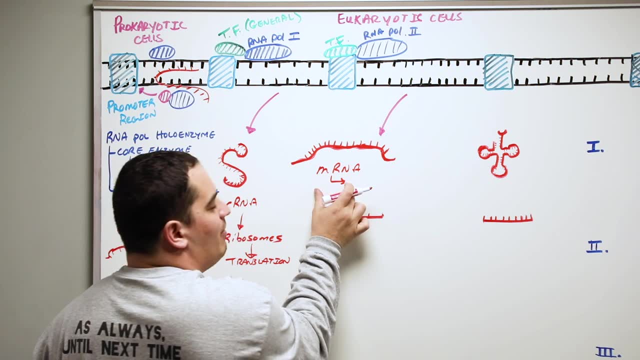 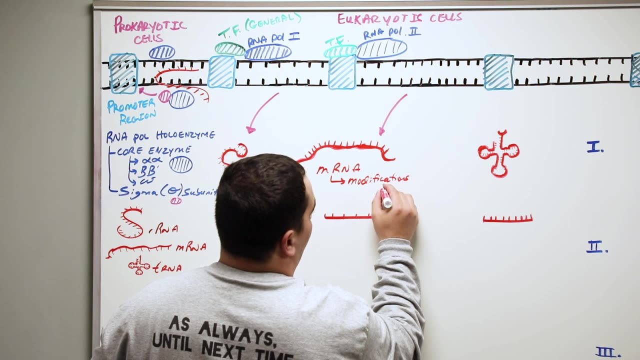 making Big thing I need you to remember is it's making mRNA. mRNA, you'll see later again, is the component. it'll have to go through some very specific modifications that we'll talk about in great detail and then eventually it'll be translated with the help of rRNA and another. 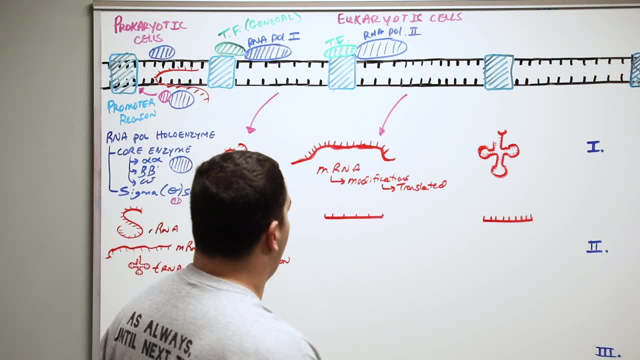 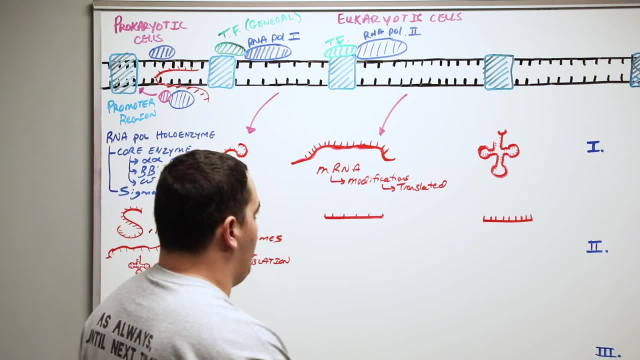 thing called tRNA at the ribosomes and making proteins. okay, The other thing that you guys can remember, if you guys want to be scholarly or ninja, if you guys want to learn a little bit more about generity, there's another RNA that's made here and we'll talk about it a little bit later. 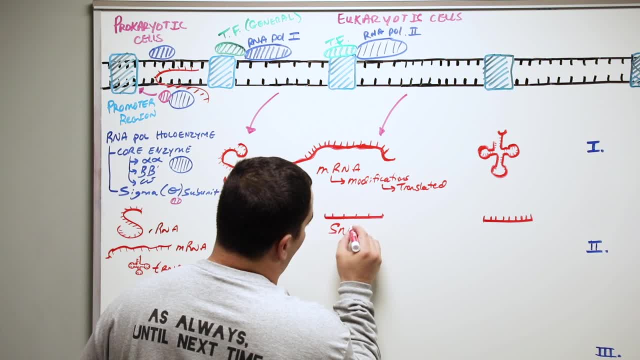 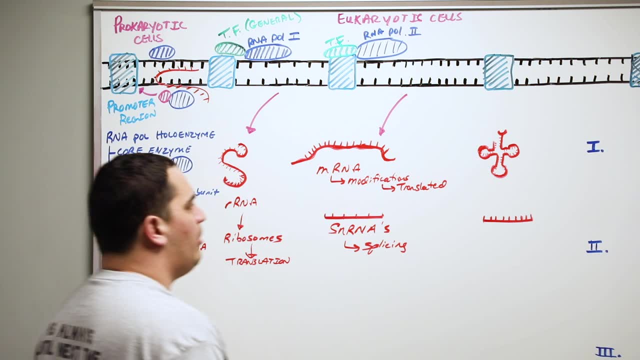 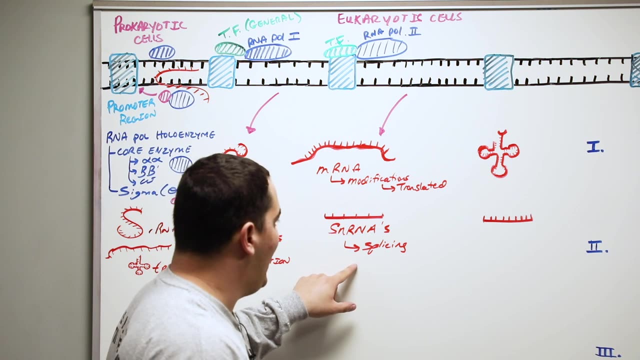 with what's called splicing and these are called small nuclear RNAs and these are involved in what's called splicing and we'll get into that a little bit more in detail later. okay, But big thing: RNA polymerase 2, with the help of general transcription factors, makes mRNA and SNRNAs RNA. 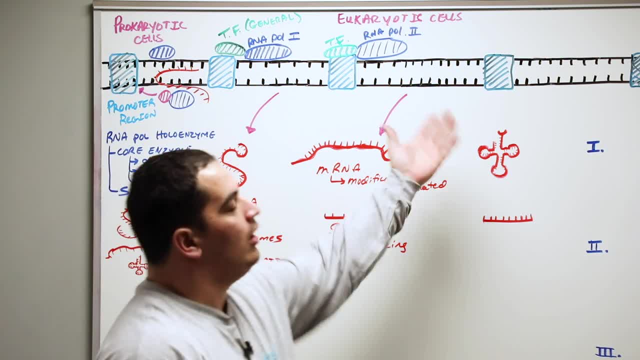 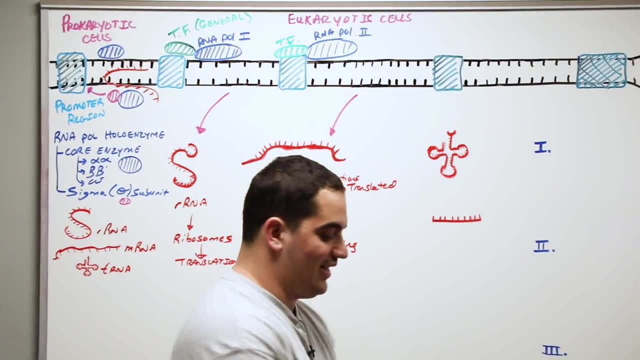 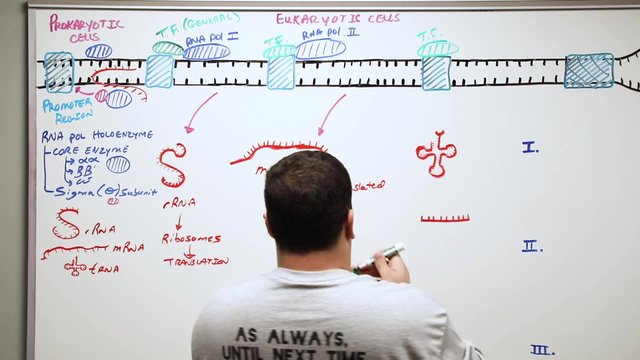 polymerase 1, with the help of general transcription factors, makes RNAs. When the heck do you think this sequence of DNA within this eukaryotic cell is going to make tRNAs? And it's the same process. What do I need here? I need general transcription factors to bind to the promoter region. When that 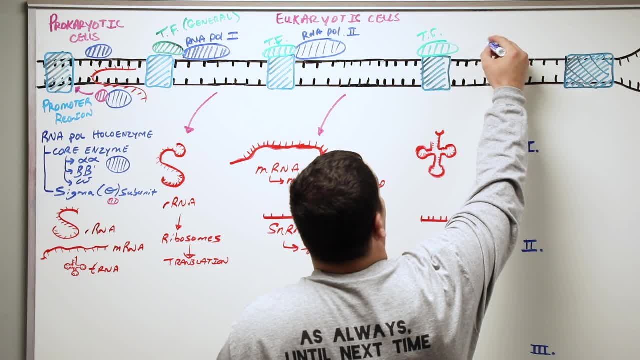 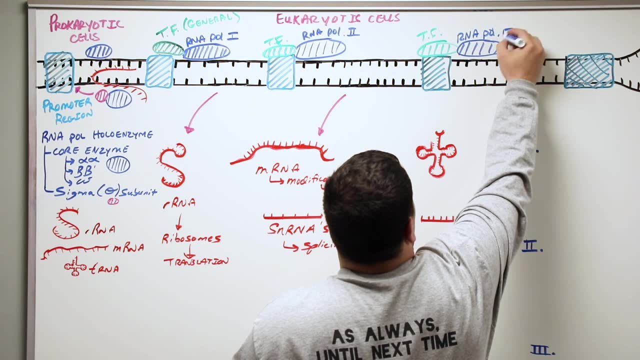 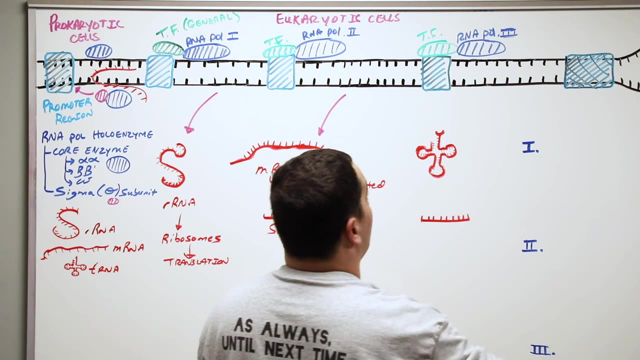 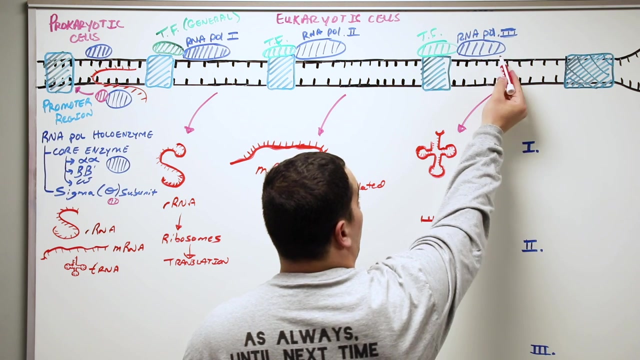 binds, that facilitates or it helps to allow the RNA polymerase type what 3 to bind to the DNA and then read the DNA and then synthesize what RNA? So what type of RNA is it making The type of RNA that is being synthesized from? RNA polymerase 3 is 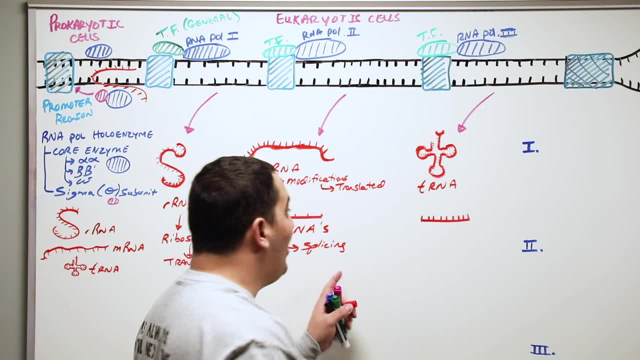 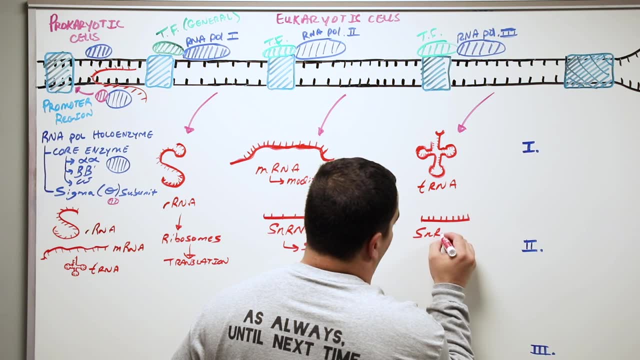 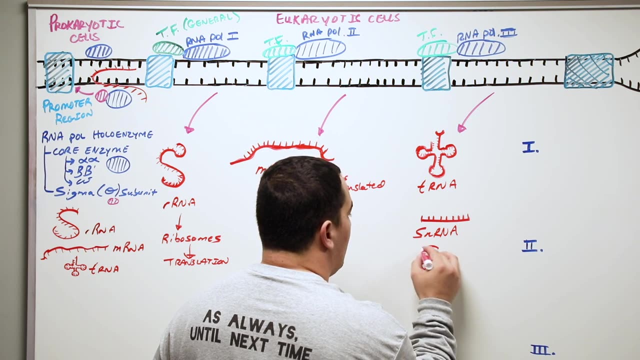 primarily tRNA, but a teensy little bit of SNRNA is also made by RNA polymerase, type 3, and if you guys really want to be extra ninja nerdy, technically even a teensy bit of rRNA is also made here as well. okay, Now tRNA. what that means is that it makes tRNAs, If you guys want to learn. 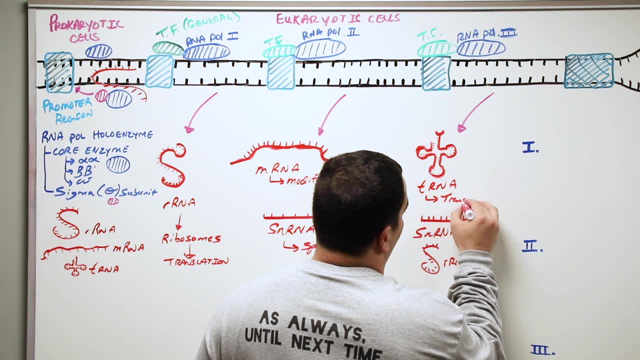 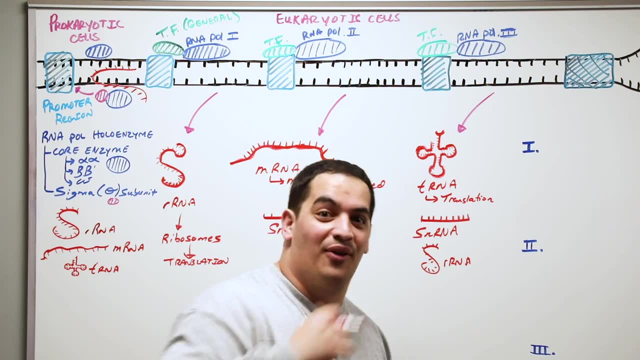 heck does this do? You'll see later that this is also involved in the translation process. It carries a particular amino acid and an anticodon which is going to be involved in that process and we'll talk about that in a separate video. So I 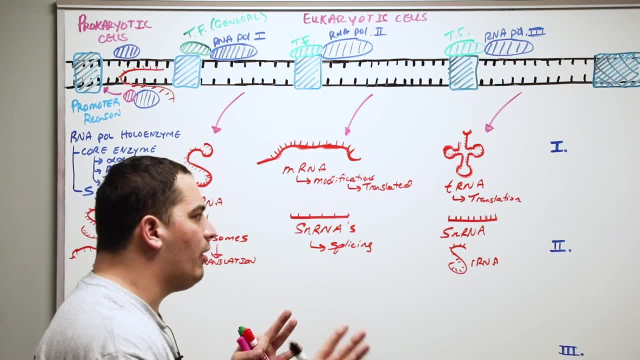 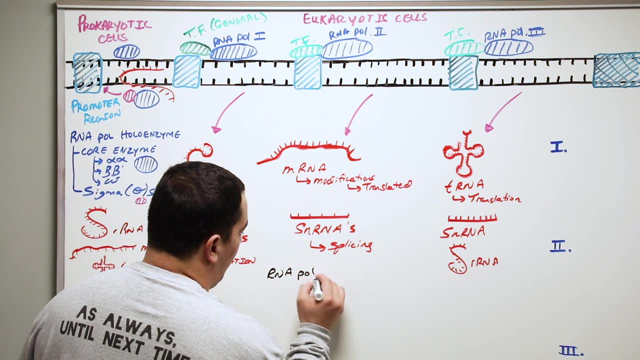 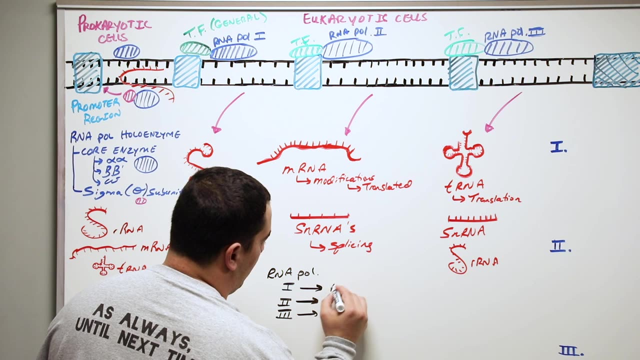 know this was a lot of stuff to take away from this, but the big overall theme that I really just add all of this. what I want you to take away from this is this quick little thing here That RNA polymerases- one, two, three- remember R, MT RNA polymerase- one primarily gives away to rRNA RNA. 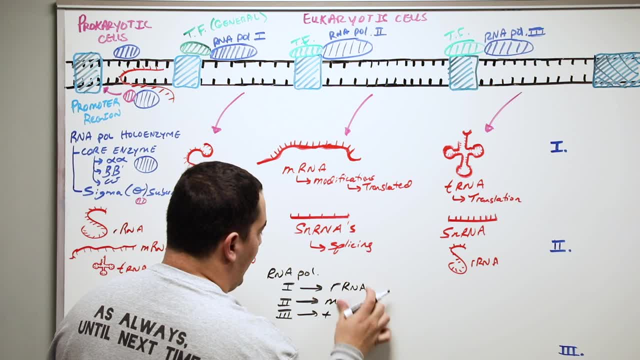 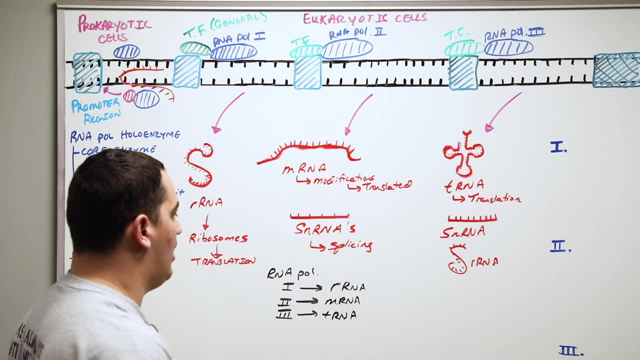 polymerase two primarily gives away to mRNA, And then RNA polymerase three primarily gives way to tRNA. These are the big things that I want you to take away from all of this If you want to go the extra mile and be extra Ninja nerdy. 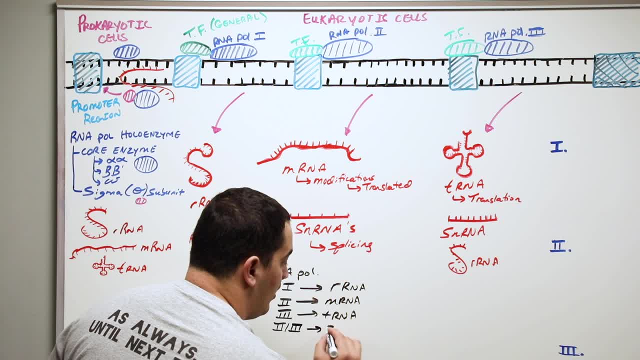 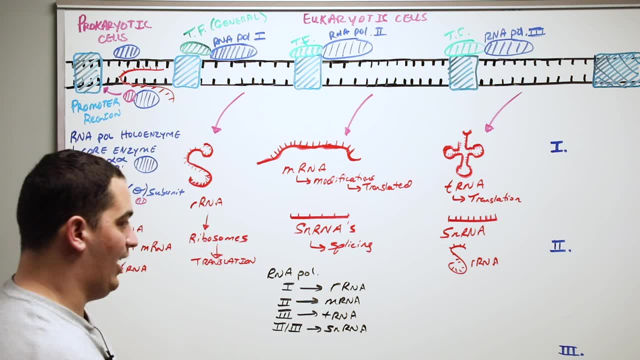 two and three also can giveway to what Small nuclear RNA? If you really want to go the extra mile and be extra ninja nerdy, you can go the extra mile and be extra. technically, three can also give way to RNA, But this is the basic thing to take. 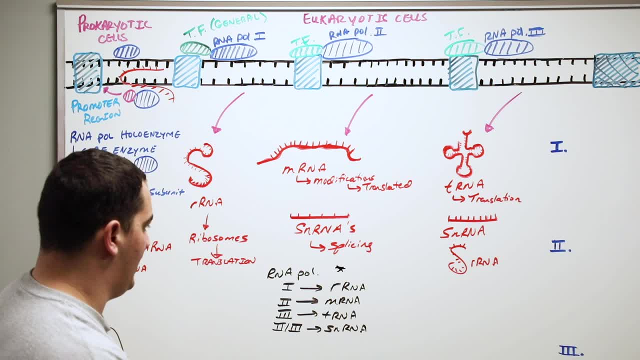 away from what we just talked about. And then the other thing is in prokaryotic cells. we don't need all of these. We need one RNA polymerase holoenzyme to make all the RNAs. One last thing is: you notice in eukaryotic cells that we have 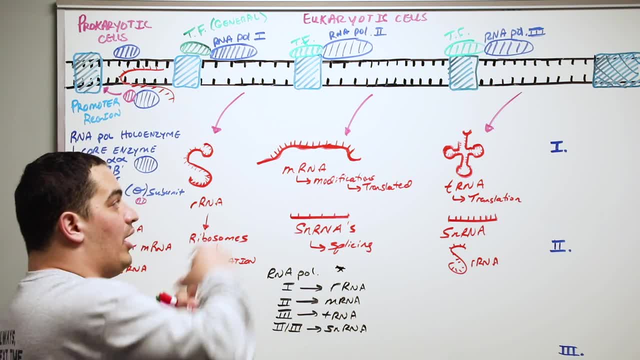 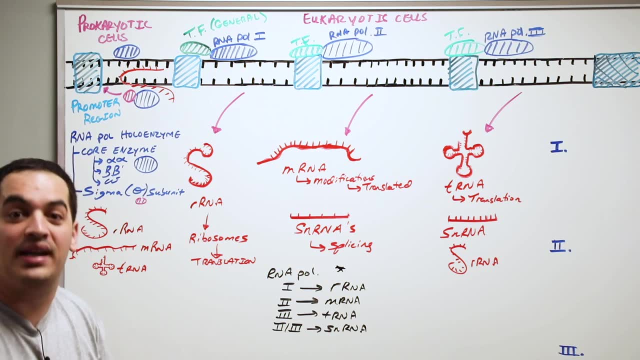 particular transcription factors that are going to be needed for each RNA polymerase. The transcription factor in prokaryotes- technically, if you want to be specific, is the Sigma subunit, because it's the portion that's binding to the promoter to allow the core enzyme of the RNA polymerase to read the DNA. Okay, So 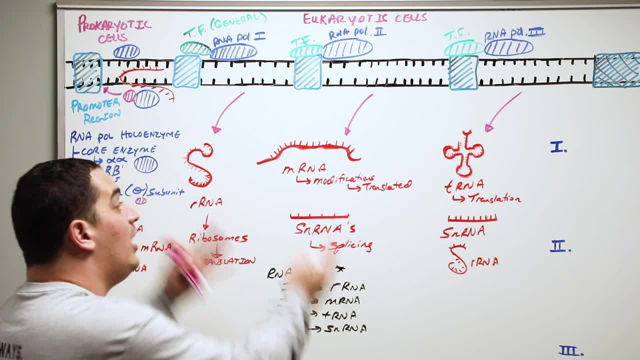 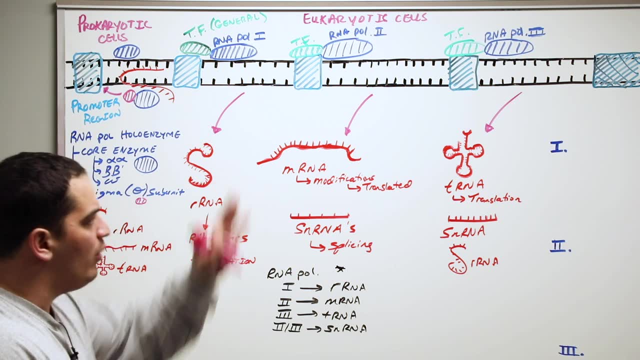 that kind of covers the basic concepts of the two main things that we need in order for this transcription process to occur. Now there's one other thing that I want to talk about very quickly, before you really start talking about mRNA, because that's going to be the primary topic here. I want to have a quick little. 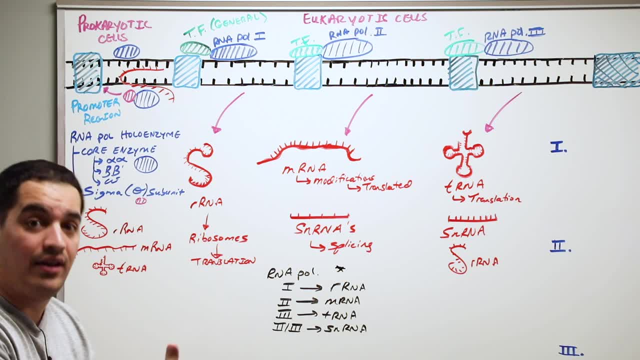 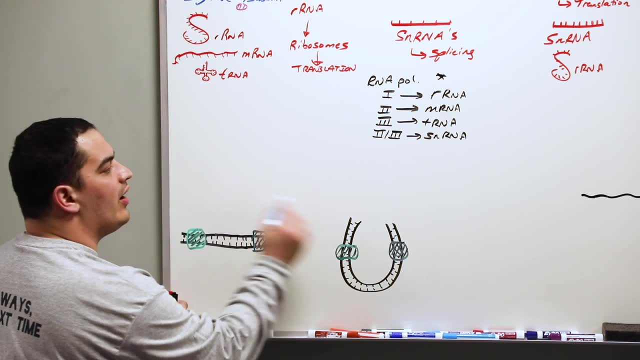 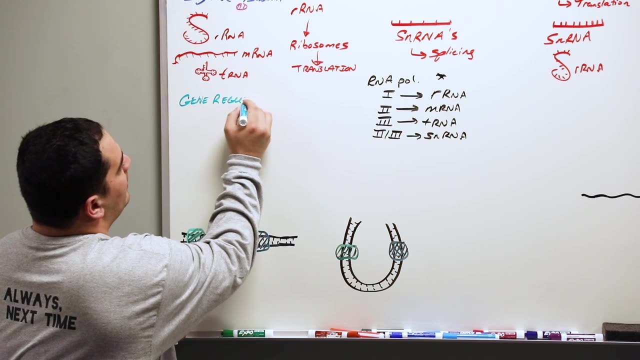 discussion on how we can modulate the rate of transcription, either speeding in up or slowing it down. okay, so the next thing I want to talk about is very, very briefly, on eukaryotic gene regulation. so I want to have a quick, quick, tiny little discussion on gene regulation. okay, and the only reason I want to 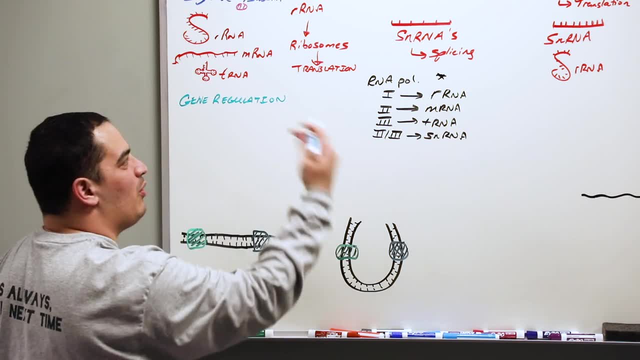 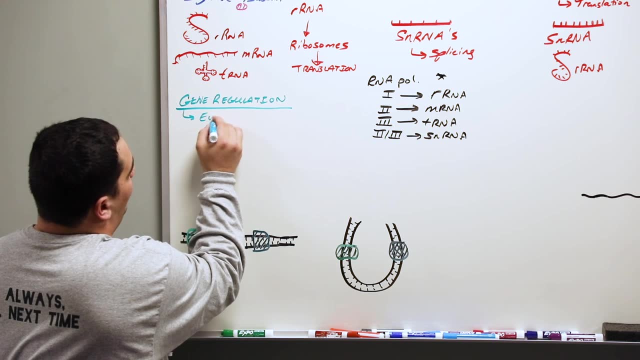 mention this is because this is very easy and it kind of makes sense along with what we've talking about. but we're not going to talk about it in prokaryotic cells. we're primarily going to talk about this gene regulation and eukaryotic cells. we're gonna have a separate video because it's more. 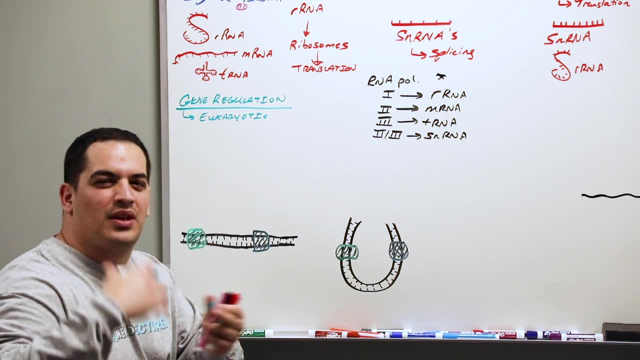 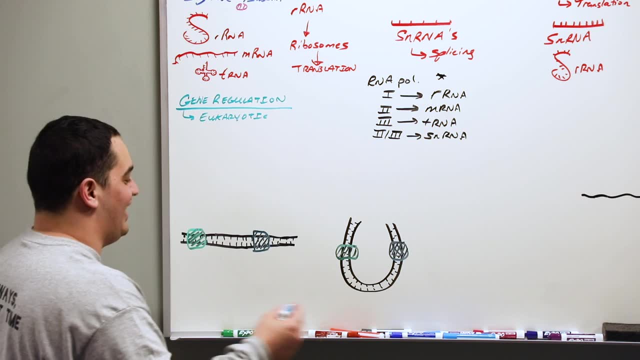 involved. we'll talk about gene regulation and prokaryotic cells with the lac operon and the tryptophan operon. we'll get into that. but in eukaryotic cells there's two ways that we can modulate and it's really easy one way. 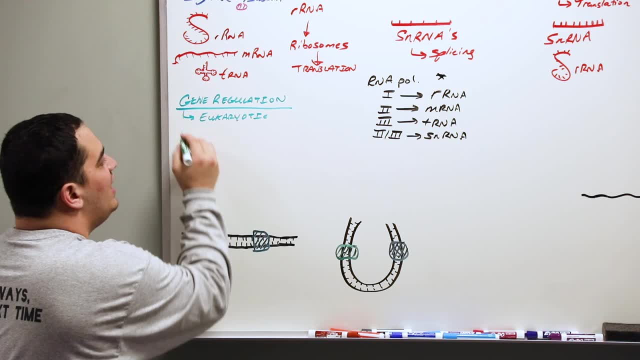 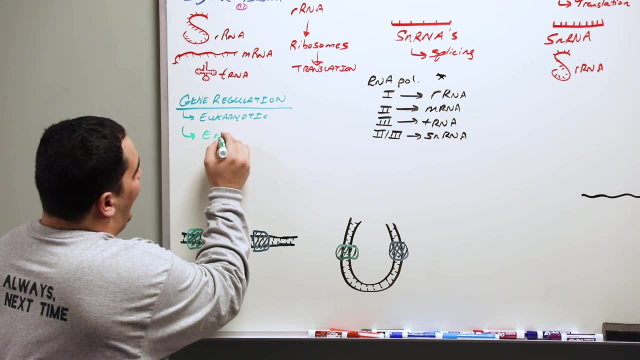 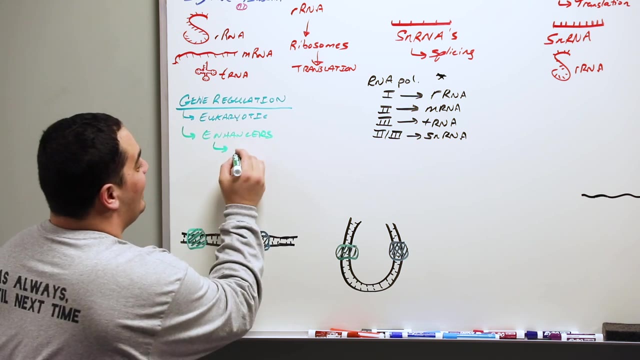 that we can modulate transcription is: we have particular DNA sequences, particular sequences of DNA, particularly palindromic sequences, which are called enhancers, and enhancers are basically DNA sequences. and the big thing I want you to take away from this, they can increase the transcription rate. so they increase the rate of transcription, or 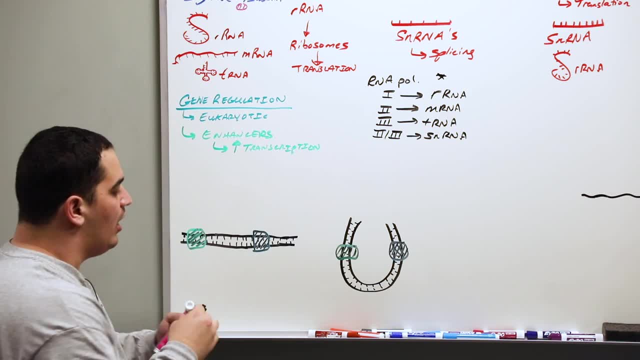 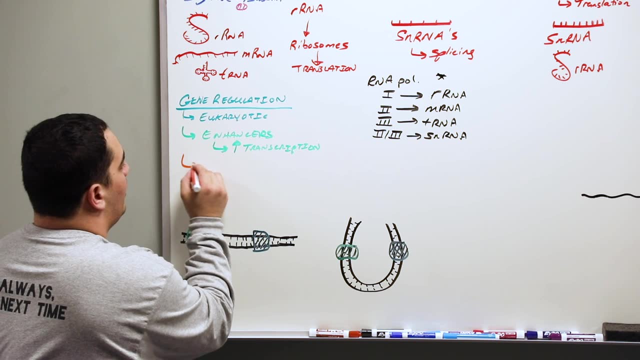 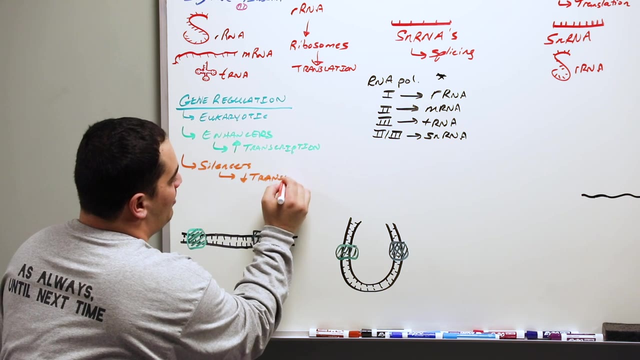 the process of transcription. okay, we'll talk about how they do that. the other thing that can regulate the, the transcription process, or gene regulation in a way, is something called silencers, and silencers they do what: they decrease the transcription rate or the transcription process. now it's. 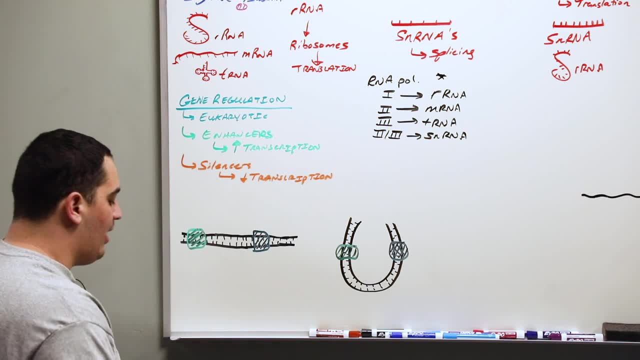 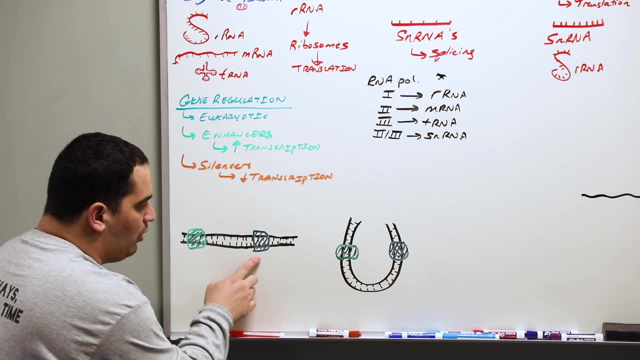 really straightforward. it's relatively simple. let me explain what I mean. let's say: here we have a strip of DNA, we're gonna explain how this happens. so here's our strip of DNA. and remember, this blue region. what did we call this blue region that we talked about above? this was 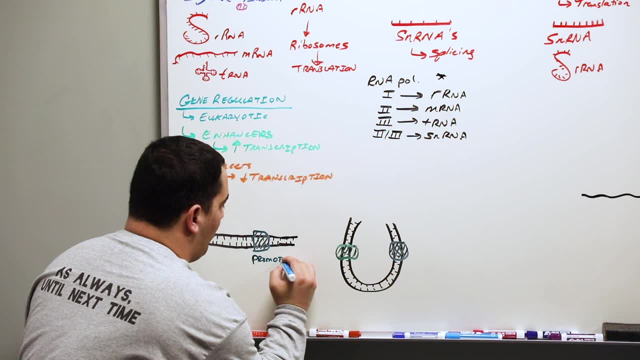 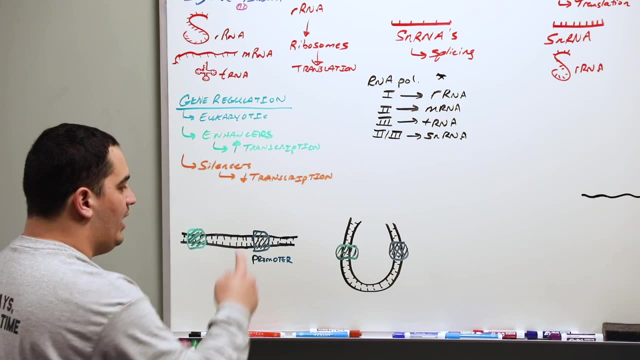 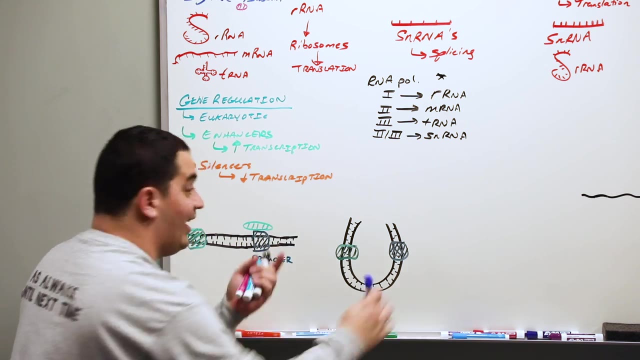 called our promoter region, and do you guys remember- let's take eukaryotic cells in this case- what we needed in order for this process to occur? we needed a particular transcription factor to bind to that promoter region. and then what else did we need in order for that- to read the DNA and make RNA? and then what else did we need in order for that- to read the DNA and make RNA? 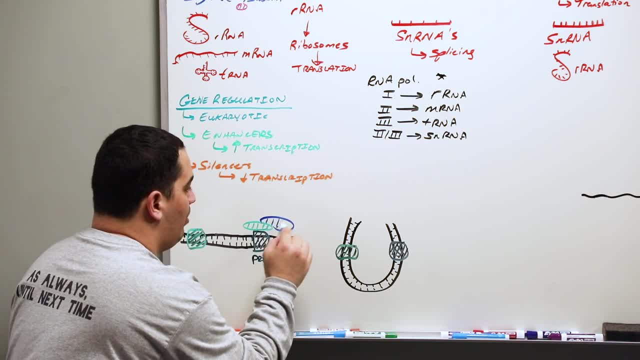 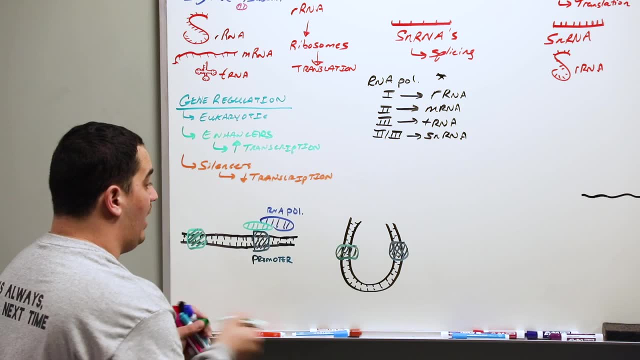 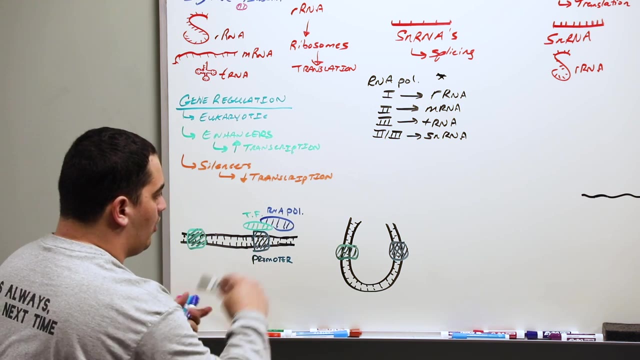 you needed a particular RNA polymerase, right, so we need an RNA polymerase- depending on which one we're talking about would depend on the type of RNA that we want to make- and then a transcription factor. okay, now this is going to go read the DNA. this RNA polymerase will read the DNA, and then 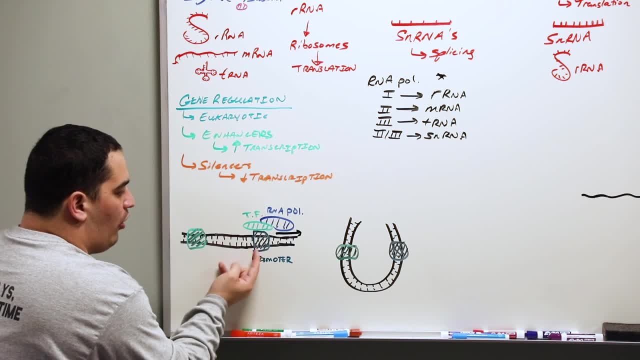 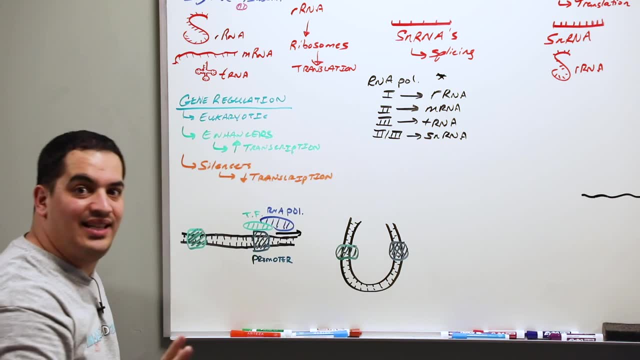 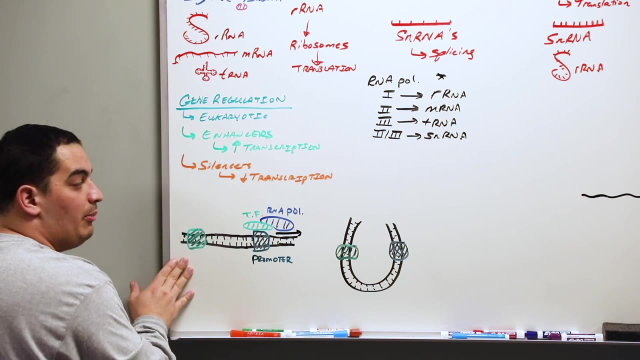 make RNA right now here. let's say that we have the promoter and you can have this enhancer upstream from the promoter, or it could be down here, downstream, where we can't see it in this diagram, but it would be all the way down here, regardless of where it is. it's usually can be close to the promoter or it can. 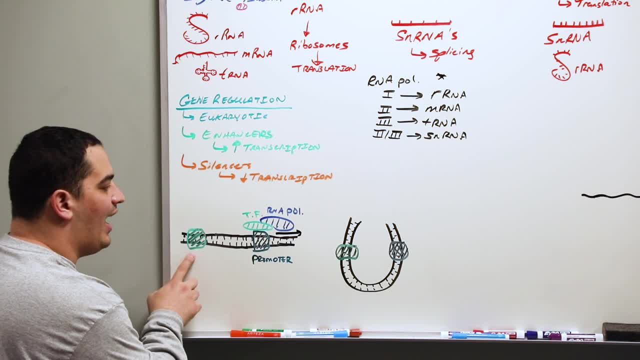 be far to the promoter. so you're probably asking the question: how the heck would an enhancer that's really far away influence a promoter that's all the way down here? how the heck does it do that? there's particular structures, there's different things that can activate. 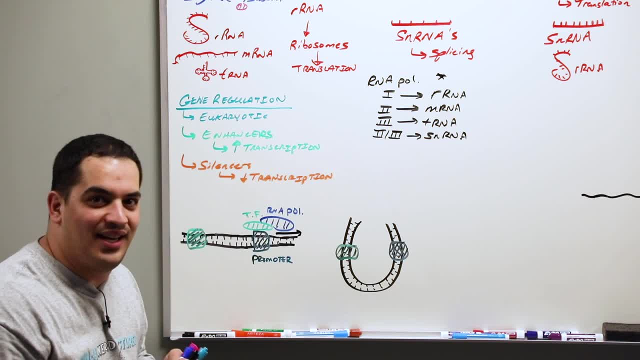 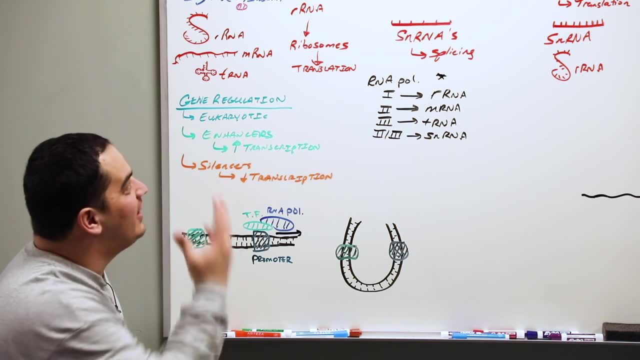 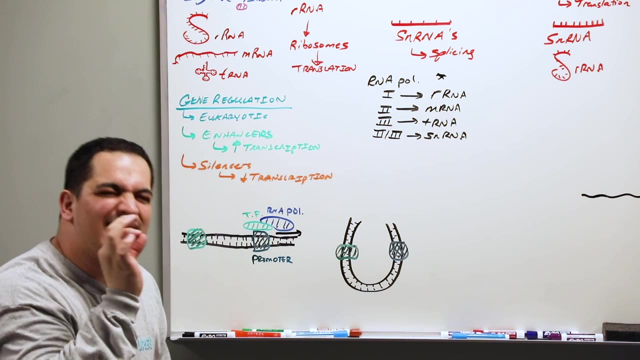 enhancers and cause conformational changes of the DNA, and these are called specific transcription factors- factors. You know why I really frustrate. I got really deep into talking about specific and general transcription factors. The general transcription factors are what bind to the promoter region. Specific transcription factors which we're going to really kind of do a different. 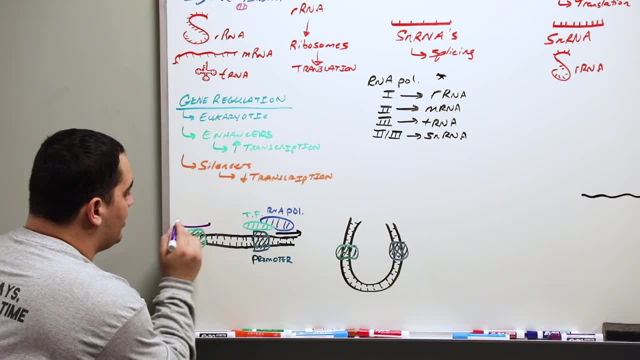 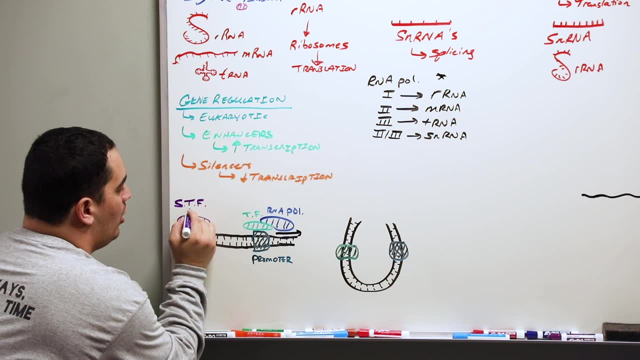 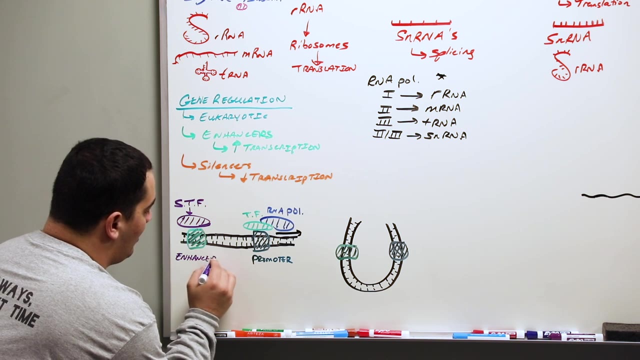 color. Let's do purple. Specific transcription factors will bind to this enhancer region. So let's put specific transcription factors. These will bind to the enhancer. When they bind to the enhancer region, it causes a looping of the DNA to where now the promoter was far. 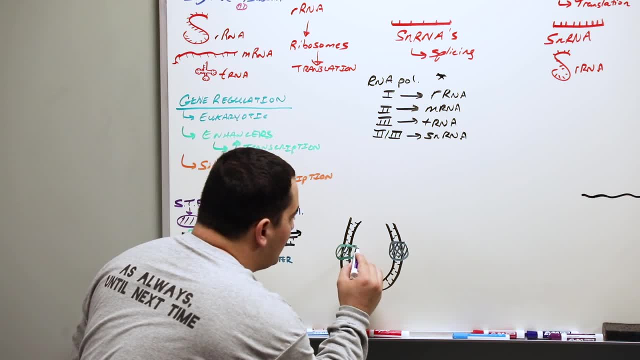 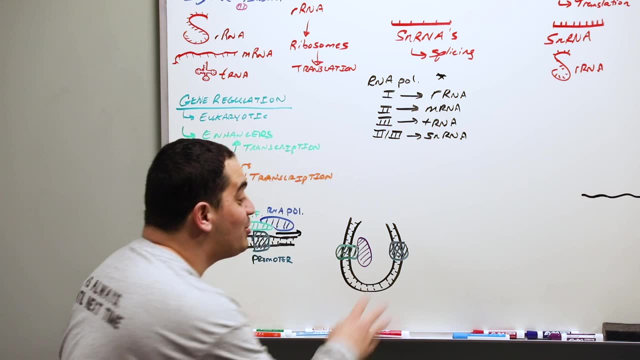 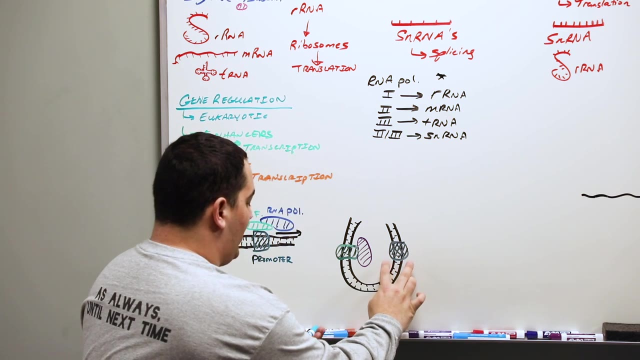 downstream from this enhancer. But when this specific transcription factor binds to the enhancer, it causes the DNA to loop in a way that it's in very close proximity to the promoter region, even though it's far upstream from it. And then what was bound to this promoter region here? 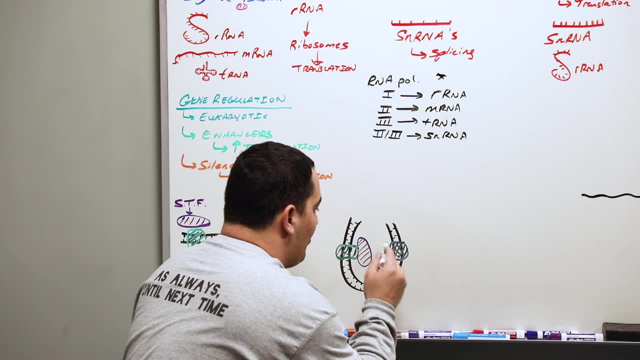 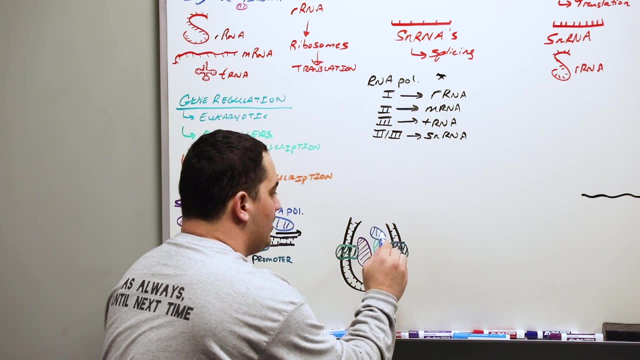 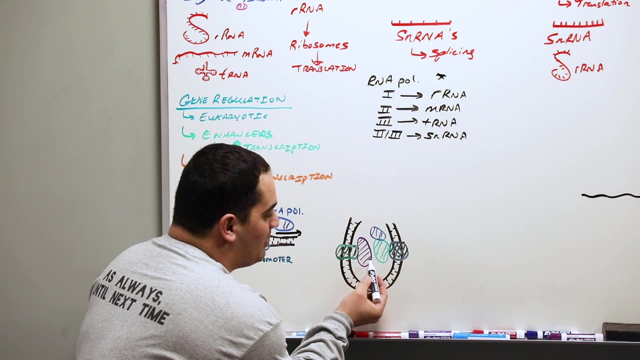 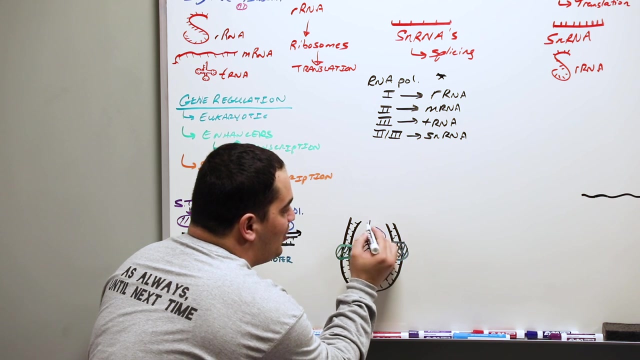 Do you guys remember The general transcription factors And what else? The RNA polymerase? So now that these are in close proximity, guess what this specific transcription factor can do to this area over here. It can act on these proteins and stimulate this reading of the DNA. The RNA polymerase is to read the DNA and 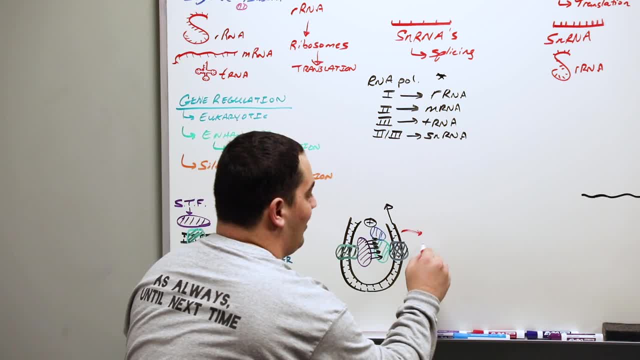 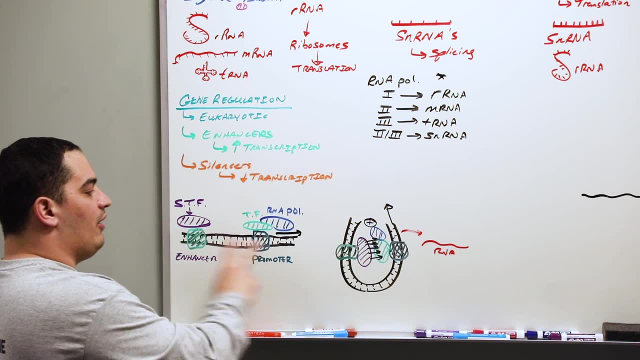 to do what Make a tomoprocess to this Cryo bound RNA, whether it be mRNA, rRNA, tRNA. So the whole point here is that enhancers can be either far upstream or far downstream, which makes it hard to interact with. 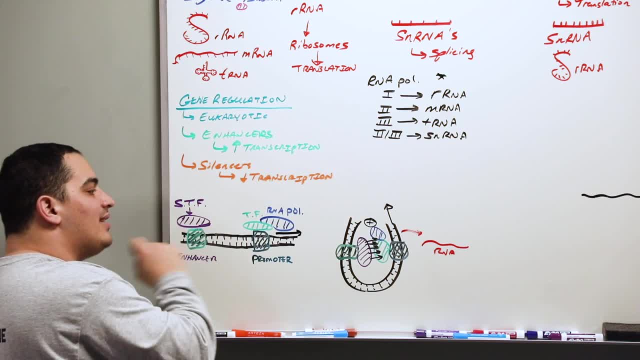 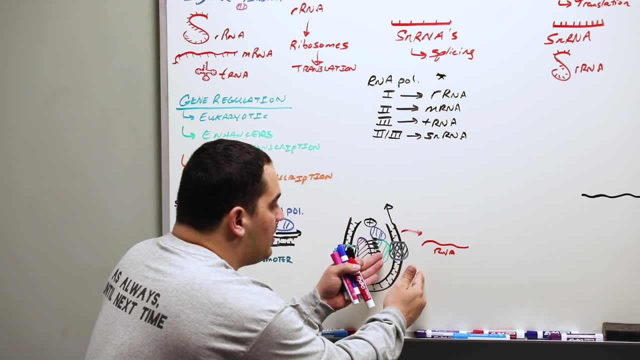 the promoter, But if a specific transcription factor binds to that enhancer, it creates a looping process, bringing it in close proximity, which can then stimulate the specific transcription factors and the RNA polymerases which are bound to the promoter, to increase the transcription of RNA. 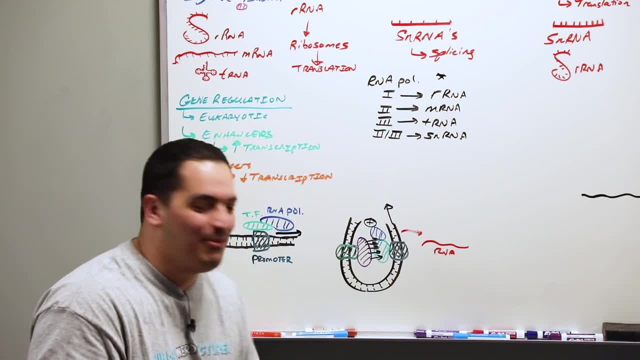 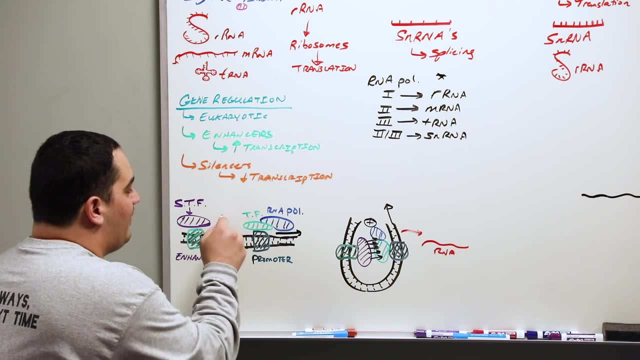 RNA. what do you think silencers do? the exact same process. we're not going to go into detail of it, but if you imagine I did the same thing. I put the silencer here and I have a specific transcription factor that bound here, it's gonna fold. 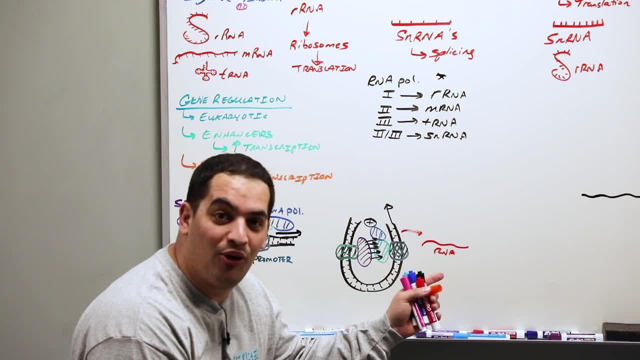 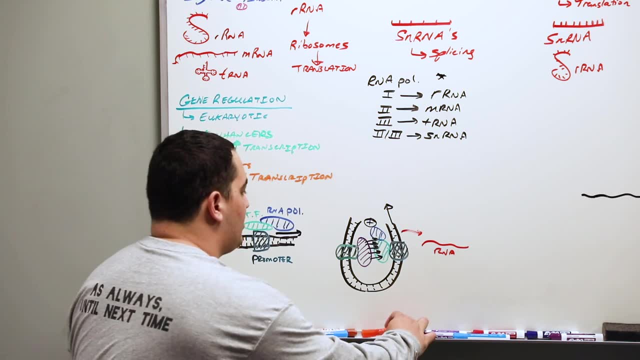 it in a particular way, bringing it close to the promoter, inhibiting that promoter region and slowing down the transcription process. it doesn't make sense. it's pretty cool too, right? so I need you guys to ask yourself the questions, because we're gonna talk about these, these general transcription. 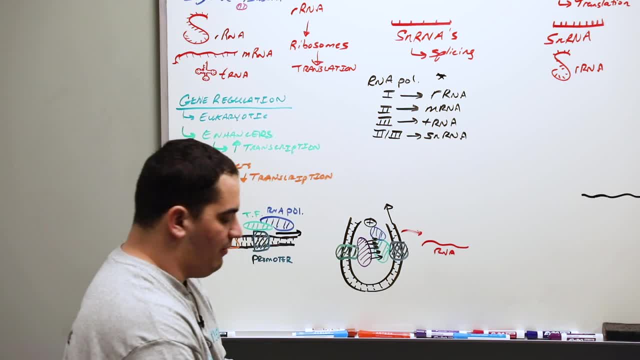 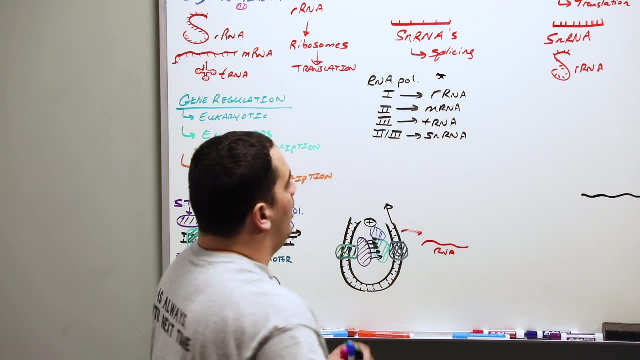 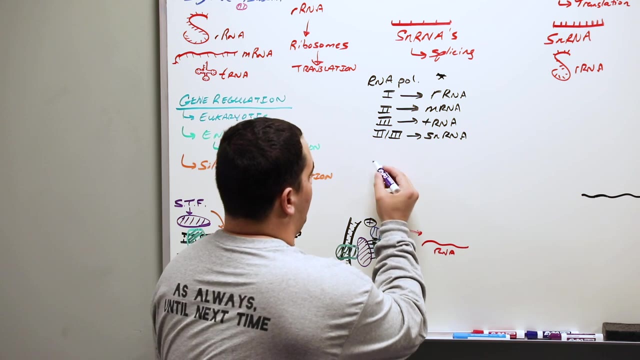 factors. what in the world are these specific transcription factors? and I know that if you guys are the OG ninjas, you'll know these processes in and out- yes, no. when we make a protein, whenever we have like a cell signaling response- we've talked about a million times here in engineered right, let's say that we 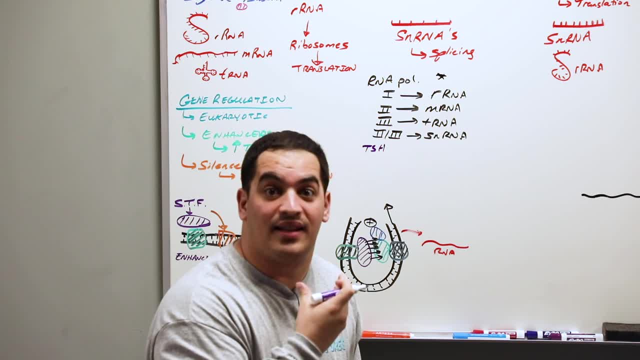 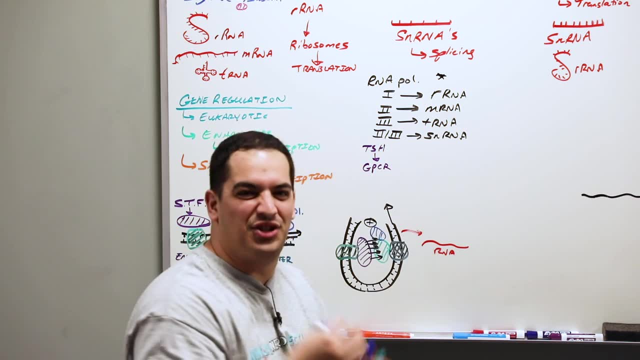 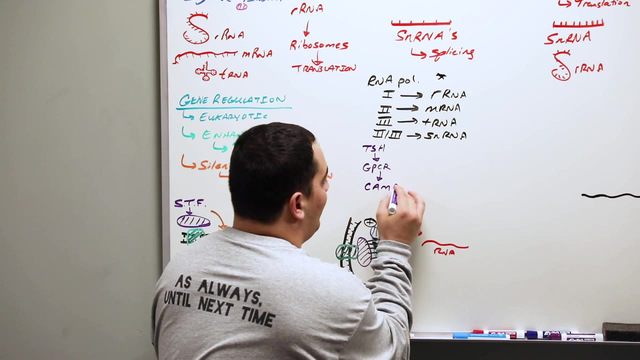 take a hormone like TSH. what stimulates thyroid hormone synthesis? right, TSH will act on a particular receptor. we call these G protein coupled receptors, right like G, C, G stimulatory proteins. those G stimulatory proteins will activate something called cyclic AMP. cyclic AMP will then activate something called: 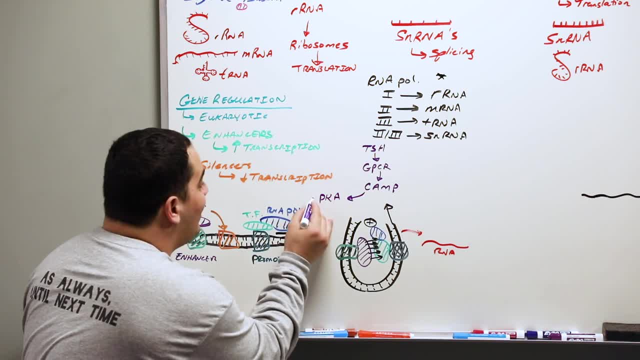 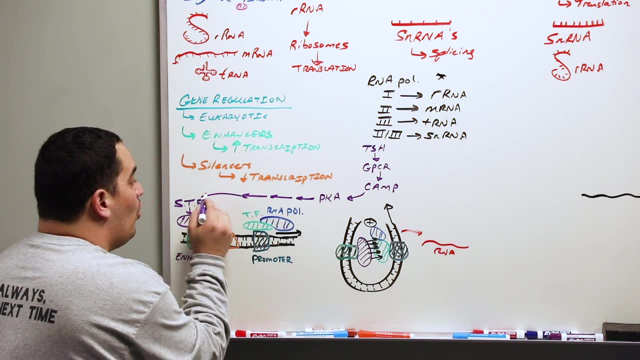 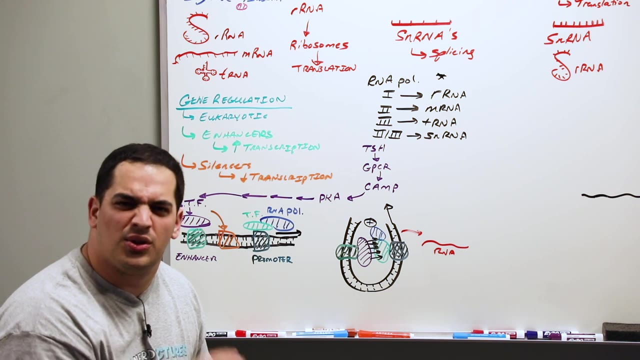 protein kinase. a protein kinase, a, depending upon what type of you know a transcription factor you need. in this case, we're gonna activate a very specific transcription factor for making what? thyroid hormone. so some type of thyroid hormone transcription factor is a very specific transcription factor for the transcription factor that will be needed to bind to the enhancer change. 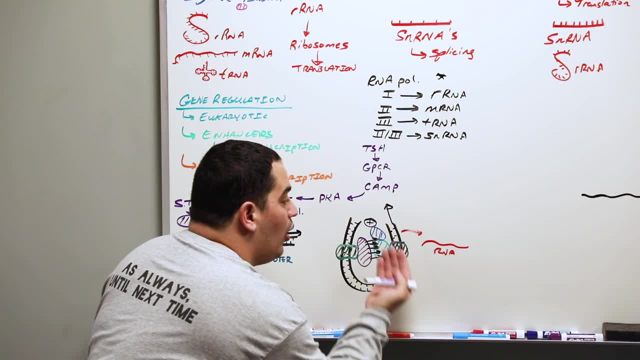 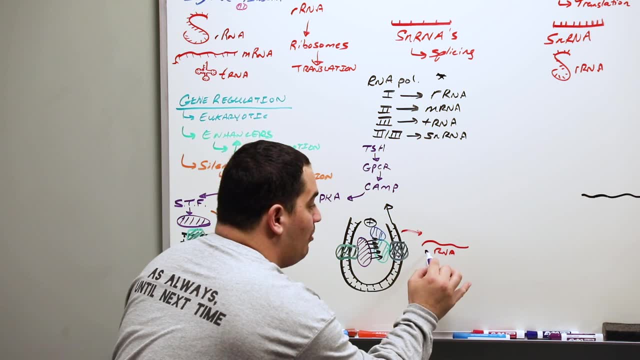 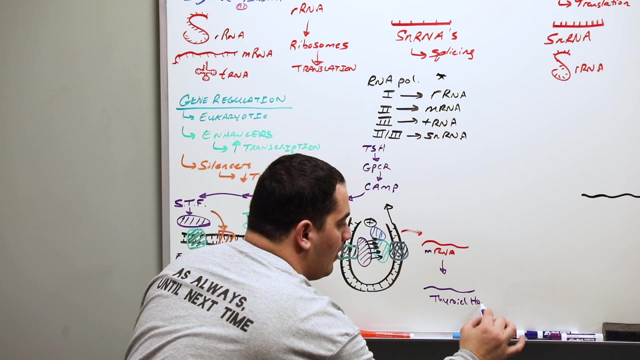 the shape of it, activate the promoter, have the RNA polymerase read the gene that makes what hormone? thyroid hormone. and so you'd have this get read, you'd make an mRNA that would then get translated and make thyroid hormone. doesn't that make sense how that process occurs, so we can increase the? 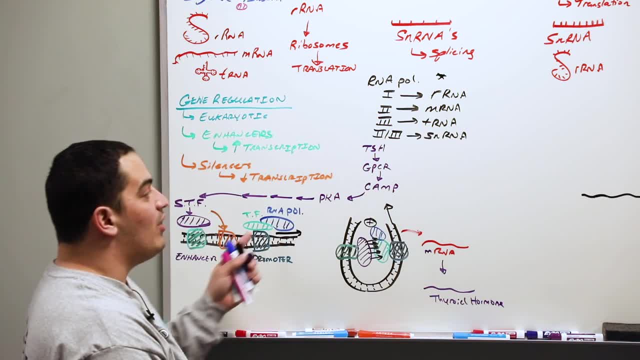 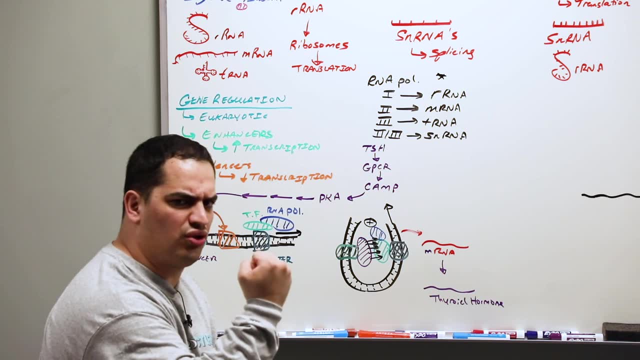 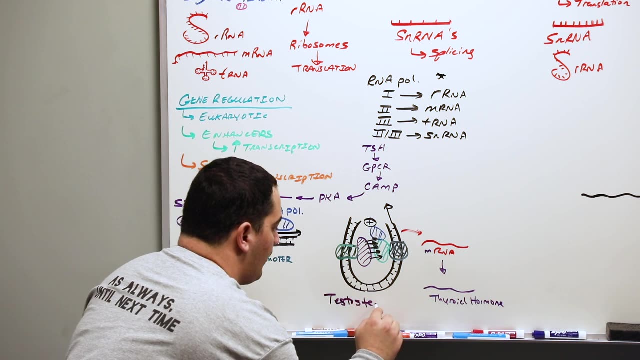 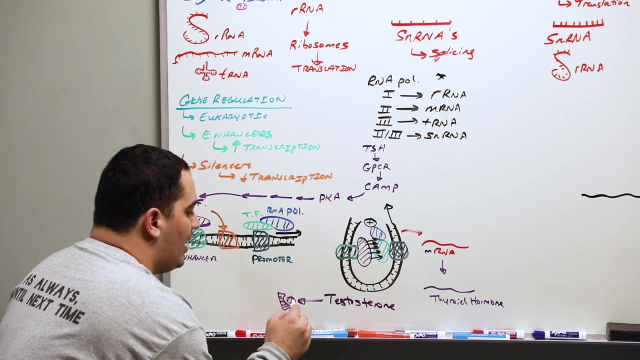 transcription and protein formation of thyroid hormone through this process. the same thing exists with steroid hormones. if I took, for example, testosterone, you guys know testosterone, right? testosterone does what testosterone will move across the cell membrane. it'll bind on to a intracellular receptor. when testosterone binds on to the intracellular receptor, what will that? 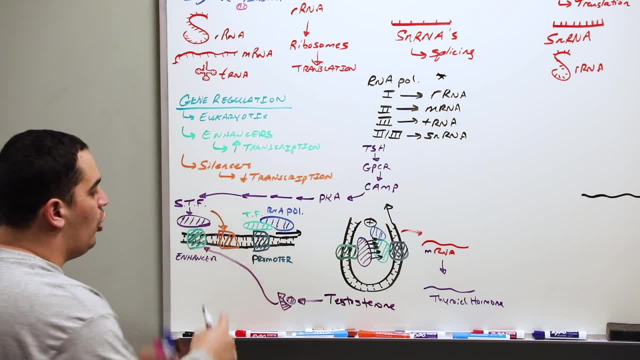 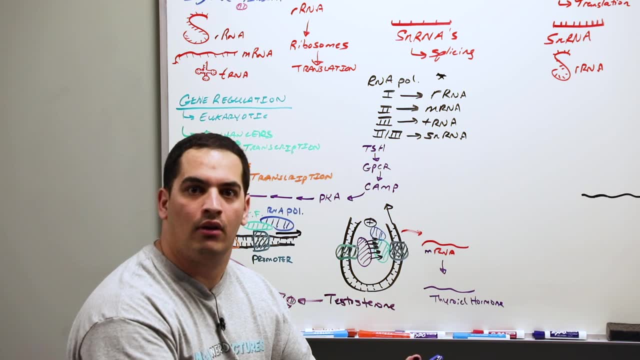 intracellular receptor do bind to the enhancer. when it binds to the enhancer loops, it brings it close to the promoter, stimulates the transcription to make proteins within muscle so that you can get direct right. that's the whole process of how we increase transcription and the same 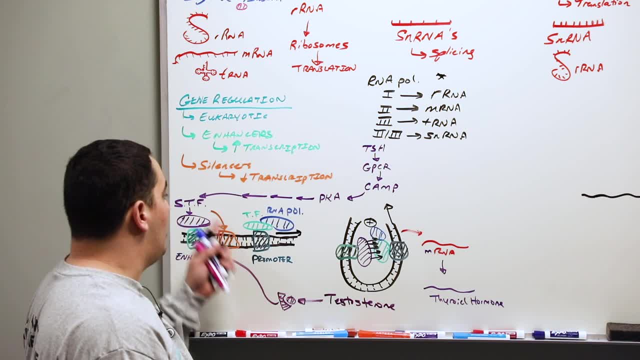 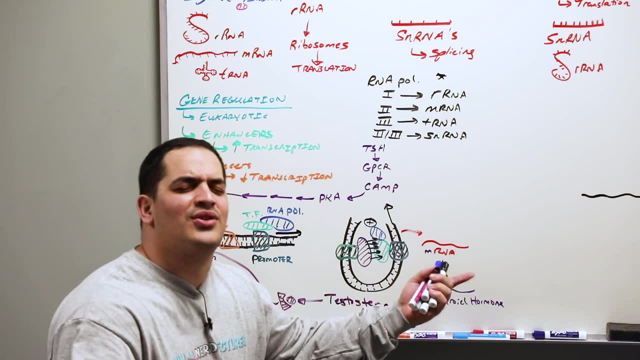 thing would happen if we wanted to decrease it. just we would have some type of repressing transcription factor binding to the silencer that would inhibit the transcription process. so I think we have a pretty good idea now of the basic concepts of eukaryotic gene regulation. now it's been most of our 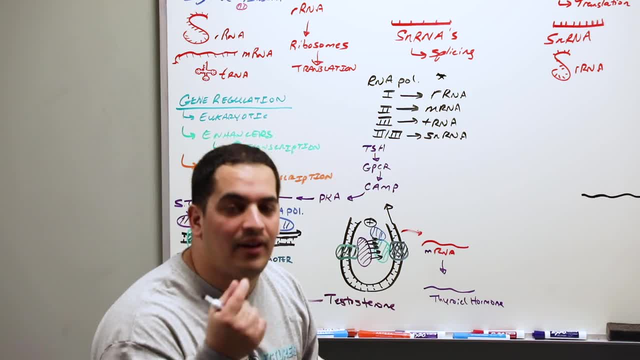 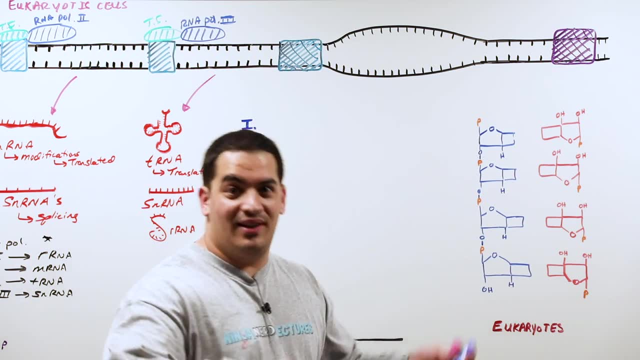 time talking about the transcription, particularly of mRNA. all right, so we're talking about transcription. we've had a basic concept of a right that we need RNA polymerases and transcription factors to read the DNA and make the RNA. but the real one that I want us to primarily focus on, which is primarily 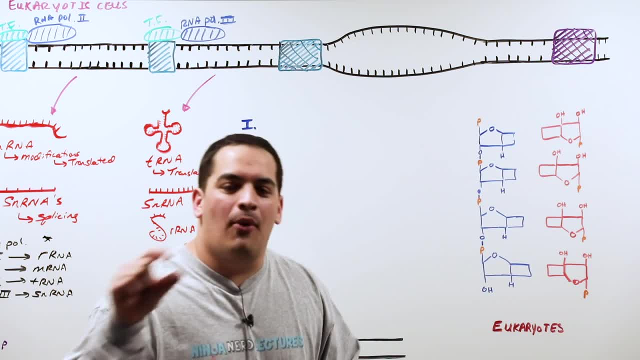 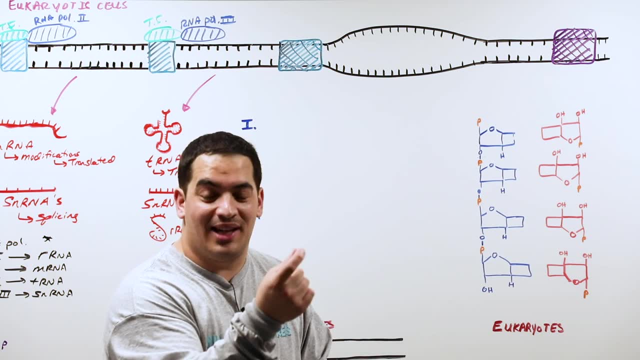 important with transcription of DNA is mRNA. that was the real important one. now, that's in eukaryotic cells. with utilizing the what RNA polymerase type 2, in prokaryotic cells we would just be using the RNA polymerase holoenzyme. so 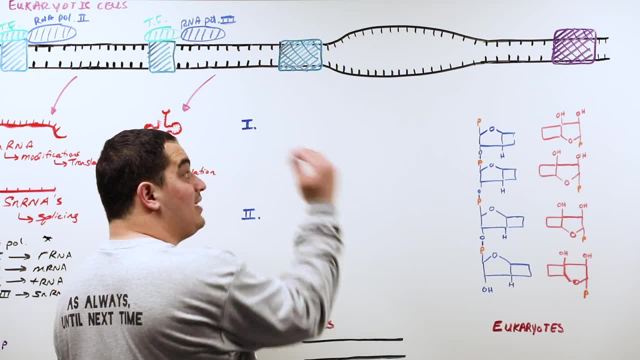 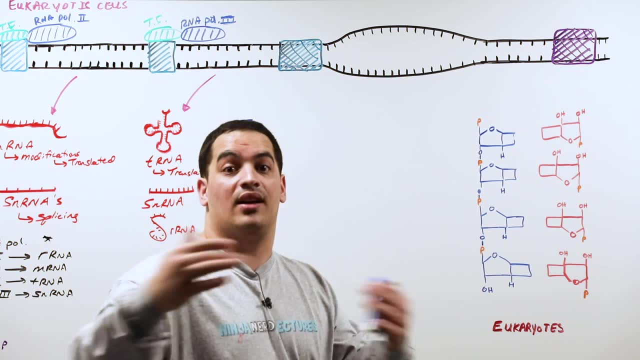 what I want us to do is I want us to go through particularly and more deep. we already have a basic concept of how this is gonna work, but let's go into the stages of transcription, particularly for mRNA within prokaryotic cells and eukaryotic cells. the first stage that is involved here is called initiation of. 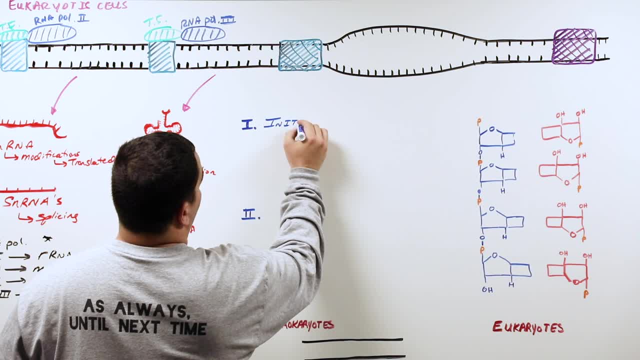 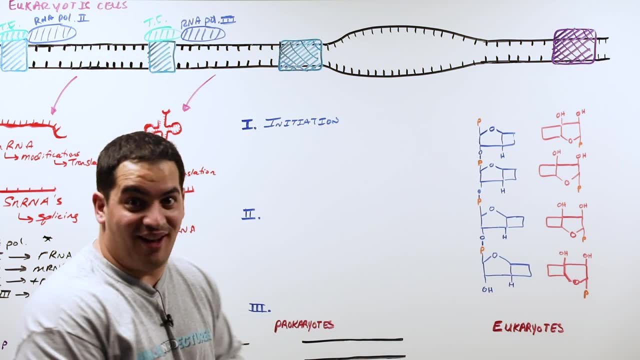 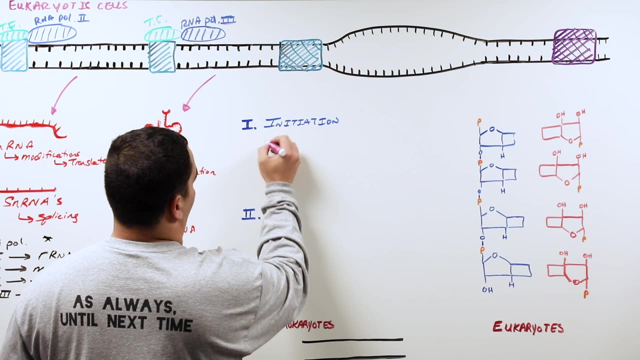 transcription. so the first step that we have to talk about is called initiation of transcription. now, this is the part that we've pretty much already familiarized ourself with. okay, now, within this, let's have our two cells. okay, that we're gonna do initiation with. 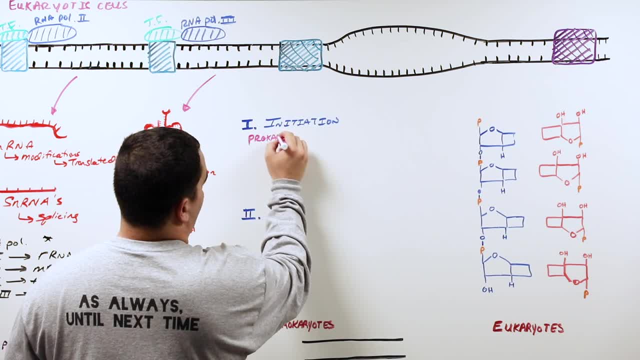 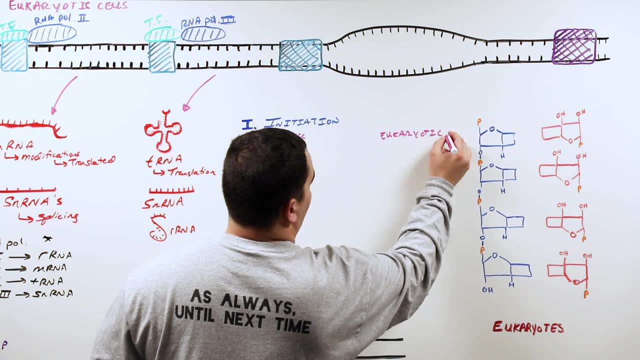 We're gonna have our prokaryotic cells here on this left side of the board and then over here we're gonna have the eukaryotic cells here on the right side of the board. What I want us to do is to have kind of a comparison. 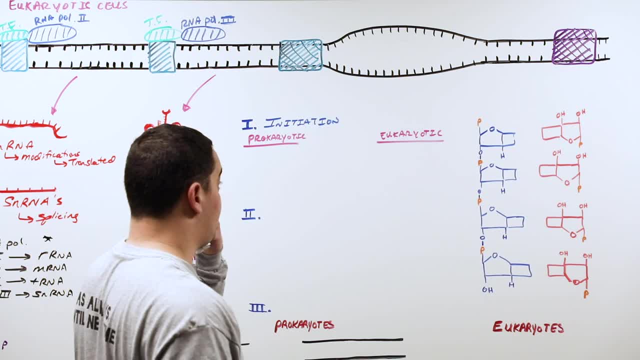 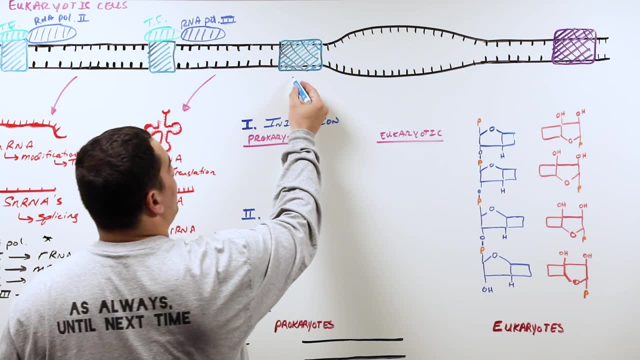 a side-by-side comparison of the initiation process. The first thing that we need to know is: we've talked a little bit about this already, but this blue region, what did we call this blue region? here again, This blue region was called the promoter region. 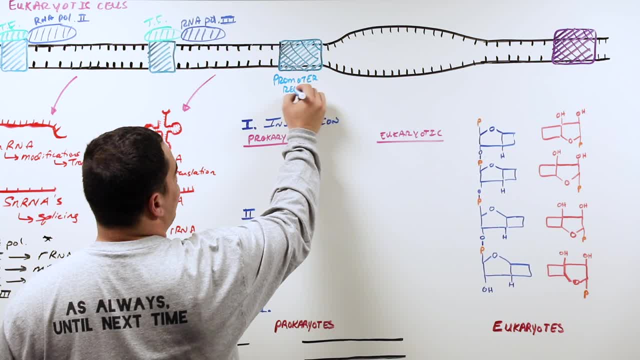 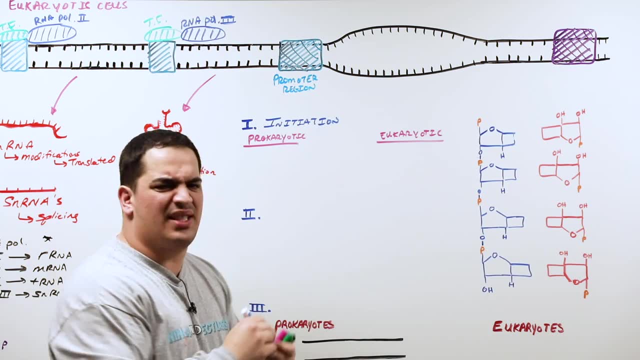 Now, the promoter region, I told you, is a particular kind of like nucleotide sequence that is very, very specific and allows transcription factors and RNA polymerases to bind to the DNA. It's kind of a signal, if you will. It's like, hey, here I am, come bind to me. 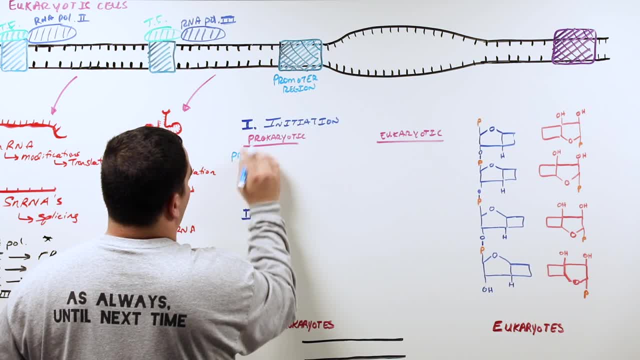 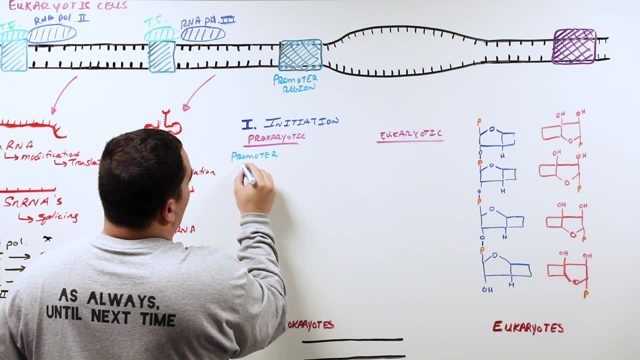 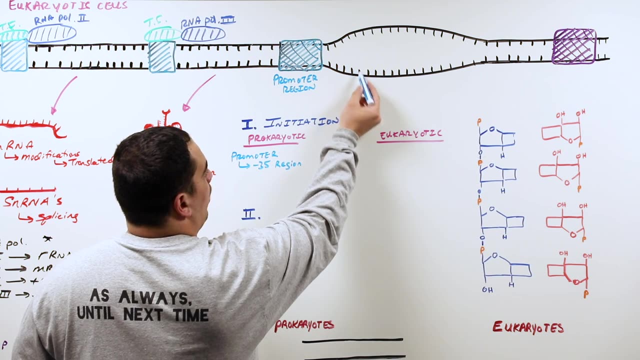 In prokaryotic cells the promoter region has particular types of like names and just weird stuff that they can ask you in your exams. So in the prokaryotic cells they call this the negative 35 region, which means from the start point. 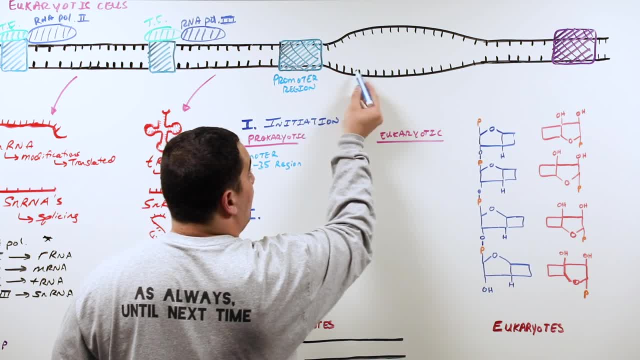 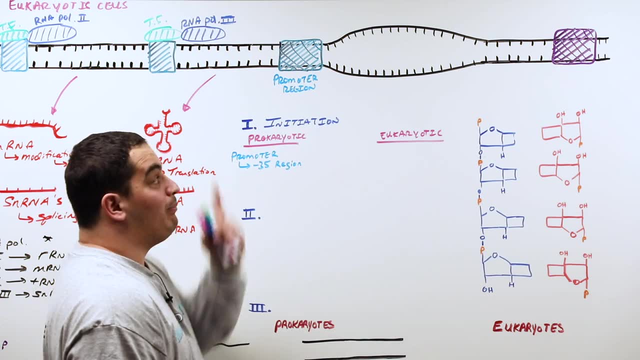 at which the RNA polymerase starts reading the DNA and making RNA. if you go back 35 nucleotides, that's kind of the point at which the RNA polymerases will bind in prokaryotic cells. Another one is called the negative 10 region. 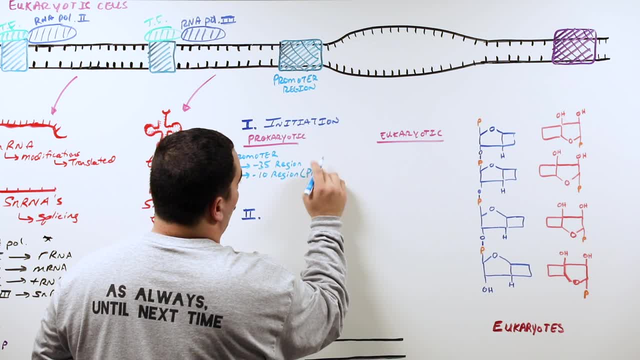 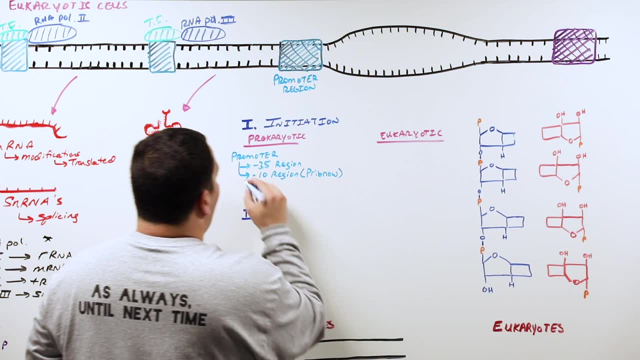 but they wanted to give this one a name, So they called it the pribno box, just meaning that it's negative. it's 10 nucleotides away from that start of transcription Right. And then the last one here is called the plus one region. 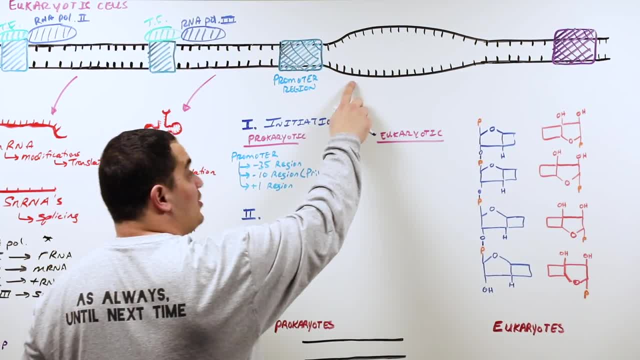 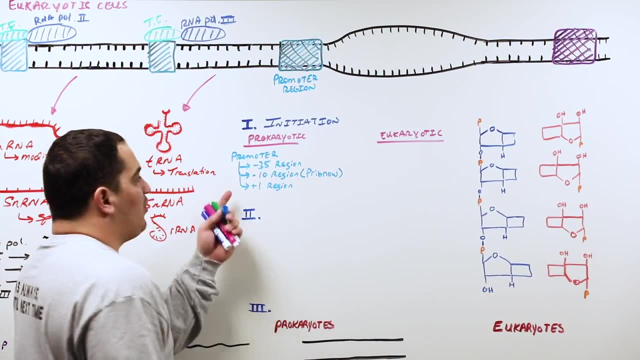 which is also called the transcription start site. So it's gonna be pretty much the nucleotide at which you just read and start making the whole process of RNA. So these are the regions that you guys need to remember within prokaryotic cells. 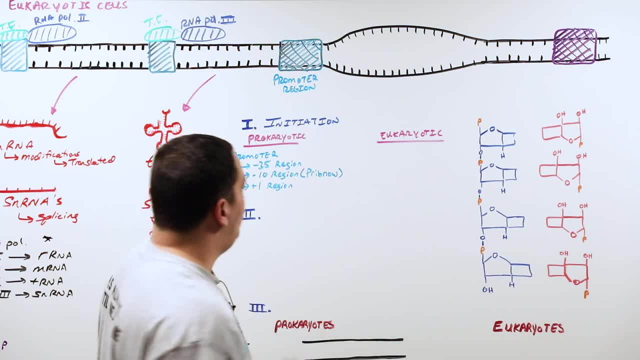 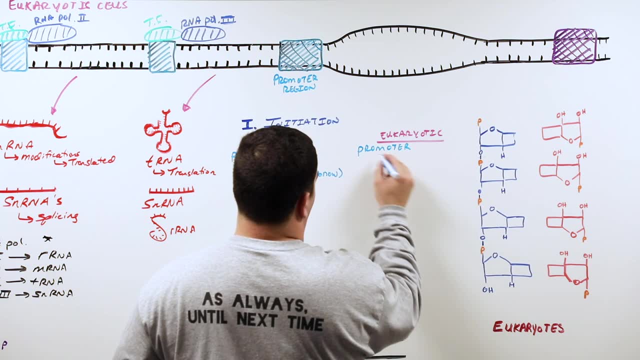 These are the kind of specific promoter regions And eukaryotic cells. the promoter regions have particular nucleotide sequences that we need to be aware of. These are called the TATA box, which means that you would have thymine adenine, thymine adenine. 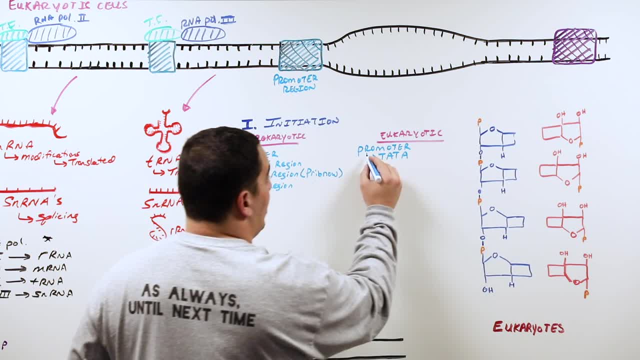 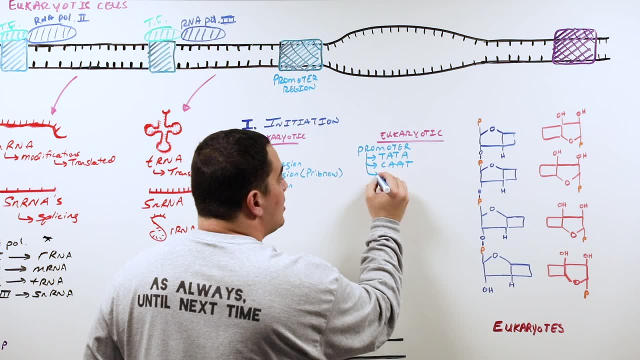 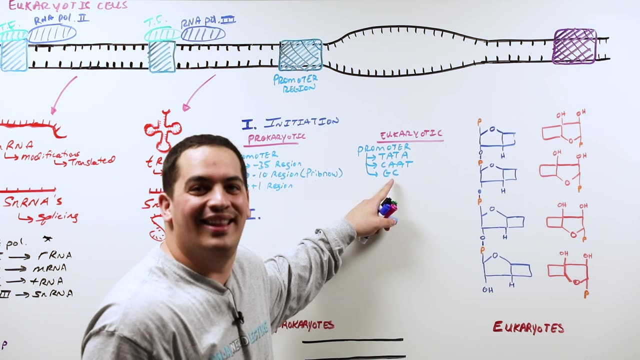 That would be a particular recognition sequence within the promoter in eukaryotic cells, Or CAT C-A-A-T, So cytosine, adenine, adenine, thymine, And the last one is a GC box. So if there's a TATA box, a CAT box or a GC box, 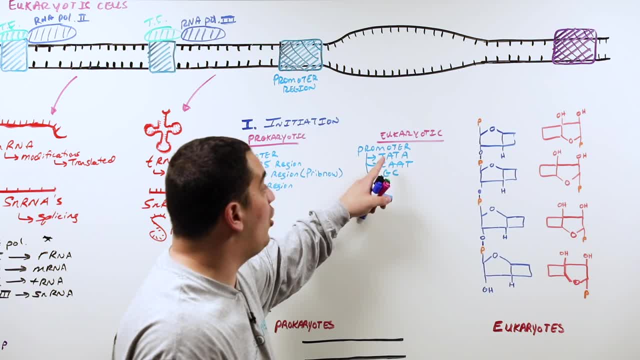 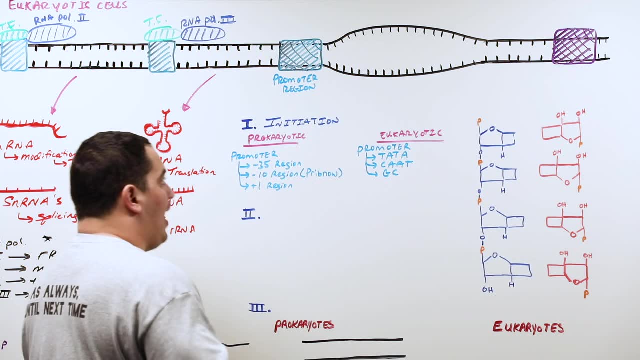 these are identifying nucleotide areas at which the RNA polymerases type two and transcription factors will bind to. That is the important thing, okay, Now the next thing here is the polymerases: The RNA polymerases within prokaryotic cells. 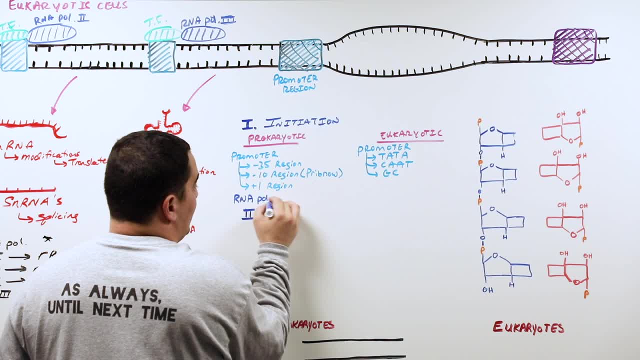 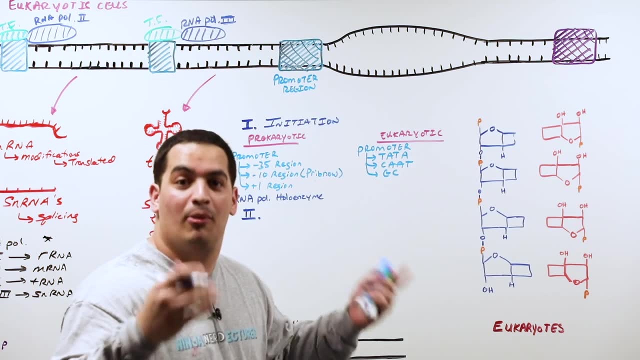 it's just one. It's RNA polymerase, holoenzyme- right, We already kind of talked about that- With the core enzyme two- alpha, beta, beta, prime, omega and then the sigma subunit. All of that's needed to bind to the promoter region. 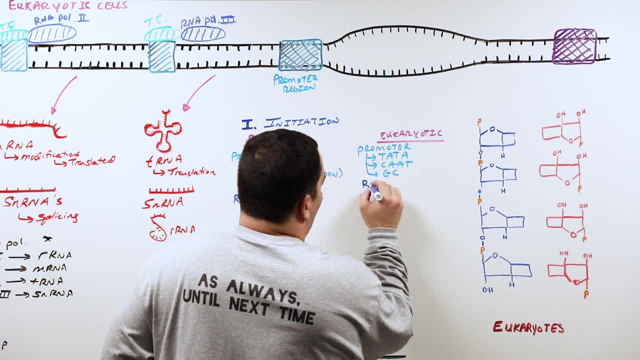 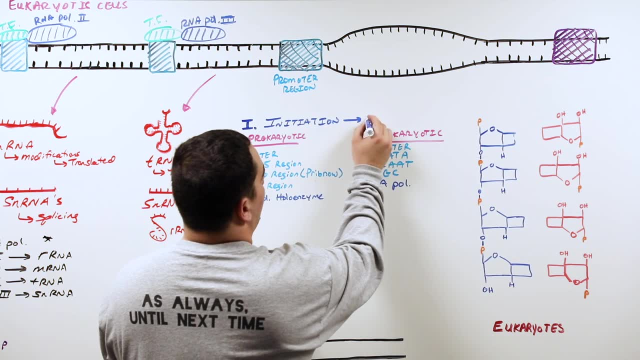 And eukaryotic cells is a little bit more right. We said that we needed two things. We needed an RNA polymerase, And what are we making here? Initiation, and we're gonna say that we're trying to make what? 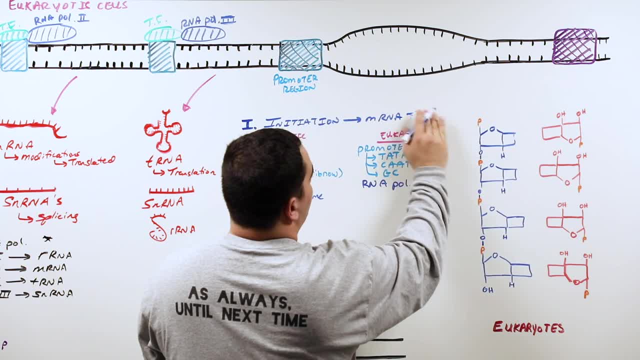 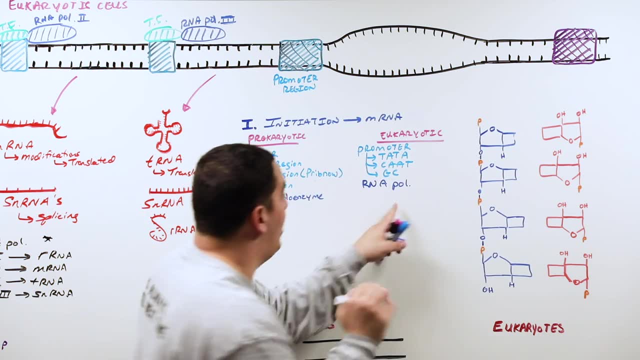 We're trying to make mRNA transcription. So we're doing transcription, but we're making mRNA. So what was the particular RNA polymerase? One, two, three, R, M, M is for the mRNA, So RNA polymerase type two. 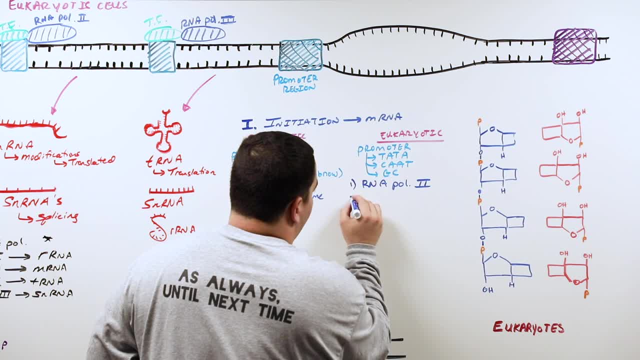 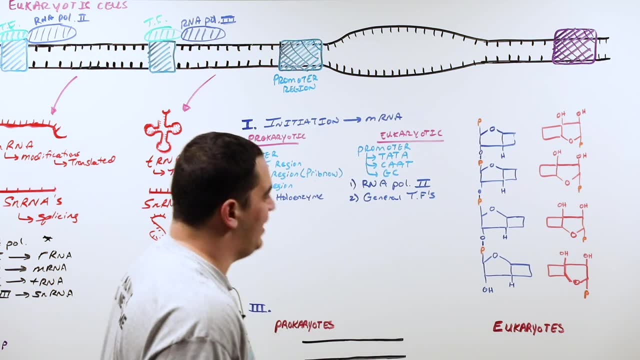 is one of the things that I need. The second thing that I need is the general transcription factors, and there's just so many of these that I don't know how important and how specific we really need to go into these. I'll give you some of them, but I just want you to know. 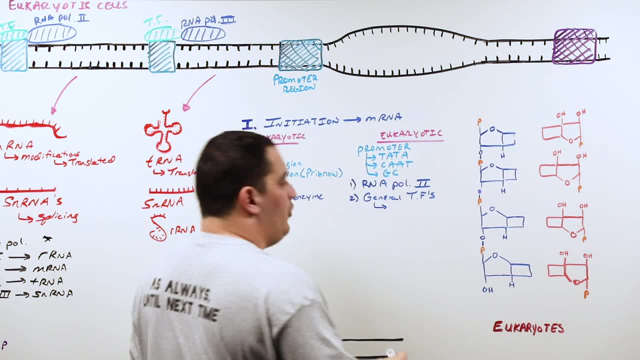 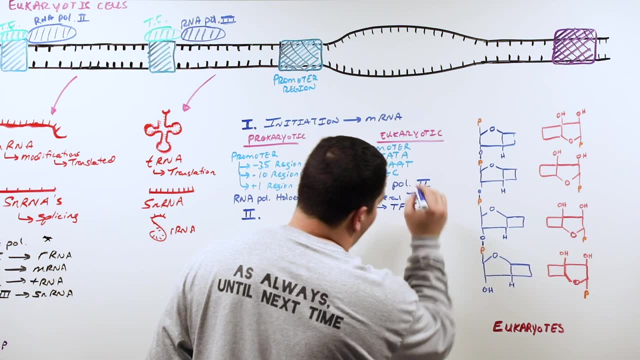 that there's so many different types of them. The main one. if you had to remember one specific out of the tons of them, I want you to remember transcription factor 2D. This is the one that I really want you to remember. 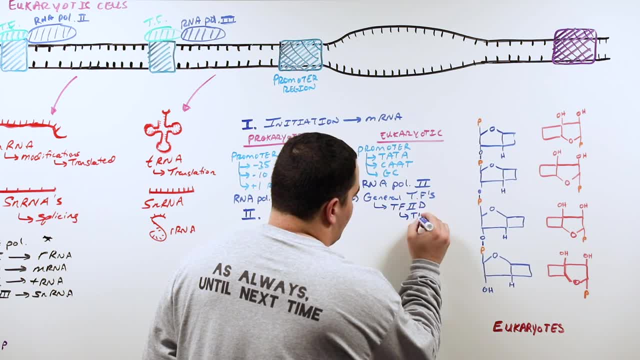 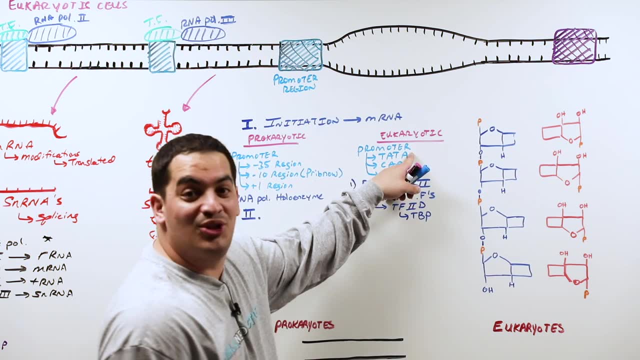 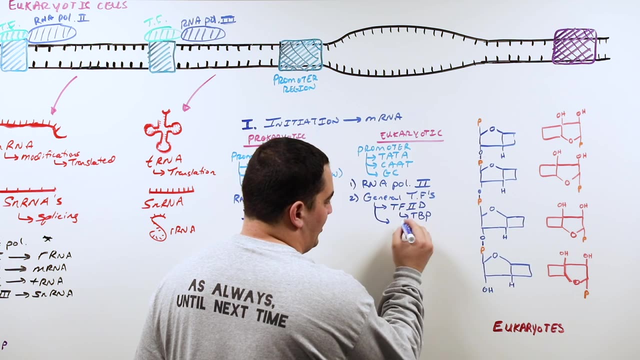 And the reason why is this contains a structure called the TATA binding protein. So this transcription factor 2D has a particular protein portion which binds to the promoter region, the TATA box. But there's many other transcription factors And you can remember these by transcription factor two. 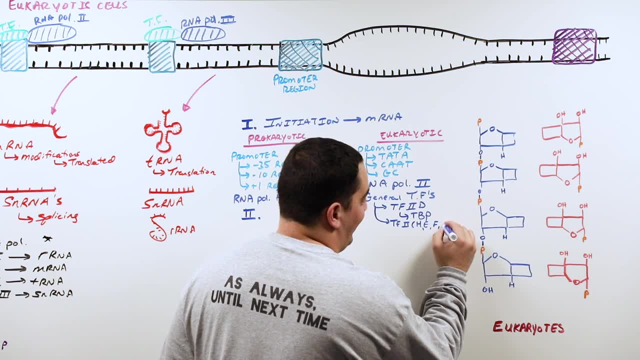 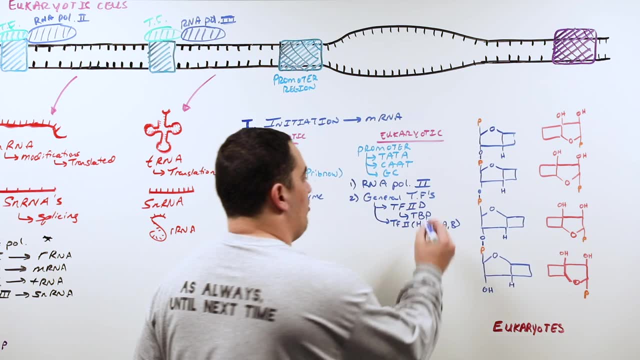 and they can be H, they can be E, they can be F, they can be A, they can be B. So there's tons of these dang things, So I don't know how important it really is to know that, but the main one I want you to remember. 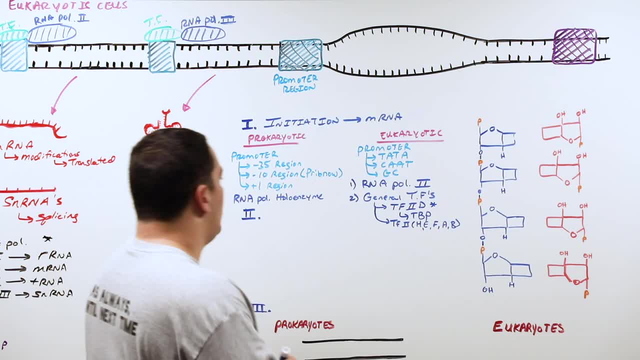 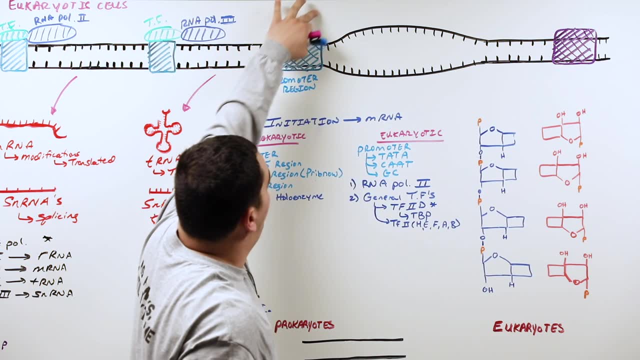 is the transcription factor 2D, All right. so these are the things that we need in order for initiation to occur. So let's take, for example, we're gonna have on one side eukaryotic cells. the eukaryotic enzymes will bind. 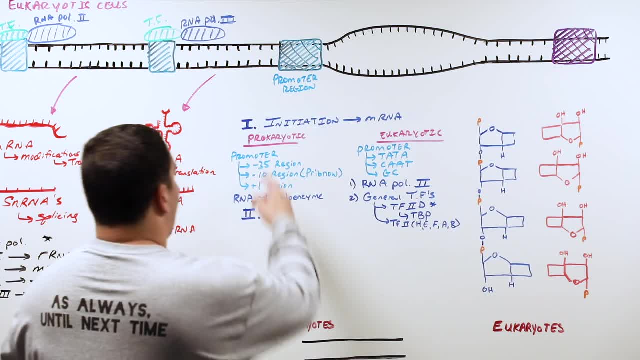 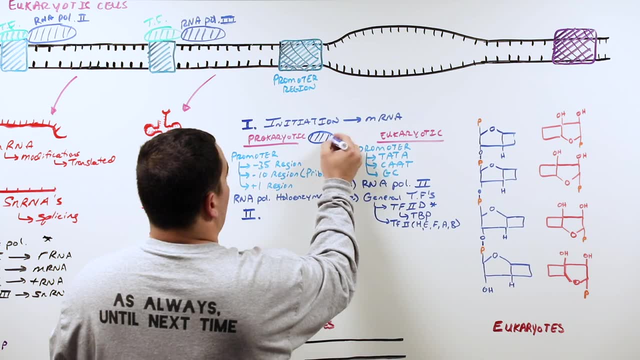 and on this side the prokaryotic will bind right. So let's say, here we take, for example, we'll make this prokaryotic RNA polymerase, we'll make this one blue and we'll make the RNA polymerase over here. 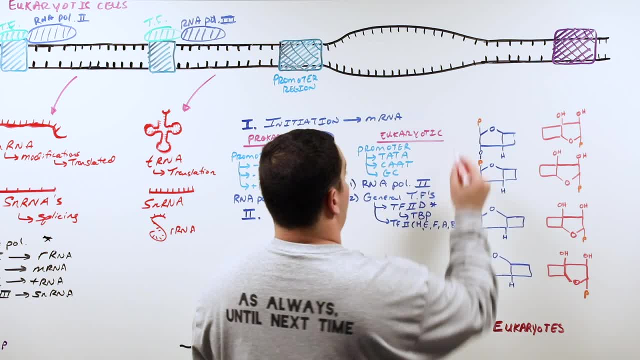 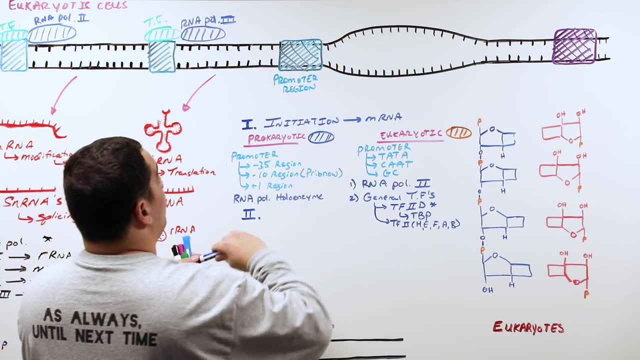 for the eukaryotic cells. just for the heck of it, we'll make it orange, okay, just so we can distinguish the difference between these. So what will happen? This whole RNA polymerase holoenzyme will do what Bind to the promoter. 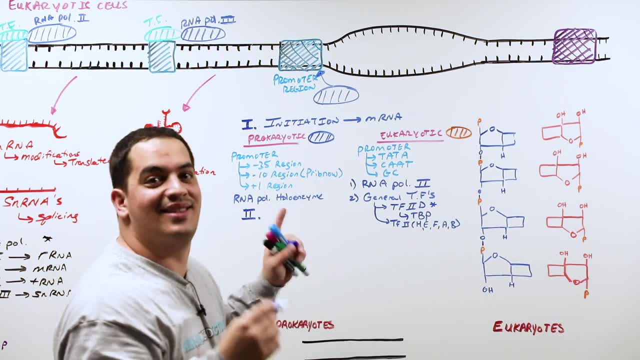 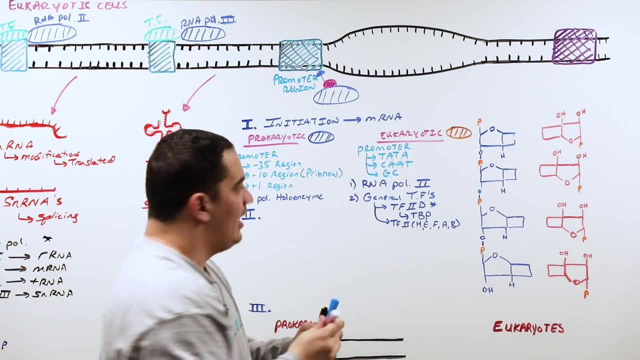 What will allow it to bind What subunit of it, The sigma subunit? And if you really wanted to go back, if you guys remember we made that pink. okay, For the eukaryotic cells. what do we need? 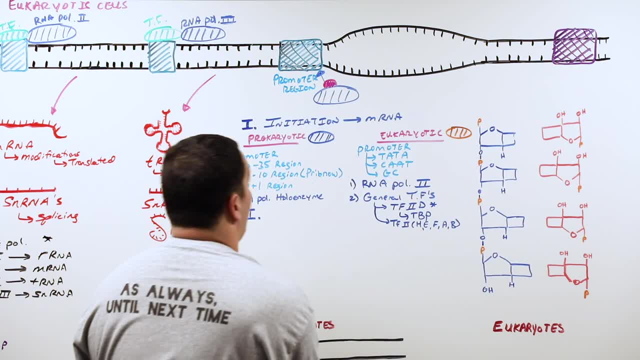 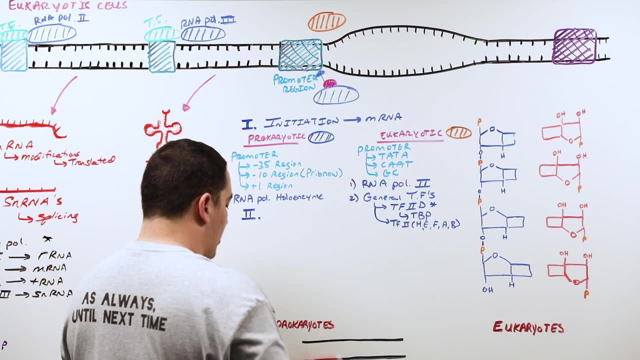 We need the RNA polymerase type two. We said we're gonna represent that with orange, So here's going to be the RNA polymerase type two. and then what else do we need? We need those general transcription factors. There's a bunch of them, but what's the particular one? 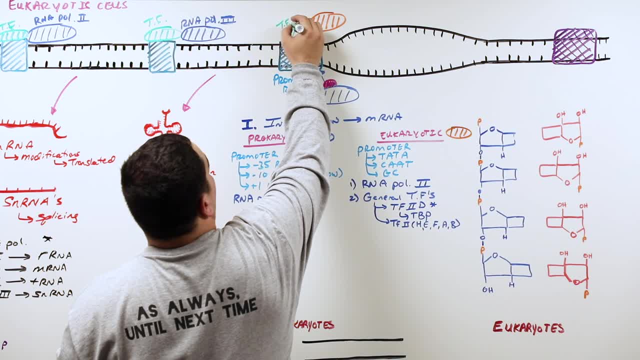 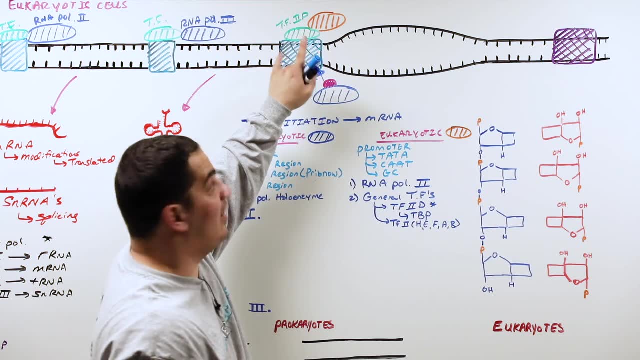 that I really want you to remember here. Transcription factor 2D, which contains the TATA binding protein, So it binds to the TATA box, which is a promoter region in the eukaryotic cells, then allows the RNA polymerase 2,2 bind to the DNA. 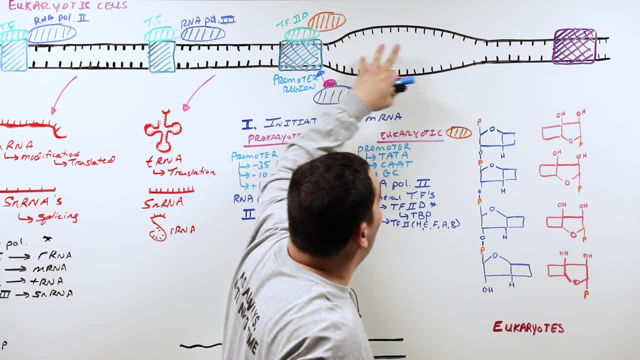 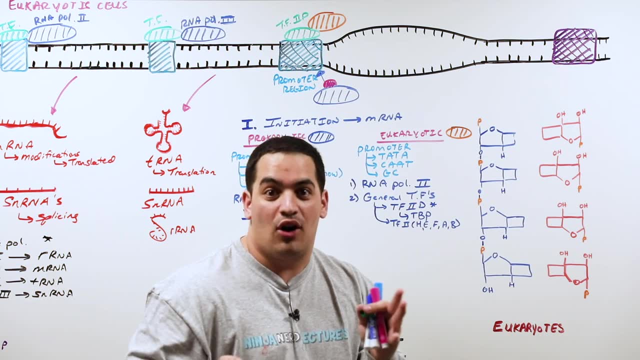 Now, once the RNA polymerase is bound to the DNA, it's gonna start moving down the DNA strands, reading it and making RNA. So we've now started the process of transcription. That's all that's happening here. The next step is that, once we've bound, had this RNA, 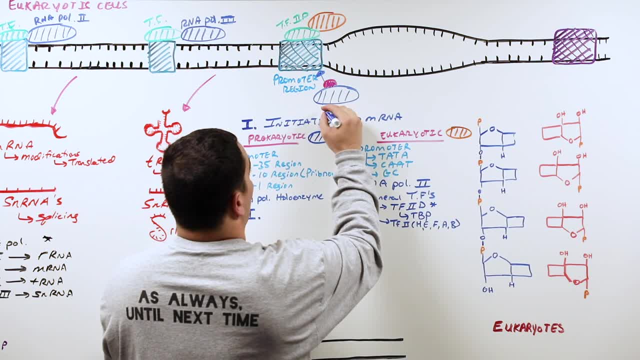 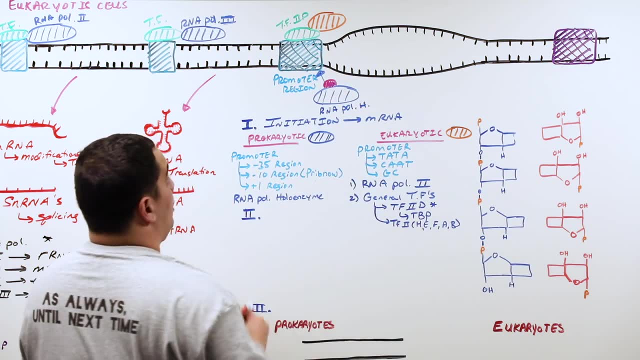 so let's write these down here. for the prokaryotic cell, this would be the, we'll put RNA polymerase and we'll put H for the holoenzyme And for that one up here, this is gonna be RNA polymerase type two, right? 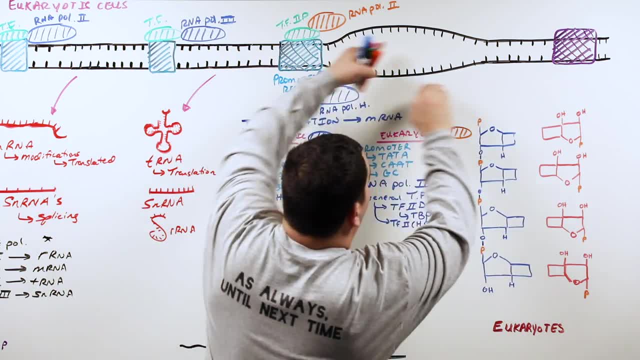 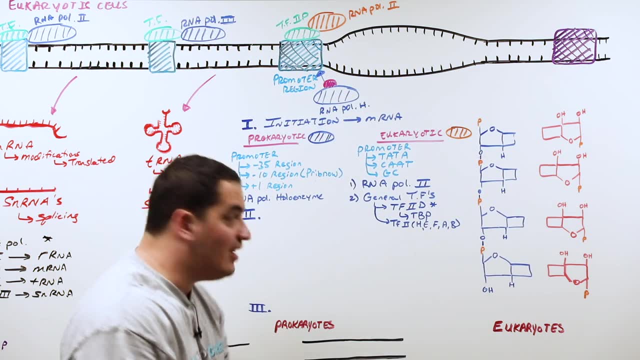 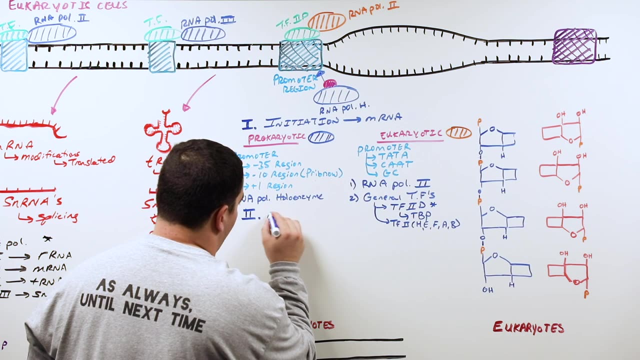 Once this is bound and it's in the DNA, it's gonna start reading the DNA. As it reads the DNA, it'll make mRNA. That process by which it does that is called elongation, So let's write that down now. So the next step is elongation to make the mRNA. 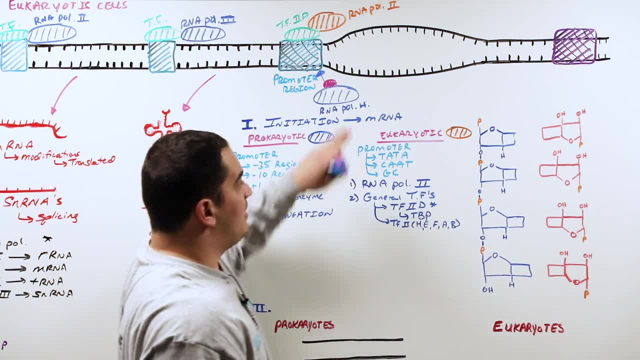 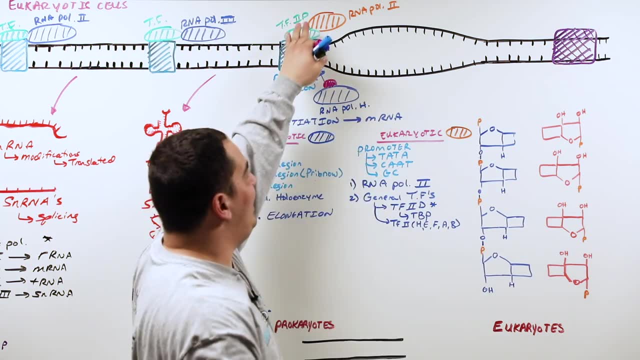 Now, within elongation, a couple different things happens, And this is thankfully the same in prokaryotic cells and eukaryotic cells. so thank the Lord for that right. So let's just say that we take either one of these RNA polymerases. 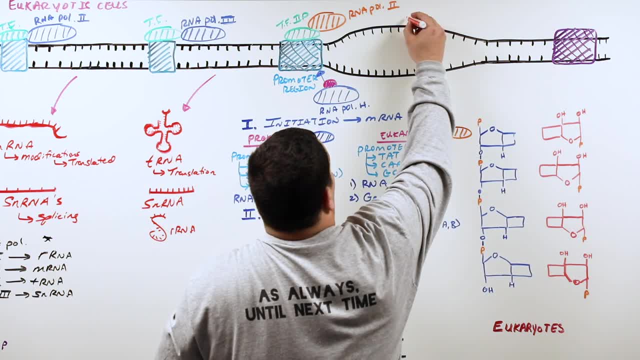 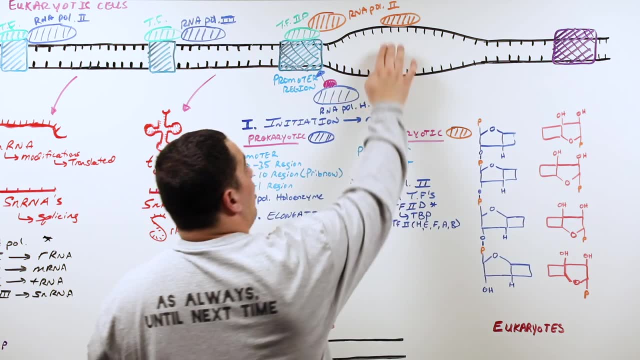 Let's just for the heck of it. we'll say: here's your RNA polymerase two. okay, Here's your RNA polymerase two. and it's reading the DNA. The DNA we already know has two strands. We're gonna call this top strand here. 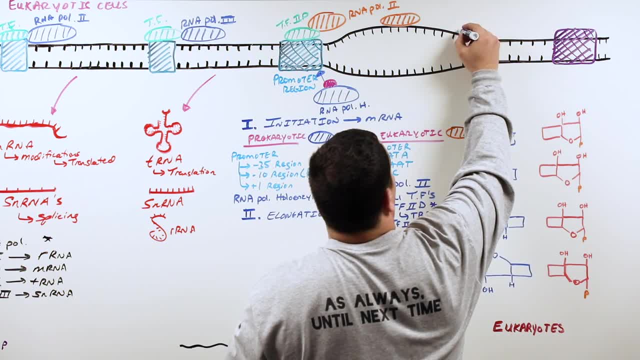 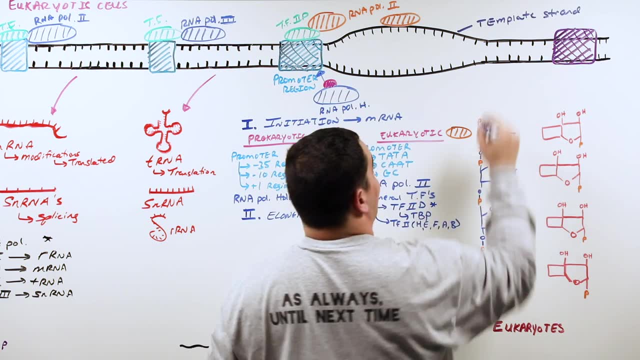 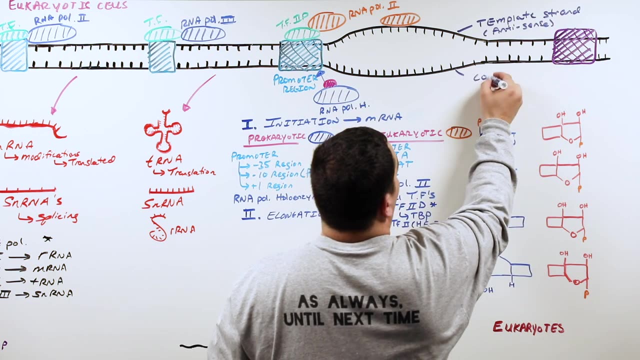 this top strand, son of a gun. this top strand up here, we're gonna call this the template strand. So the template strand, Also sometimes referred to as the antisense strand, This strand down here we're gonna call the coding strand. 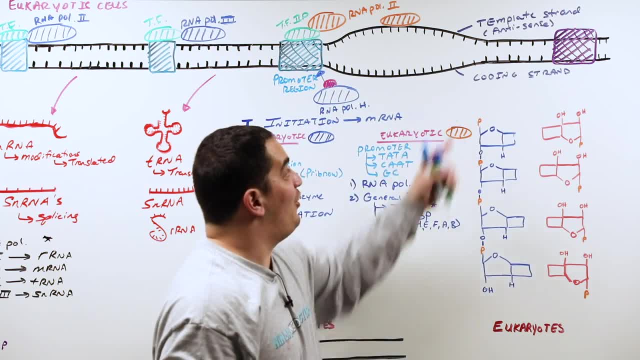 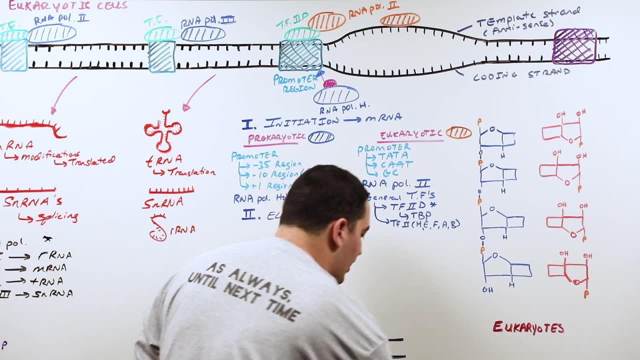 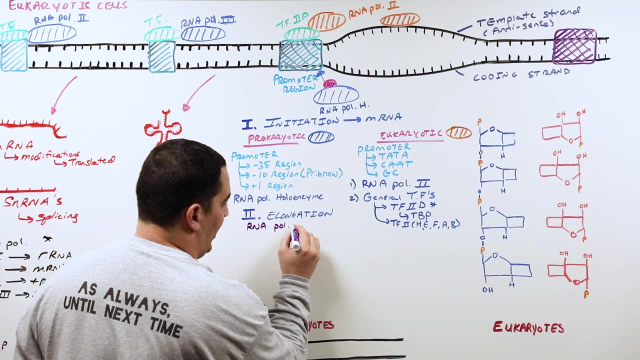 Now, when RNA polymerases read DNA, the strand that they read is the template strand or the antisense strand. So that's the first thing I really need you guys to remember is that the RNA polymerases. what strand do they read? 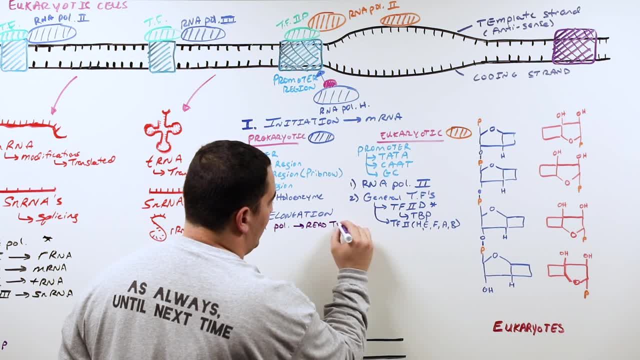 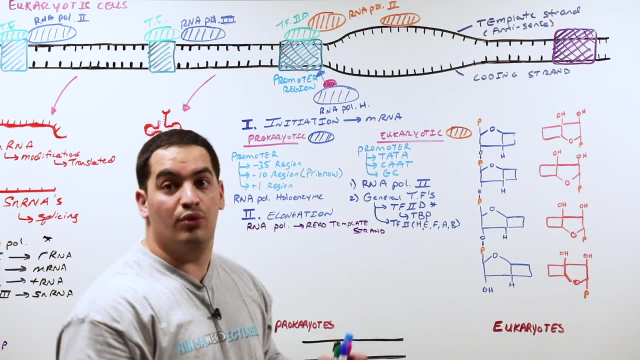 They read: we're gonna put the template strand, or also referred to as what else, The antisense strand, And that's the strand that they use to make the mRNA. They do not use the coding strand, So let's kind of put a little asterisk here. 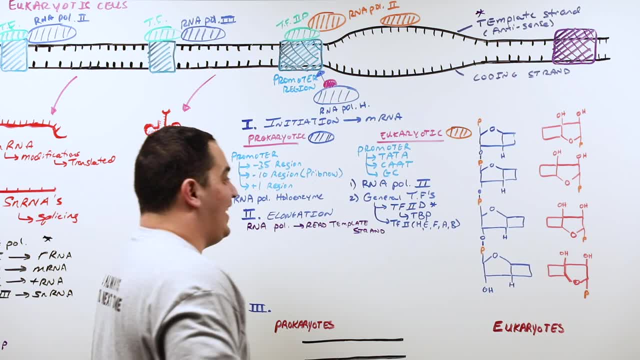 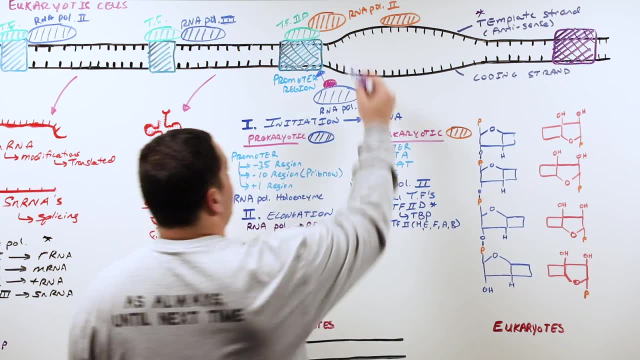 that this is the strand that we're gonna read. Now, when it reads it, it does it in a way that you guys, if you guys watch our DNA replication video, this should be so darn easy. Let's say here: this end of the DNA is the three prime end. 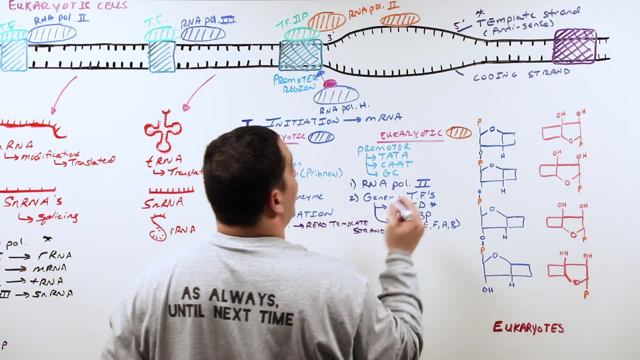 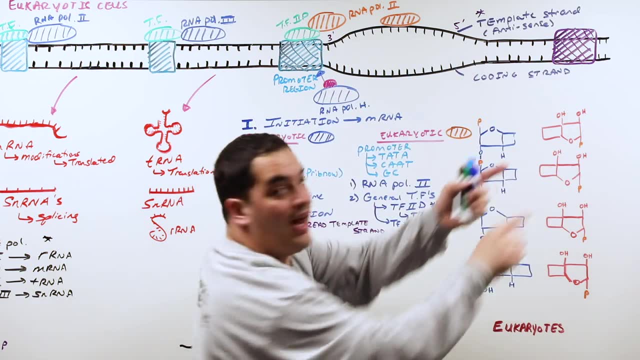 That means that this end is the five prime end. And remember, one strand of DNA on this side should have a complimentary anti-parallel strand on the other side, which means that this is the three end on here. this has to be the five end on this side. 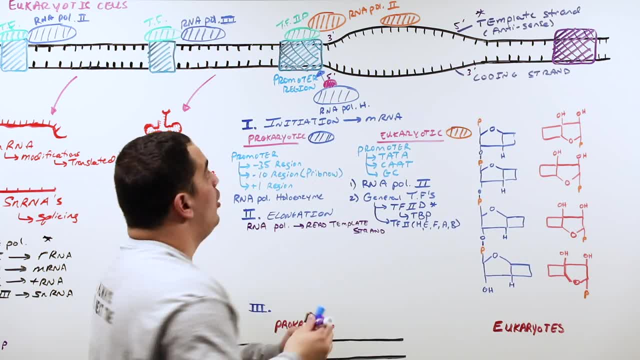 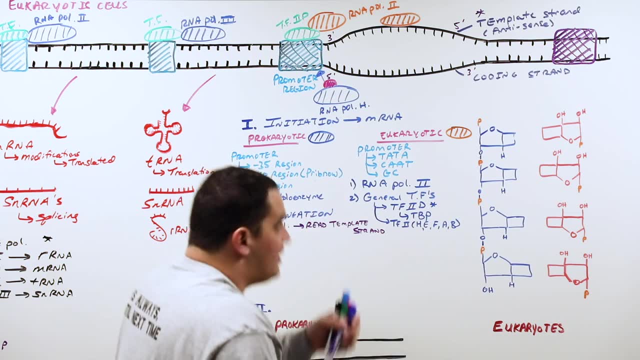 and this has to be the three end. on that side. What happens is this RNA polymerase. when it binds into the DNA, it does something very interesting. It binds to the DNA through the initiation process and then opens up the DNA. Who opened up the DNA before? 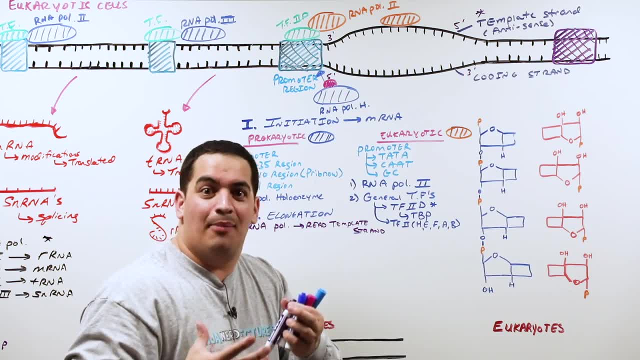 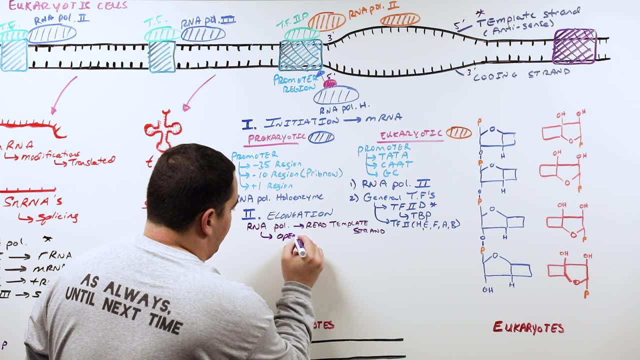 It was that whole replication. it was that whole like replication. complex RNA polymerase does that. So the first thing we need to know is that RNA polymerase does what It opens the DNA. Now, in replication, what else happened? You opened the DNA and you had those single-stranded. 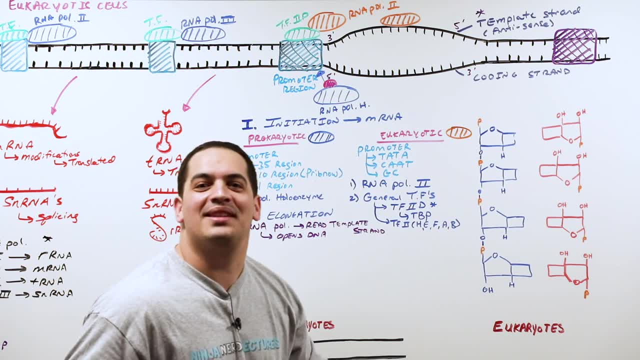 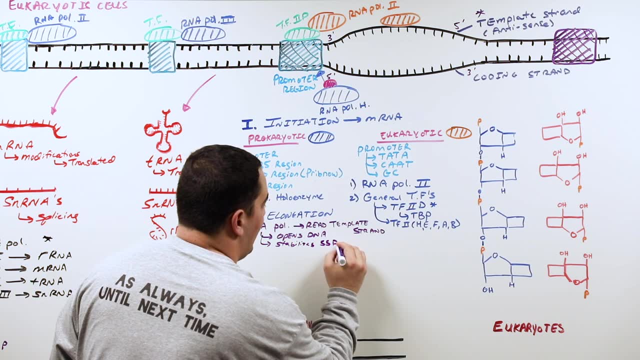 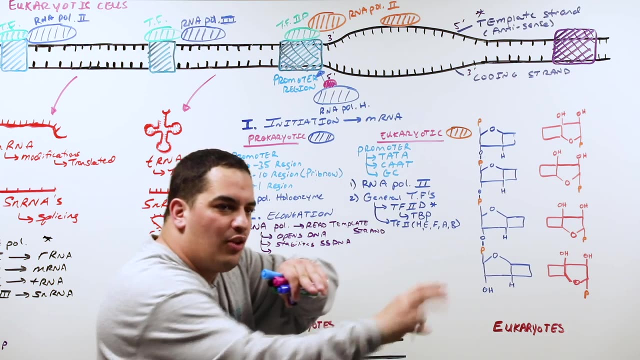 binding proteins which keep it stable and kept it open. right? RNA polymerase does that on its own. It stabilizes the single-stranded DNA molecules, right. So it stabilizes the single strands. Then what was the enzyme in replication that opened up and unwound the DNA? 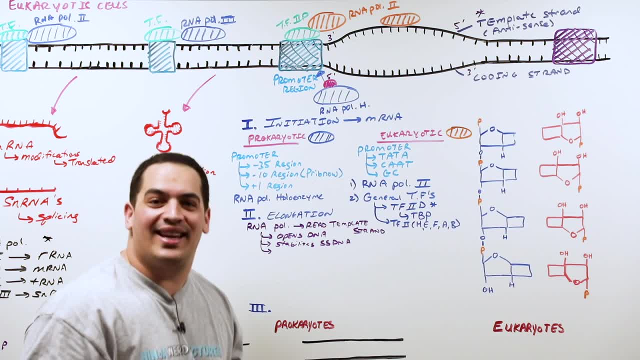 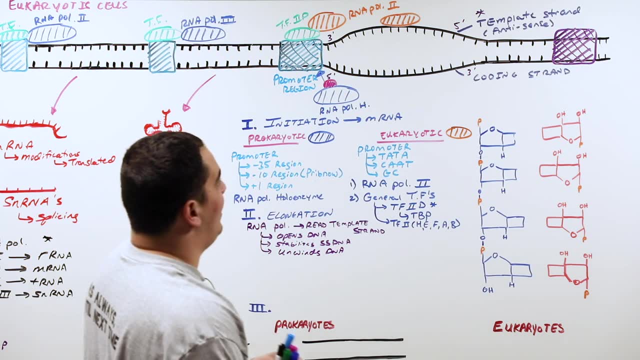 Helicase RNA polymerase has its intrinsic helicase activity, so it also unwinds the DNA. After it unwinds the DNA, then it starts reading the DNA. So let's say here, as it reads the DNA in this direction. 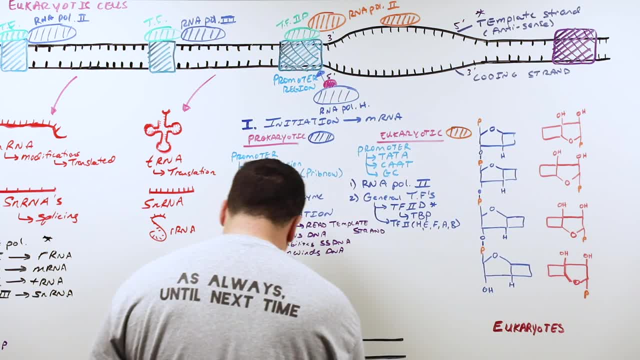 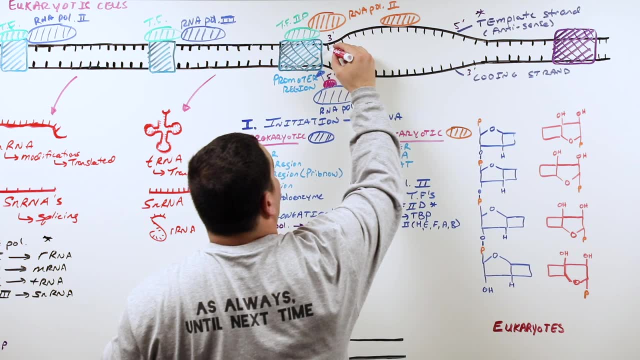 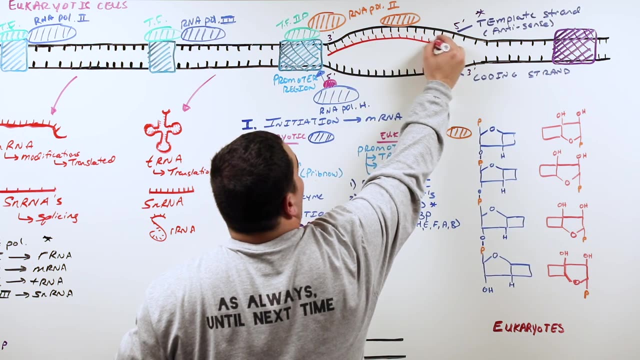 three to five, it'll make mRNA that'll be going in the opposite direction. So it's gonna read this three all the way to the five direction And as it does that, it starts synthesizing mRNA. right. And this mRNA will be synthesized in what direction? 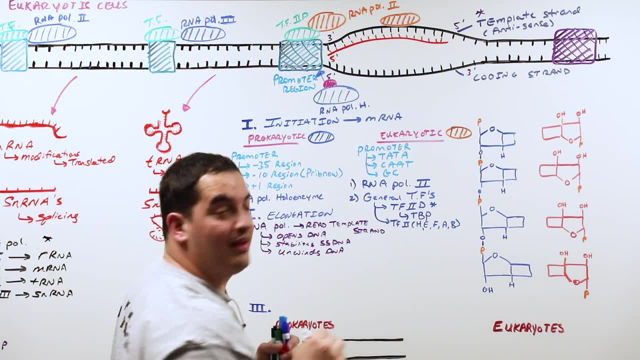 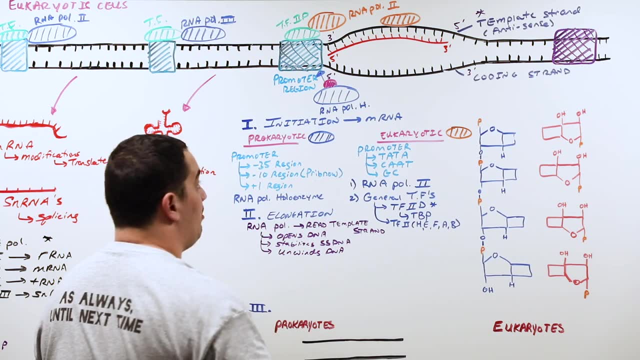 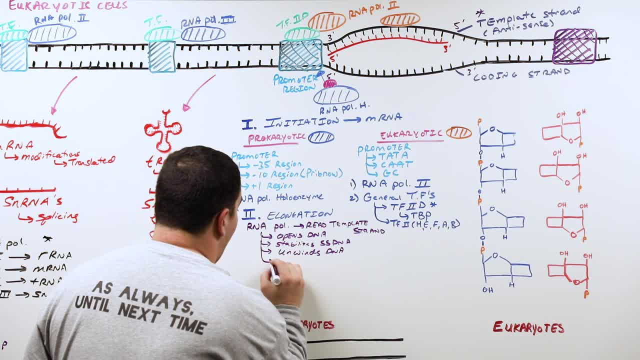 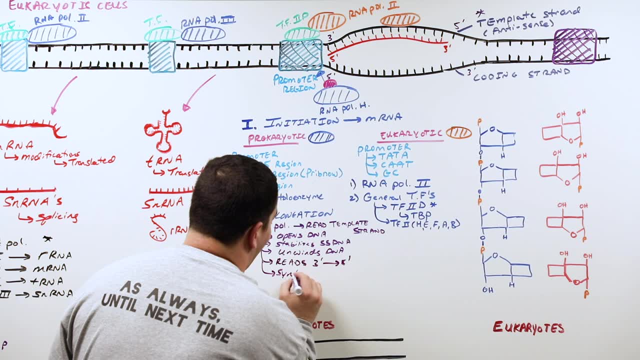 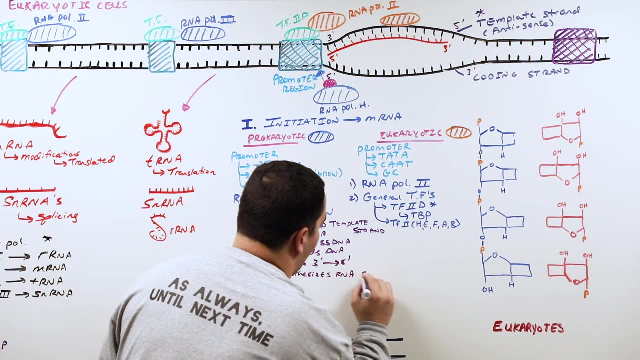 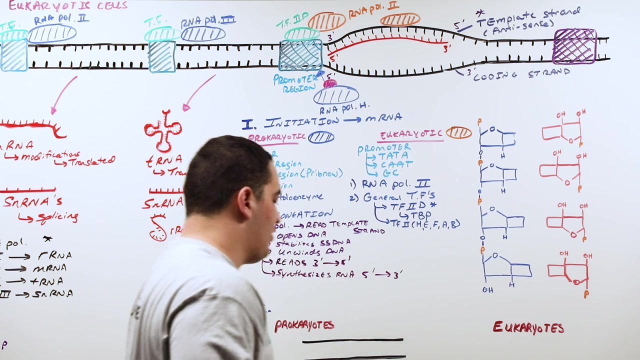 Whether it be in prokaryotic cells or eukaryotic cells, is it reads the DNA from three to five, Then it synthesizes RNA. from what direction, guys? Five to three, Very, very important. The last thing that you guys should be asking is: 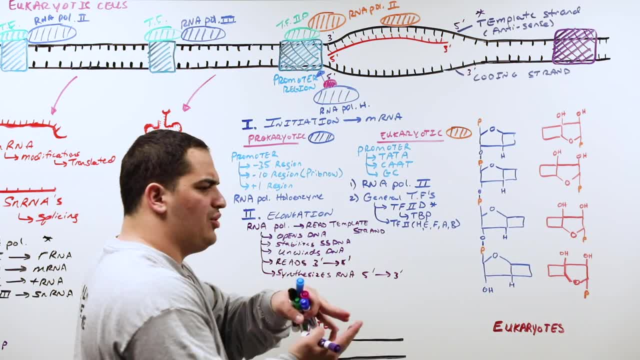 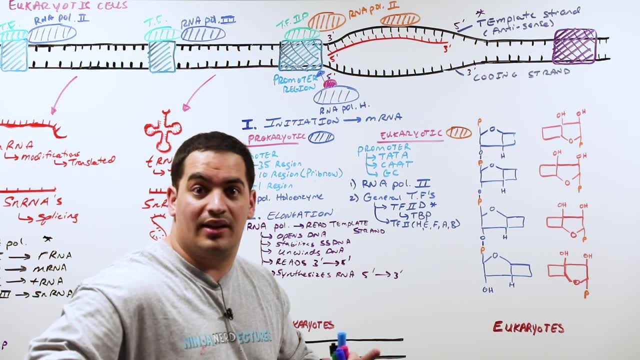 okay, Zach, you also said that in replication, the DNA polymerases, the DNA polymerase, the DNA polymerase read the DNA and then, if there was an accident or a mistake, they would proofread it and then cut out the nucleotide. What about RNA polymerases? Do they do that as well, Because it looks like. 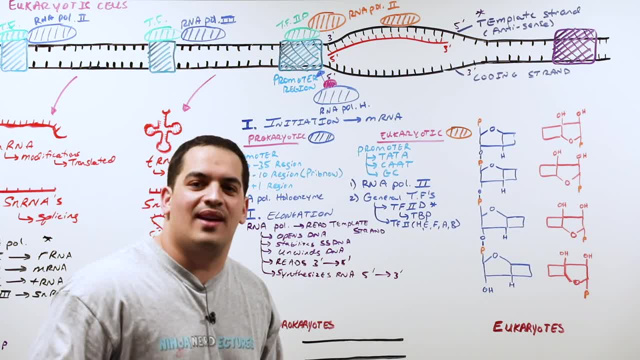 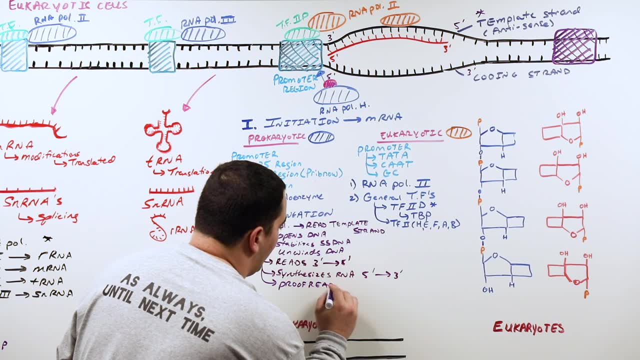 they've done everything that was similar in DNA replication. That's the one thing that's controversial. So the only thing that's kind of relatively controversial is: is there a proof reading function? We don't really know. It's still subject to study. So that's one thing to 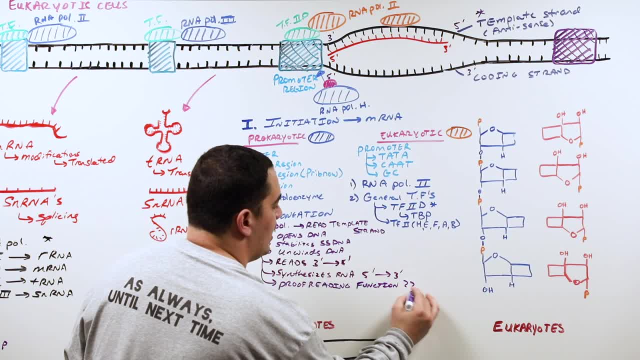 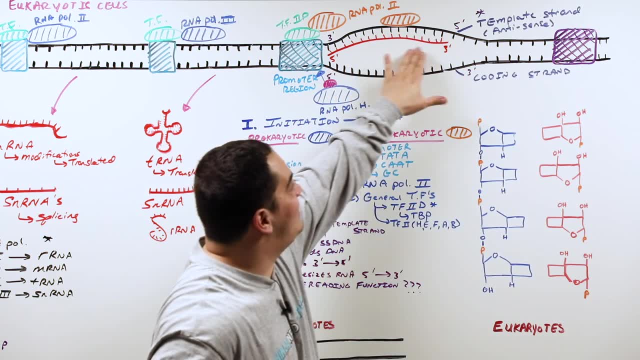 remember. If you want to compare this, the proofreading function is somewhat uncertain at this point in time. All right, so we have an idea now. We've read this DNA and we've made RNA. I know we talked about this a lot in DNA replication. We're talking about it here. 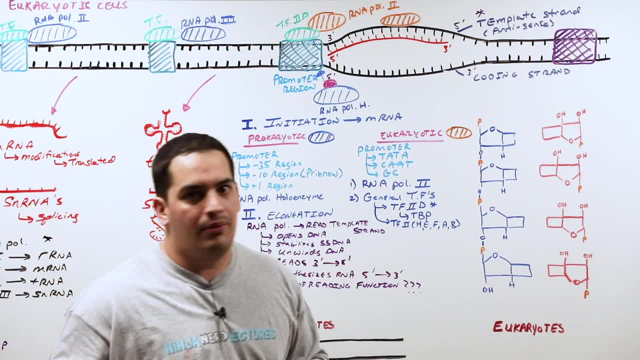 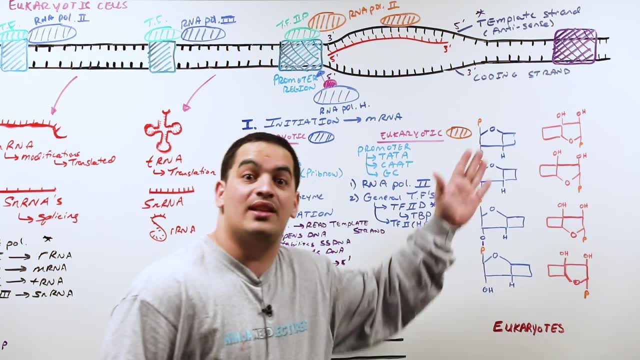 and sometimes it really can be confusing when you're saying 5-end, 3-end. I don't freaking get what you're talking about, Zach. So I want to take a quick little second and explain what the heck I mean when I say it reads it from 3 to 5 and synthesizes it from 5 to 3.. A diagram: I. 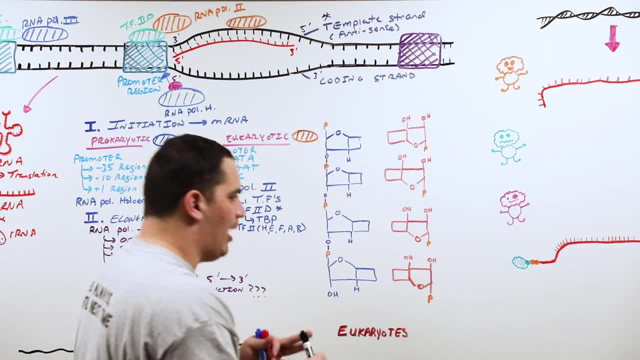 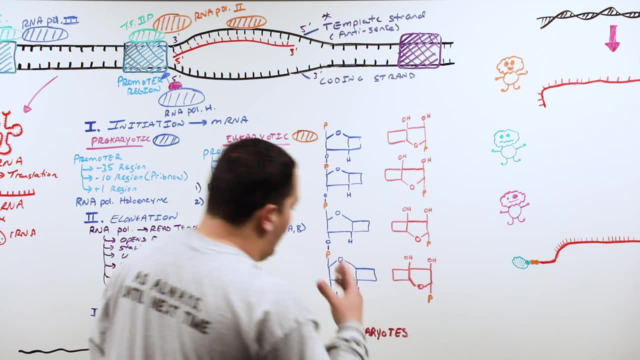 really think will clear this up for you. Let's take a second to understand what I mean by that, By reading the DNA 3 to 5 and then synthesizing it 5 to 3.. I think it's really important to understand that. So let's say: here we have this strand of DNA, So this is going to be our DNA. 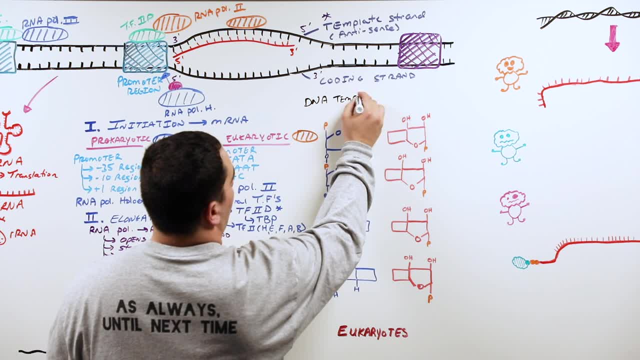 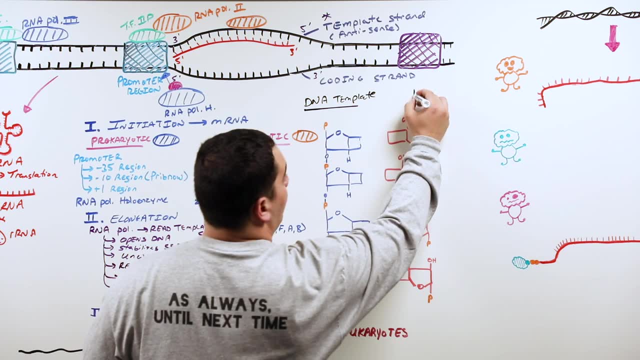 template, if you will. Okay, so this is our DNA template on this side, the blue one- And then this is going to be the RNA that we're going to synthesize utilizing the RNA polymerase. type 2 and eukaryotes are the RNA polymerase whole enzyme and prokaryotes. 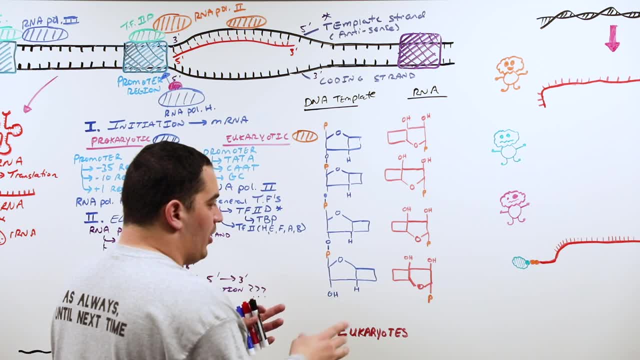 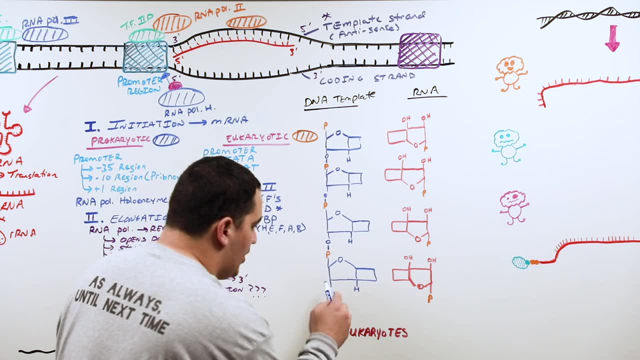 When we're making this RNA, we have to read the DNA. in what direction? The 3-end to the 5-end? What is the 3-end? You guys remember the video on DNA structure? It's the OH. So this is going. 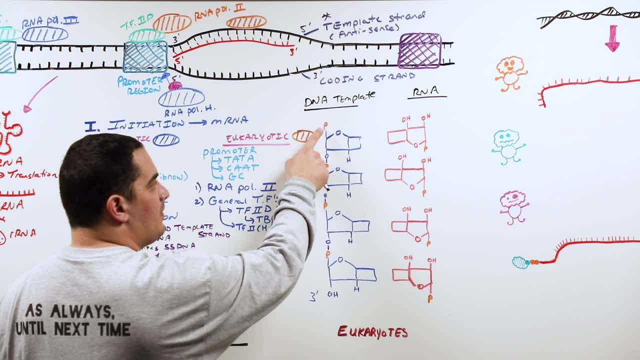 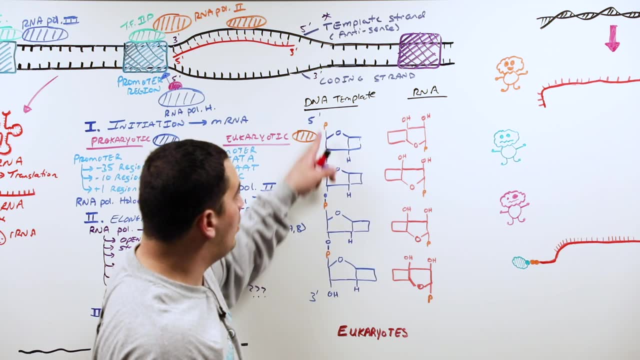 to be the 3-end. What's the 5-end? It's the phosphate group. So the phosphate group is going to be the 5-end. So I have to read this, starting at the OH portion towards the 5-end, where the 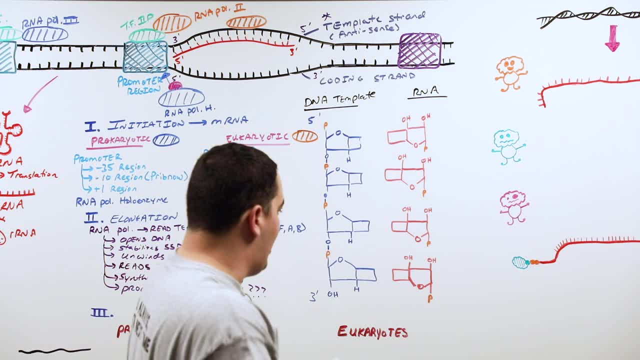 phosphate is So the RNA polymerase. let's pretend I'm the RNA polymerase. I'm walking around, I find the 3-prime and I'm like, oh there, it is Okay, I'm going to move up. Oh, I found the. 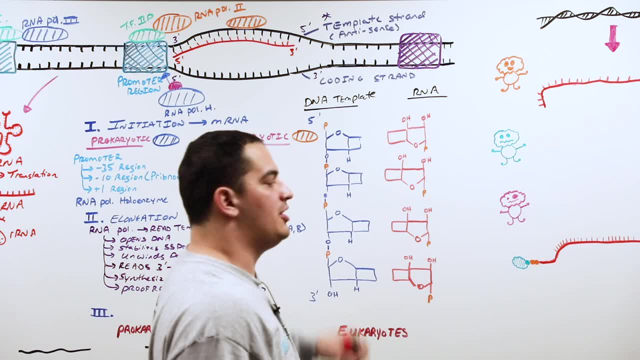 3-prime, 5-prime. Let me just feel this up. Oh, I feel my nitrogenous base, The nitrogenous base that it feels is adenine. So it picks into its little satchel of nucleotides. It's like okay. 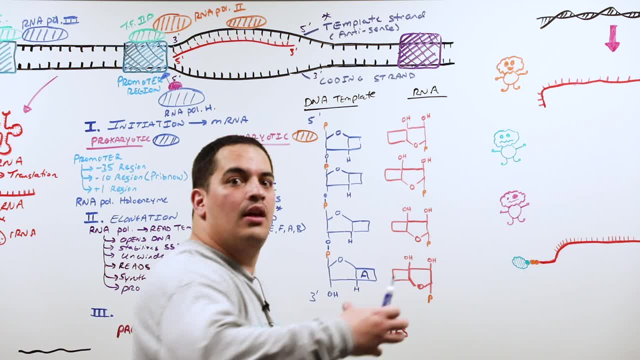 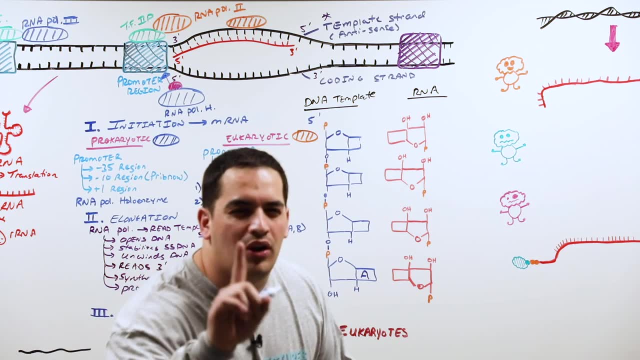 this is adenine. The complementary base for it is thymine. Uh-oh, no, that's not correct, Because you guys know that if we're taking DNA and making RNA, what's the one nucleotide that switches from DNA and RNA? Adenine is no longer complementary. It's a nucleotide that switches from DNA and RNA. 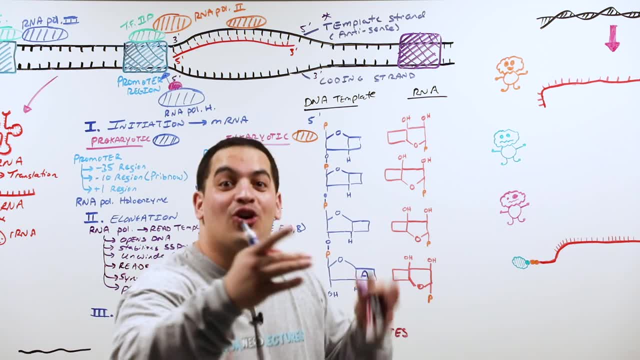 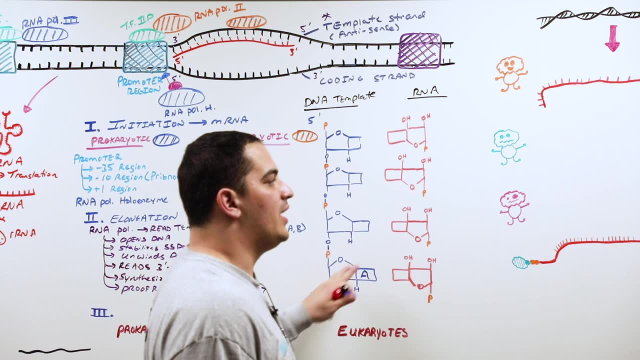 It's not complementary to thymine in the RNA, It is uracil. So the DNA, the RNA polymerase, will come read, find the 3-end, read the nucleotide and say, oh okay, this is an adenine, reach into. 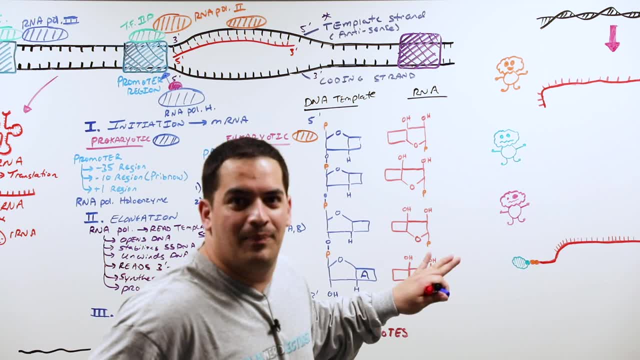 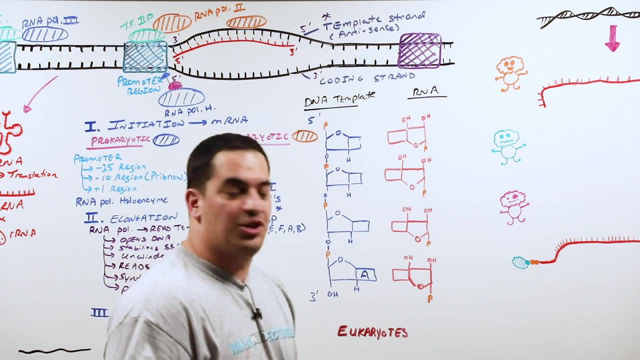 its satchel of a bunch of nucleotides and pull out uracil. When it pulls that out, it then puts the nucleotide in a particular orientation. What's the orientation We said? it reads it from 3 to 5. 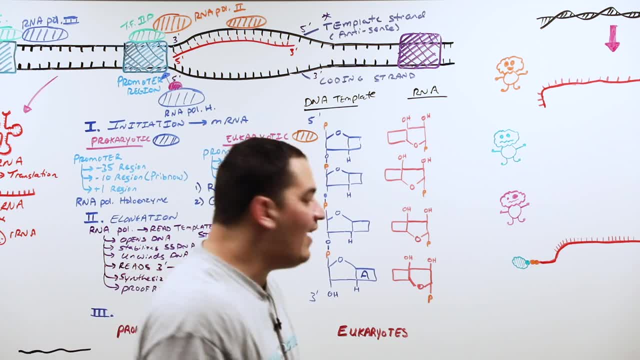 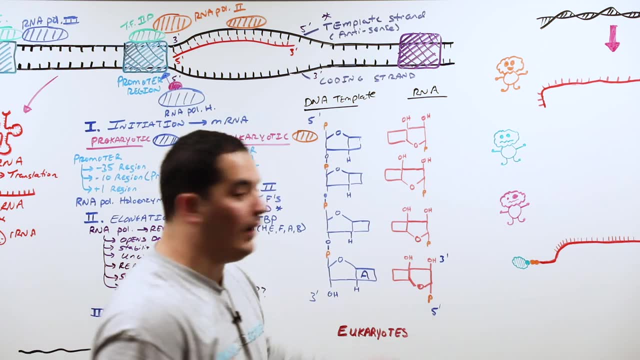 and synthesizes it from 5 to 3.. What's the 5-end? Here's the 5-end. Here's the 5-end. Here's the nucleotide. The 5-end is this phosphate group, The 3-end is this OH group. So it's going to kind. 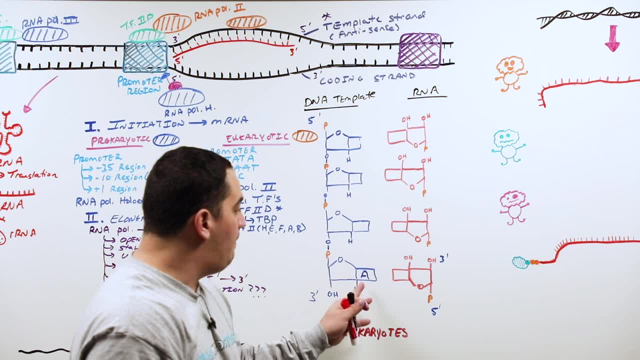 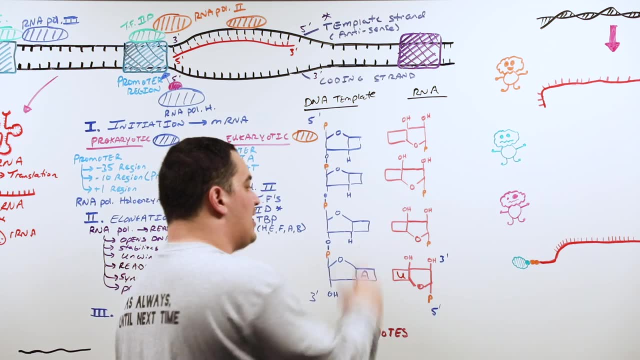 of flip the nucleotide the opposite direction and make sure that the nitrogenous base here is what Uracil. Then when it does that, it's going to go to the next one. So it's going to continue, It's going to go to the next point. Here's where the next OH group would be right: The 3-prime end. 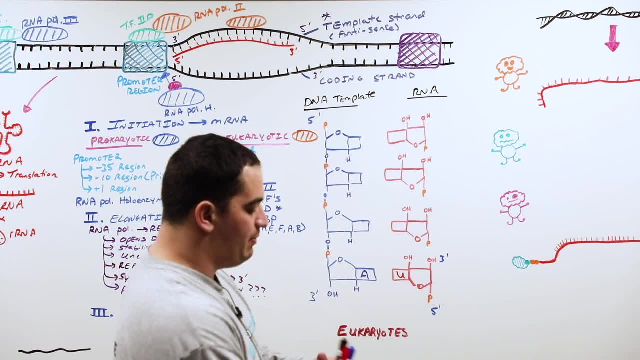 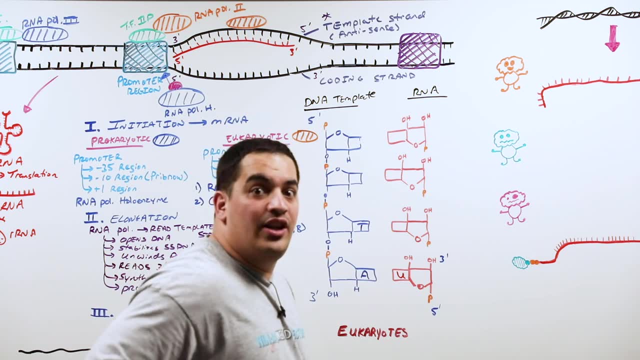 Reads it, finds that, finds the nucleotide, and says: oh, the nitrogenous base, here is T. Let me reach into my satchel of a bunch of different good old nucleotides. I'm going to read it: T goes with A. I'm going to put my nucleotide and I'm going to flip it where it's 5-prime end. 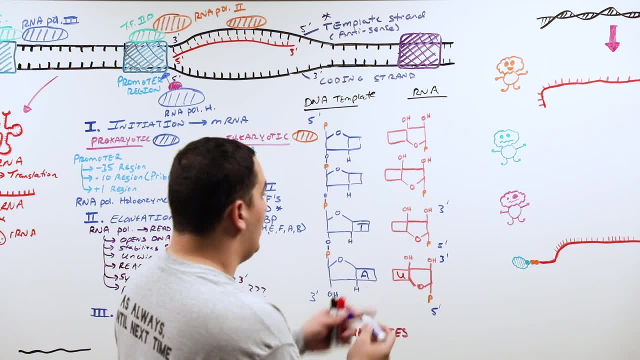 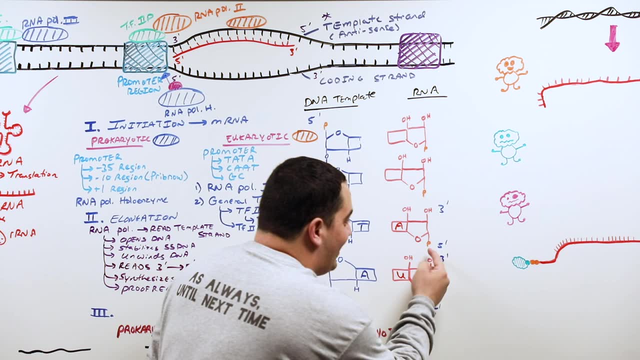 going down 3-prime end, pointing up, And then the nitrogenous base, which is complementary to the T, is A. When it does that, it then fuses the 3-prime end and the 5-prime end together. 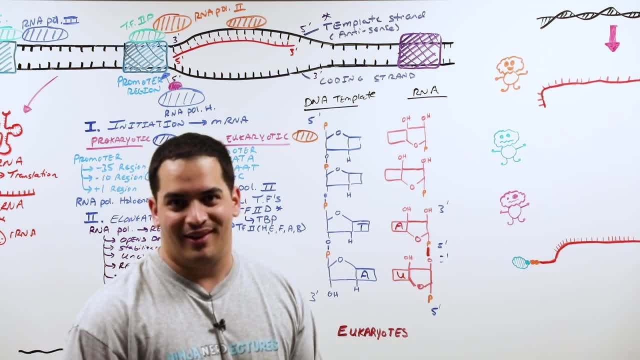 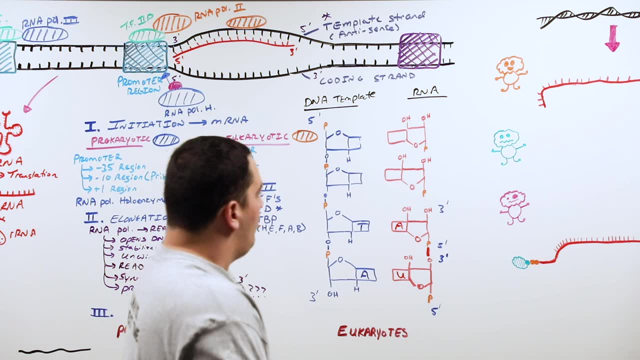 making a bond. What is that bond called The phosphodiester bond? And the same process occurs. So then it'll do what. Let's fix this 3-prime end there. It'll then go go to the next nucleotide. Here's the 3-prime end where the OH 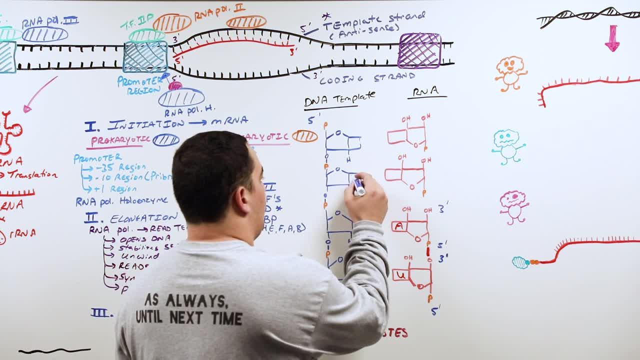 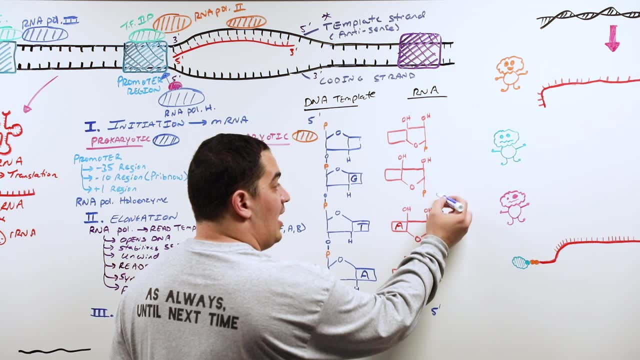 group is: Reads it finds the nucleotide, says that it's a G, reaches into its satchel, pulls out a nucleotide with the cytosine. When it does it, it flips it to where the 5-end is on this side. 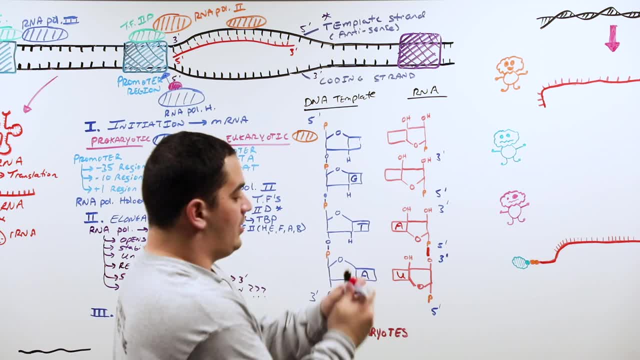 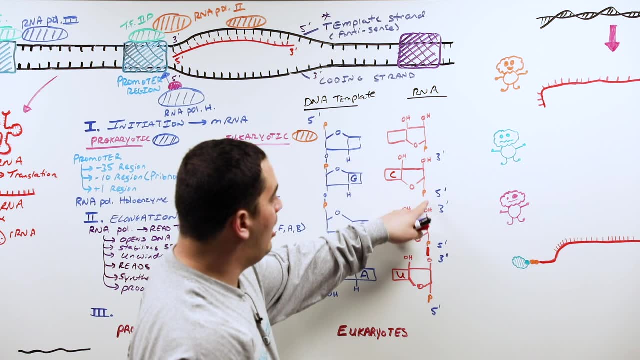 There's my phosphate. The 3-prime end is upwards And it says, oh, the nucleotide that goes with this is with the nitrogenous base C. Then it says, oh, I have my 5-prime end situated close to the 3-prime end of the preceding. 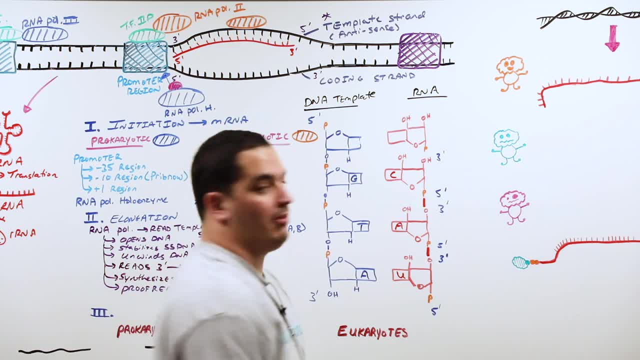 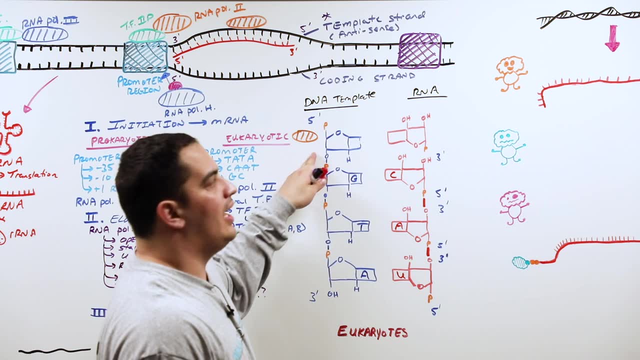 nucleotide. Let me fuse these two together and make my phosphodiester bond. And just for the heck of it- because repetition, I guess, is helpful- we go. reads. this says: okay, next one. here's my 3-prime end, where the OH group is: Read it: find the nitrogenous base. It's a cytosine. 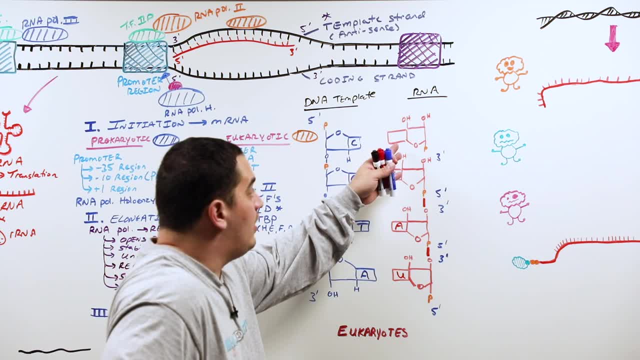 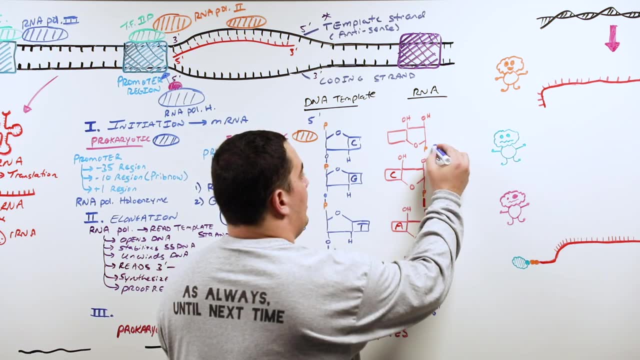 Digs into its satchel, pulls out the nucleotide Guanosine, I'm sorry, the guanine nitrogenous base, Then, when it does that, it situates it where the 5-prime end is situated down. 3-prime end is situated. 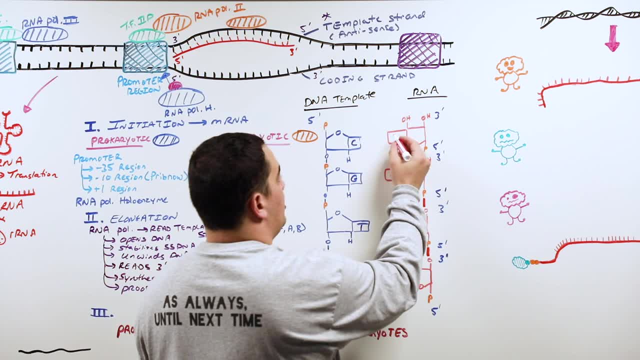 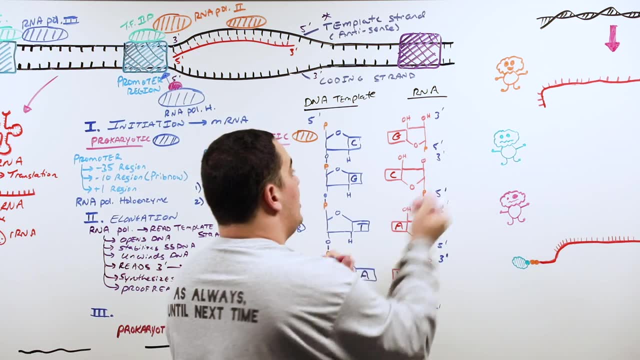 upwards, in this case, And then the nitrogenous base is guanine. Then it says: oh, my 5-prime end. I can stitch it to the 3-prime end of the preceding nucleotide and form my phosphodiester bond. 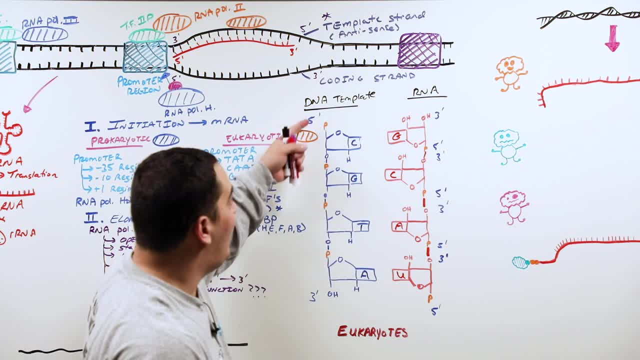 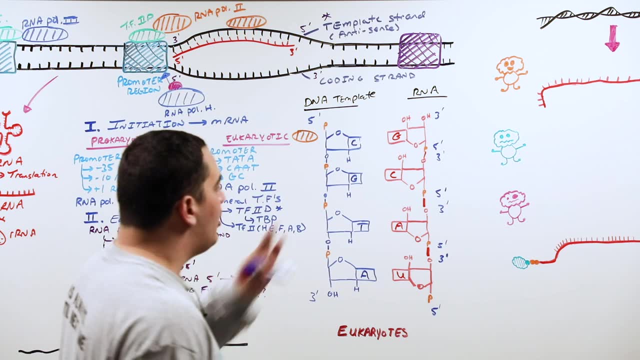 And that's how we make RNA: reading it 3 to 5 and synthesizing it from 5 to 3.. Dang we good All right, now that we've done that, the last thing I need you to understand is that. 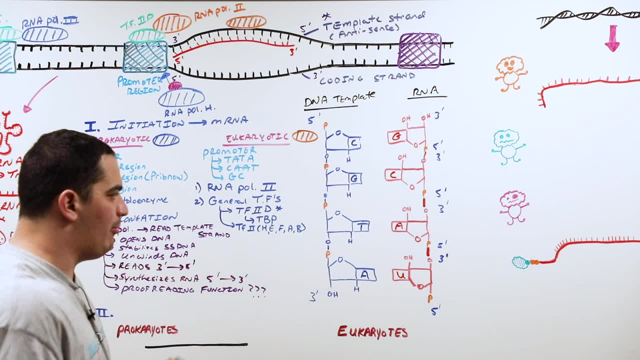 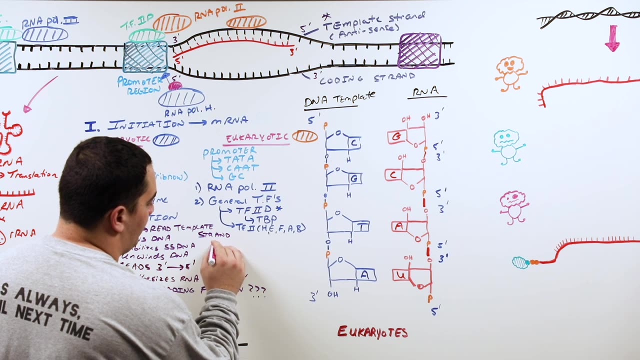 RNA polymerase is a very important enzyme within eukaryotic and prokaryotic cells. A question that can come up- and it's so dumb and annoying but you should know it- is that in eukaryotic cells we can inhibit the RNA polymerase by using a kind of toxin. 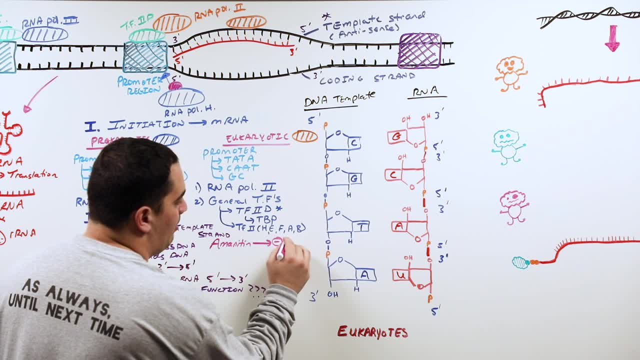 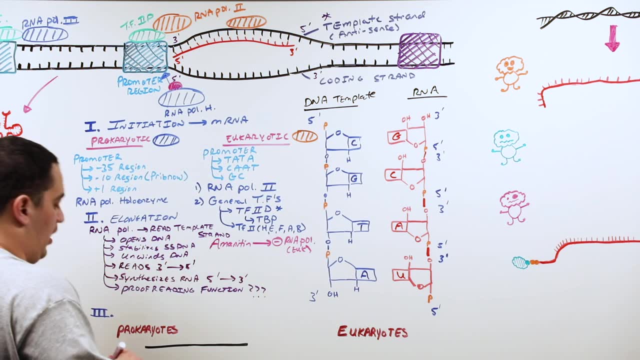 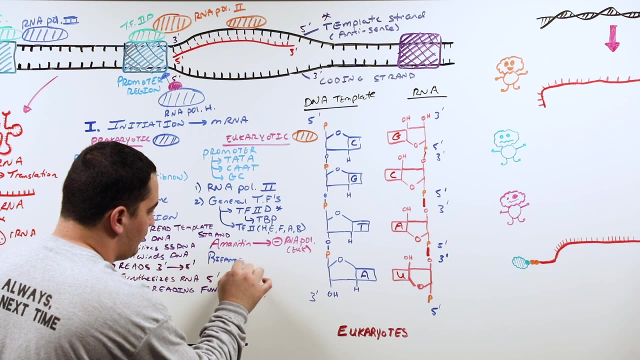 a mannitin. It's for mushrooms And this can inhibit the RNA polymerase. within we'll put eukaryotic cells. There's another drug which they love to ask in the exams as well, called rifampicin. It's an antibiotic And this inhibits the RNA polymerase. 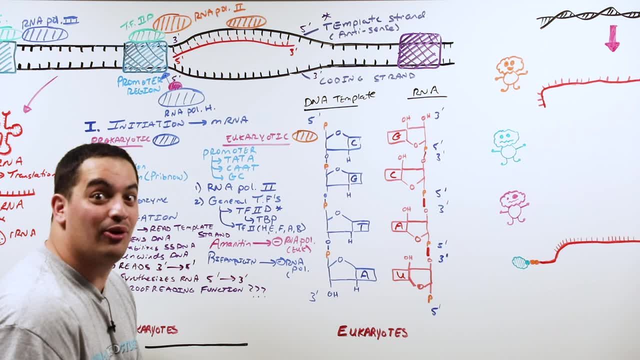 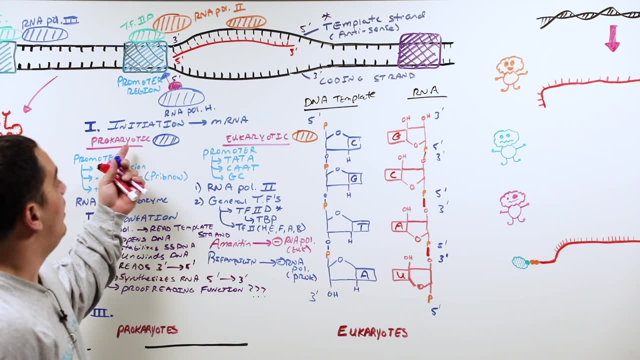 within- if it's an antibiotic that's good against bacteria- prokaryotic cells. So this would inhibit the RNA polymerase within prokaryotic cells, which would inhibit what? The part of the initiation, the elongation, Making RNA. If you can't make RNA, you can't make proteins. If you can't make proteins. 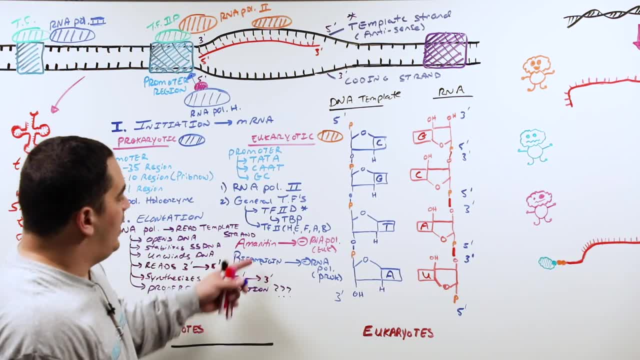 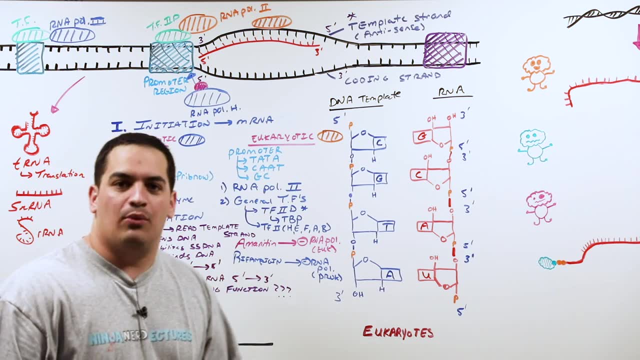 you can't perform the general functions of the cell. So this is kind of from a poisonous mushroom which is stupid to know that. but they like to ask it on your exams. And then rifampicin is an antibiotic which they also love to ask. Okay, now we've talked about elongation, We've made 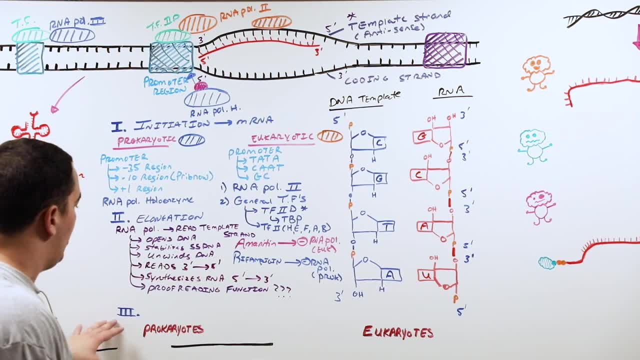 the dang. RNA. RNA polymerase is working real hard. The last thing we got to do is we got to just end it. We don't need any more RNA. We've made the RNA that we need to make the protein That is called. 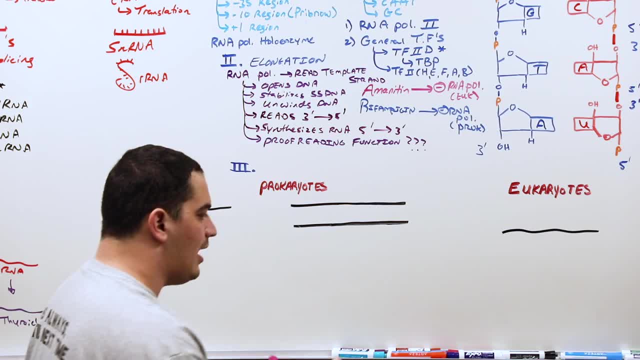 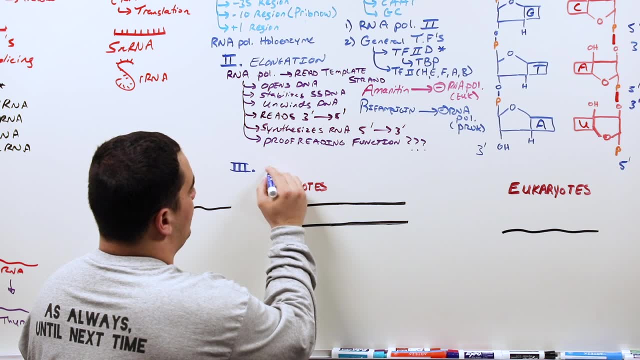 termination. All right, so we talked about elongation. The next step, the last step really that we got to discuss here, is termination. We got to end this whole transcription process, So the last step is termination. Now, unfortunately, termination is probably one of the more annoying. 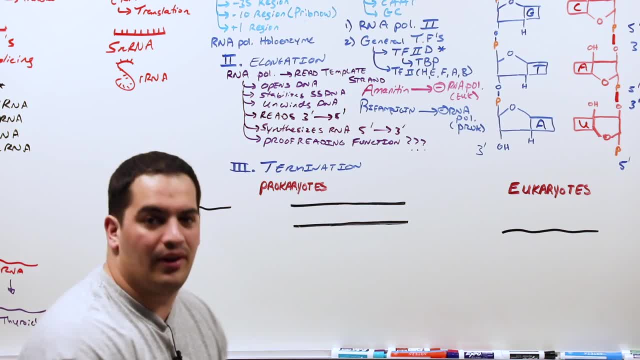 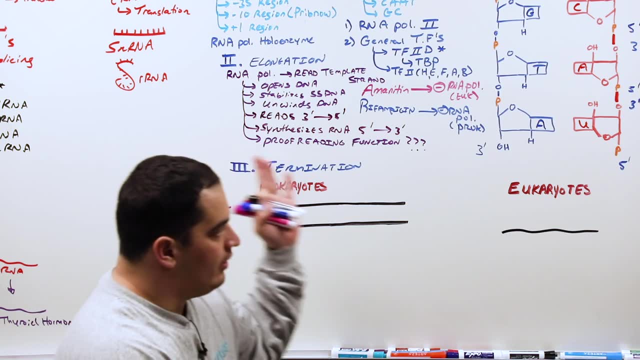 and complicated ones, unfortunately, And it is different in prokaryotes and eukaryotes. That's why it kind of makes it a little bit frustrating. But termination is basically where we've already made our RNA transcript and we just need to detach it. 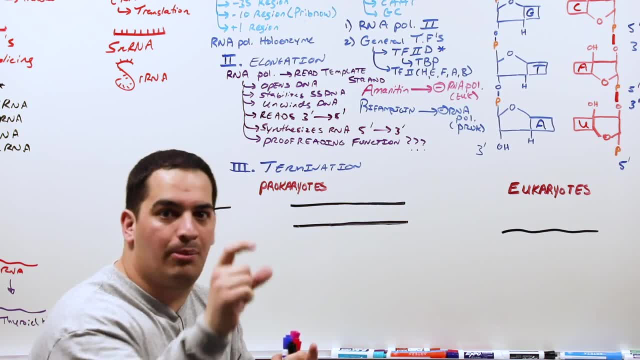 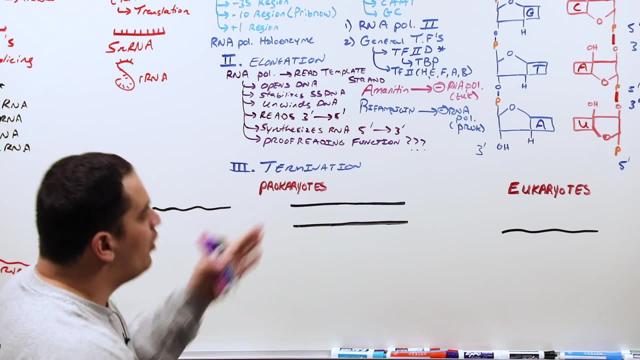 We're disassociated away from the DNA and prevent that RNA polymerase from reading any more of the DNA and making any more RNA. So just stop transcription. How do we do that In prokaryotes? there's two mechanisms. One of the ways that this happens is through what's called 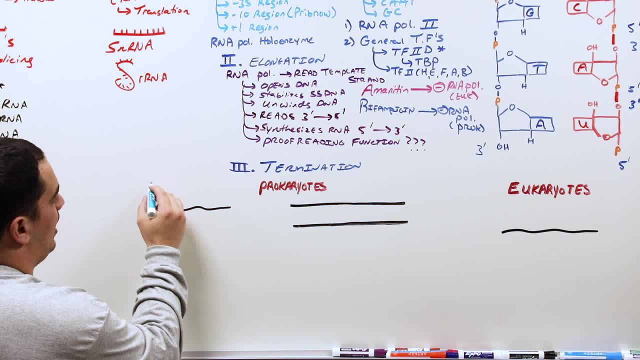 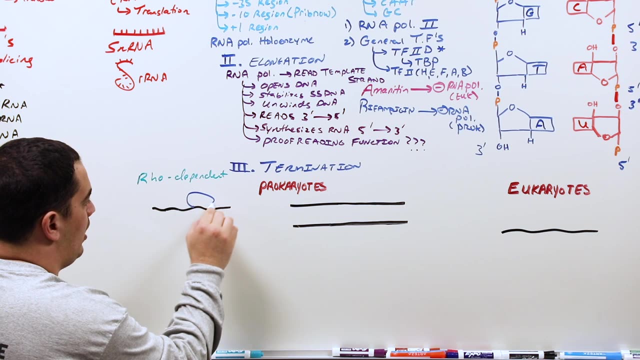 rhodependent termination. So one is, via this process, called rhodependent termination And it's really simple, believe it or not. So let's say, here we take the prokaryotics, We, we picked blue for our RNA polymerase. So the RNA polymerase. here's our RNA polymerase. It's 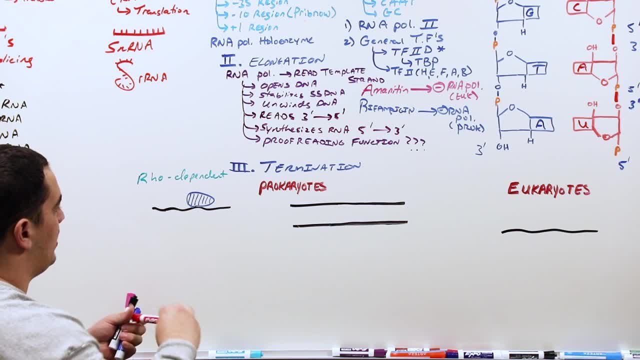 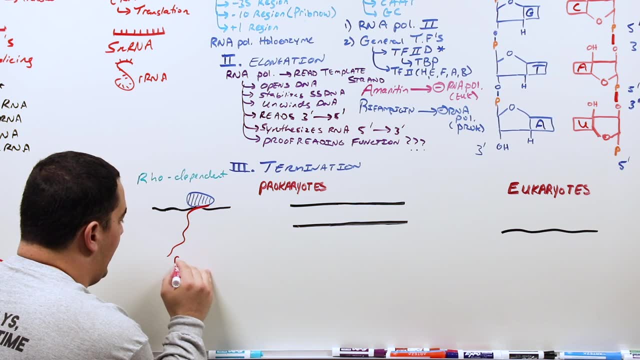 reading this DNA. As it's reading the DNA again, what is it making from it? You guys remember it's making the RNA. In this case, it could be any RNA, It could be the mRNA, tRNA, RNA, whatever. 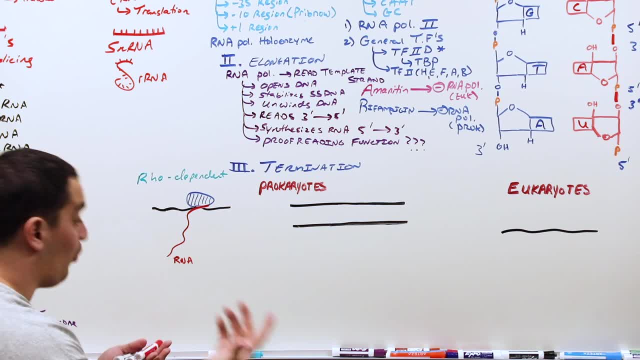 As it does this, there's a protein called Rho, And what Rho does is this Rho protein will start moving up the mRNA And, as it moves up the RNA that's being synthesized by the RNA polymerase, as it gets to this RNA polymerase, 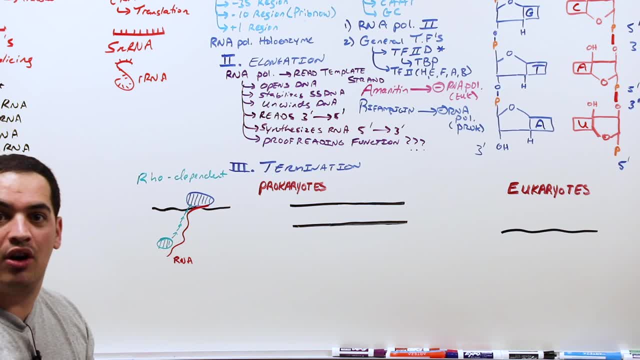 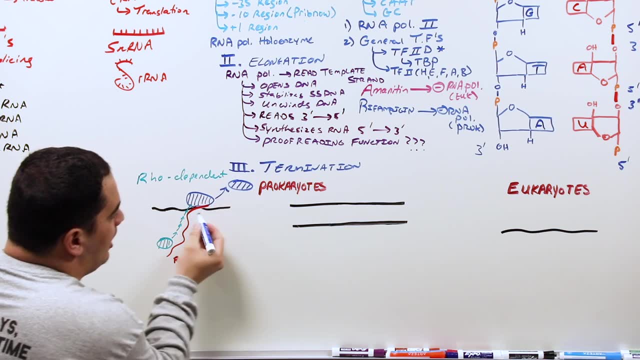 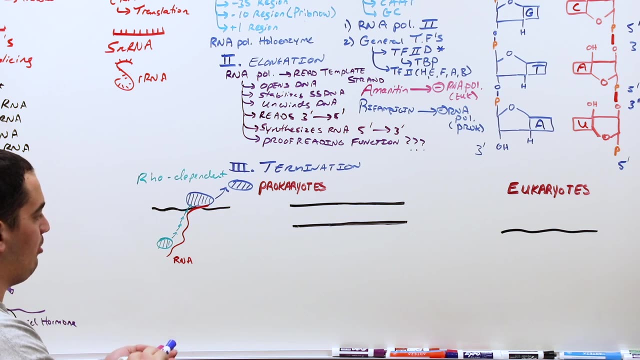 it basically says: hey, it just punches the RNA polymerase off the DNA. If you punch the RNA polymerase off the DNA, is it going to be able to continue to keep reading the DNA and making any more RNA? No, So that terminates the transcription process. So the big thing I need you guys to know here is that with the 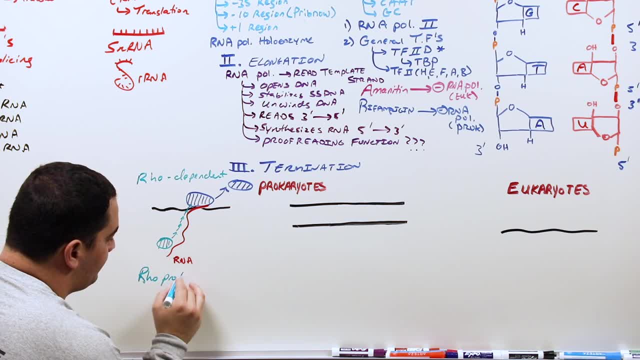 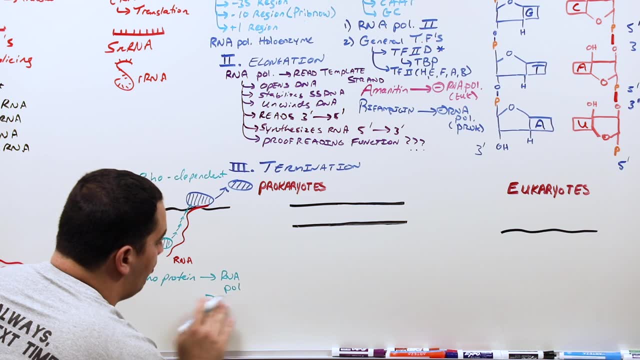 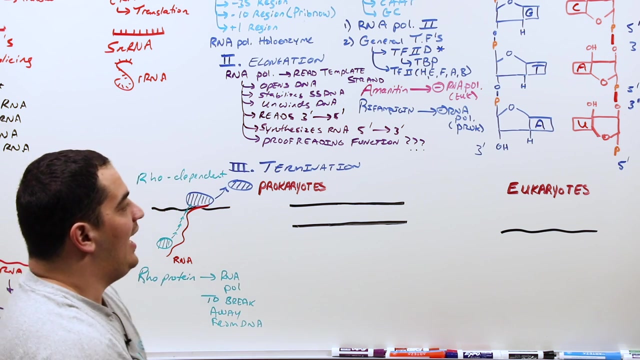 rhodependent termination is Rho protein causes RNA polymerase to break away- to disassociate, if you will. Okay, to break away from the DNA. Okay, Alright, beautiful. The next mechanism within prokaryotes is Rho independent termination. 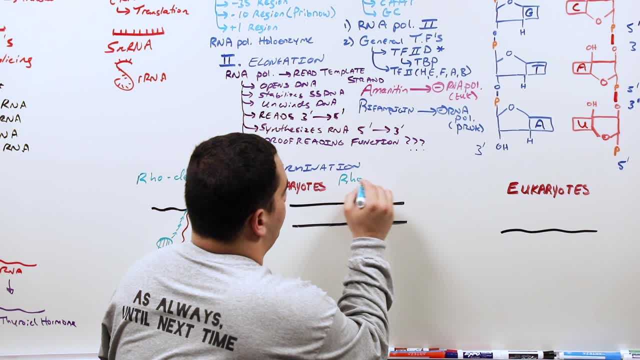 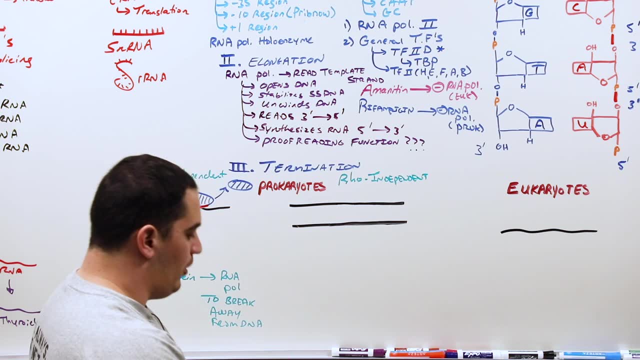 So we don't use the Rho protein, So we call this Rho independent termination. Now, with this process it's a little bit more complicated and a little annoying. Let's say: here we have the DNA right And within the DNA we're going to mark these here. 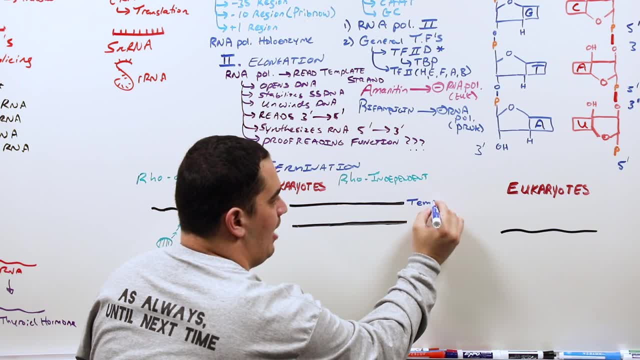 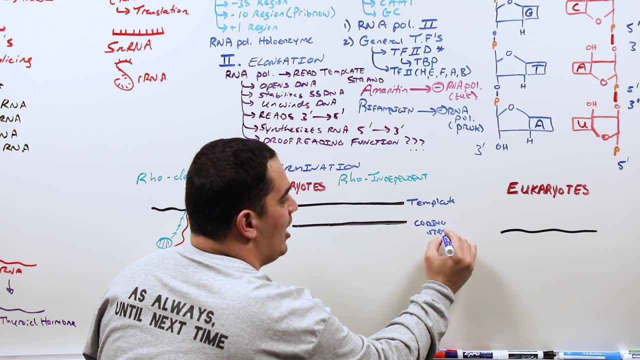 We're going to say: this is our template strand, right? So this strand is the template strand, right? Or the antisense strand, And then this is going to be our coding strand. So which one does the RNA polymerase read? It reads the template strand or the antisense strand. 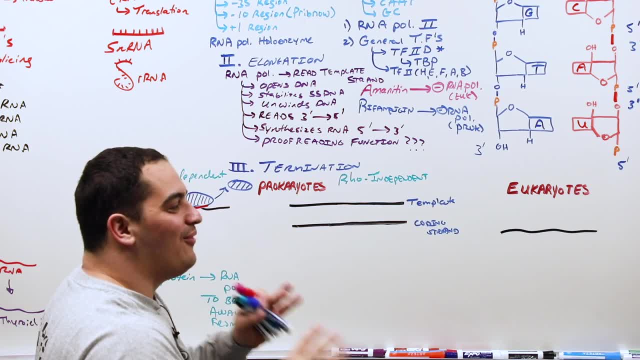 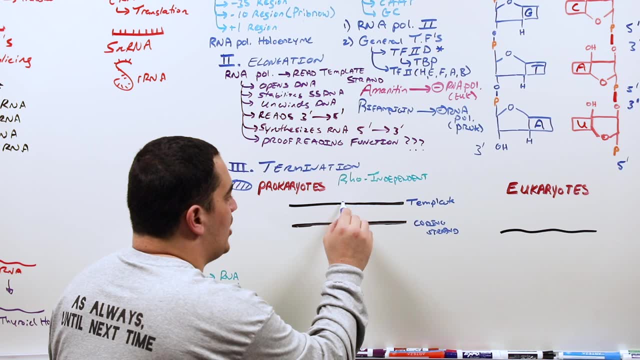 There's a particular like thing called in the DNA. There's a particular like thing called in the DNA polymerase. There's a particular like thing called inverted repeats, that form within the DNA that the RNA polymerase is reading. So what happens is this RNA polymerase will bind to that template strand. 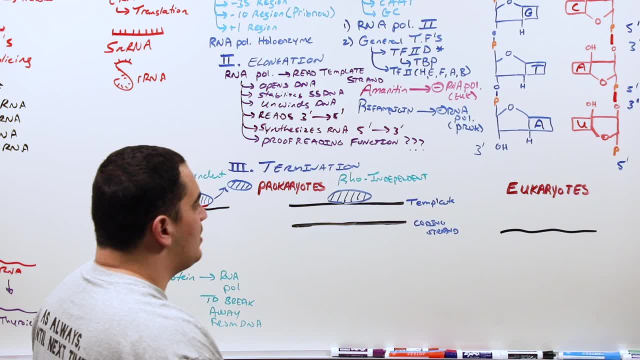 and it'll start reading it, making the RNA. As it starts making this RNA, it encounters a particular sequence of DNA called inverted repeats. Let's write these inverted repeats out in kind of a nice little color. Let's do. let's do orange. 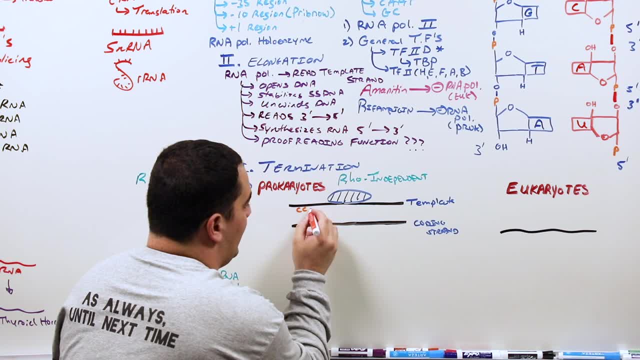 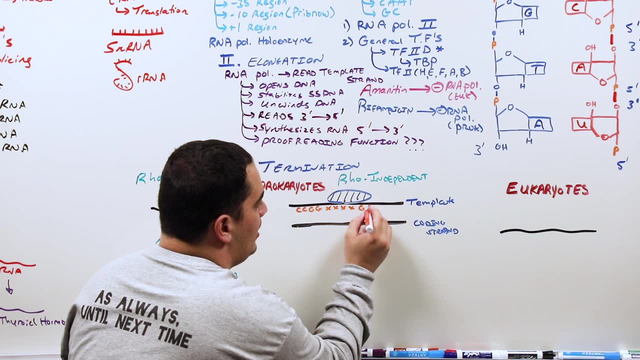 And let's say, here we have a inverted repeat where we have CCGG And then a bunch of nucleotides that we don't care about, And then here we'll have GGCC. okay, Then we're just going to have. this is the template. 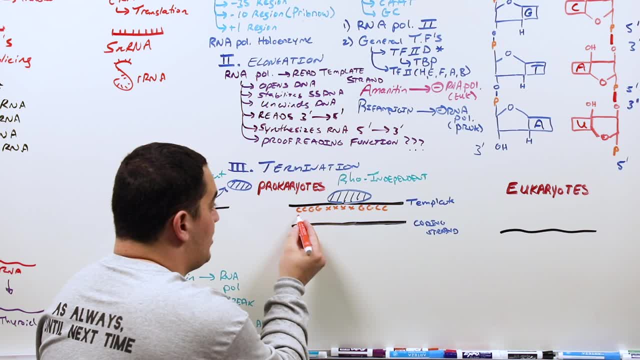 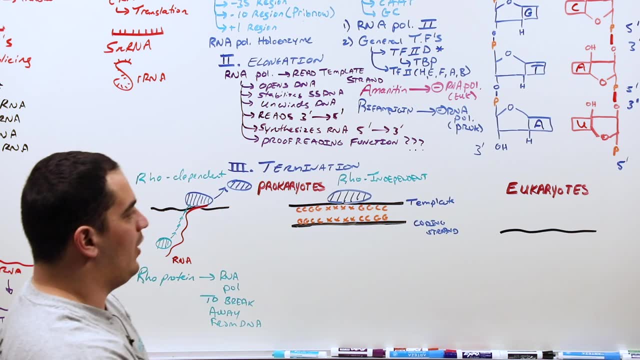 Again on the coding strand, it would just be the complementary base. So if this was CC, this would be GGCC. We don't really care about these nucleotides. CCGG, right? The RNA polymerase is going to read this template strand. 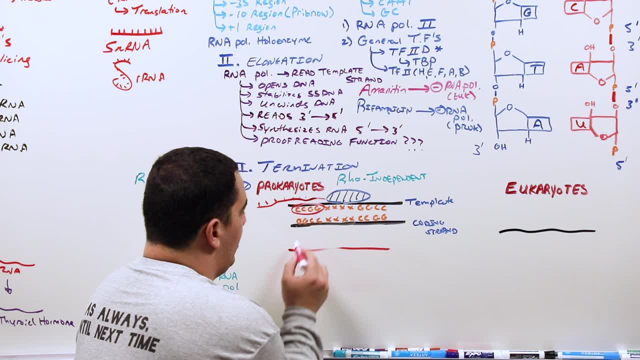 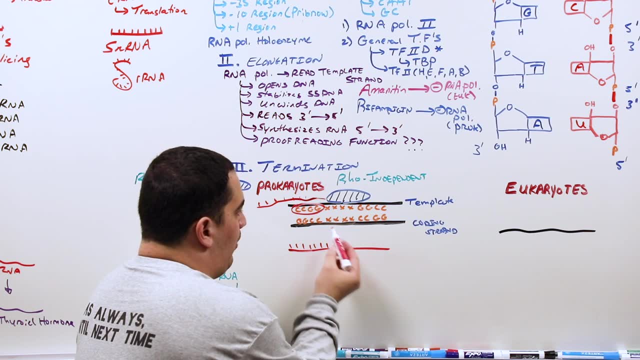 What happens is right is you're going to get this kind of strand here where you'll have a bunch of nucleotides already kind of made up here And then it reaches this kind of like inverted repeat area. And what happens is it reads this and then basically everything you read: 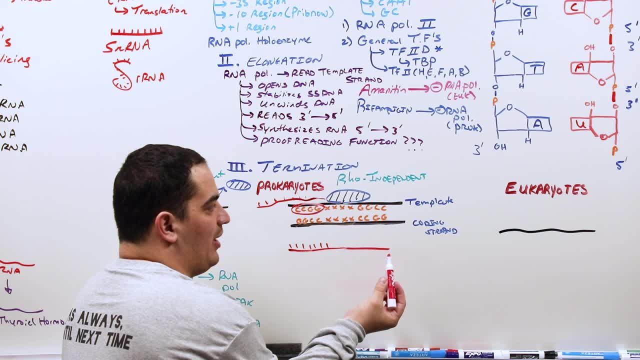 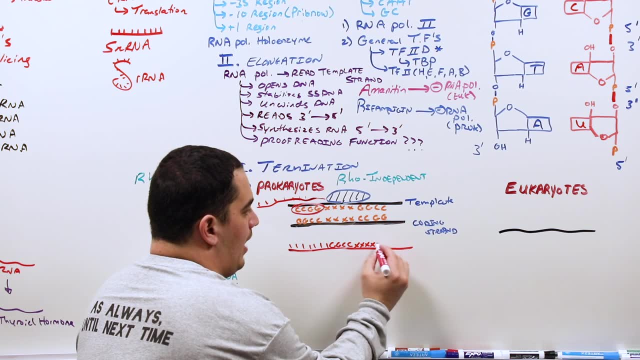 within the template strand should be the same as it is in the coding strand, because it's the complementary base. So you'll have GGCC, that it'll make a bunch of nucleotides we don't care about, and then CCGG. 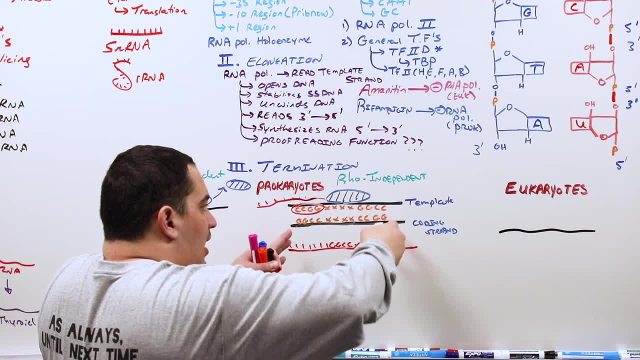 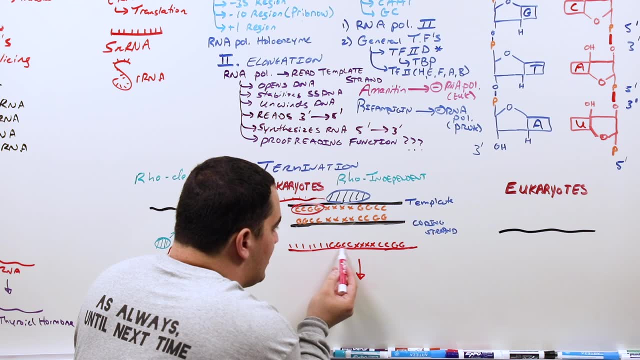 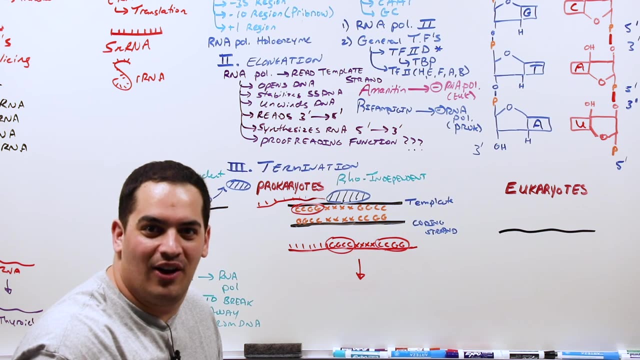 What happens is whenever this RNA is kind of coming and being transcribed from the RNA polymerase, something interesting happens where some of these Cs and some of these Gs on this portion have a strong affinity for some of the Cs and some of the Gs in this portion of the RNA. 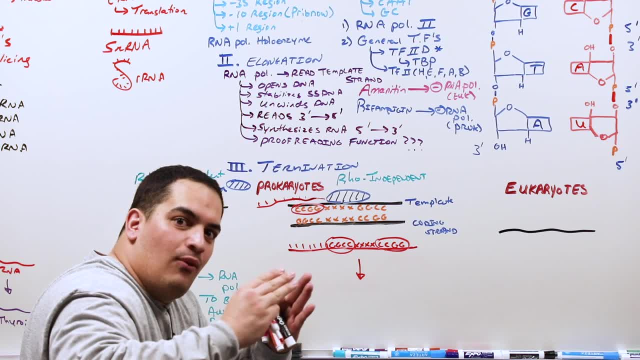 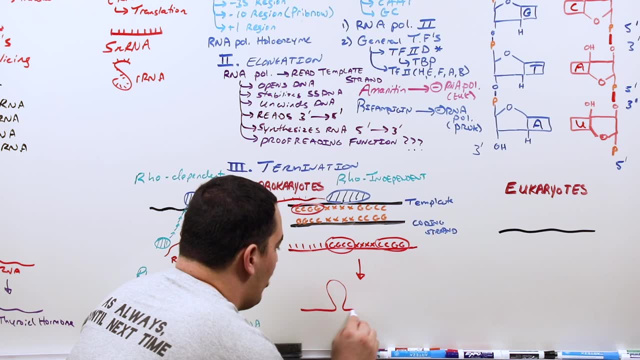 And as they start having this affinity, they start approaching and kind of wanting to interact with one another via these hydrogen bonds And so it creates this really interesting kind of like hairpin loop, if you will. a bunch of Gs and Cs within this kind of hairpin loop. 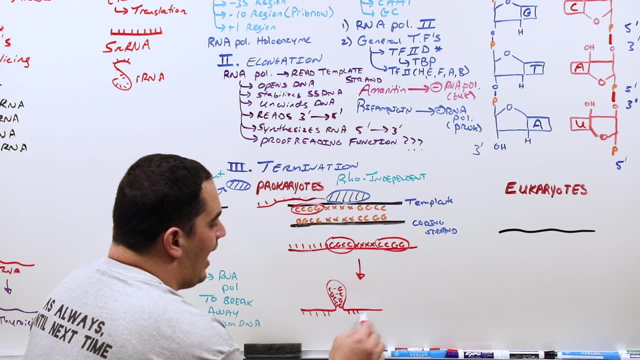 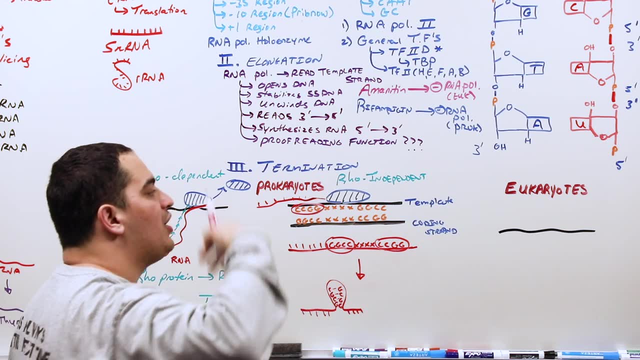 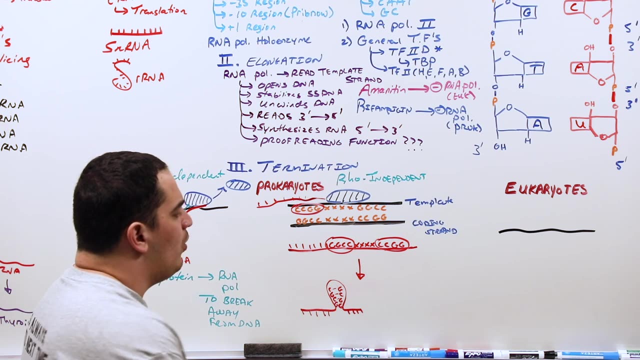 that are kind of interacting with one another And what happens is that hairpin loop is what triggers the RNA polymerase to pretty much hop off of the DNA and terminate the transcription process. Because what happens is, once you form this hairpin loop, 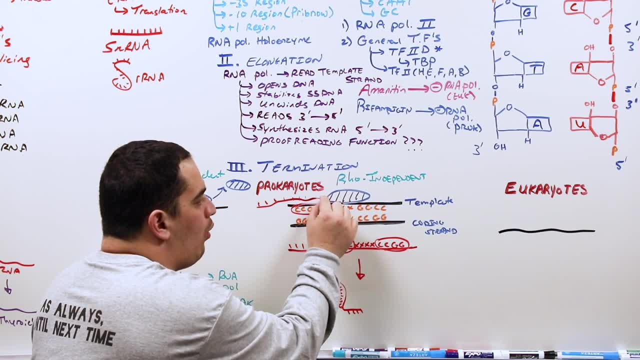 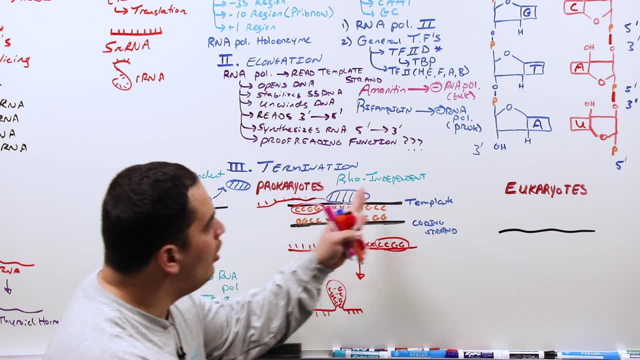 what will happen is there's going to be particular enzymes that'll bind to that portion and cleave the DNA, the RNA, away from the RNA polymerase. So the big thing I need you to know within a row-independent termination is that you'll hit this area. 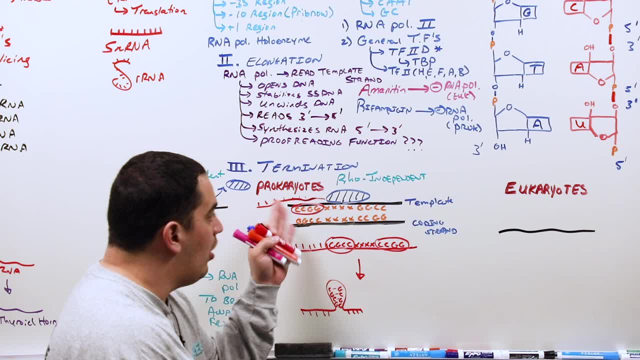 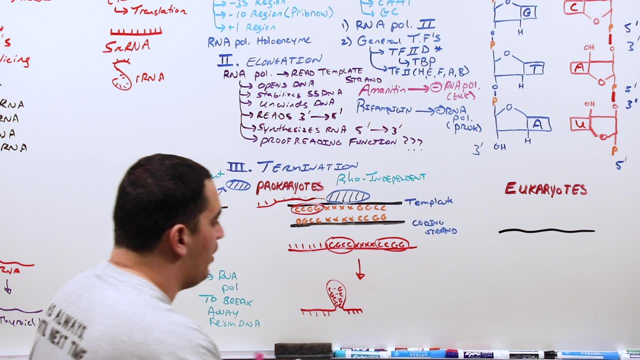 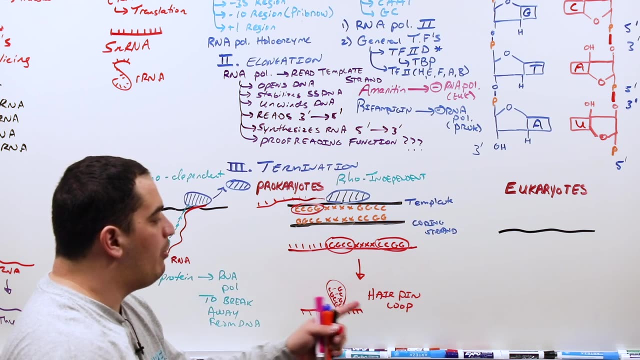 The RNA polymerase will be transcribing, reading the DNA making RNA. It'll hit these areas of inverted repeats. When these inverted repeats are made, they create this thing called a hairpin loop. This hairpin loop will then trigger particular cleavage enzymes. 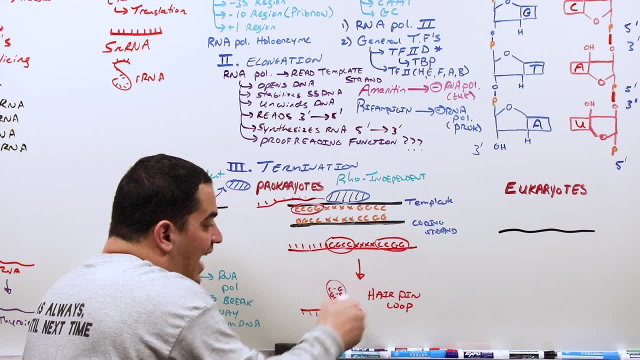 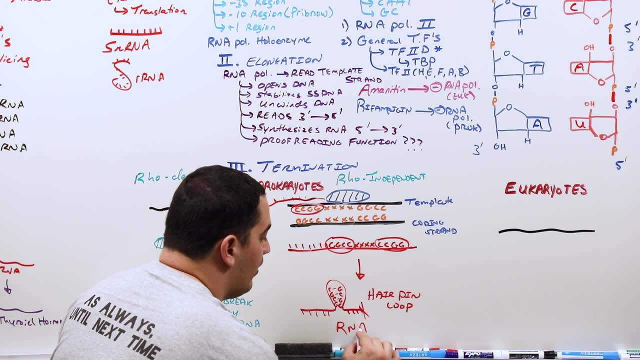 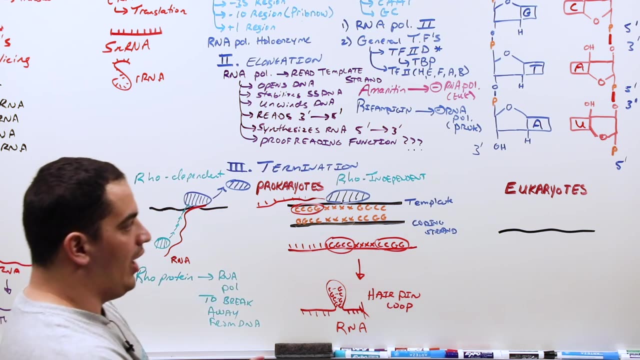 to come and cleave a couple nucleotides after that hairpin loop to cleave that away from the RNA polymerase, And then here you have your RNA that you've formed. So that is one of the ways that we have termination row-independent via prokaryotes. 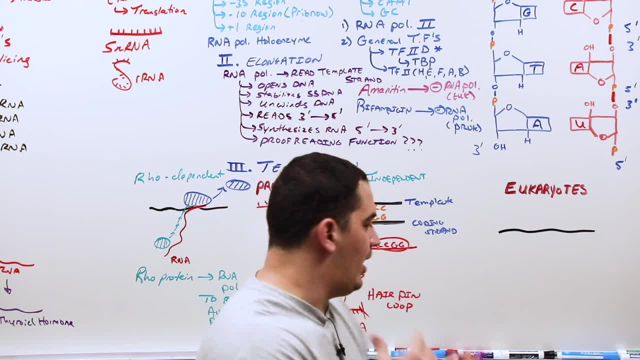 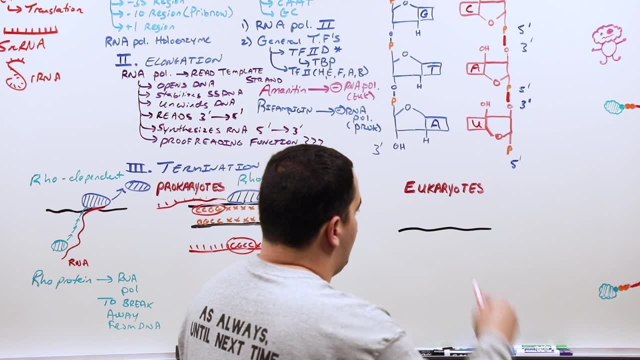 The last termination mechanism is going to be eukaryotic cells. Now how does this work? This one's actually relatively simple. So we had the RNA polymerase in eukaryotes and this was orange. It's binding to the DNA. it's reading the DNA. 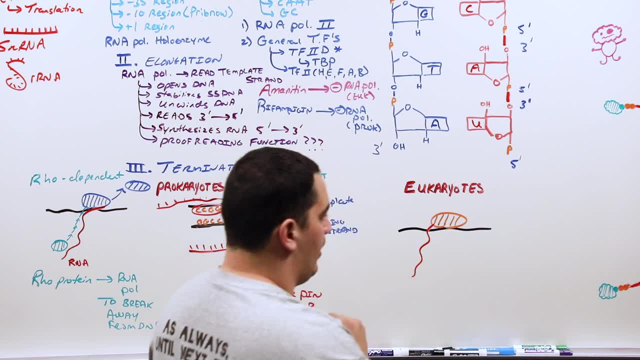 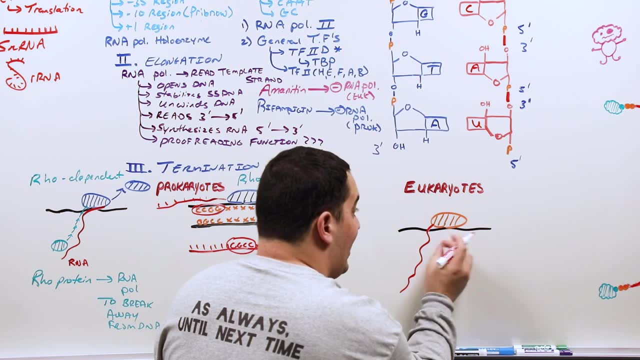 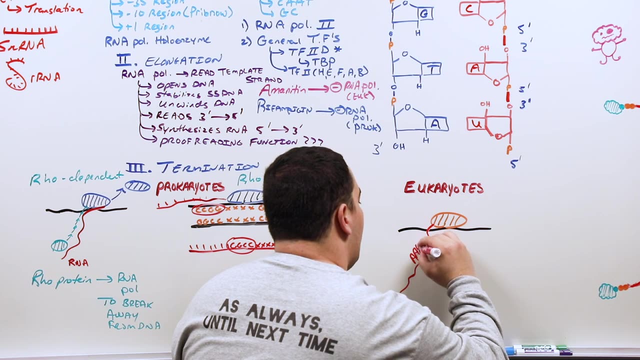 As it's reading the DNA, it's making RNA. As it starts making this RNA, it hits a particular sequence where, when it starts reading the DNA and makes RNA, it makes a particular sequence of AAUAAA. So what does the nucleotide sequence say? Let's write it out. 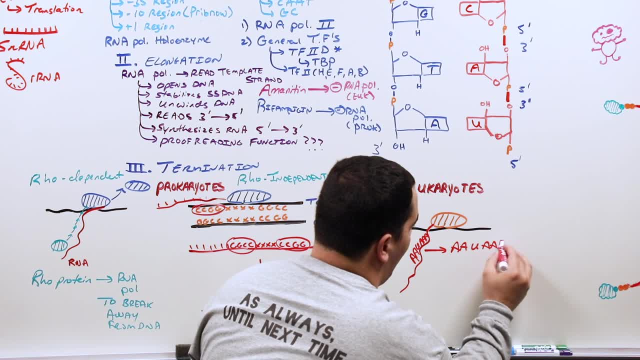 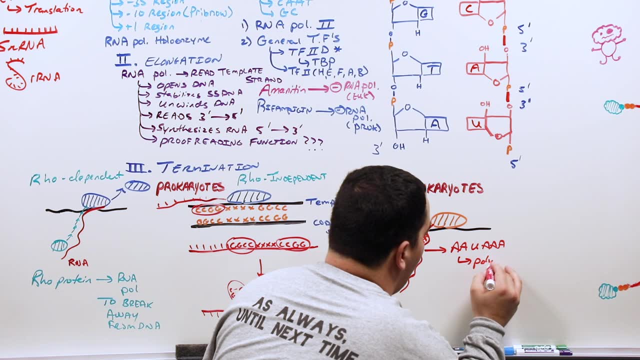 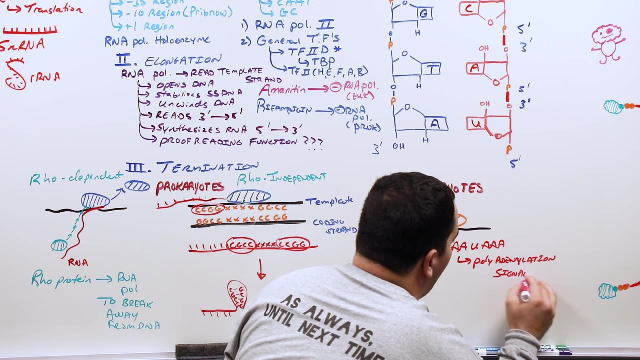 This portion here will be AAUAAA. This is what's called a polyadenylation signal. So what is this called here? This is called a polyadenylation signal And once this kind of nucleotide sequence occurs, so it's kind of now that we know what that nucleotide sequence is. 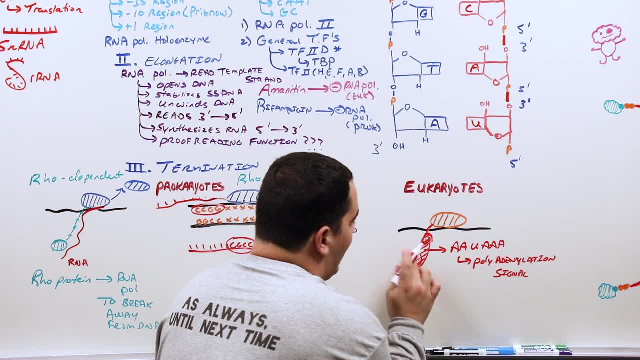 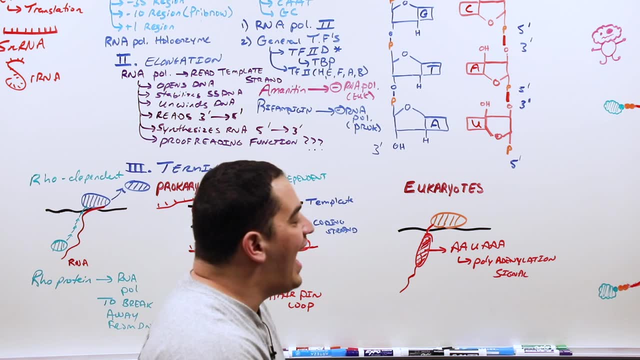 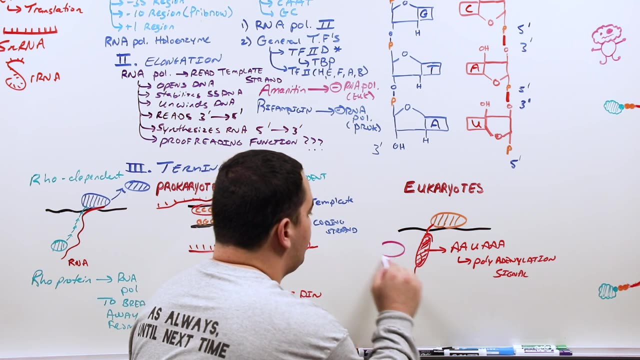 let's kind of just put it like this: Here's that nucleotide sequence, that polyadenylation signal that's been synthesized or formed by the RNA polymerase with the eukaryotes. Once that happens, it activates particular enzymes And those enzymes will come to the area here. 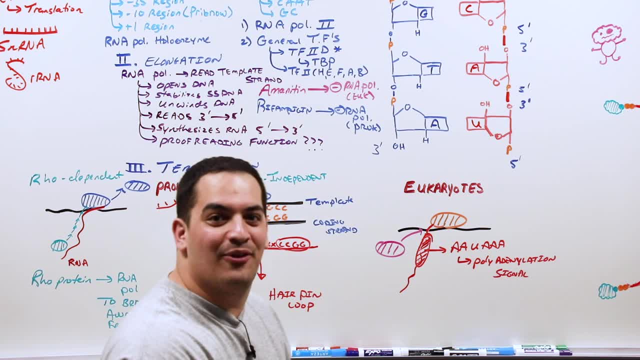 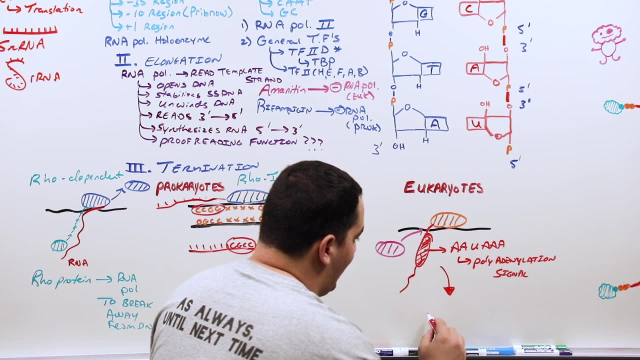 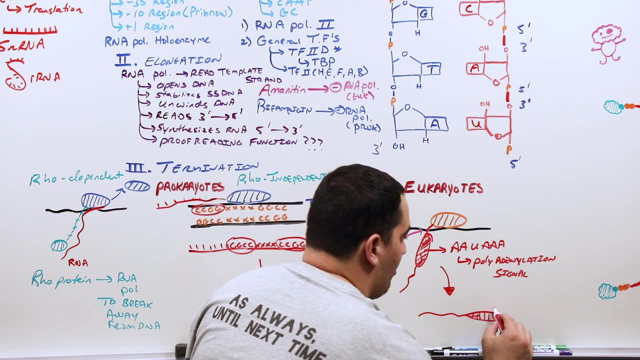 and cleave the RNA away from the RNA polymerase, separating out this RNA away from the DNA and the RNA polymerase. And then again, what will I have at this portion here, Just as kind of a diagrammatic portion here. this will be my polyadenylation signal. 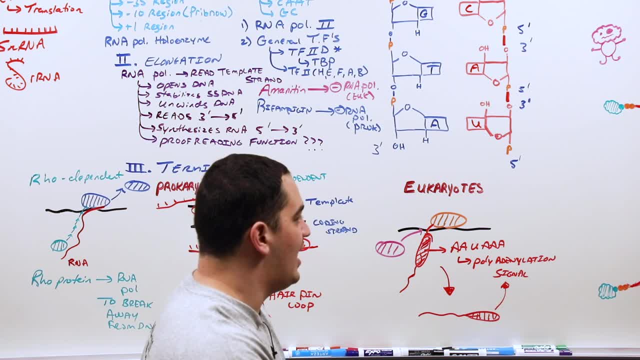 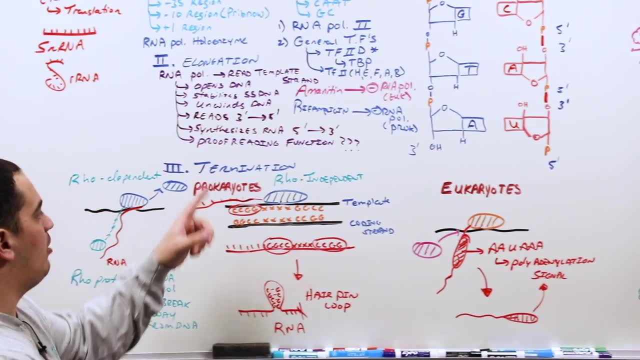 And this is important because we're going to talk about post-transcriptional modification. So I know this was a lot of crap. Just really quickly recap, because this is one of the toughest parts of transcription is termination Prokaryotes. there's two ways. 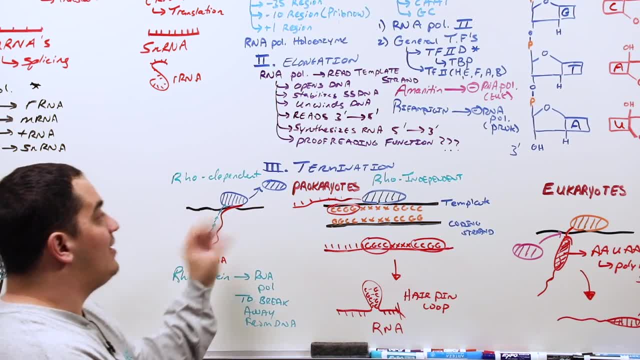 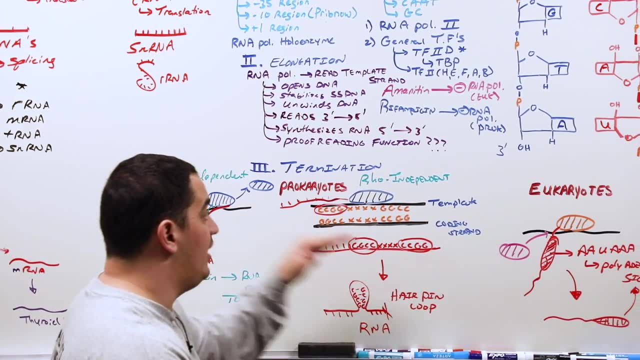 Rho-dependent, Rho-independent. With this one, you need a Rho protein to knock the RNA polymerase off. If you don't have him, he can't make any more RNA. The other one is Rho-independent. You don't have a Rho protein. 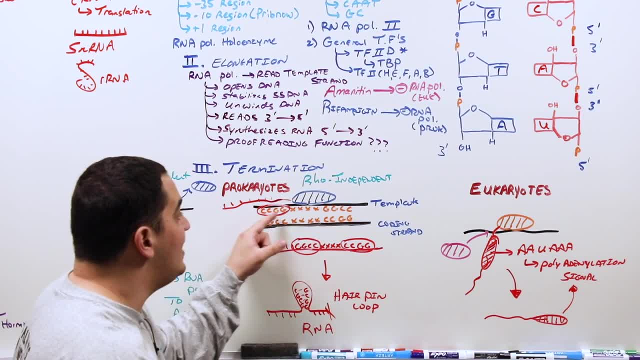 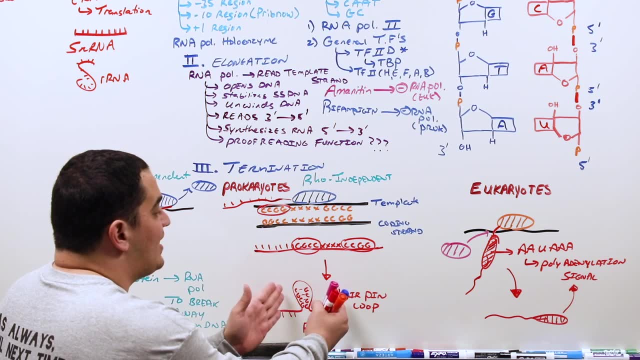 The RNA polymerase is reading the DNA and making RNA, and it hits these areas of inverted repeats. These inverted repeats, when they're made within the RNA, it creates a hydrogen bond interaction between them which causes it to loop, forming a hairpin loop. 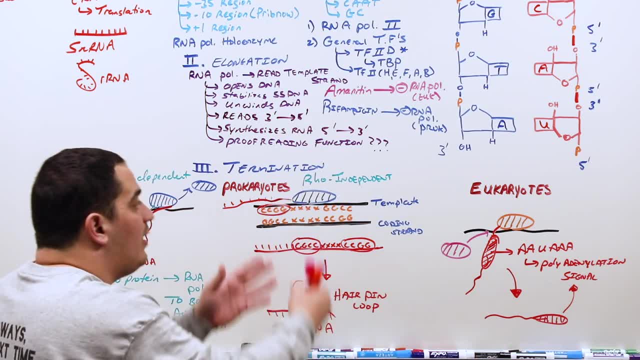 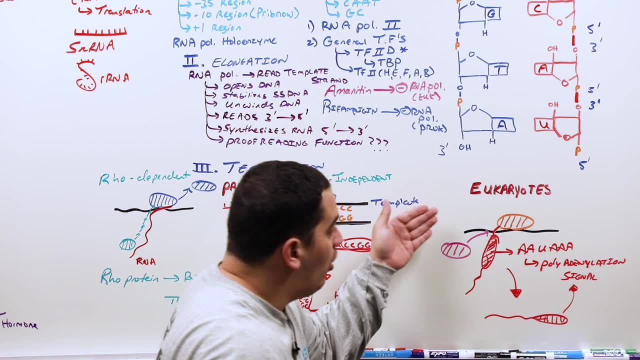 That signals particular enzymes to break the RNA away from the RNA polymerase, and we've made our RNA there. The last one is in eukaryotes. The RNA polymerase is reading the DNA and it reaches a particular sequence of nucleotides where it reads: 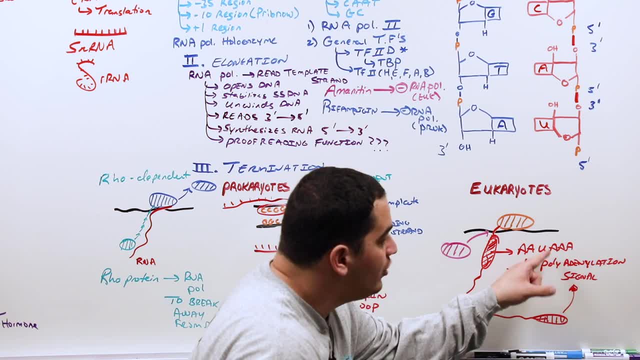 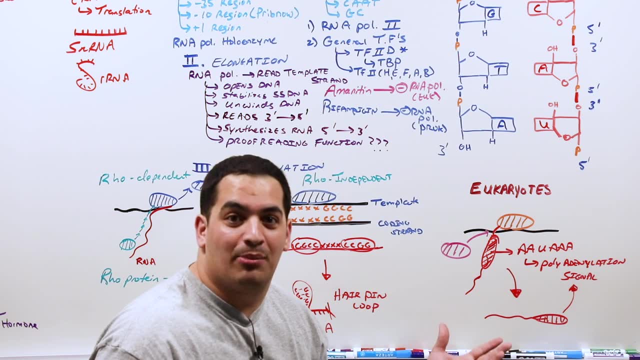 and then makes AAU triple A, A polyadenylation, A polyadenylation signal which activates enzymes to come cleave the RNA away from the RNA polymerase, terminating the transcription process. That really hammers this home. Let's now talk about post-transcriptional modification. 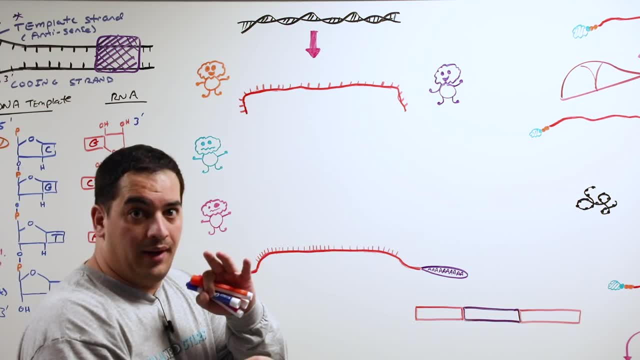 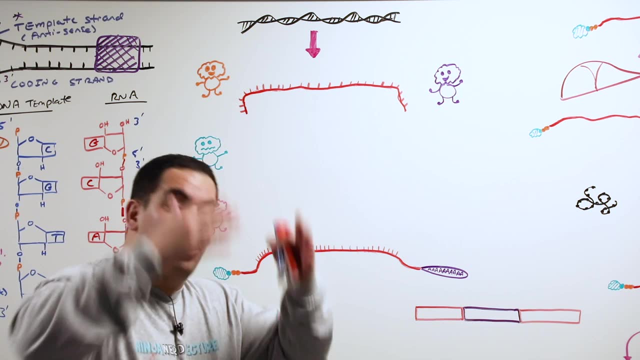 We know at this point how to take DNA and make RNA. We talked about all the different types of RNA, utilizing the RNA polymerases, utilizing the transcription factors. We talked a little bit about gene regulation. We even went through all the stages of transcription. 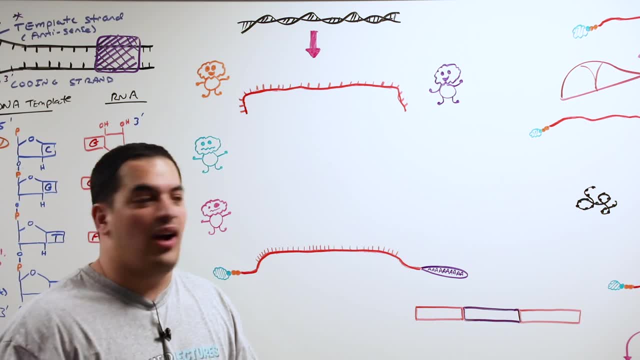 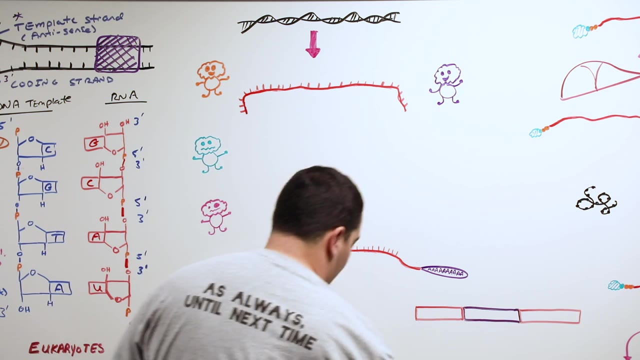 taking the DNA and making the mRNA all the way up until the point where we finally made the mRNA and broken it away from the DNA. Unfortunately, that's not it for transcription. Now we have this mRNA. Basically, what have we covered up to this point? 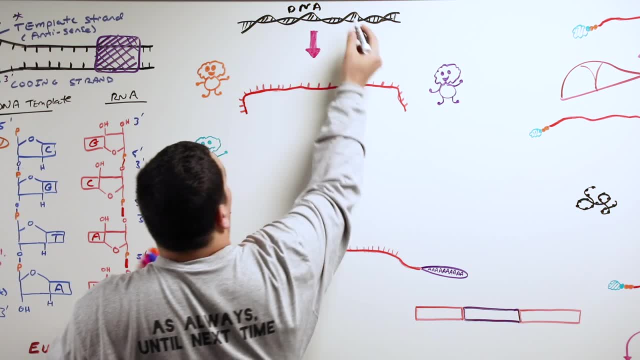 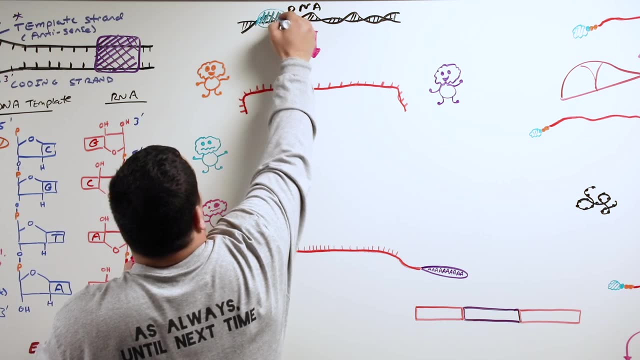 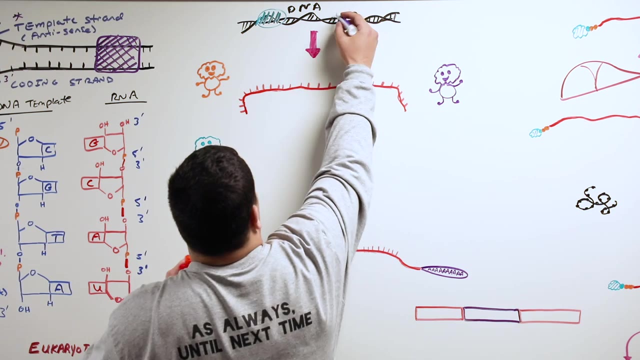 We took the DNA, We read: let's just say here, at this portion I'll just put: here's our promoter. Our RNA polymerase has read this gene sequence. We hit a termination sequence. Let's say: here's our termination sequence. 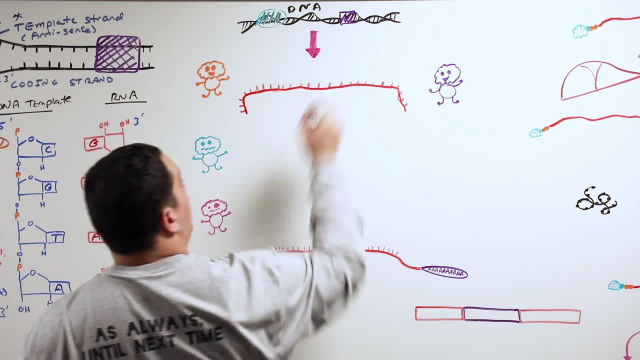 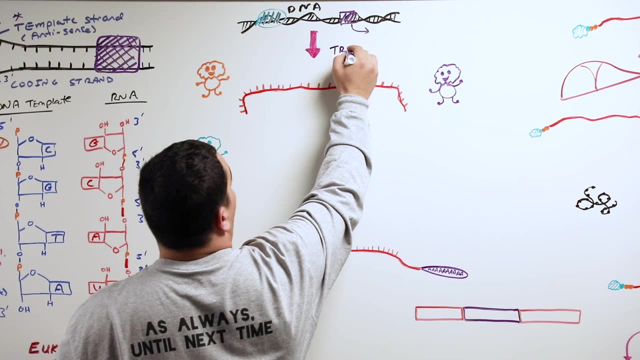 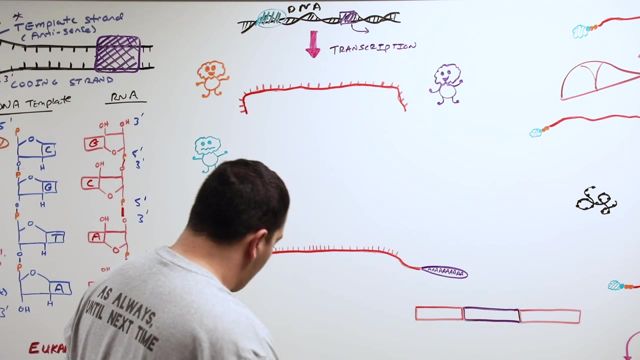 that we talked about here. Once we hit that termination sequence, the RNA polymerase will fall off. Then from this you'll make the RNA. This was pretty much the basic aspects of the transcription. Now we got to modify this. Here's the thing. 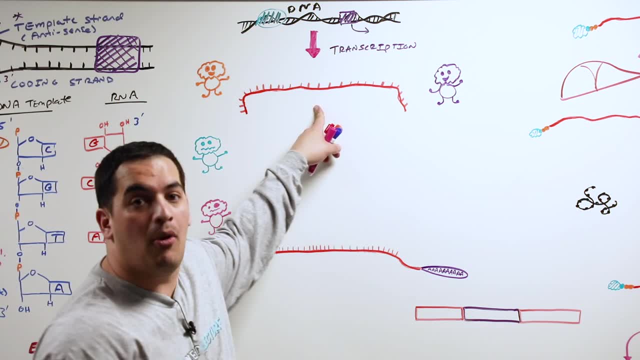 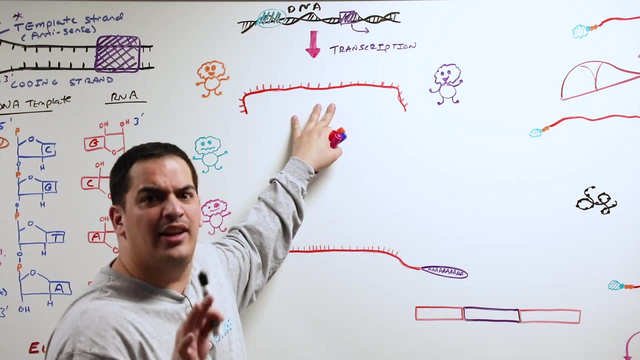 It's actually kind of a misnomer to say that this is mRNA. It's technically not mRNA right now, This piece of RNA that we made and this process of post-transcriptional modification- this only occurs. that's very important. 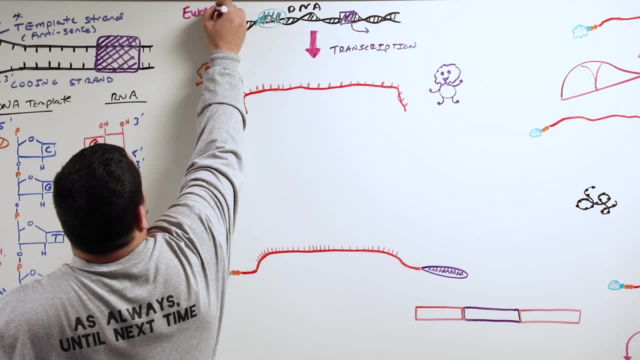 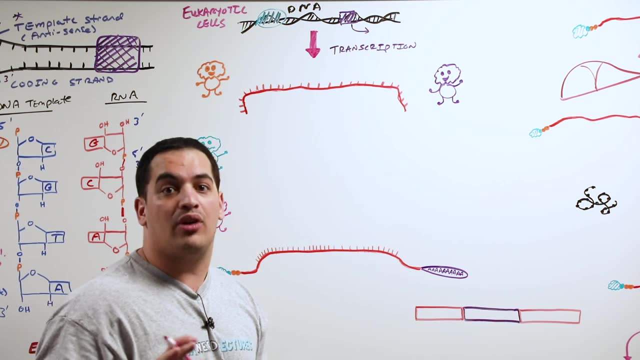 Let me actually write this down. This only occurs in eukaryotic cells. That's nice. All this stuff that we're going to talk about here is only in eukaryotic cells. It doesn't happen in prokaryotic cells. 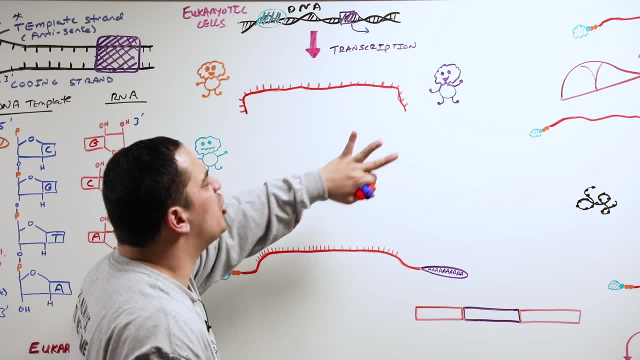 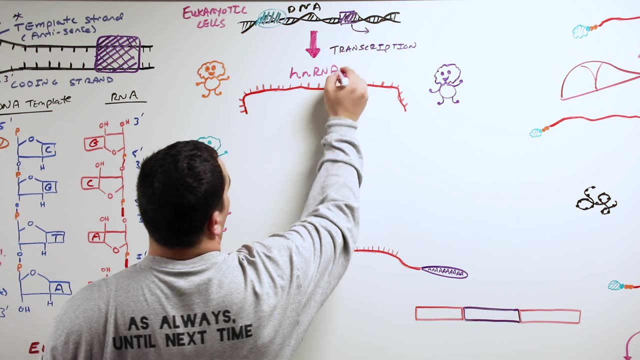 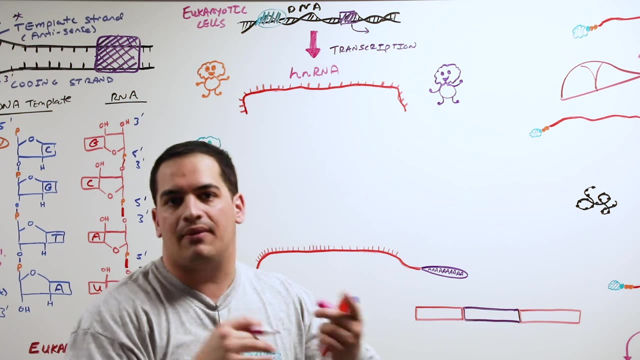 They just make their RNA and that's it Technically, this immature mRNA, if you will. we actually give it a very specific name. We call it heterogeneous neutral mRNA. Now, this heterogeneous nuclear RNA is kind of an immature mRNA that has to go through some modifications. 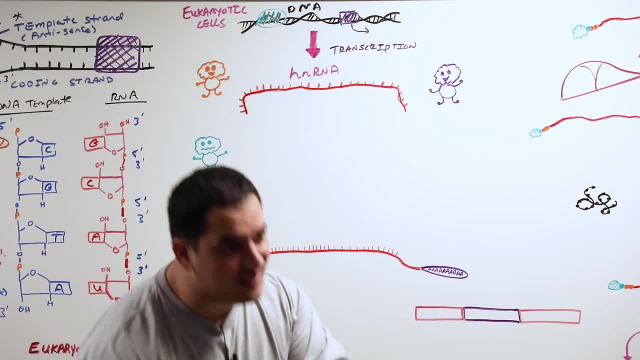 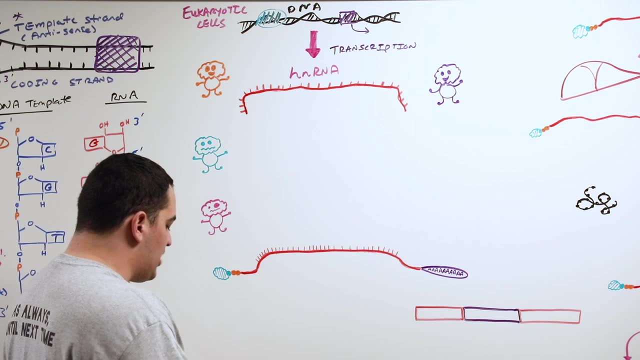 to really make mature mRNA that then can be translated to make proteins. What are those modifications? The first thing that we have to do is we have to put something on one of these ends. Now we got to know a little bit about the terminology. 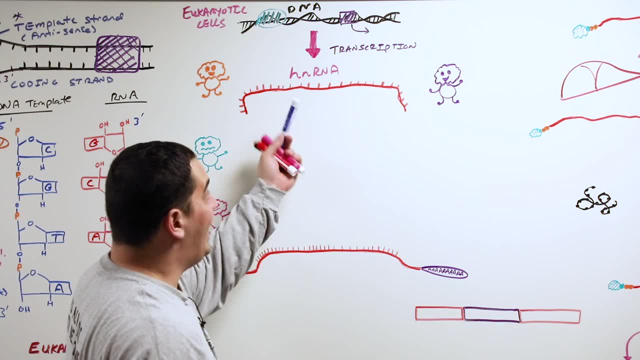 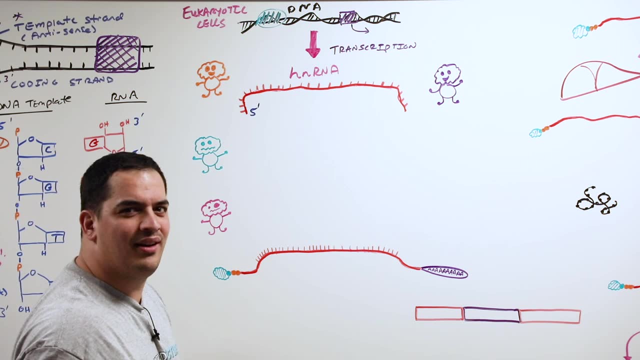 of the ends of this immature mRNA or hnRNA On this end? we're going to call this the 5' end. What's on that 5' end? Do you guys remember The phosphate groups? What's on this end? 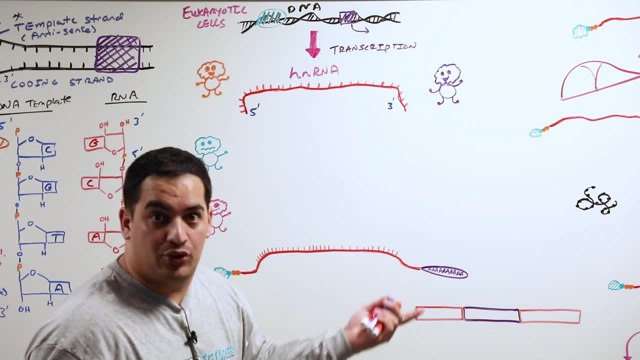 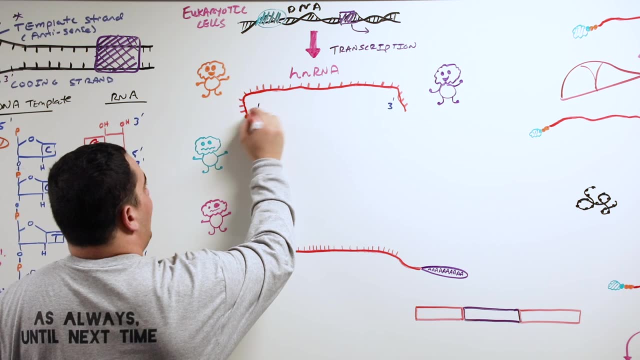 The 3' end. What's on the 3' end? The OH group. Okay, Now something very interesting is on the 5' end. On the 5' end of this heterogeneous nuclear RNA, or the hnRNA, you have a triphosphate. 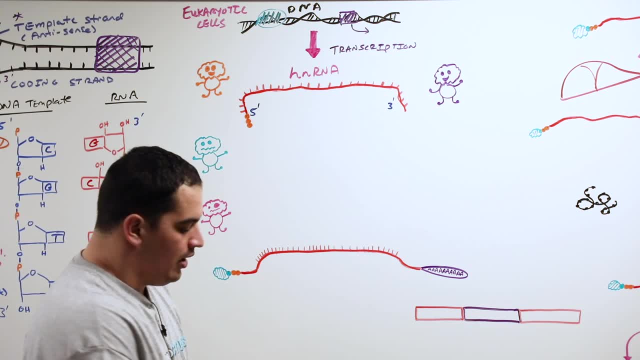 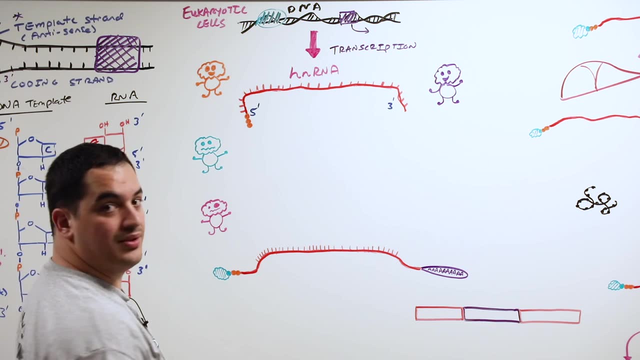 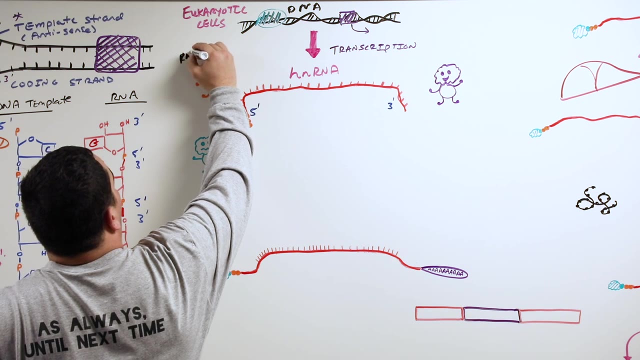 which we're representing here with these orange circles. An enzyme comes to this end, goes into the rescue and cleaves off one of those phosphate molecules. What is that enzyme called? It's this orange, little cute enzyme. This orange enzyme is called RNA triphosphatase. 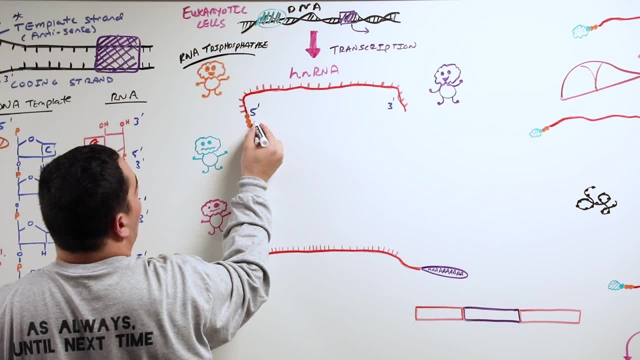 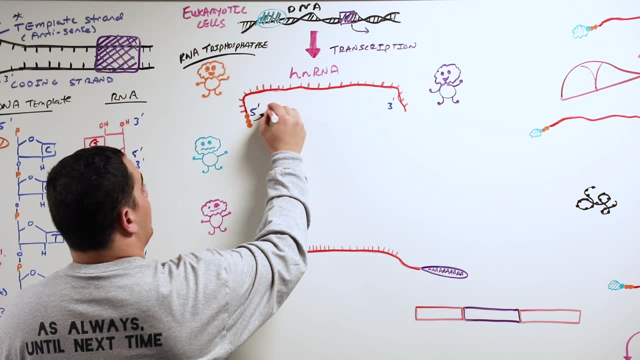 And what it does is it comes and cleaves off what portion. It cleaves off one of these phosphate groups. It's going to cleave off one of the phosphate groups, So we only have two phosphates on the end of this 5' end. 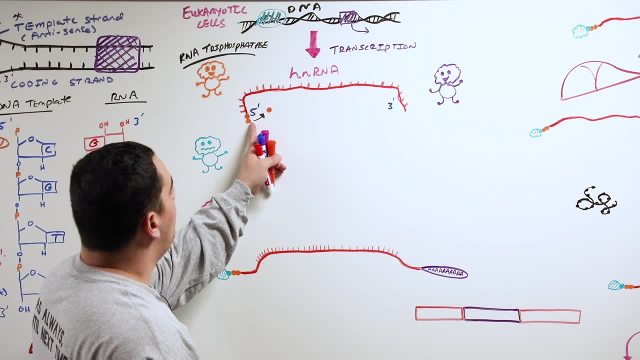 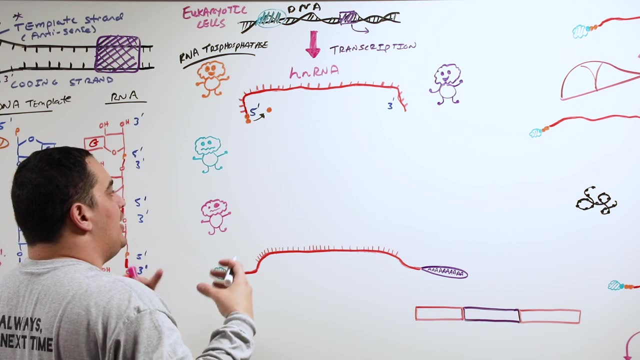 Then another enzyme comes in And it says: hey, there's only two phosphates here. I can now add something on here, And I'm going to add on what's called a GMP molecule. What am I going to add on again? 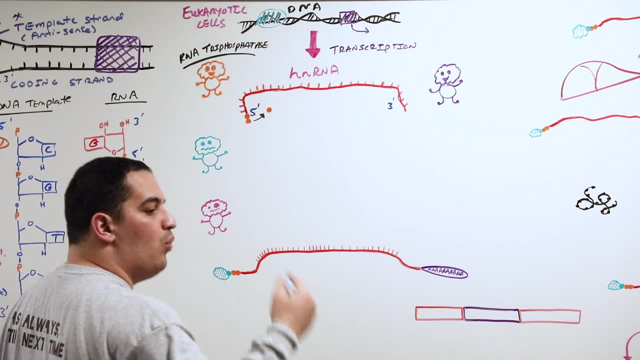 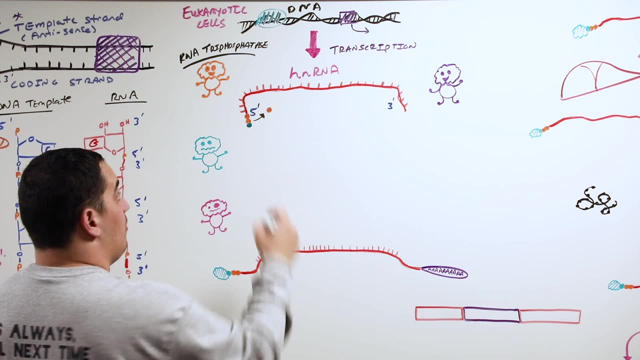 I'm going to add a GMP molecule which is guanosine monophosphate. So we're going to represent that here, which we add on the phosphate for the guanosine monophosphate, And then we're going to just represent this as the guanosine. 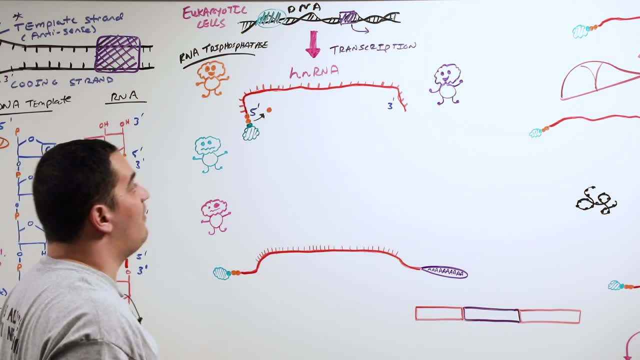 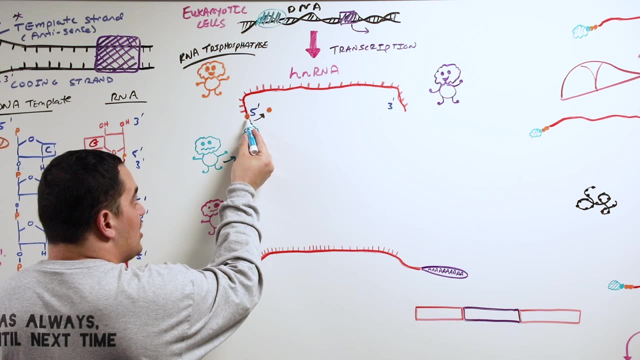 So this is our guanosine And that blue circle there is the phosphate on the guanosine. So what does he add on? Technically, he adds on to this little two phosphates. It adds in GTP. But when it does that, 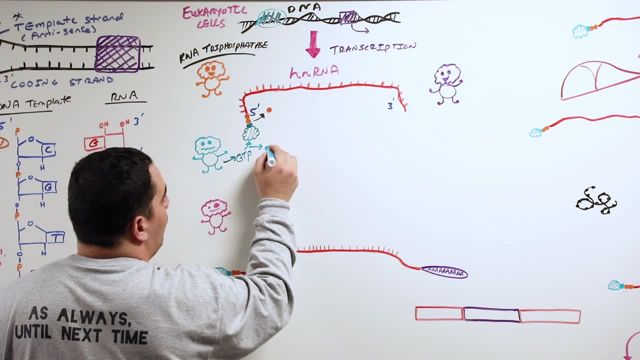 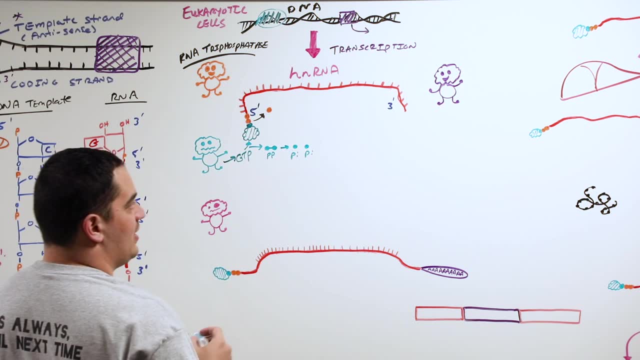 two phosphates are released in the form of pyrophosphate, which then get broken down by pyrophosphatase into individual phosphates. So if I took GTP and I removed two phosphates, what am I left with GMP? 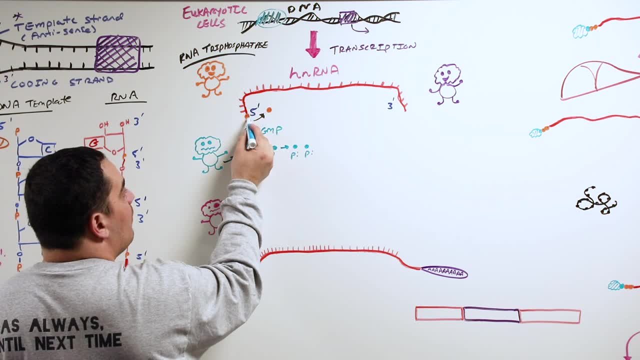 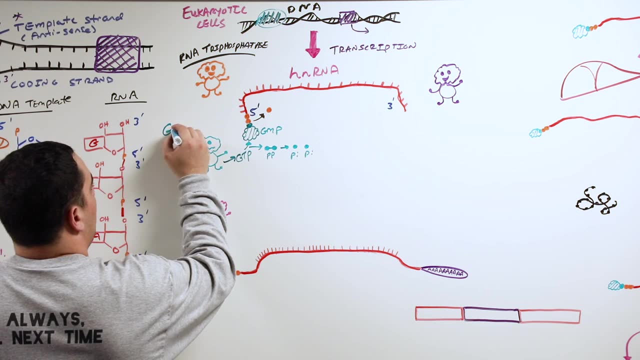 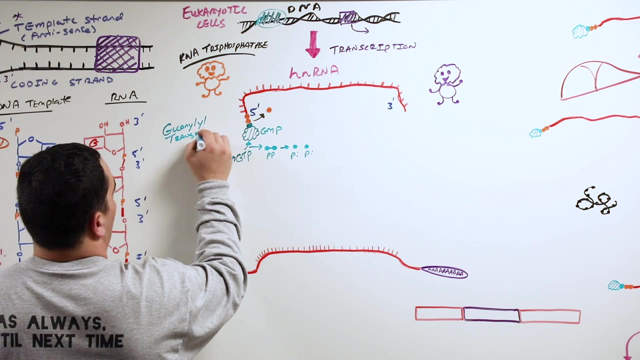 So it adds on this GMP group onto that two phosphate end on the five prime end. So this enzyme that adds that GMP on in the form of GTP is called guanylyl transferase, Guanylyl transferase. 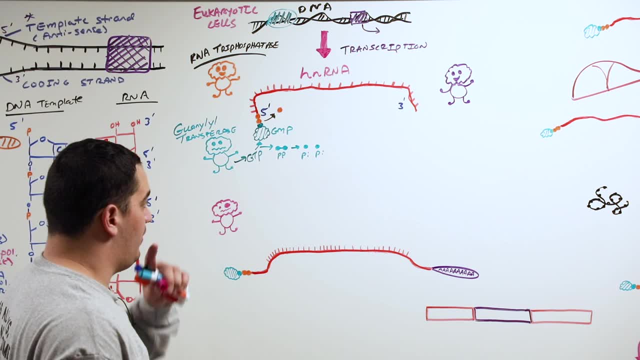 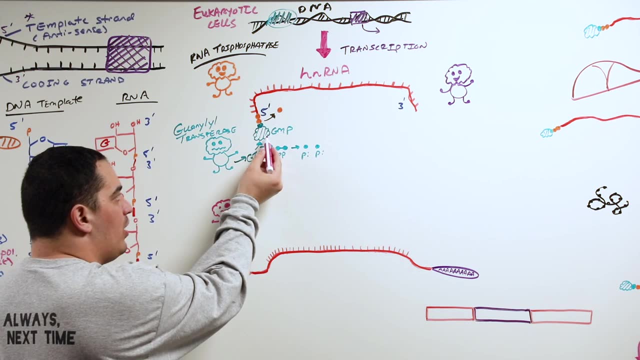 Beautiful. So this last enzyme here, which is involved in this step here on the five prime end, is going to add on a methyl group onto one of the components of the guanosine monophosphate. It's actually like one of the seventh components on that structure. 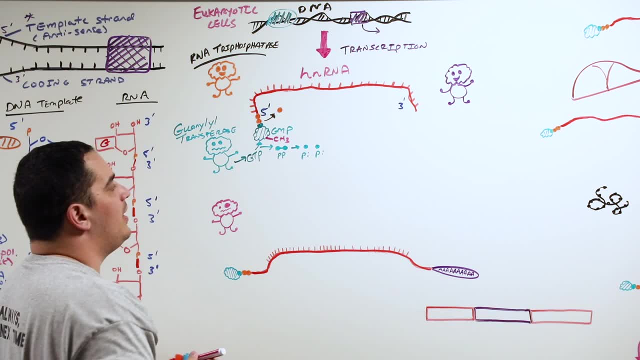 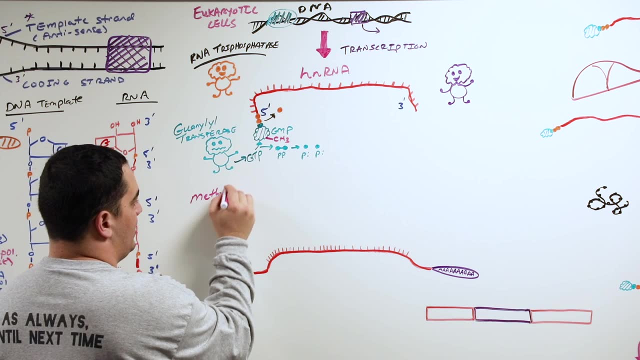 It adds on a methyl group. And so, at the end of this, this enzyme which adds a methyl group, on what do you think? it's called Methyltransferase. At the end of this process, we took the five prime end. 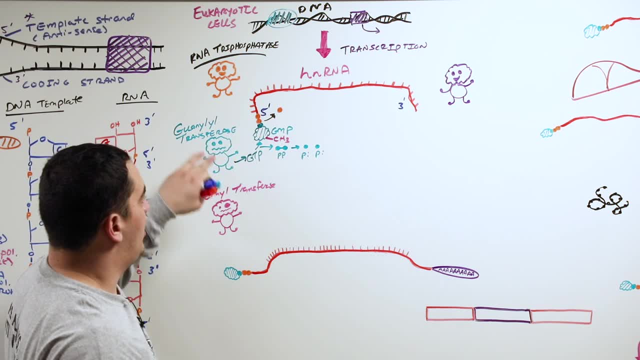 which had three phosphates, got rid of one. took the guanylyl transferase, added on the GMP, took the methyltransferase, added on that methyl group. You formed this complex here and we call this whole complex that we just added on. 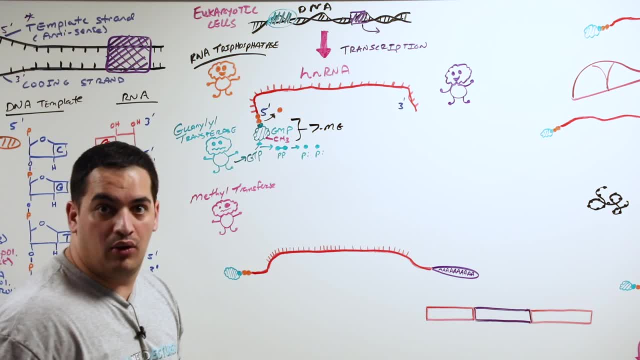 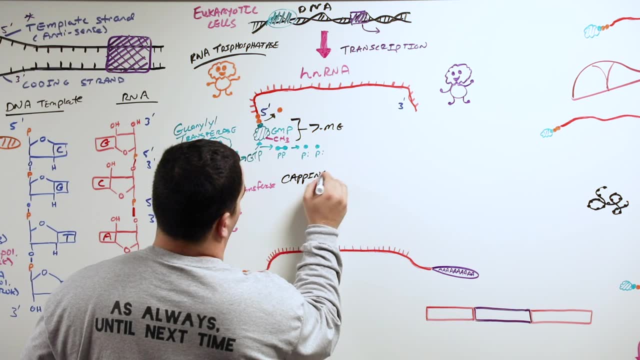 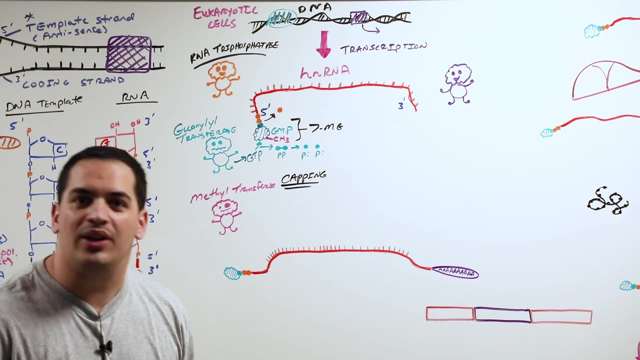 a seven methyl guanosine group. Okay, And that's on that five prime end. This is called capping, This is called capping. So whatever we've just done on this five prime end is called capping. What the heck do we do all this stuff for? 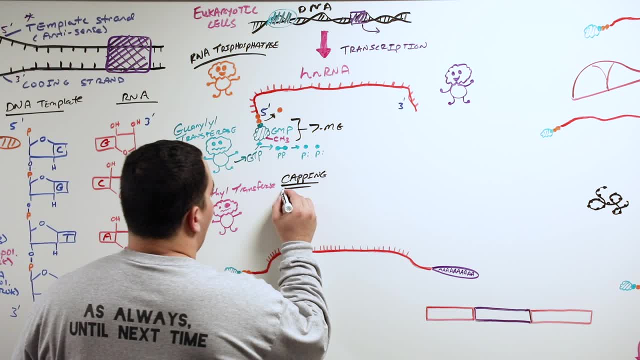 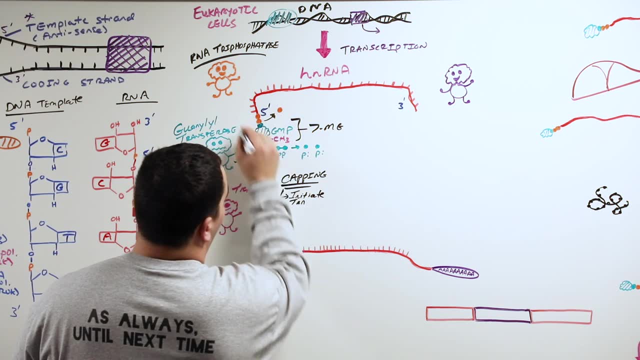 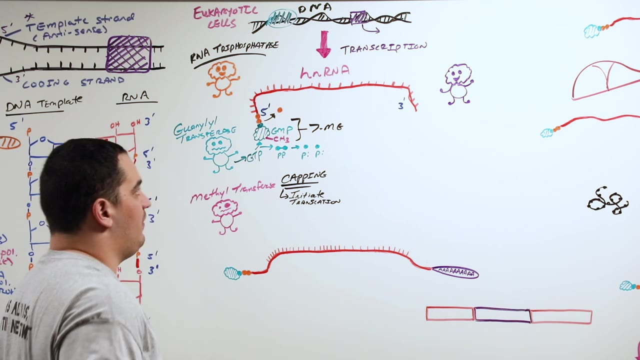 The whole purpose of capping is to help to initiate translation. So this sequence, this kind of five prime end with that seven methyl guanosine, or that five prime capping, if you will, it's kind of a signal sequence, if you will. 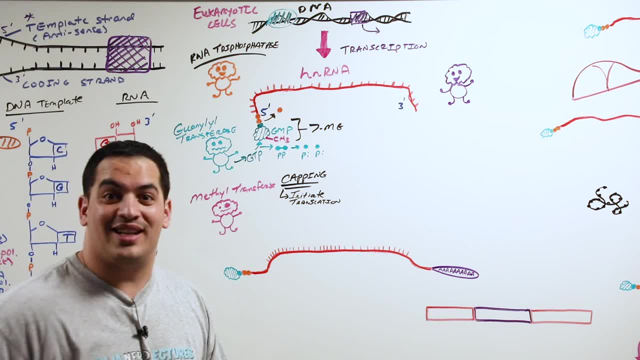 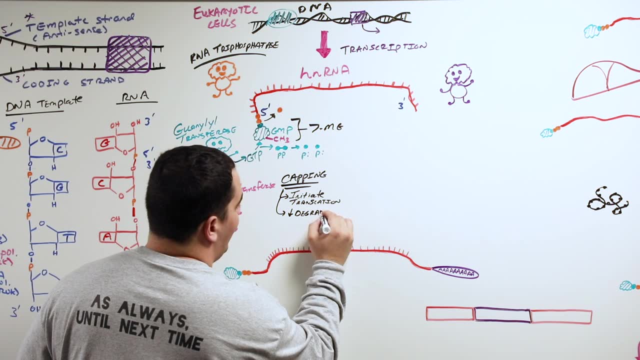 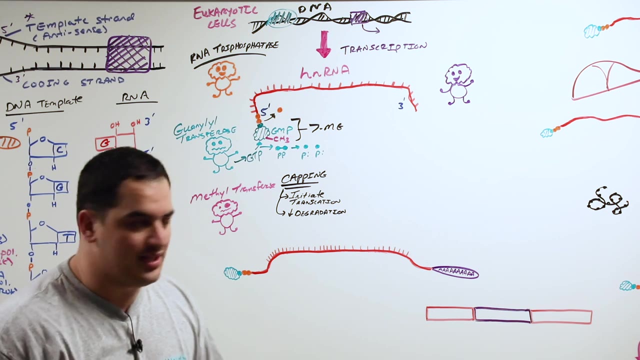 that allow for it to interact with the ribosome and undergo translation. The other thing it does is it prevents degradation by nuclease enzymes that want to come and break down the RNA. So it helps to prevent degradation, helps to initiate the translation process. 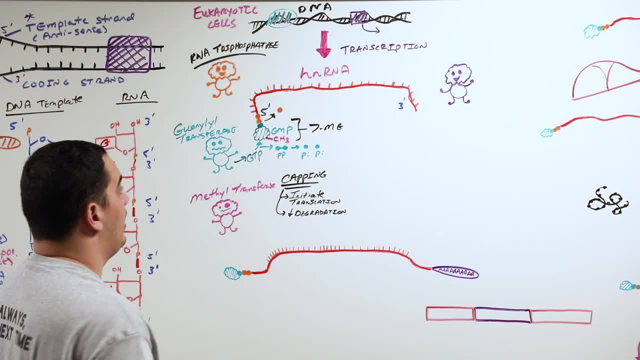 One more thing that they- it's a dumb thing to know, but they love to ask it- is that there is a particular molecule that this methyltransferase uses to add that methyl group on, And sometimes it's really important to know it. 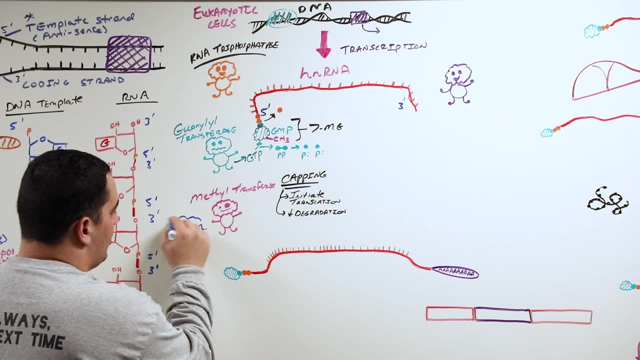 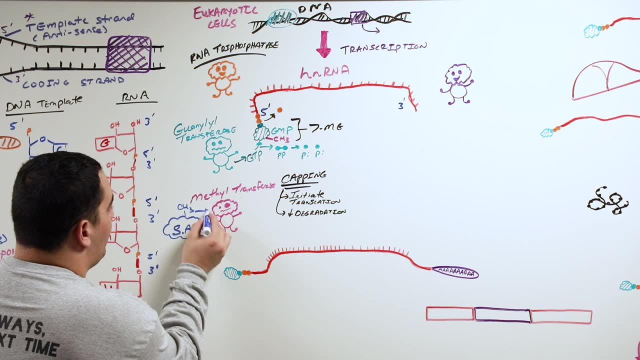 And this is called S-adenosylmethionine, also known as SAM. SAM carries a methyl group. It's like a methyl donor, if you will. It gives that methyl group to the methyltransferase and the methyltransferase adds that methyl group. 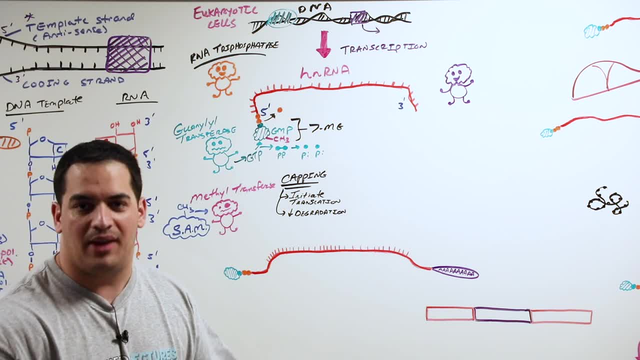 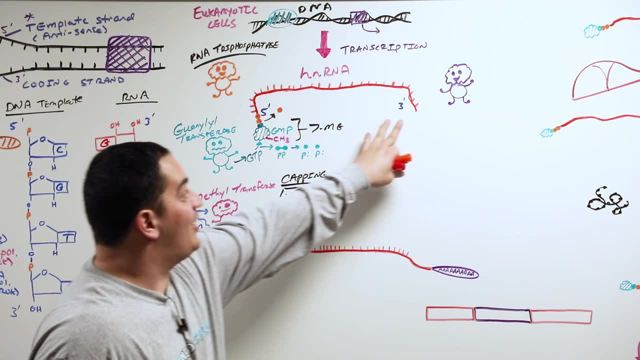 onto the guanosine monophosphate, forming the seven methyl guanosine or that five prime cap. Okay, So that's the first thing that happens. Now we got to talk about the three prime end. On the three prime end, 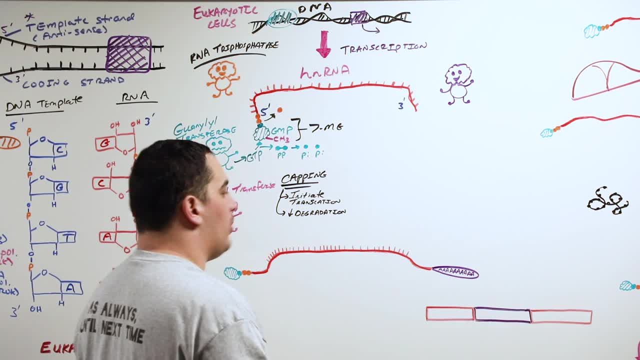 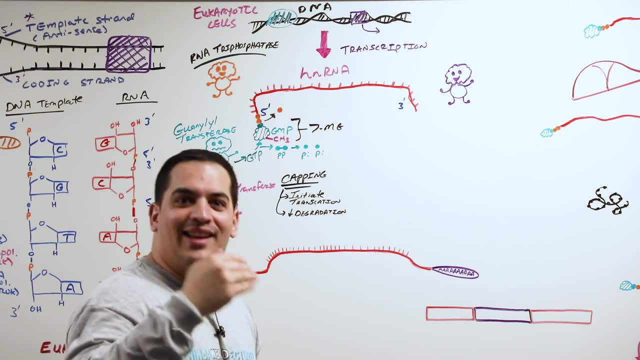 we had that OH group right. That's the OH end. But do you remember in eukaryote there was a particular signal that generated that terminated transcription. What was that? nucleotide signal. Do you guys remember? Test your knowledge, guys. 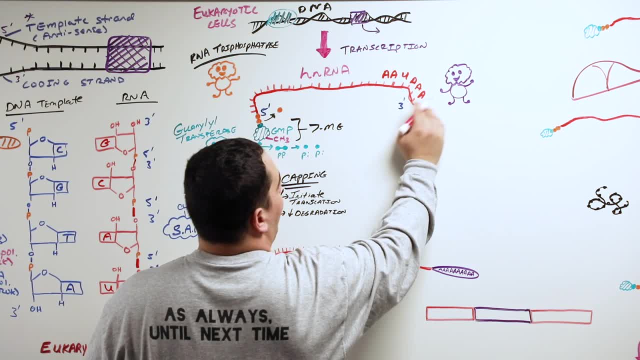 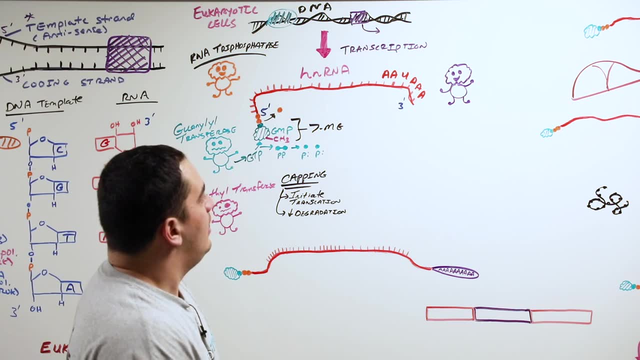 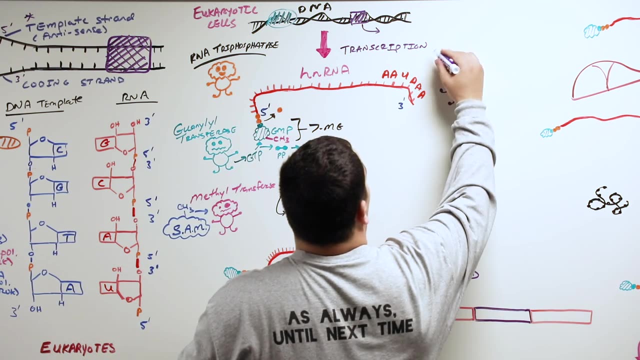 AAUAAA. right, That was that polyadenylation signal. Do you guys remember that? The polyadenylation signal we talked about in eukaryotes? That polyadenylation signal is recognizable by this cute little purple enzyme. here, This cute little purple enzyme: 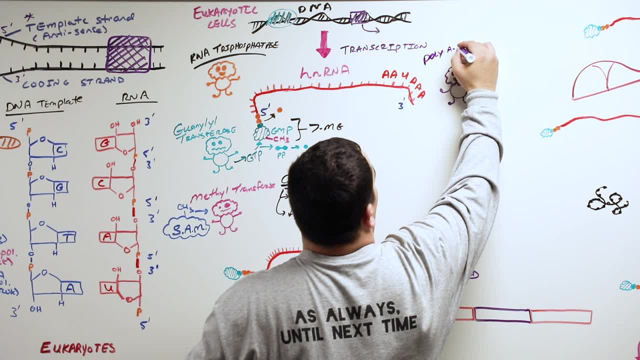 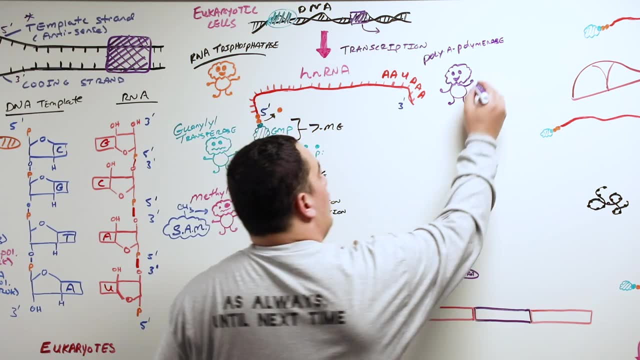 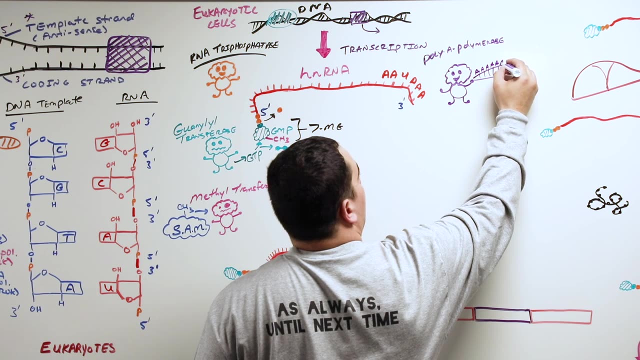 is called poly-A-polymerase. It's called poly-A-polymerase. What it does is is: on this hand, it has a bunch of adenine nucleotides, right? So it contains a lot of nucleotides. 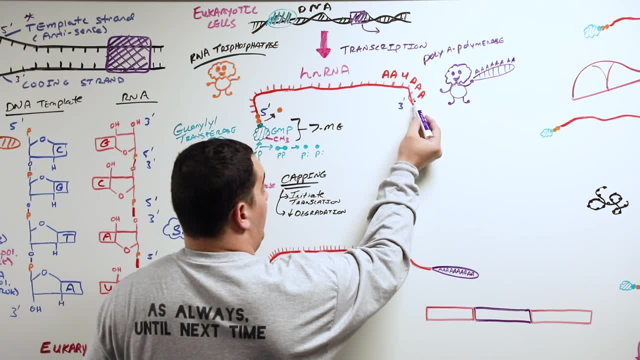 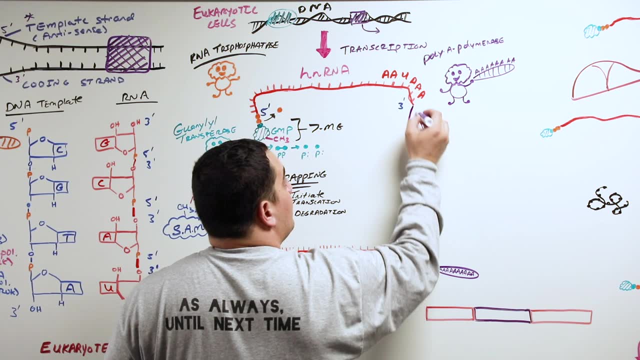 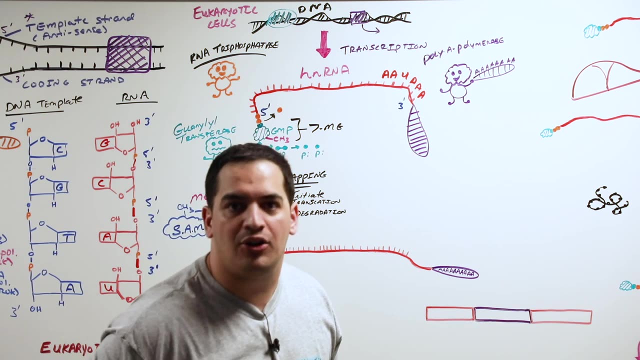 containing the adenine nitrogenous base. It takes one end and identifies that polyadenylation signal, takes the other end and adds on all of those adenine nucleotides, a bunch of them, sometimes up to 200 adenine nucleotides. 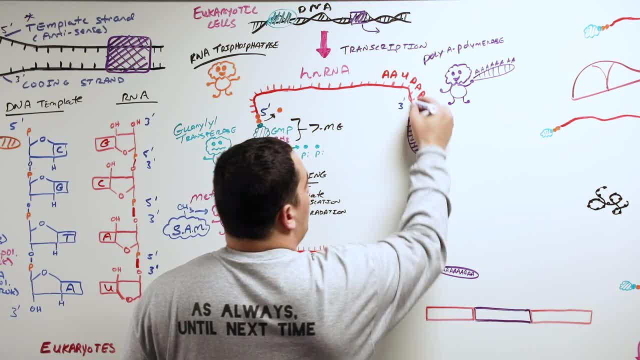 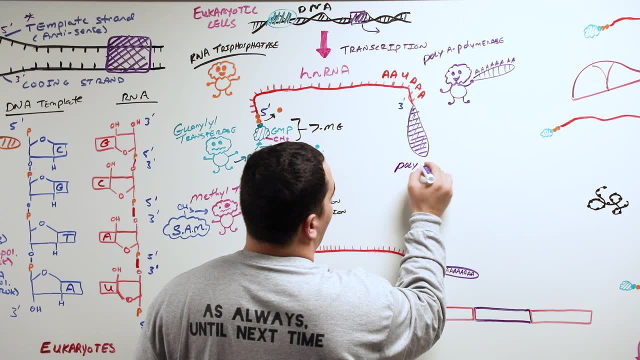 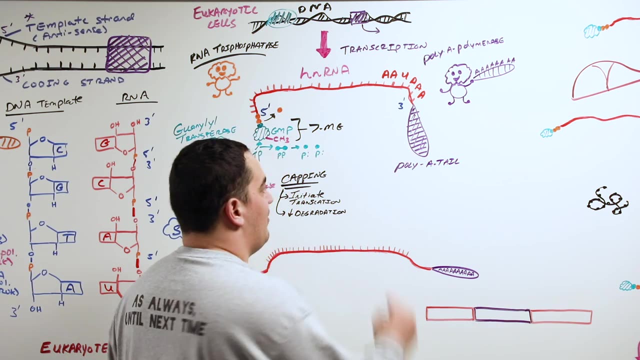 When it does that, this forms a tail on that three prime end with a bunch of adenine nucleotides and we call this the poly-A tail. So the poly-A tail- what's the purpose of this? It's the exact same thing. 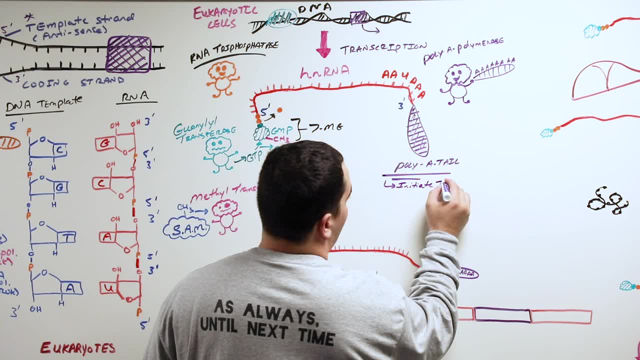 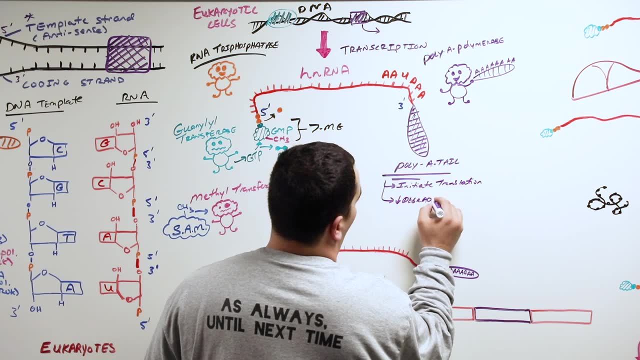 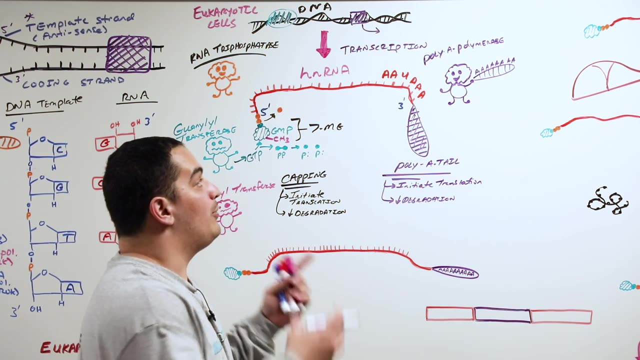 It helps to initiate the translation process and helps to decrease degradation. by what kind of enzymes, Nucleases that will try to come and break down that end? Okay, The other thing that they do is they help transport this HNRNA Eventually. 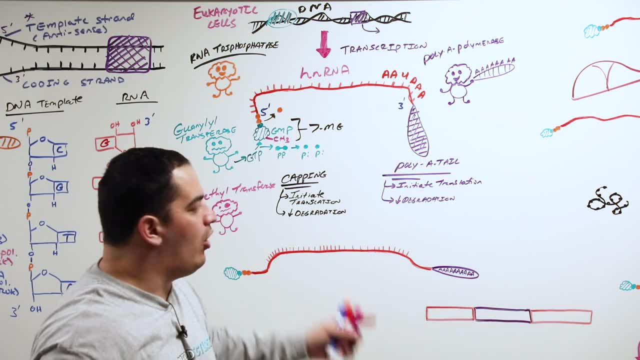 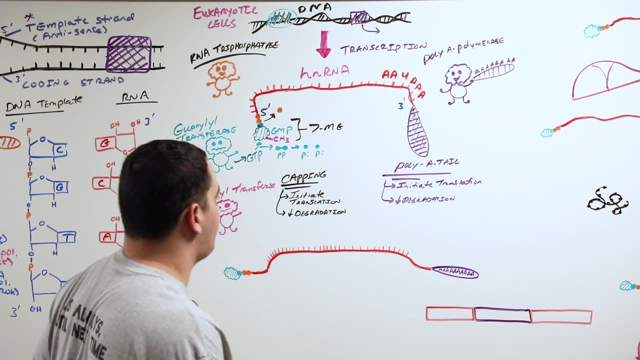 they're going to help to transport the HNRNA, which will become mRNA, out of the nucleus into the cytosol. So they also play a little bit of a role in transport out of the nucleus and into the cytosol. 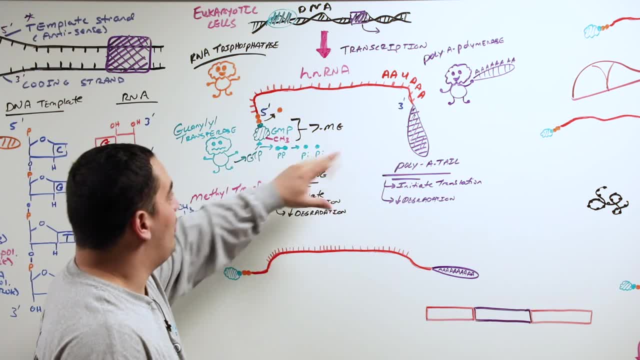 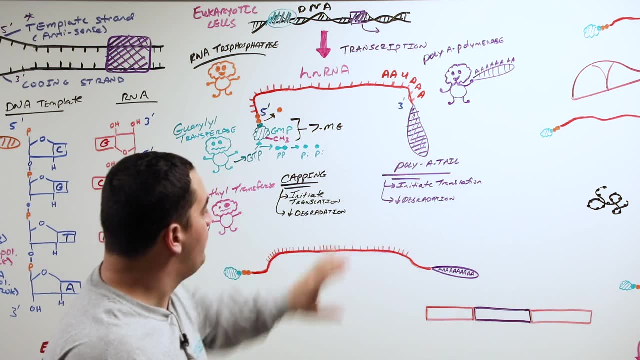 Okay. So, within this first step, what did we do? We did five prime capping, We went over that part and the three prime poly-A tail that we did. Okay, Now we have this. So, after we did all of this massive mess, 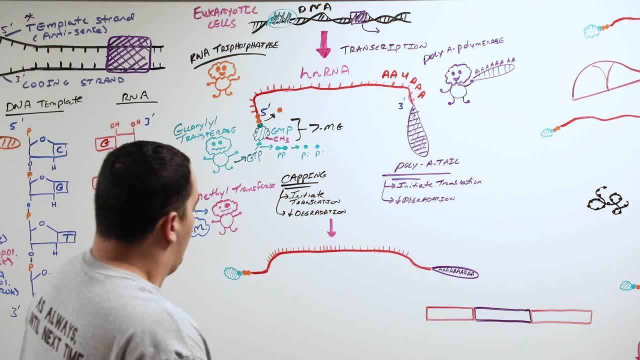 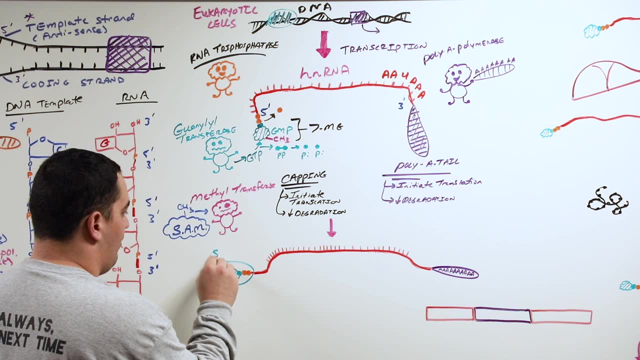 we've come to this point. Okay, On this part, what do we have? We're just going to write these, We're going to circle it here. This is our five prime cap with the seven methyl guanosine. And on this end, 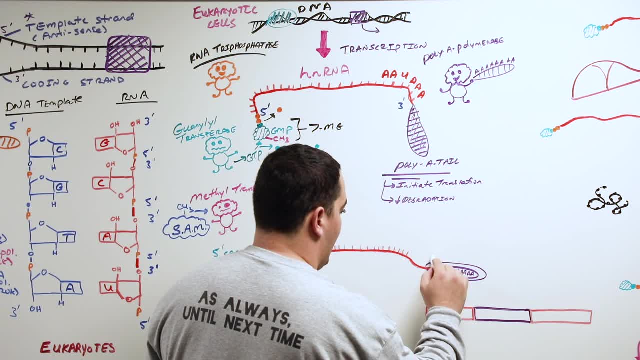 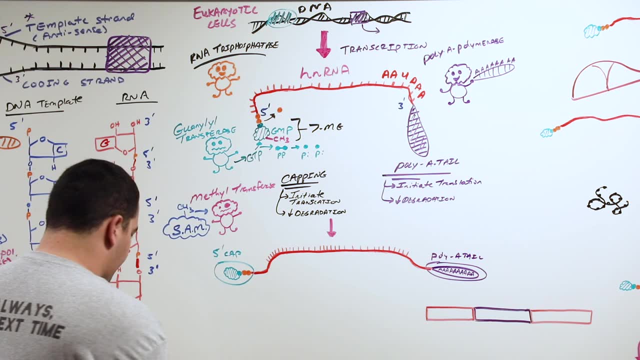 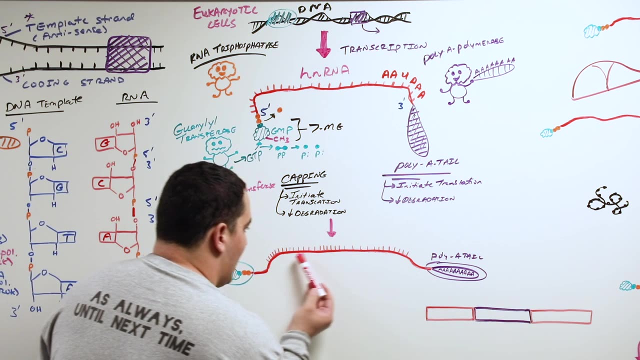 we already have kind of formed our poly-A tail. The next thing that happens is what's called splicing, And this can be sometimes a little annoying, but it's not too bad, I promise. Let's say here: this is the sequence of nucleotides. 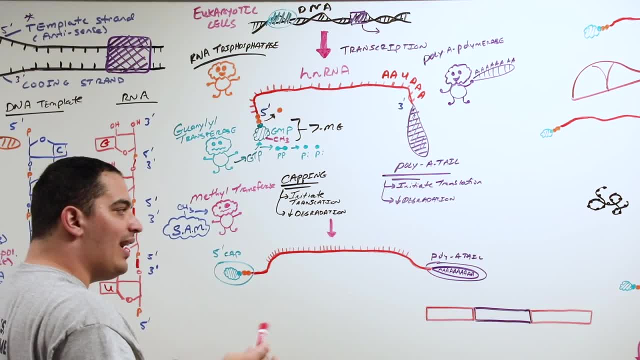 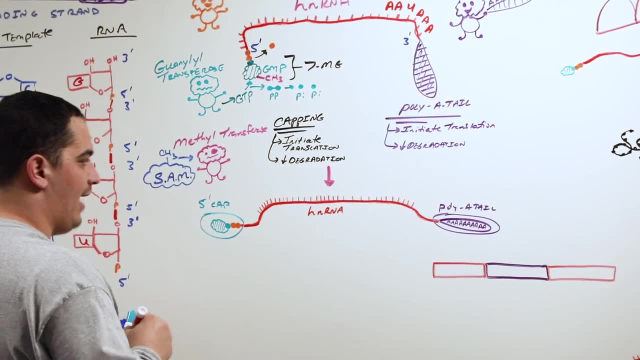 within this RNA. Okay, We're not at mRNA yet, We're still at this HNRNA. We're still kind of at this HNRNA at this point. We haven't made mRNA yet. Within this HNRNA there's particular nucleotides. 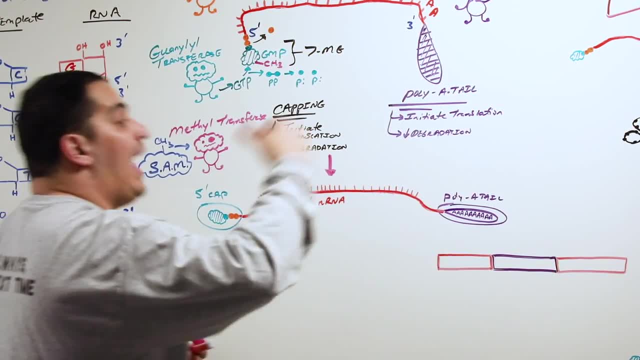 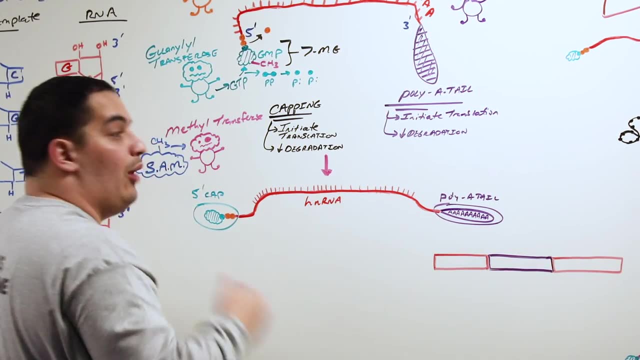 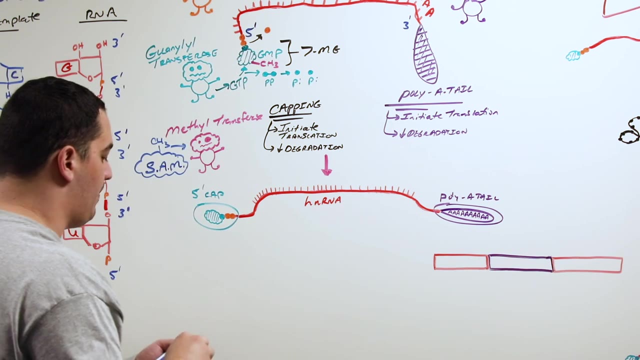 that will be read, translated, and actually will code for particular amino acids. There's other nucleotides within this HNRNA that will not be read and they do not code for a particular amino acid. We give those very specific names. I'm going to highlight them. 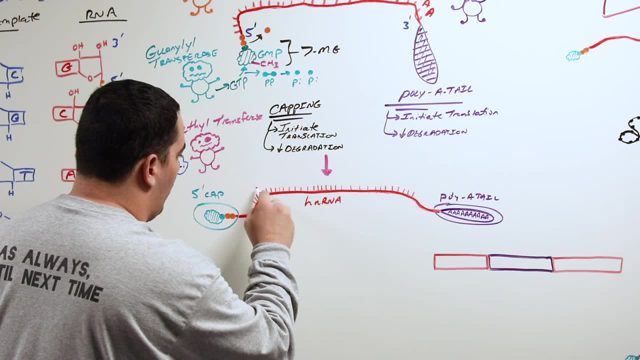 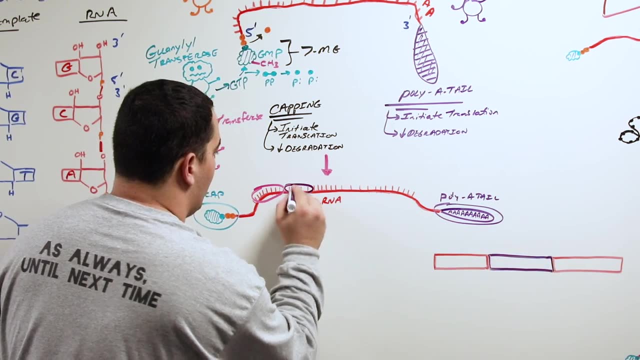 in different colors. So let's say, I highlight this one here in pink And then I will highlight this one here in this kind of maroon color, And then I'll pick here a blue And then we'll do another maroon color. 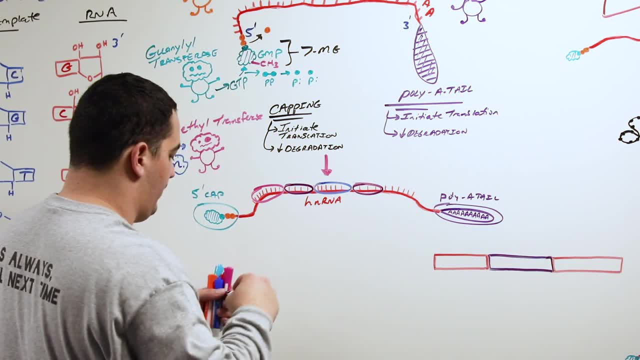 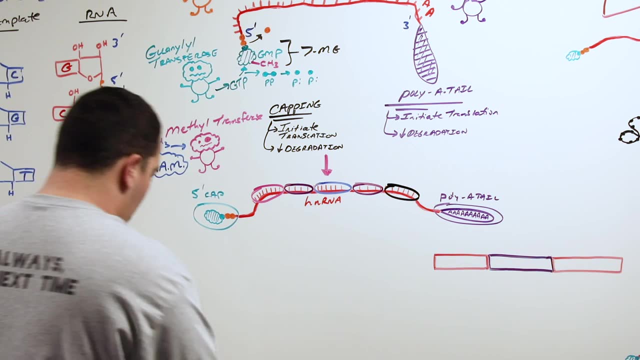 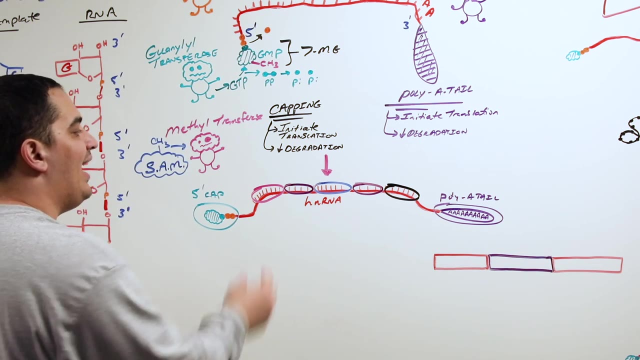 And then we'll do one more color after this. Here's another maroon, And then we will do, just for the heck of it, black. Okay, These portions here, the pink one. this is actually going to code for an amino acid. 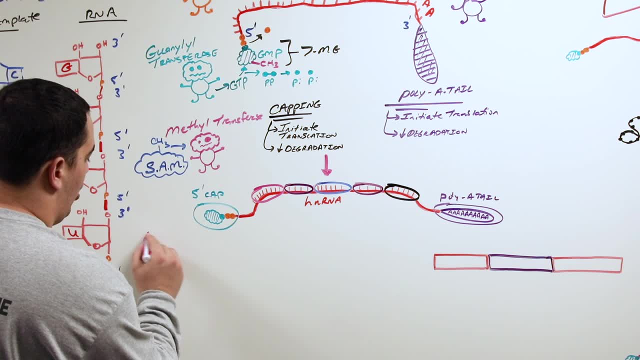 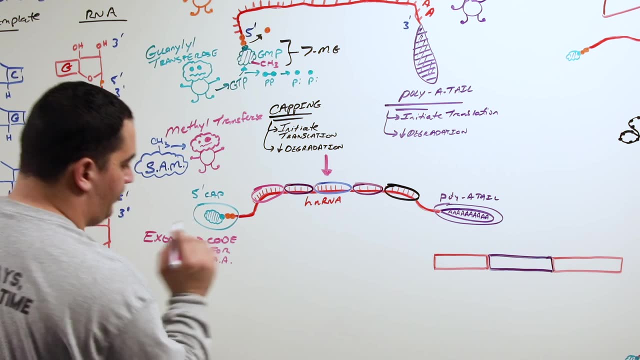 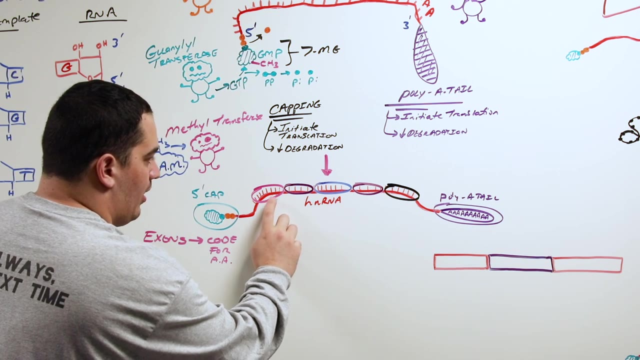 If it codes for an amino acid, we give a very specific name for that and we call it exons. So exons code for an amino acid. Okay, Particularly amino acids will make proteins, These other portions, and again that's going to be. 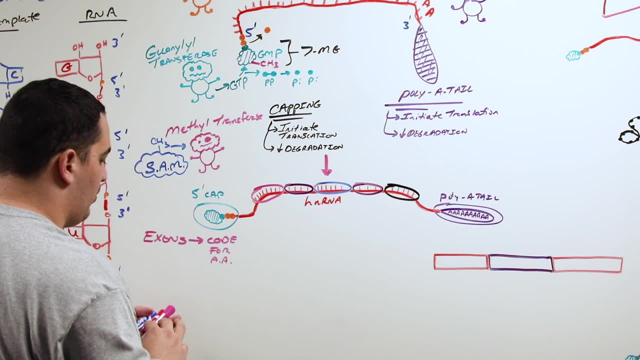 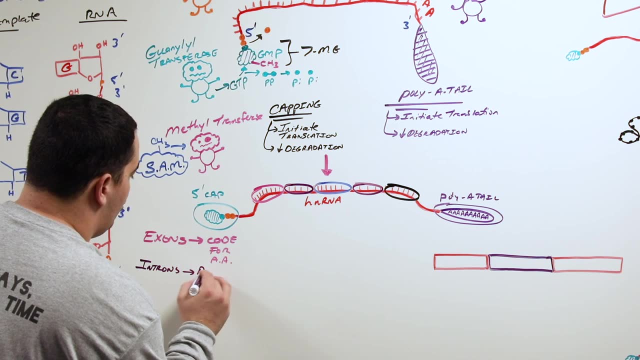 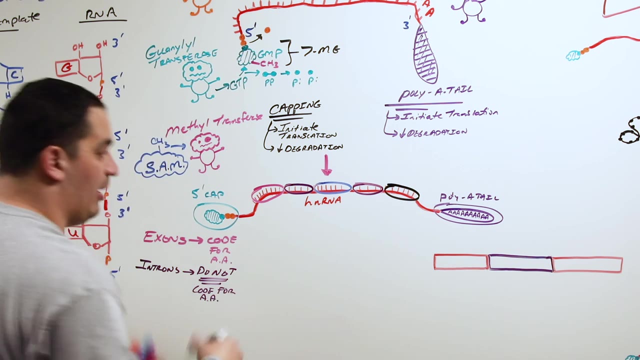 I'll mention which ones are exons and which ones are the next thing, which is called introns. Introns are basically nucleotide sequences that do not code for amino acids, which will help to make proteins Very important. I'm going to call this pink portion. 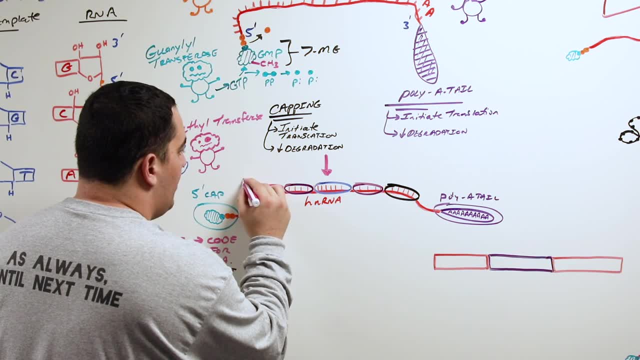 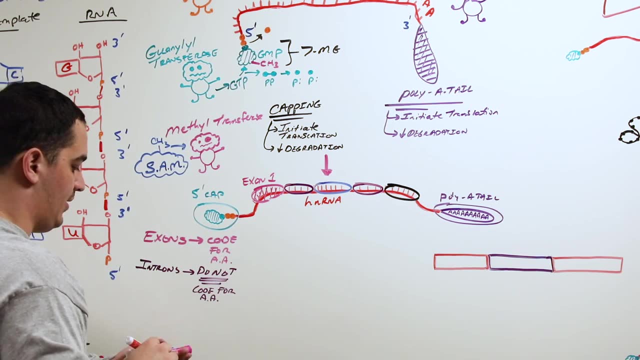 of the HNRNA. I'm going to call this an exon, but we have a bunch of them in this HNRNA, So I'm going to call this exon 1.. Okay, So that's going to code for some amino acids. 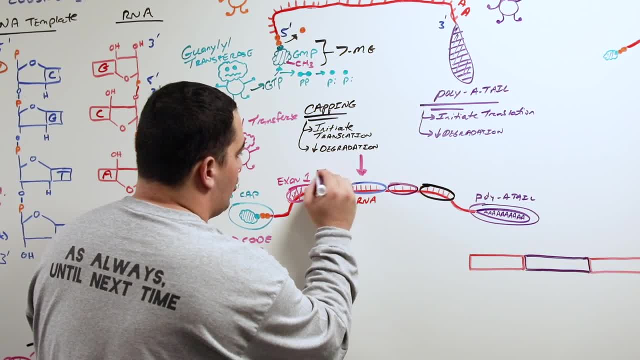 I'm going to have this portion here which is going to be in the maroon. I'm going to call this an intron, but you can have multiple introns, So I'm going to call this intron 1.. Same thing here. 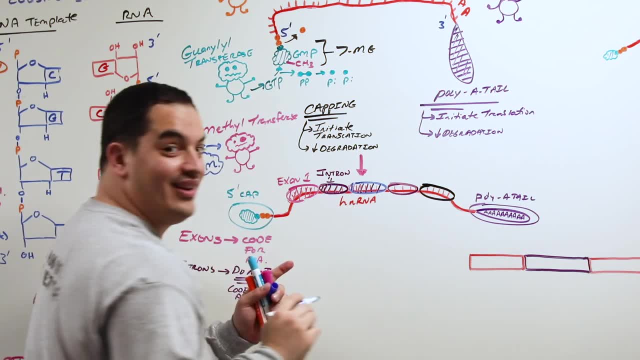 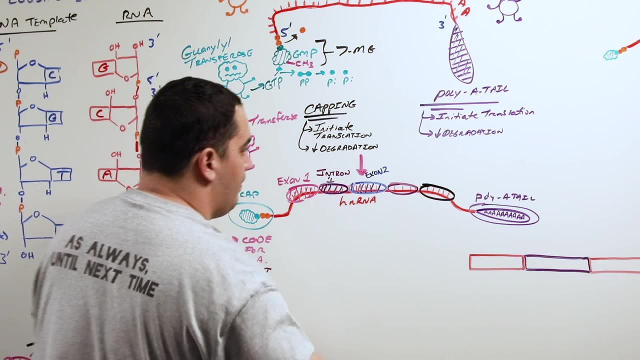 This is going to be coding. So if it codes, it's what? It's an exon, but we have multiple types, so we're going to call this exon 2.. Then I'm going to test you again. This one does not code. 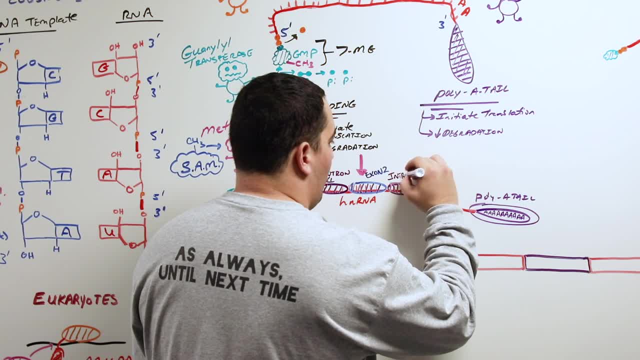 for amino acids. So this is going to be an intron, but we have already intron 1, so we're going to call this Intron 2.. And you guys already kind of get the pattern that I'm going with here. 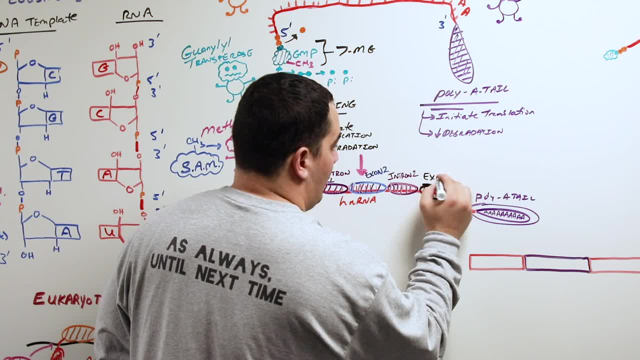 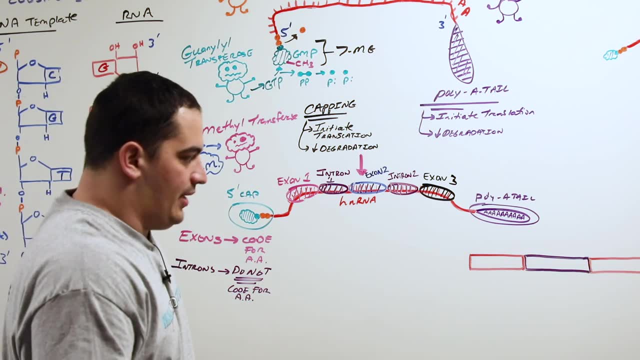 This one does code, so it's going to be an exon, And we already have 1,, 2,, so this will be 3.. Okay, We're going to do something called splicing where- let's think about this- If the introns don't code. 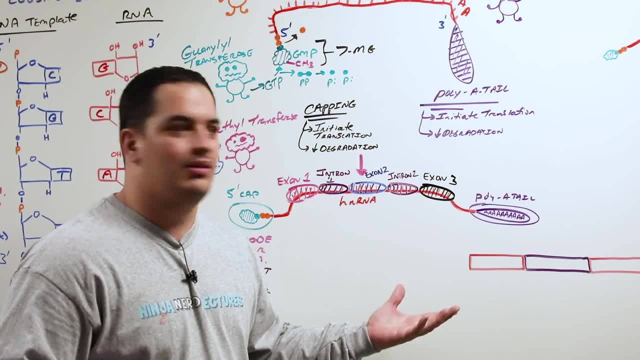 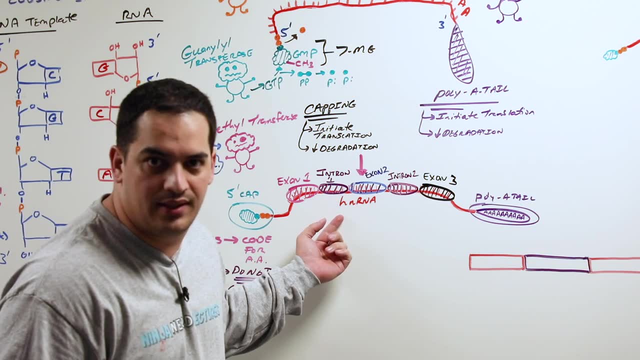 for any amino acids? do we even need them? No, So let's get rid of them. That's all that splicing is. It's getting rid of these introns, or also known as intervening sequences, and then stitching together the exons. 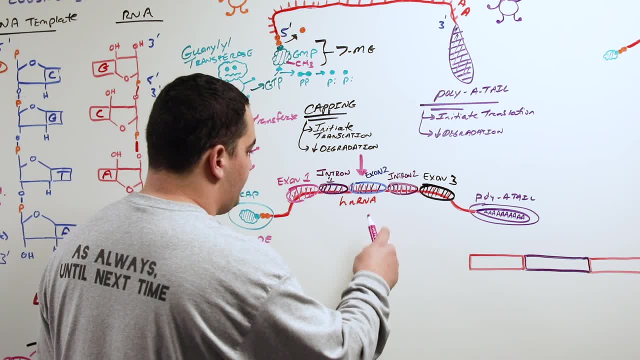 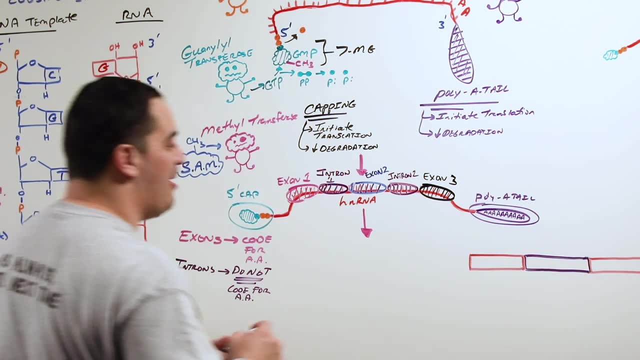 Now, in order for that process to occur, we need very specific molecules, and we talked about it before. Let's see if you guys remember him: RNA, polymerase 2 and 3, they made another very interesting small little RNA. What was that RNA called? 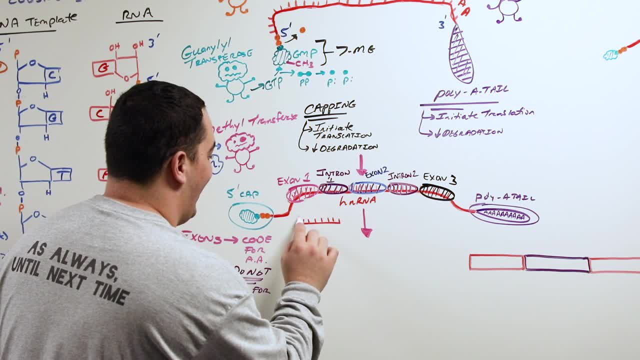 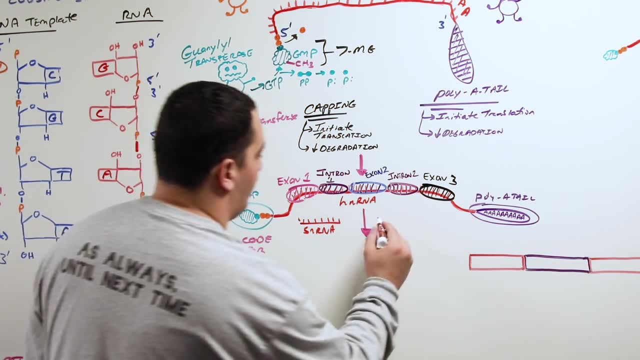 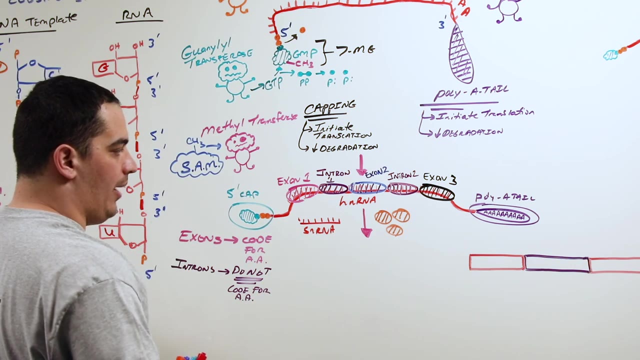 Small nuclear RNA: right, Original, right. So small nuclear RNA is going to combine. we haven't used this color yet, so let's add this: These brown proteins. Okay, So you're going to have some proteins and some small nuclear RNA. 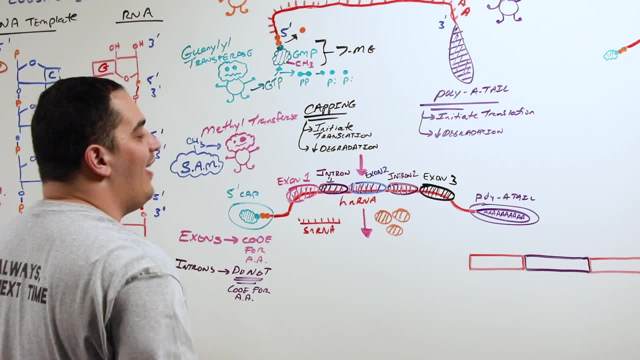 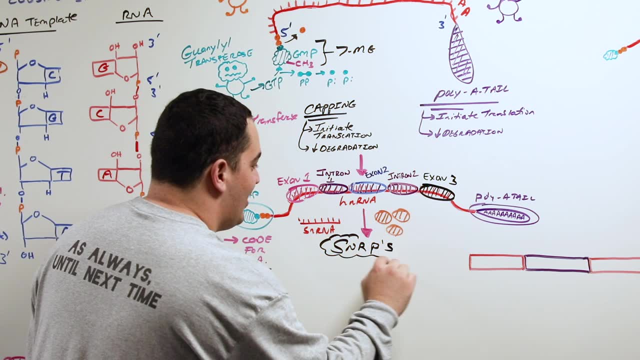 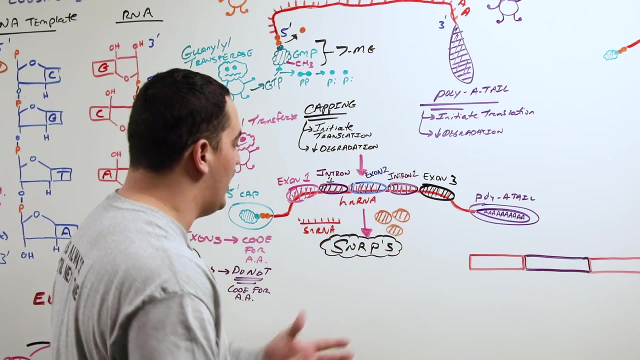 Together, these two things make up a very weird name called a SNRP. Okay, SNRP's Small nuclear ribonuclear proteins, So our small nuclear ribonuclear proteins. And what they do is these SNRP's are going to bind. 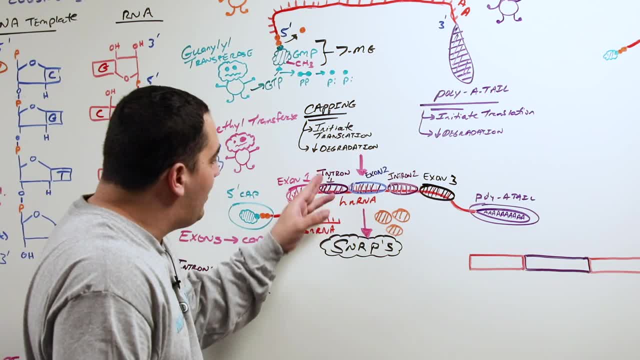 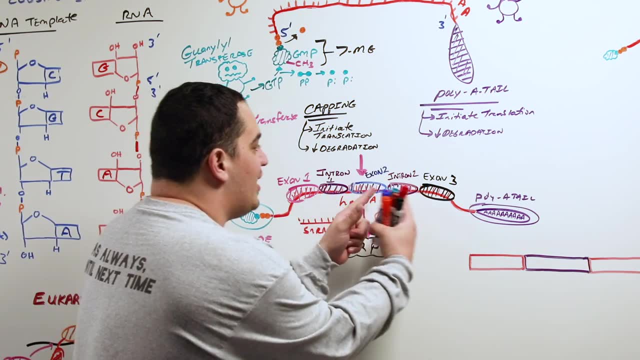 to this ancient RNA And they're going to cleave out the introns in this actual RNA And then they're going to stitch together the exons. So let's show that in a very basic way, of how that happens. So these SNRP's- 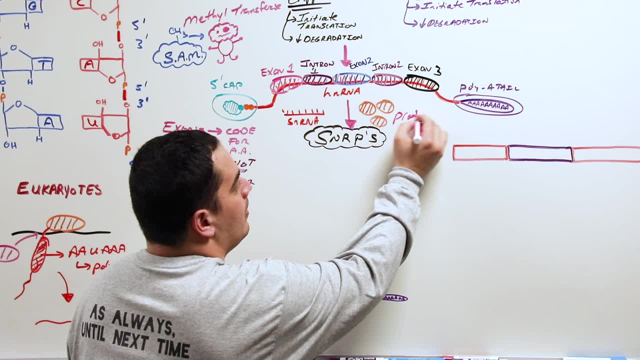 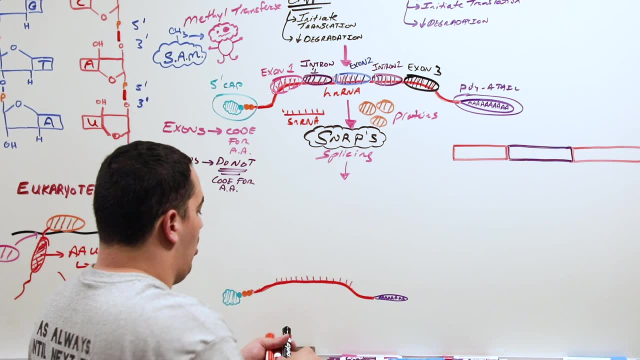 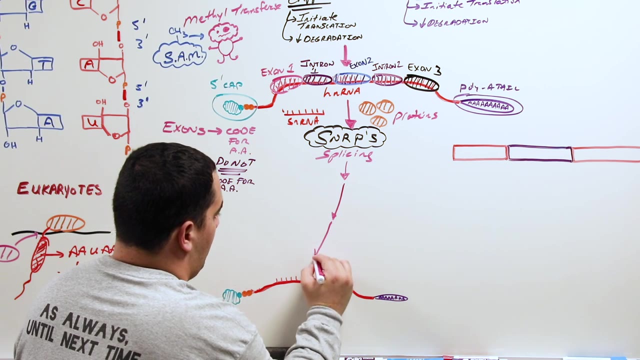 which are the SNRNA and your proteins are going to perform splicing. So what would that look like? Let's take here our transcript here And bring it down here, all the way down to this portion here. So here we're going to make. 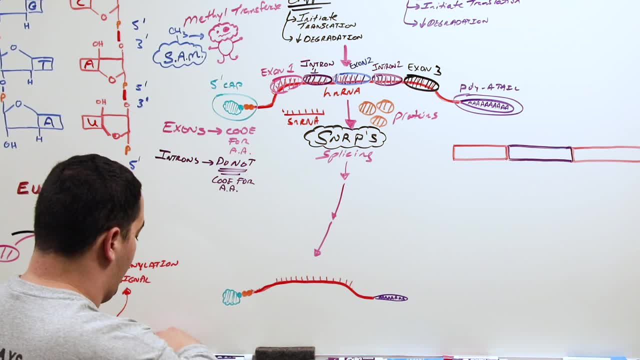 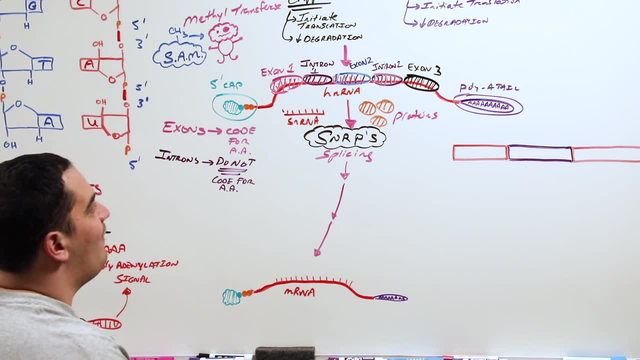 our functional mRNA. So at this point in time we've actually made what. at this point We've made the mature mRNA. And if I were to show, kind of, what was the end result, what am I going to have here? Let's say, here I have a sequence. 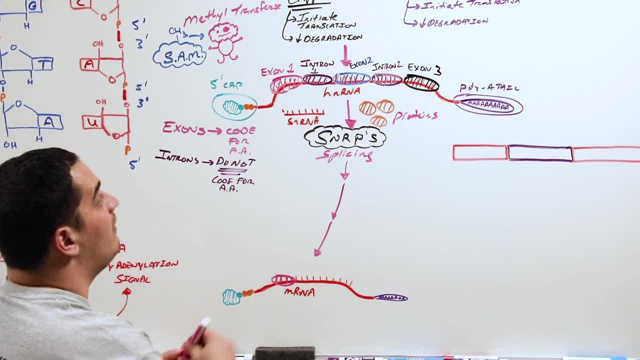 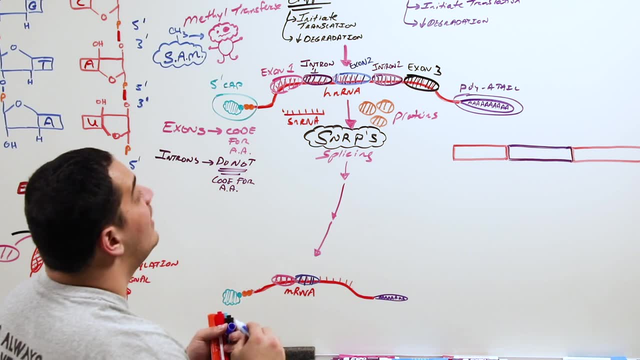 that's in pink, That's exon one. I got rid of entron one, so what should be next? I should have exon two. I got rid of entron two, so what should be left? We're going to expand it a little bit here. 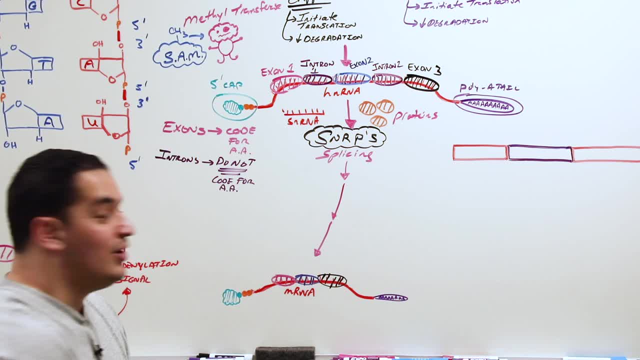 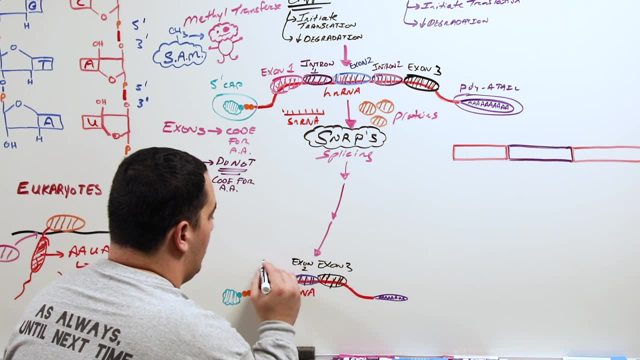 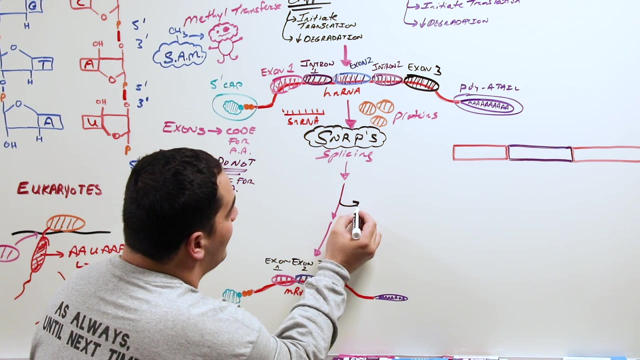 Get rid of that one Exon three. So all I did was I took and got rid of each exon, I mean each entron, and stitched together only the exons. So now let's show kind of coming out of this process here. 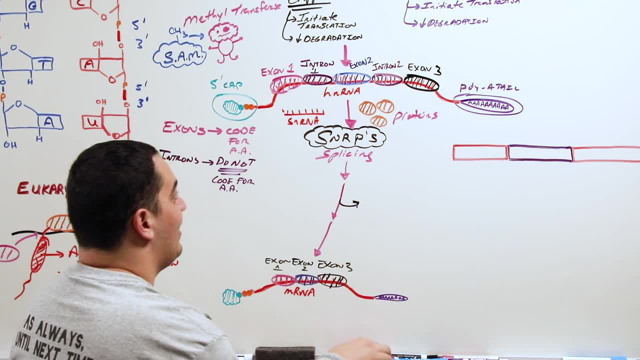 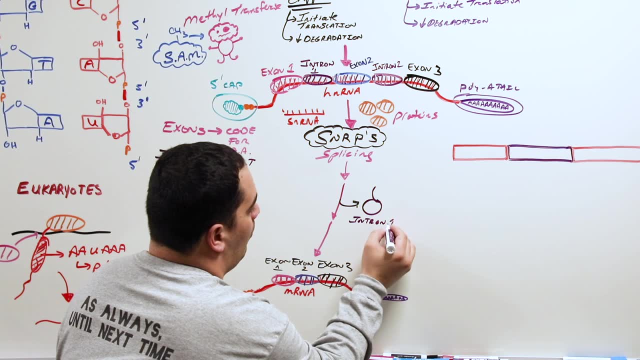 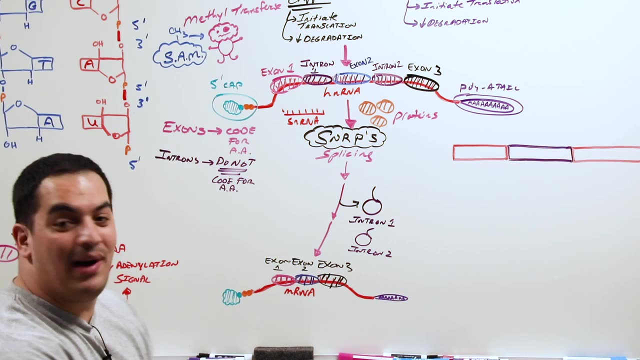 What am I going to have kind of popping out off of this? The introns. And when the introns pop off, this can be entron one, and then you can have another one, let's say entron two. These are going to get popped off. 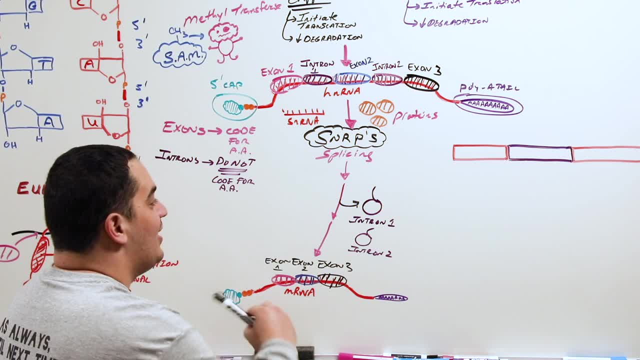 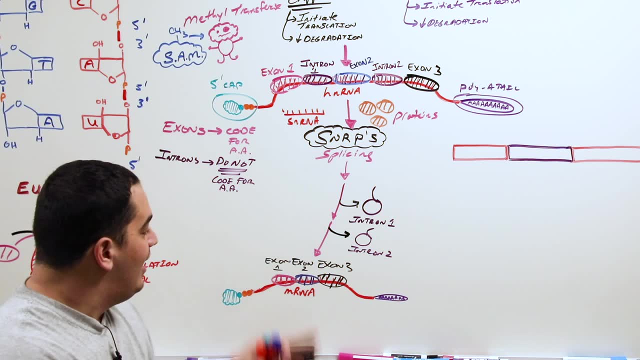 We don't need these dang things anymore. So since we don't need them, we're just going to spit them off during that splicing process and only lead to the formation of exons. Now, within this mRNA, I have my five prime cap. 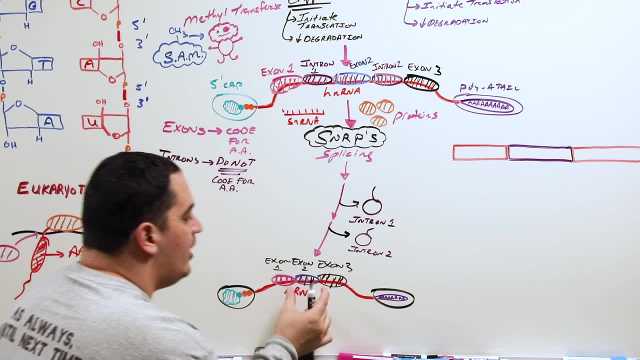 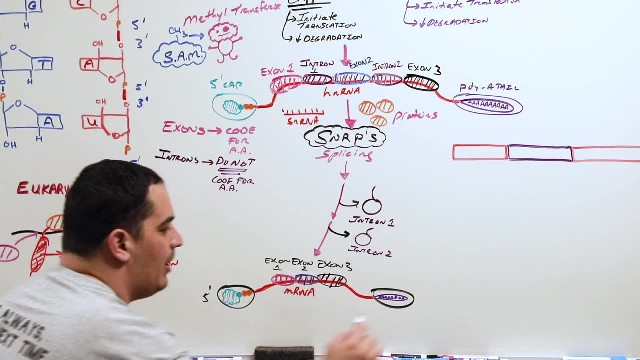 I have my poly-A tail. I have only the nucleotide sequence which is going to code for amino acids. and then, if you really want to go the extra mile, we said this is the five prime end, this is the three prime end. 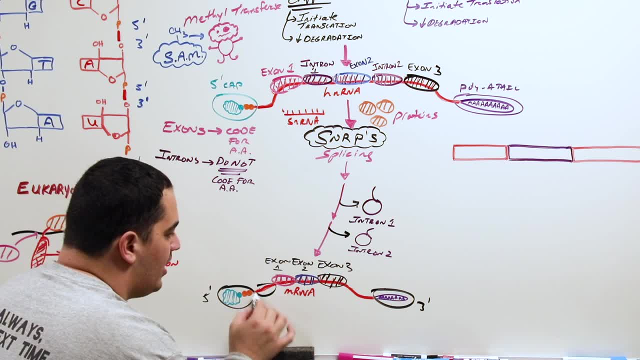 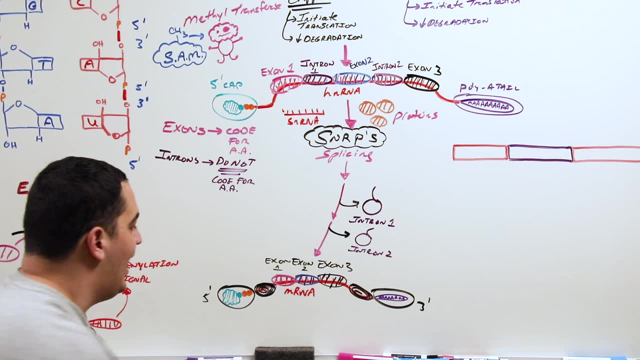 I'm not representing any kind of like dashes here. So this portion here and this portion here doesn't get translated or read at all by the ribosomes, And so we call these regions, since they don't get translated, the five prime, since it's near the five prime. 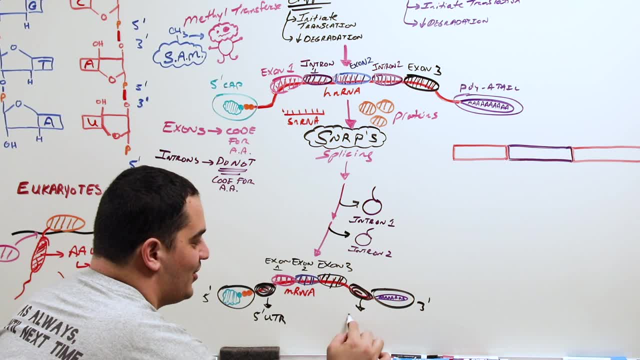 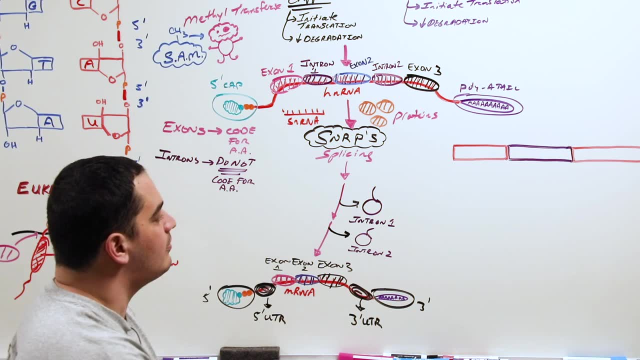 untranslated region, And this one doesn't get translated, So it's called the three prime untranslated region. The only portion that gets translated is the exons. Now, I don't know why, but they love to ask this stuff in your exams. 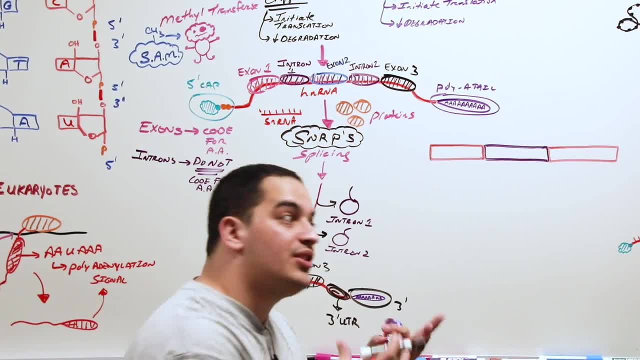 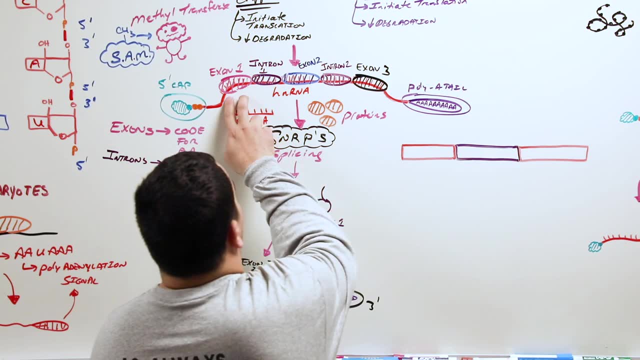 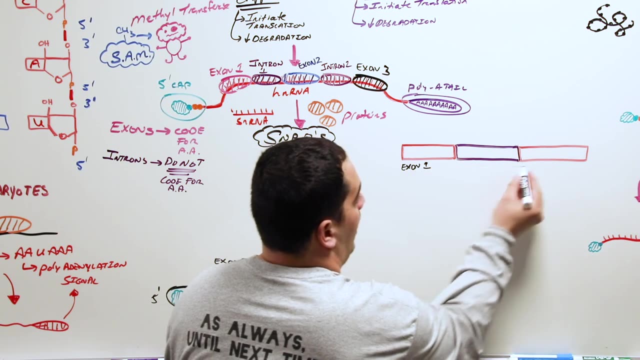 Where you actually go through the specific mechanism of how the SNRPs truly do pull the introns out and splice together the exons. So let's say we take just exon one, let's write this one as exon one and this one is going to be exon two. 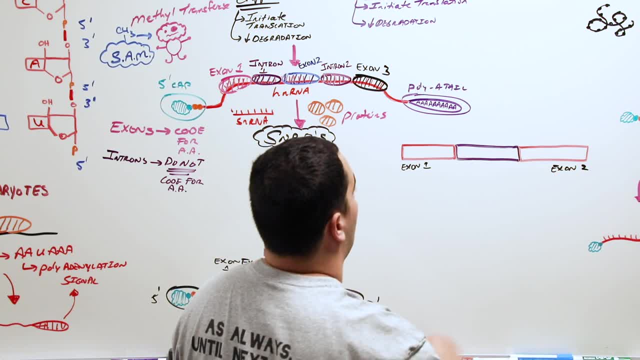 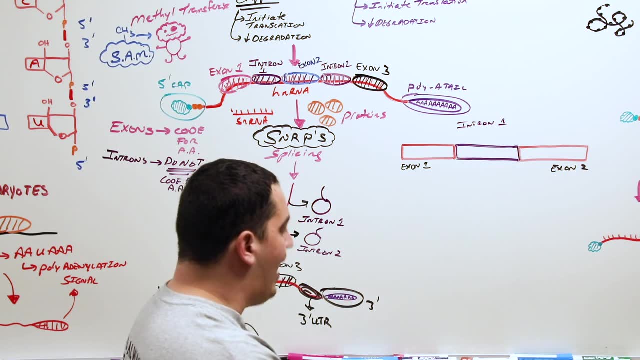 And then here in the middle we're going to make this intron one. So let's kind of show you how these SNRPs- again the SNRPs, which is the SNRNA and the proteins- do this. So if you really wanted to show it, 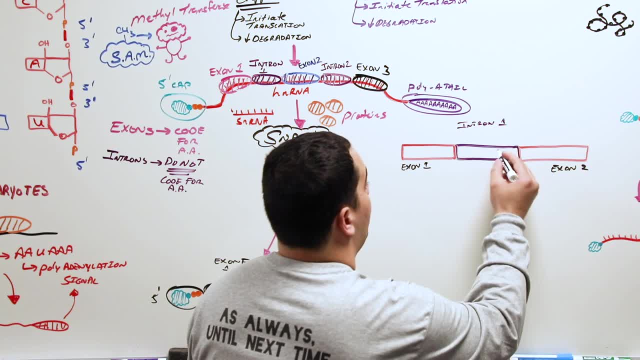 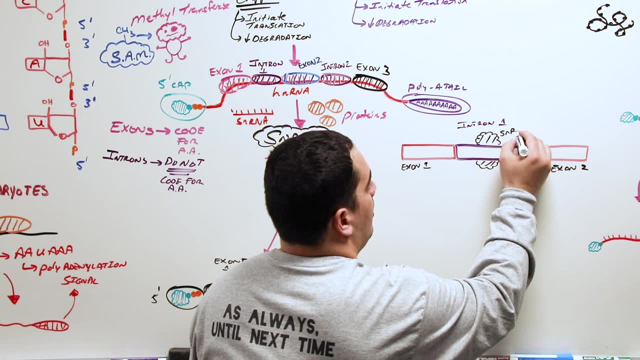 let's just represent the SNRPs as kind of a black blob, if you will. They're going to kind of bind near this portion here. So here's my SNRP Within this portion, here, right at the intron at this portion. 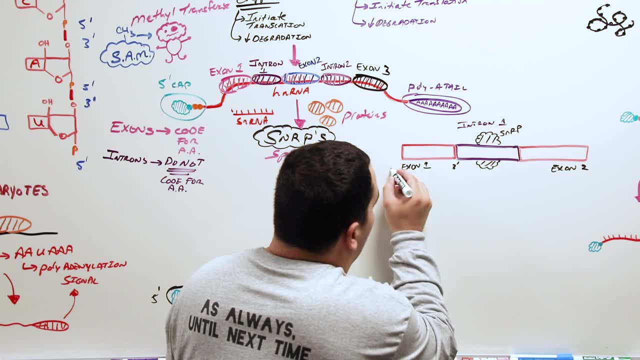 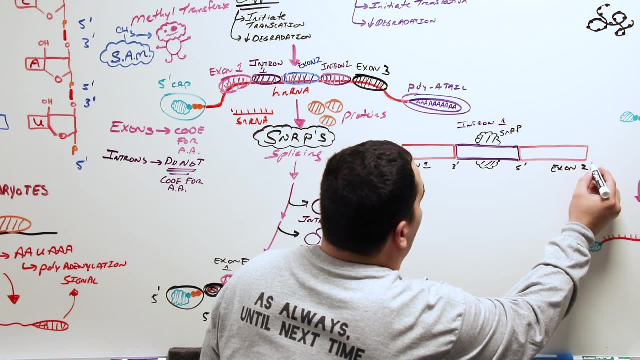 let's say here is the three prime end of this exon, five prime end of this exon. And let's say that here is going to be the five prime end of exon two and then the three prime end of exon two. Okay, And then here's going to be. 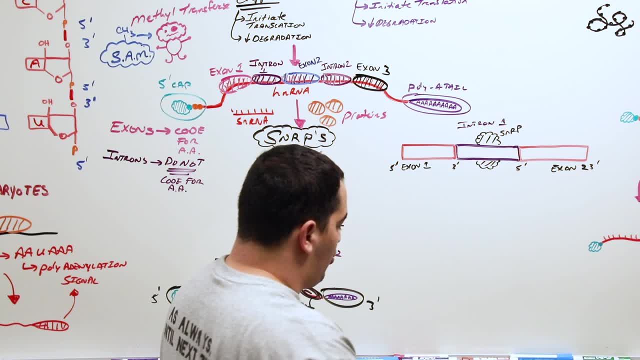 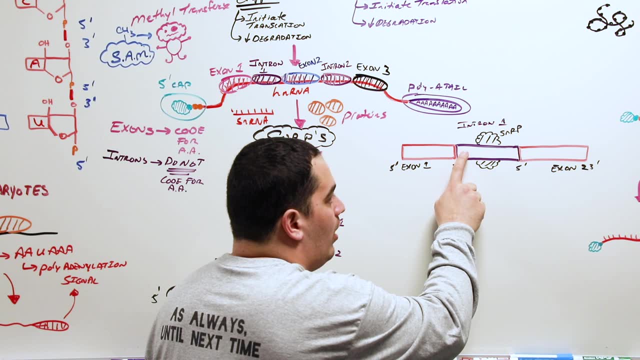 the intron. inside. Within this intron you have a very specific nucleotide sequence that's near the three prime splice site, near exon one and the beginning of intron one, And then you have a very specific nucleotide sequence near the five prime splice site. 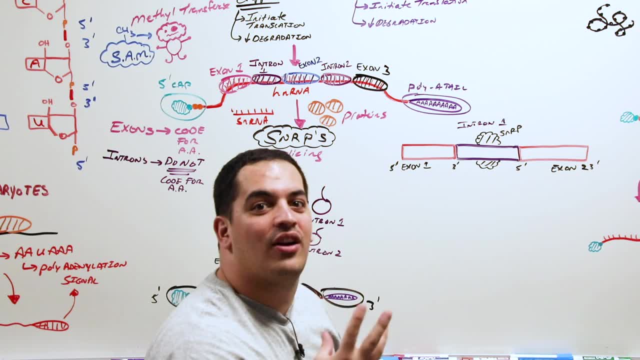 at exon two and at the end of intron one. What are that nucleotide sequence? It's dumb but it helps me to remember it. So I say I'm a G. How about you? I'm a G, So you remember G U. 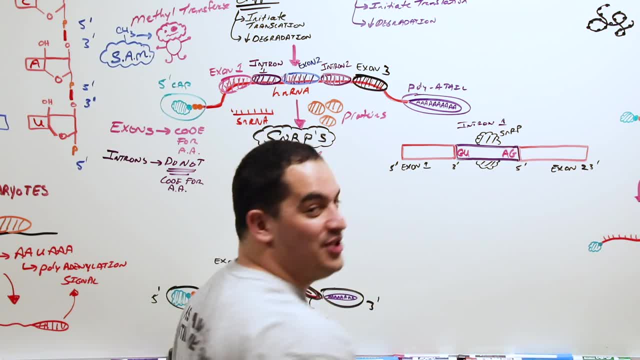 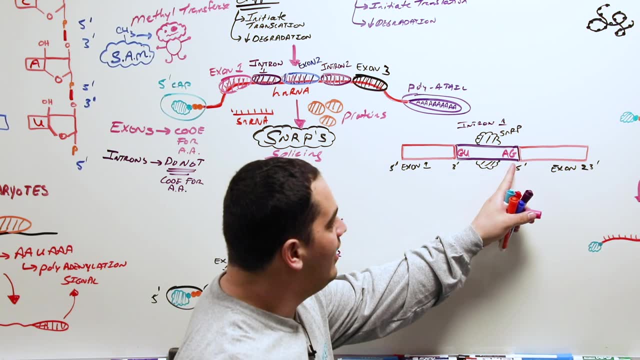 I'm a G, How about you? I'm a G. That's the basic way that I remember the nucleotide sequence at the three prime splice site and then the one at the five prime splice site between exon one, exon two and intron one in this example. 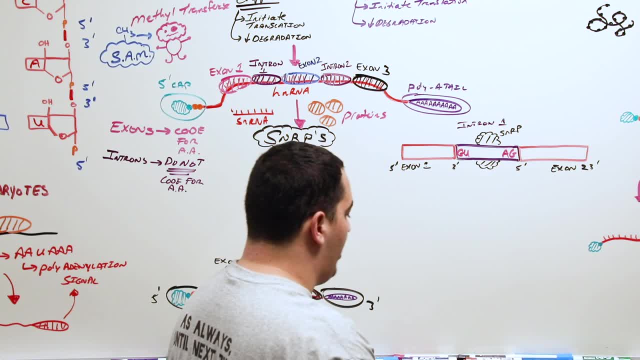 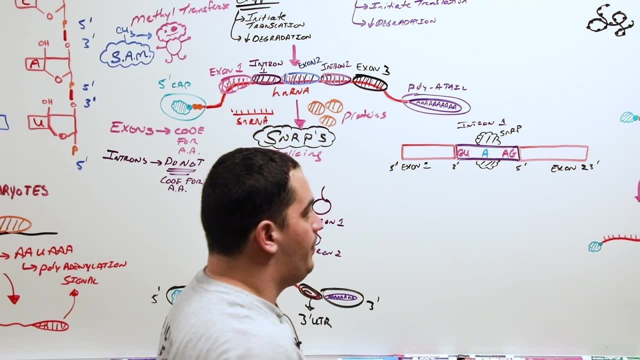 At the. there's another one right, smack dab in the middle. Let's make him a different color so we don't confuse it. Smack dab in the middle, there's a branch point which is an adenine. Okay, There's an adenine. 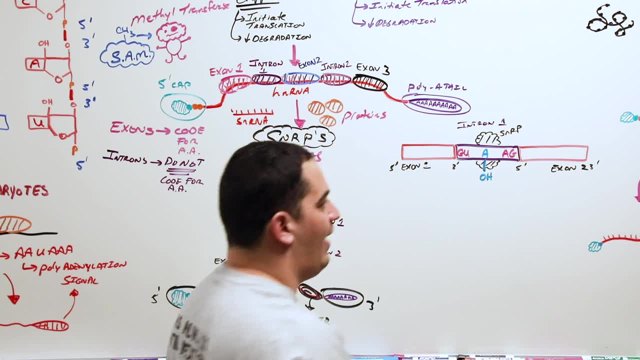 right at this branch point It has a very specific OH group kind of hanging from it. Okay, So this is called your branch point. What happens is is the snurps will come in and they're gonna cleave at that three prime splice site. 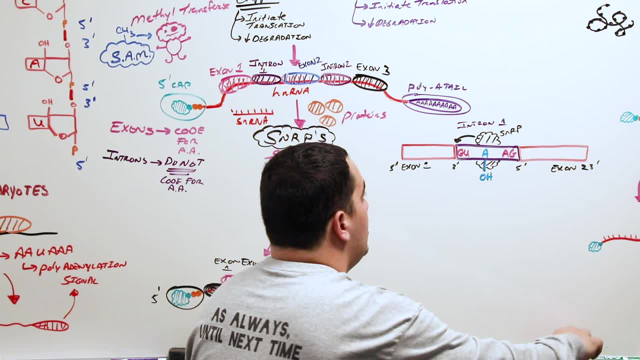 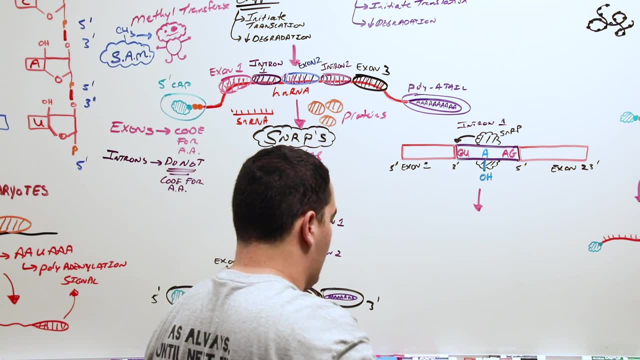 Okay, They're gonna cleave this portion off. So what would that look like afterwards? So the snurps come in and they cleave at that three prime splice site, And so what's gonna be left over here is we're going to have 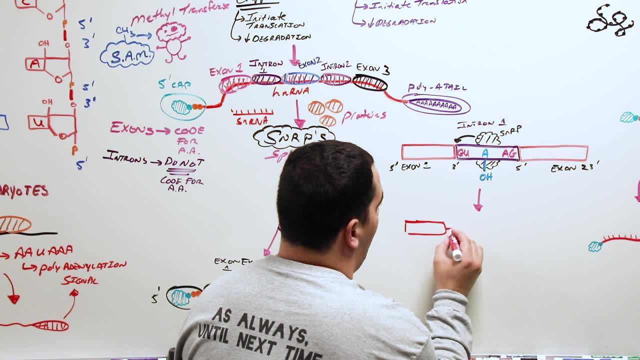 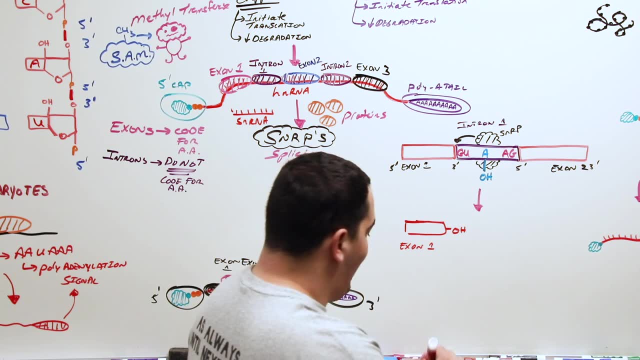 exon one, somewhat separated here And coming off here. what's? the three prime end contain An OH group right And again, this is exon one. Then the next thing you have here is intron one And it's gonna have that kind of portion here. 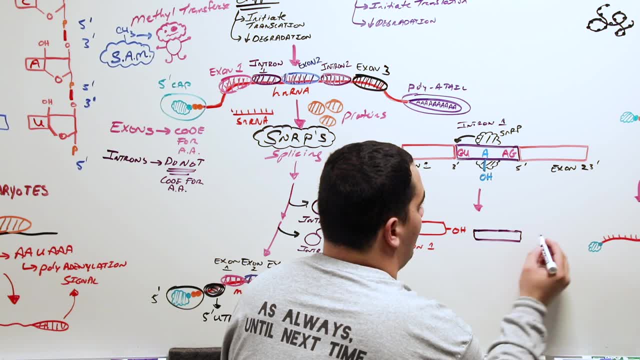 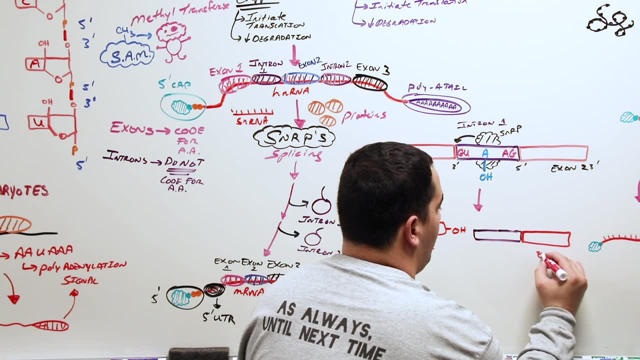 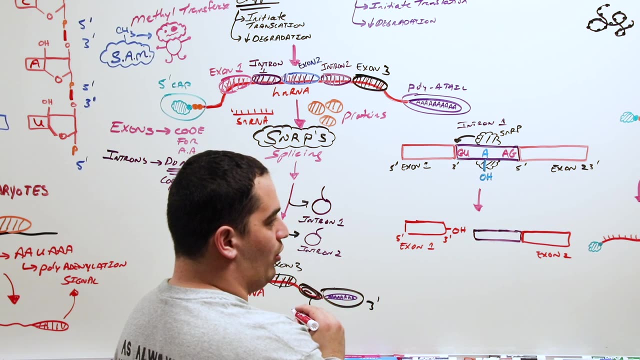 kind of split off, if you will right, Kind of broken off here And then again over here. we're gonna have still fused at this end exon two. So again, this is my three prime end, which has that. OH, This is the five prime end of that portion. 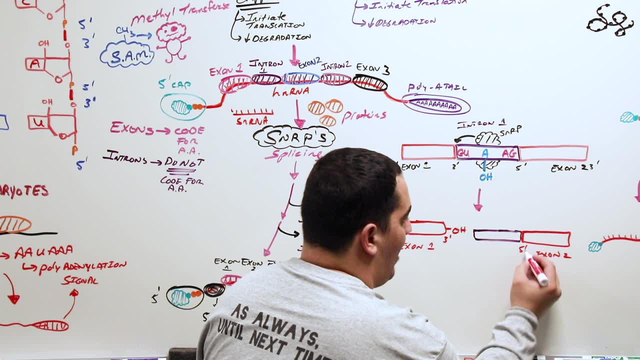 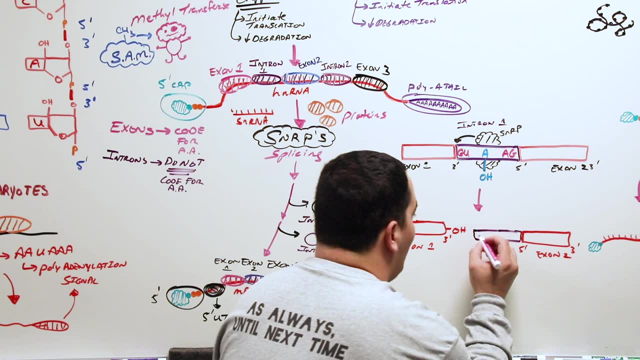 of the exon, And then again same thing over here. This is the five prime end of exon two. Three prime end of exon two. And then again, what kind of nucleotides do we have in here? We have that GU, which was pretty much the marker. 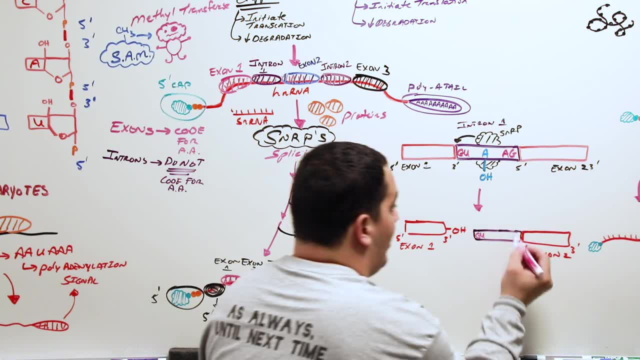 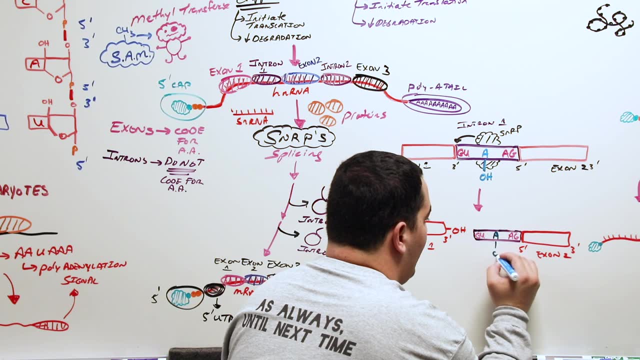 which the snurp would cut at that three prime site, Then on this five prime splice site I still have that AG. And then here in the middle I have that branch point with the adenine, with the OH group. Here's the next thing that happens. 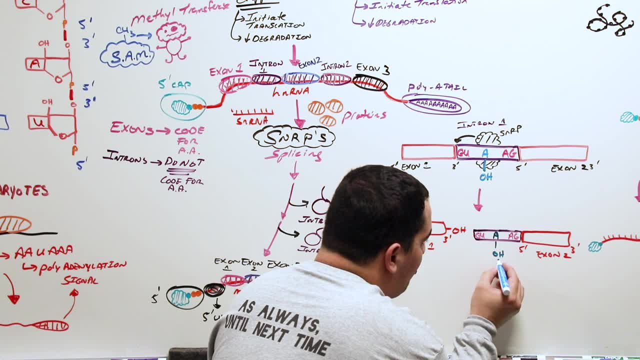 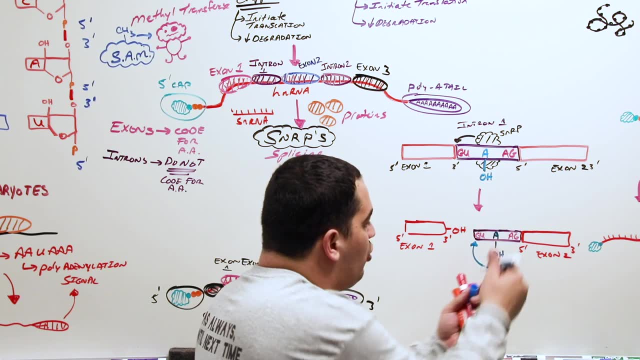 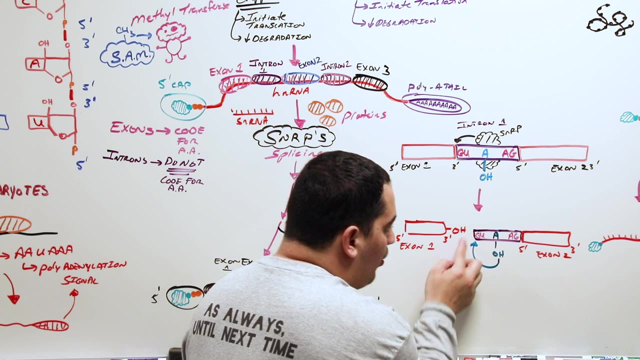 The OH group of that branch point will then bind or attack that GU site And pull it in to where it kind of fuses at this point. So it makes kind of like a little loop, if you will. So let's show that It attacks the GU. 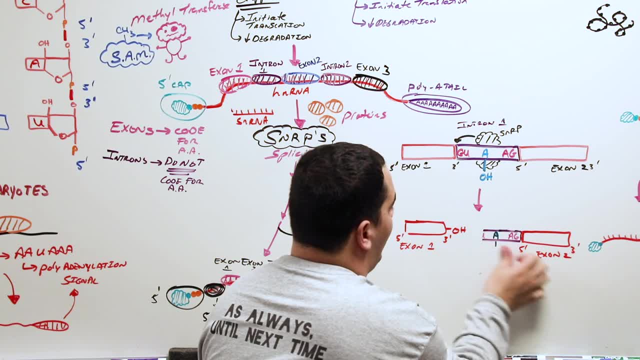 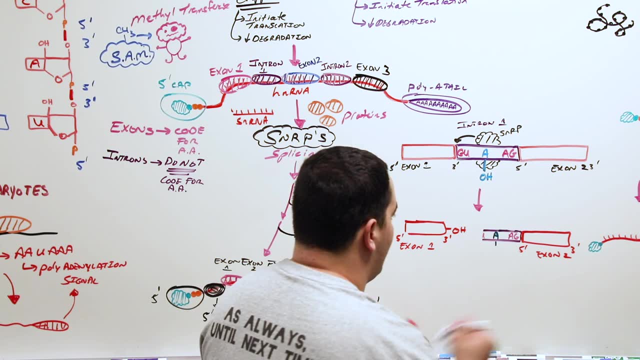 and pulls it in After that happens. you kind of form this weird little like loopy structure, if you will. So what would that look like if we kind of drew after we had that attack, After that attack point. it's going to kind of look somewhat. 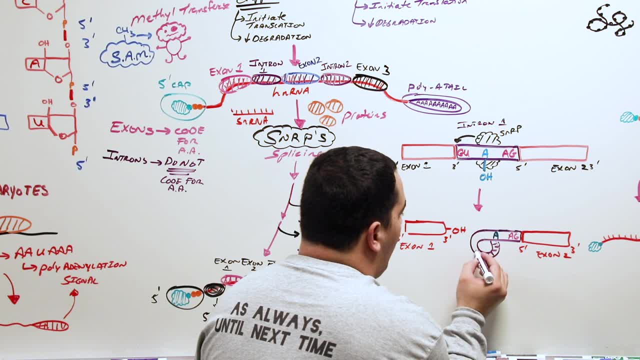 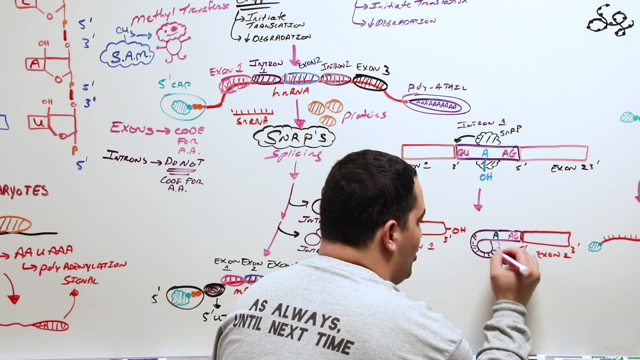 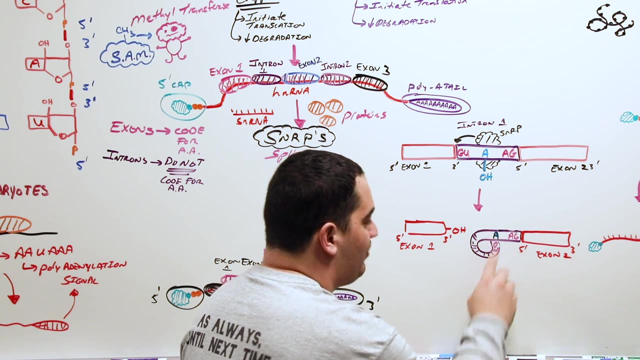 like this, if you will, Where we have now that portion, where what would be here, What would be the kind of the nucleotide sequence at that point, right there, GU was attacked at that point by the OH, at that branch point. Then the next thing happens: 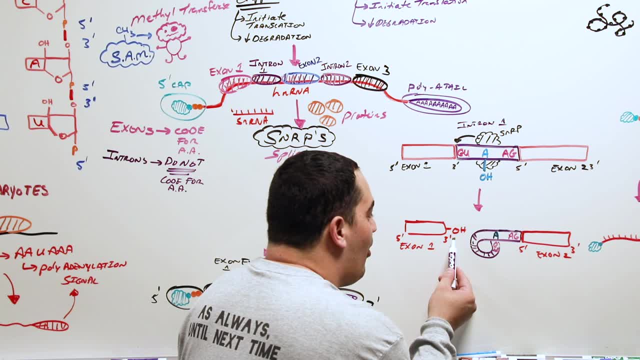 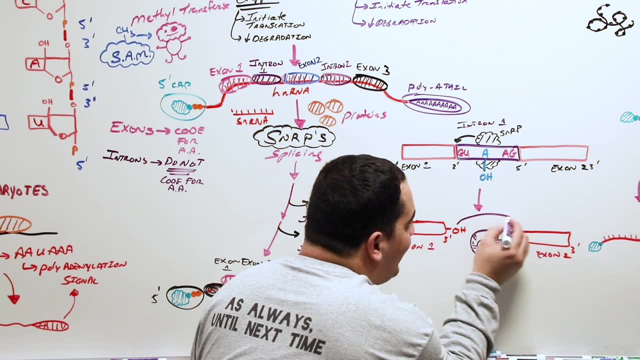 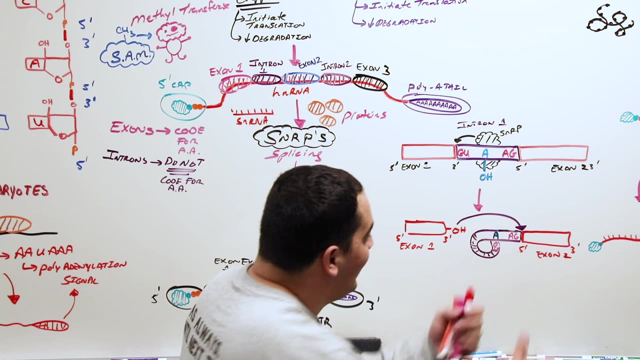 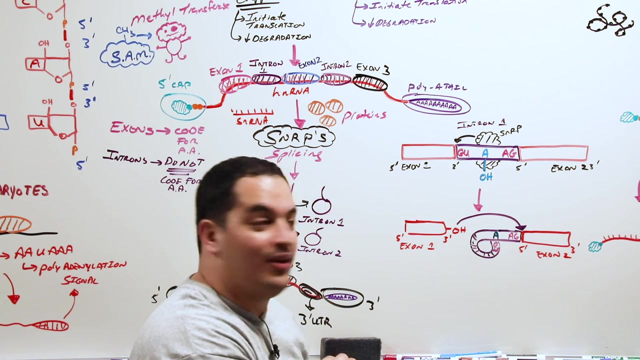 This is crazy. This three prime OH of exon one will then see that five prime splice site and it will attack the five prime splice site at exon two. When it attacks it it then breaks away the nucleotide sequence AG of this intron away from exon two. 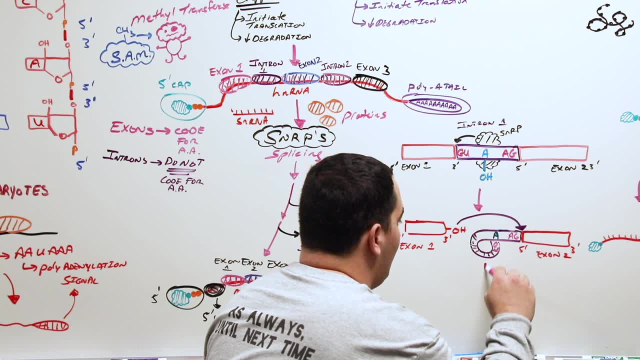 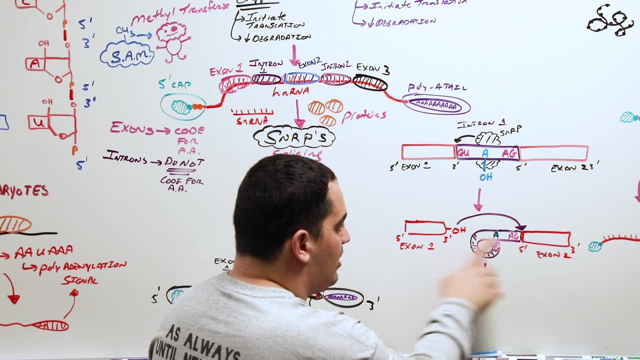 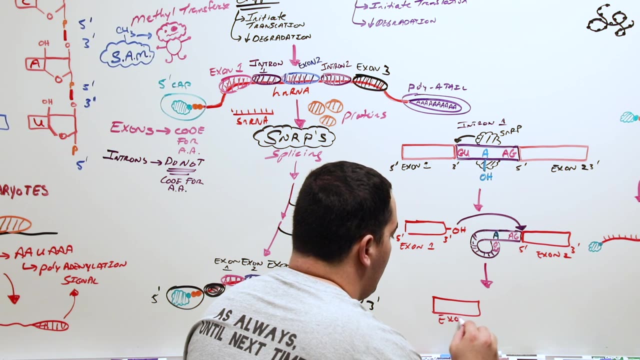 So okay, now let's show what that would look like. So if the three prime OH attacks the five prime N, three prime OH of exon one attacks the five prime N of exon two, now what do we have here? Exon one fused with exon two. 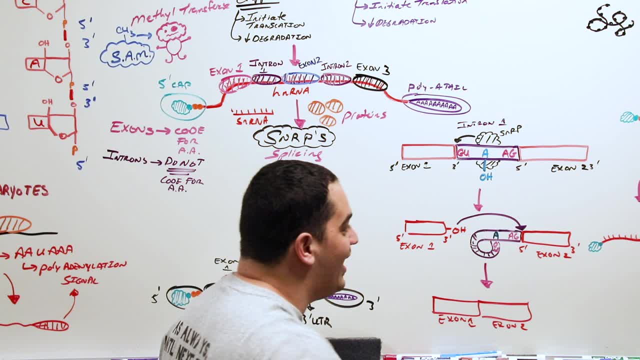 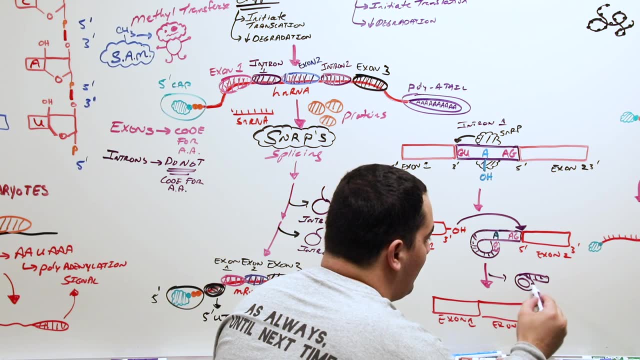 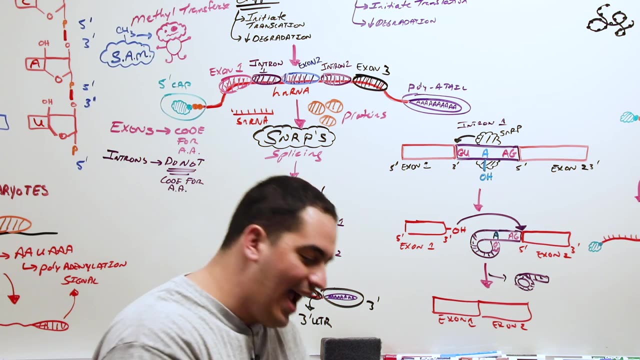 And we just fused the exons. and then what do we spit out after we break this off? The intron lariat, which I showed you like that before. That is how this whole splicing process technically occurs: Super quick Again, Snurps bind. 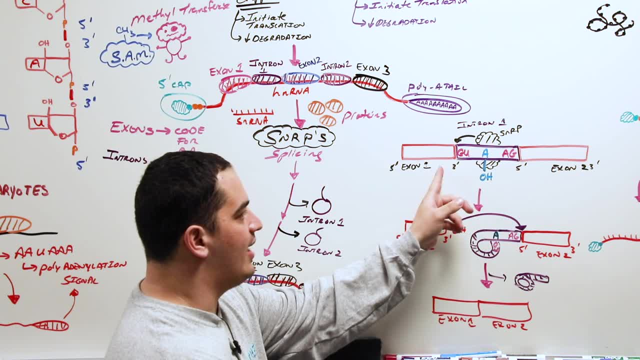 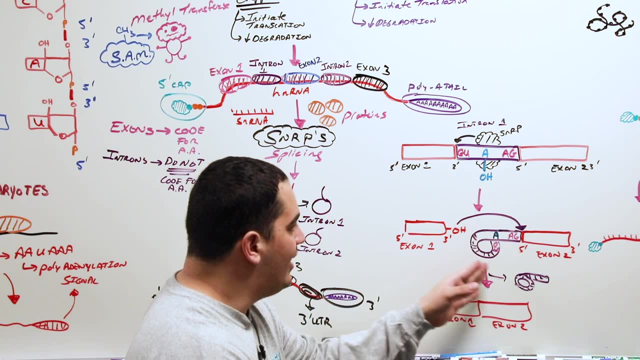 What do they do? Cut the three prime splice site between exon one and intron one. When it does that, the OH of the adenine at the branch point attacks the GU site, Pulls it in, Creates this loop: The three prime OH of exon one. 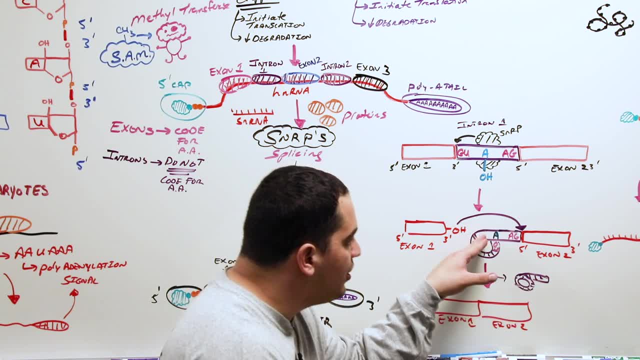 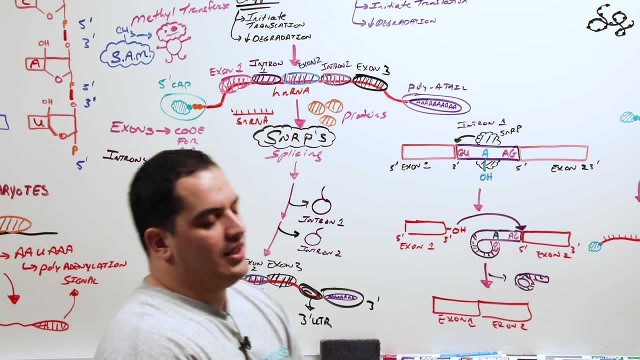 attacks the five prime N of exon two, which snaps the intron out and stitches together exon one and exon two. That is splicing. You're like Zach. why the heck do I need to know all this crap? There's a reason why: Whenever there's abnormalities, 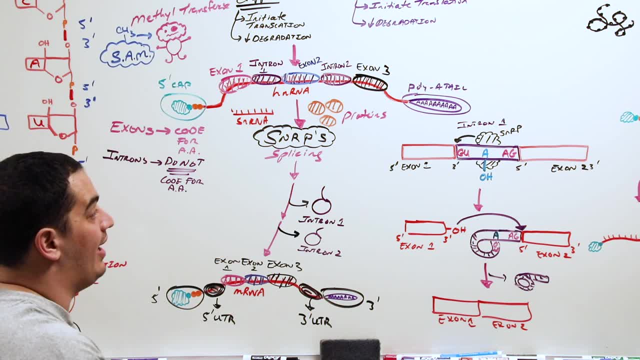 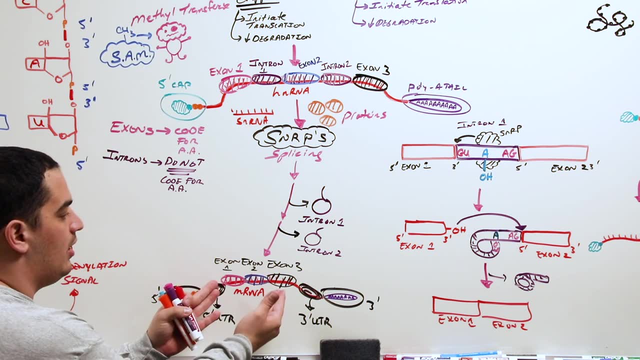 within splicing it can produce a various amounts of diseases because, think about it, If I don't cut out the introns properly and I have introns mixed in with the exons and introns don't code for amino acids, am I going to make a proper protein? 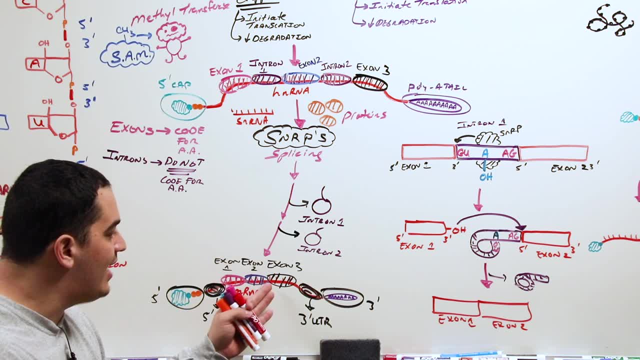 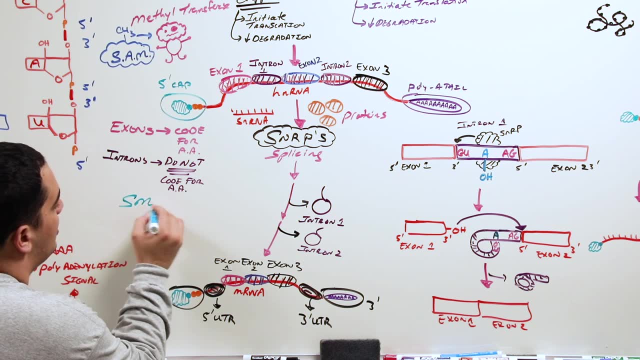 No, because I'm going to have areas that will code for amino acids and areas that don't code for amino acids. You know there's a very devastating condition called spinal muscular atrophy, where they are deficient in an SMN protein. You want to know why? 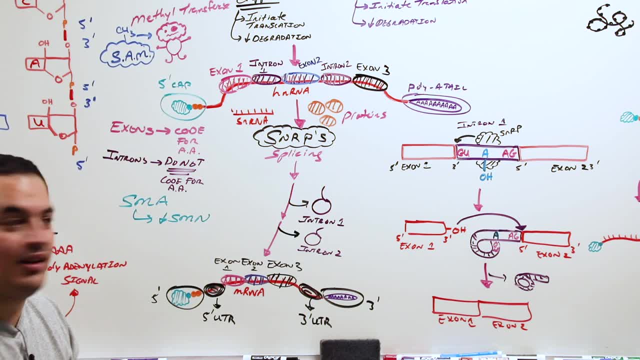 Because the snrps aren't working properly. So there's a deficiency or there's a problem with the snrps not performing the proper splicing. You know what else? There's another disease called beta thalassemia. Beta thalassemia- guess what? 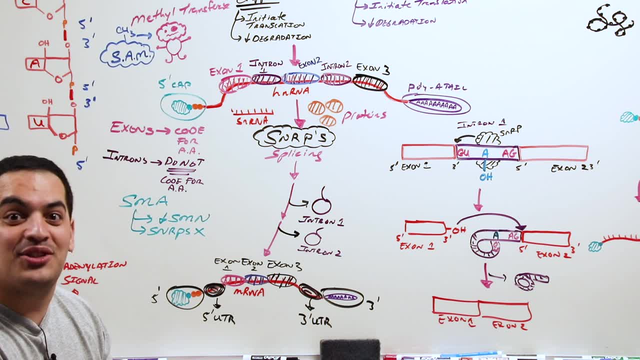 You don't remove a particular intron and because you don't remove that intron, you make a protein that's abnormal and it produces beta thalassemia. So there's reasons to know this stuff. and again, if someone has spinal muscular atrophy, 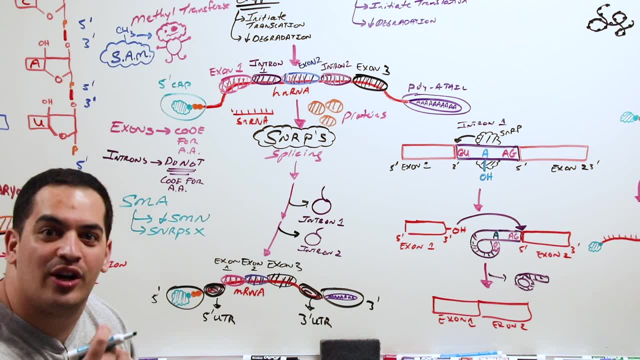 do you know what that affects The anterior gray horn neurons and then they develop lower motor neuron lesions, hypotonia, hyporeflexia, floppy baby syndrome. So it's a dangerous condition that can be traced back to something at the molecular level. Alright, now that we talked about this. 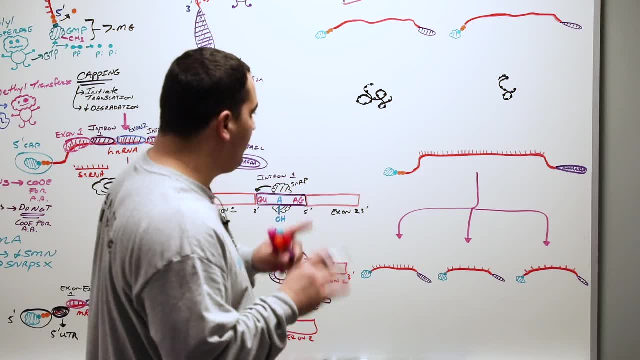 there's two more things and I promise we're done. So I want to talk about two more things, and then we're done. The first thing I want to talk about, because it's very pretty much similar to what we talked about over here with splicing: 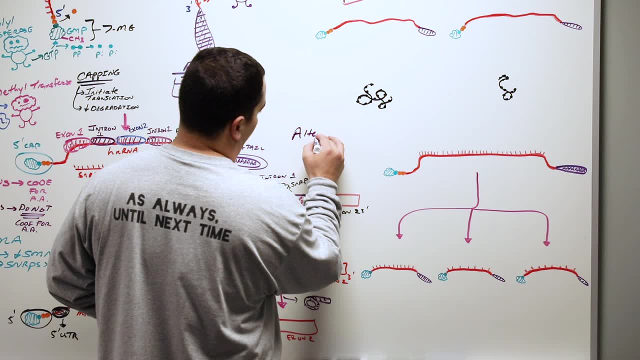 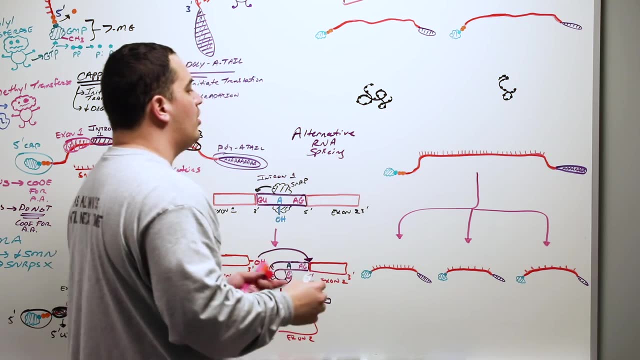 I want to talk about something called alternative RNA splicing. We understand the specific reason for splicing: It's making sure that we only utilize exons to code for proteins and there's no introns, because if we have introns in there, it's going to frack up. 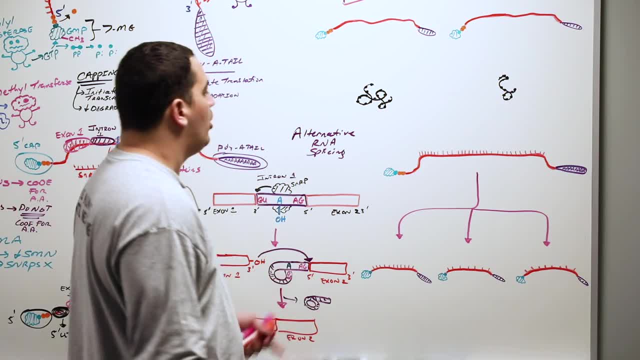 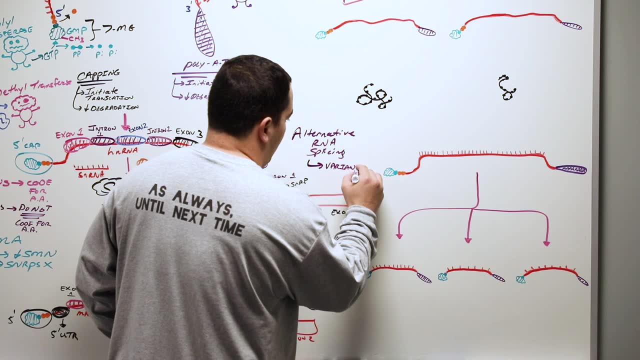 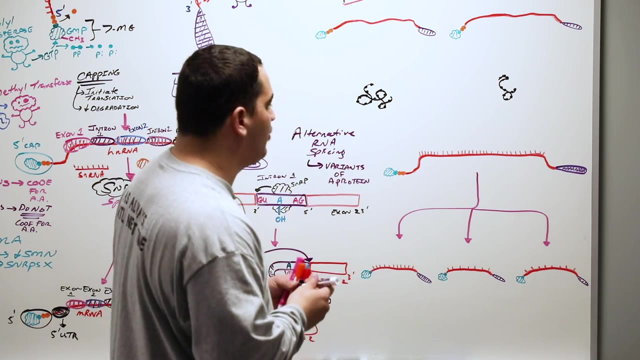 the whole protein production process We'll get an abnormal protein With alternative RNA splicing. it gives variance of a protein And I'll give you guys an example in just a second. but let me kind of talk about how this works. It's literally the same thing. 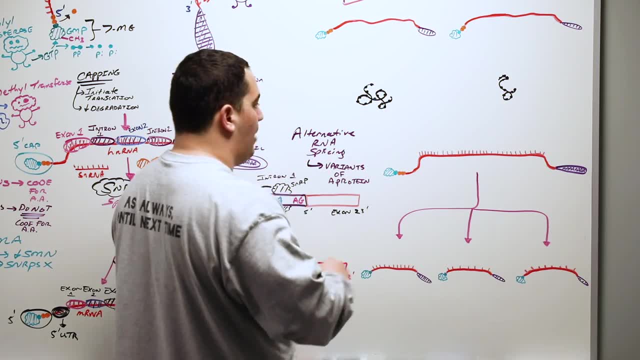 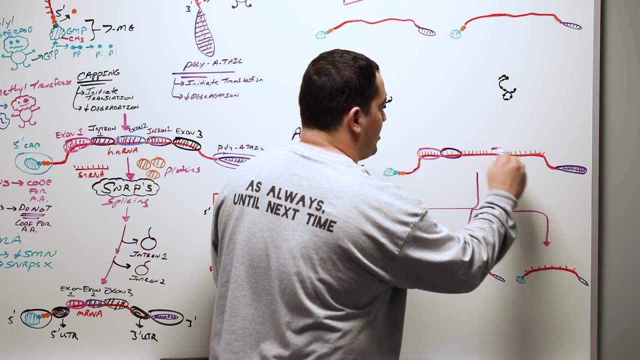 We're not going to go too ham on this, Let's use the same colors here. Here was exon one, and then here we had intron one- and we'll just skip this part here where that was intron two, and then blue. here we had 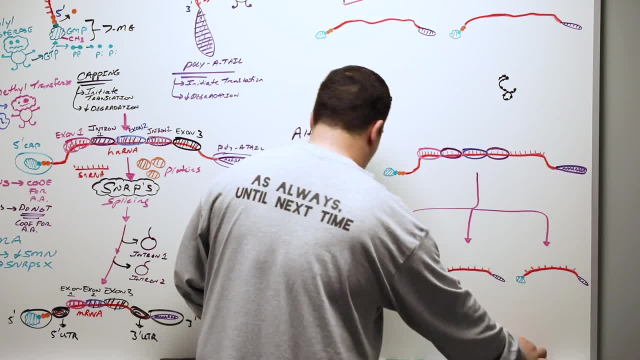 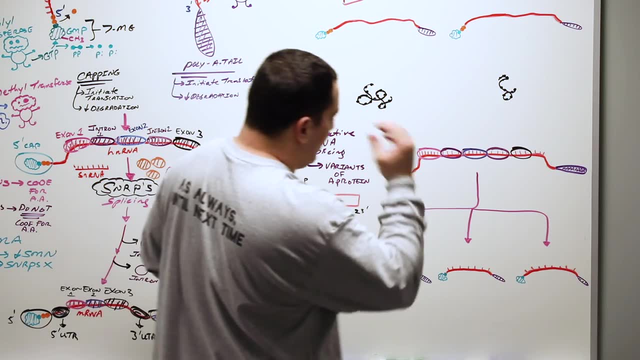 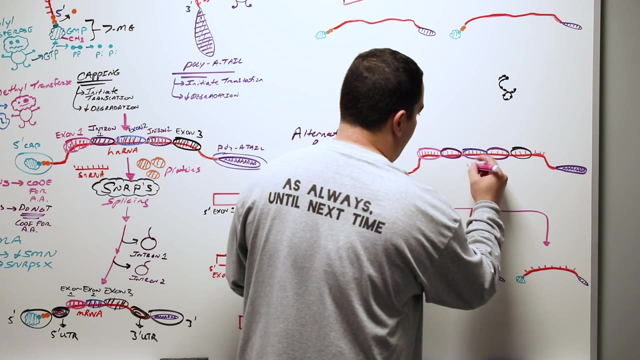 exon two and then at the end here we had in black exon three. So let's say that we take an example here of this kind of H in RNA. So here's our H in RNA and we want to make different mRNAs That'll give variance of proteins. 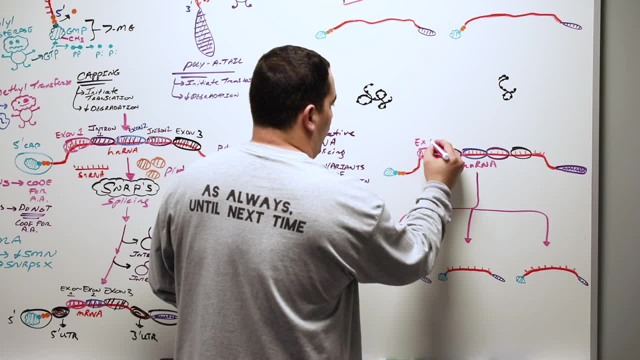 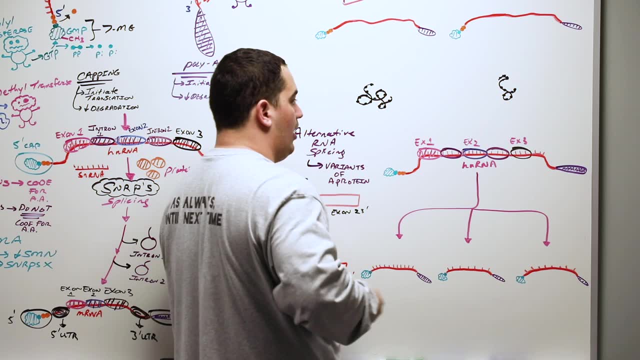 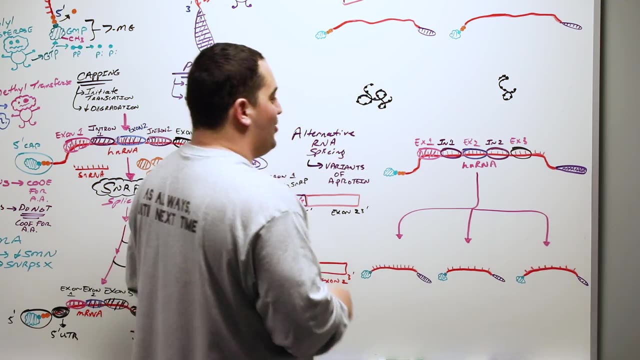 So let's say here that we have, I'm just going to put exon one and I'm going to do all the same color here: exon two, exon three, and then here in between we're going to have intron one and intron two. Here's what I can do. 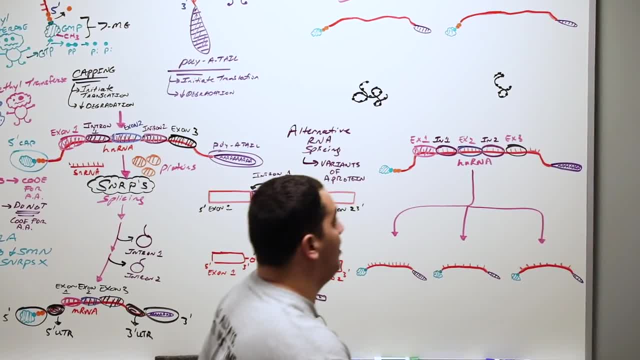 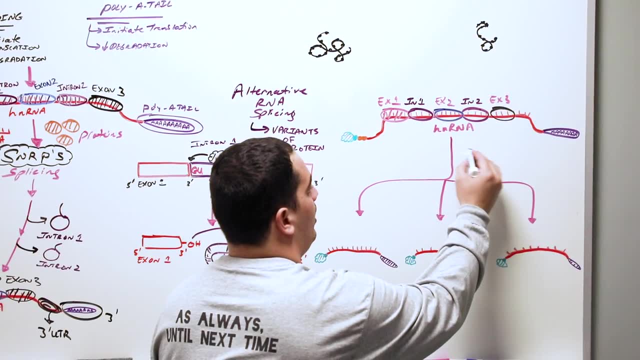 which is really interesting and it's very cool when it comes to plasma cells and antibodies. So let's say I use those SNRPs. So let's say, here I put my SNRPs, my SNRPs, which are my small nuclear ribonuclear proteins. 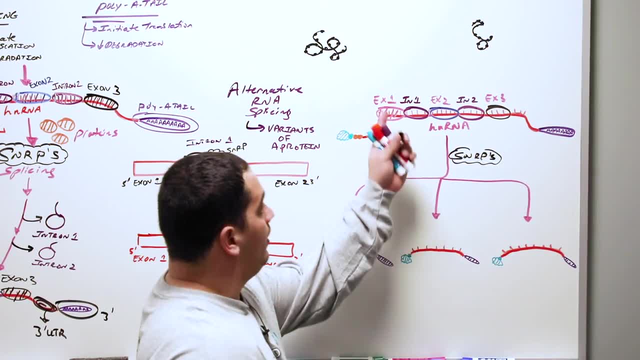 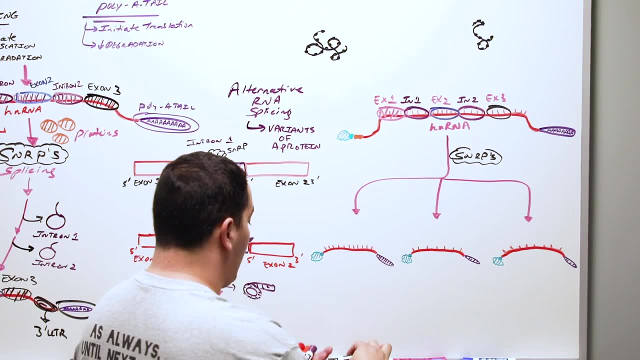 with the SNRNA and the proteins. They're going to splice, but they're going to do it in a very interesting way. So let's say that the first one over here we get the same thing that we did with that whole process of splicing. 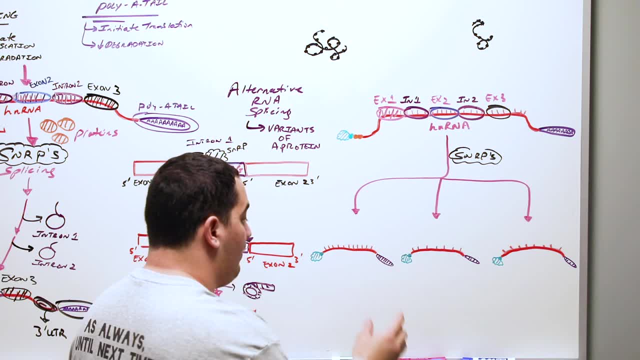 where we got rid of all the introns and we only have in exons. And let's say that we have exon one, let's say that we have exon two and then we have exon three. So we have all those exons here: exon one, exon two and exon three. 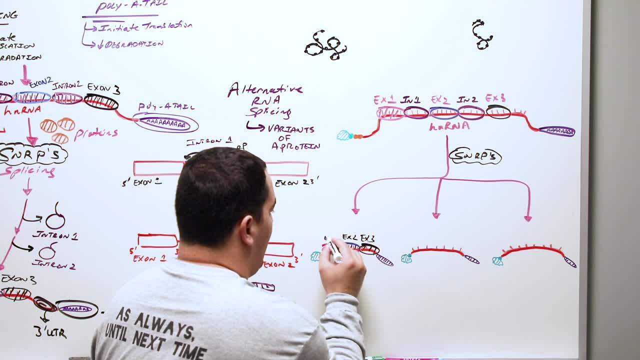 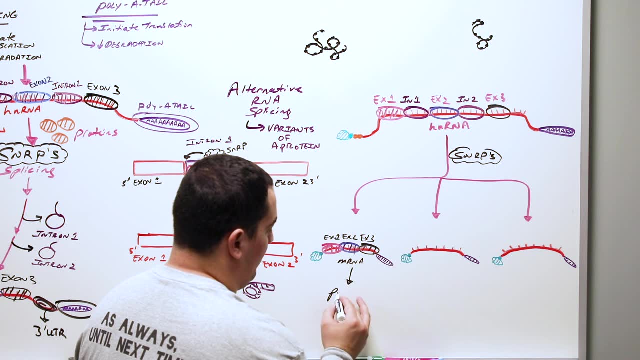 So we'll put these exon three, exon two, exon one, So that's one. this is going to be mRNA, after we've kind of done that process, and it'll give way to a particular protein And we'll call this protein A, if you will. 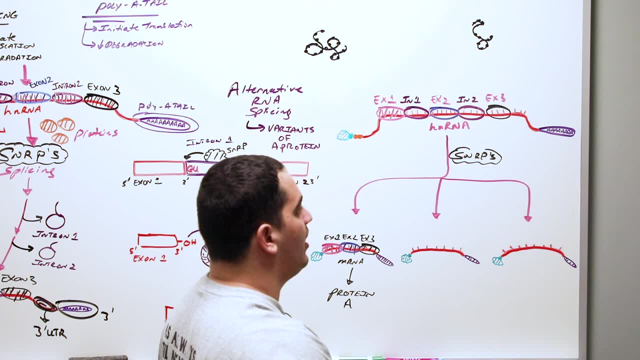 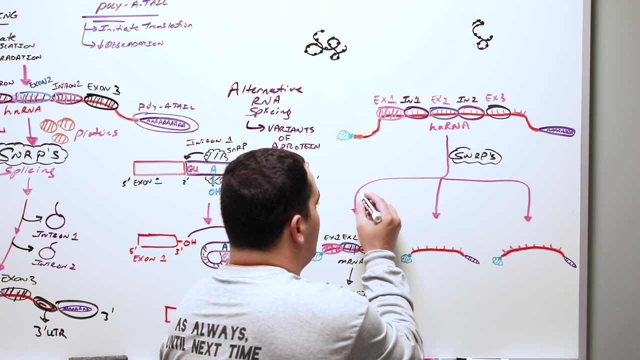 Then we're going to go through the same thing. The SNRPs are going to cleave out the introns and only leave in the exons. But let's say, for this example we pop out, so this one we popped out introns. but let's say, with this one we pop out both the introns. 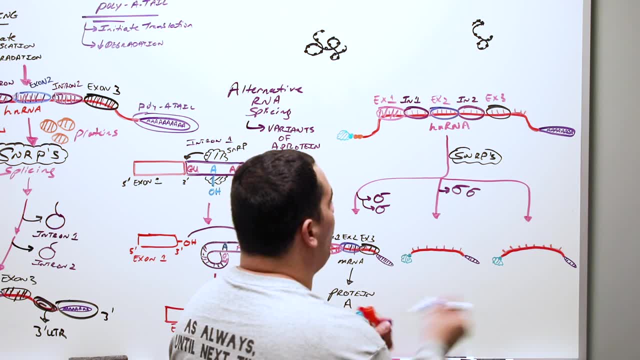 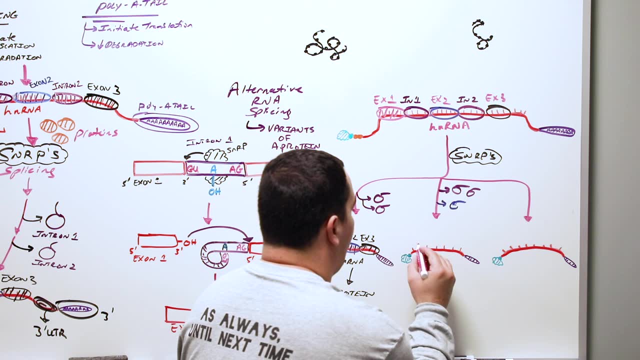 and let's say that we pop out exon two, Let's say that we don't want exon two in this one. So then, what am I going to be left with? I'm going to be left with only exon one and exon three. And by doing that, 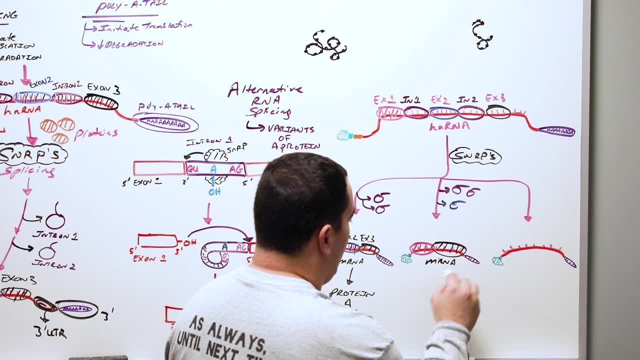 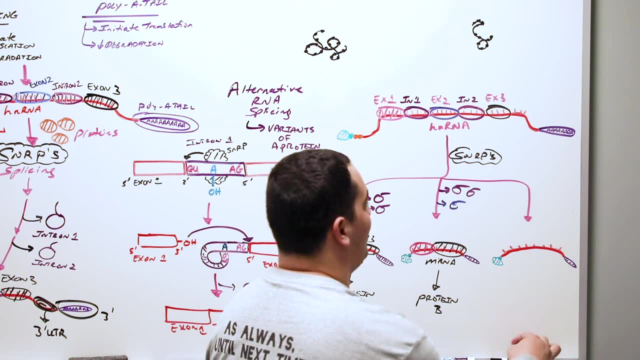 that's going to give me an mRNA that'll code for another protein. Let's call this protein B. And then, last but not least- you guys can already probably see where I'm going with this- Let's say that this last one example three: again, we cut out the introns. 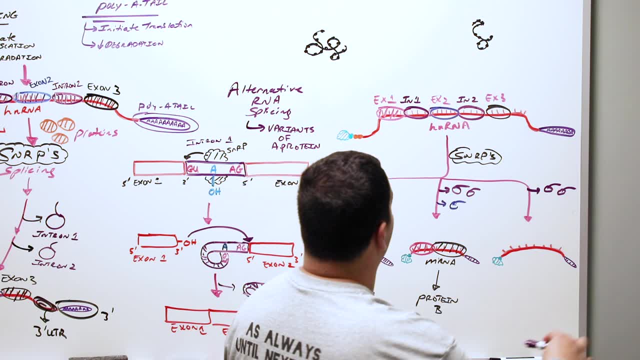 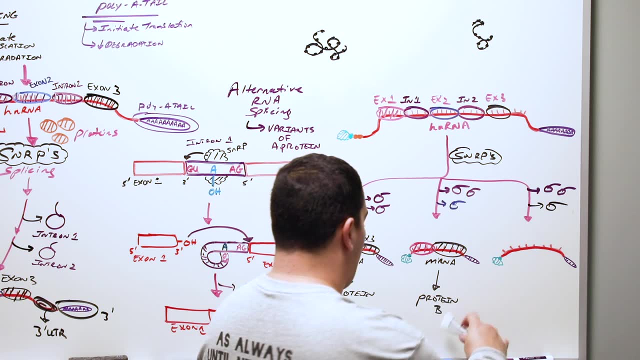 we always got to cut out those introns, But in this case we cut out exon three. I don't want that one in the diagram, I don't want this one in that mRNA. So what am I left with? I'll be left with. 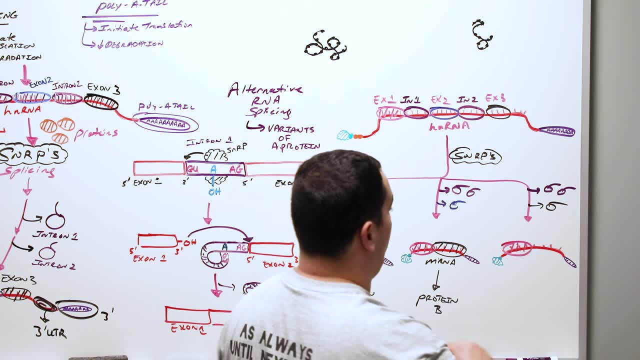 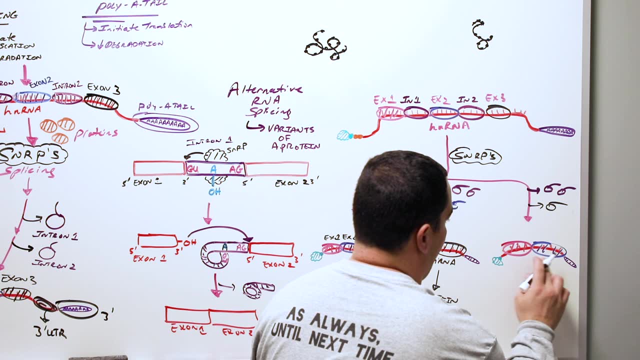 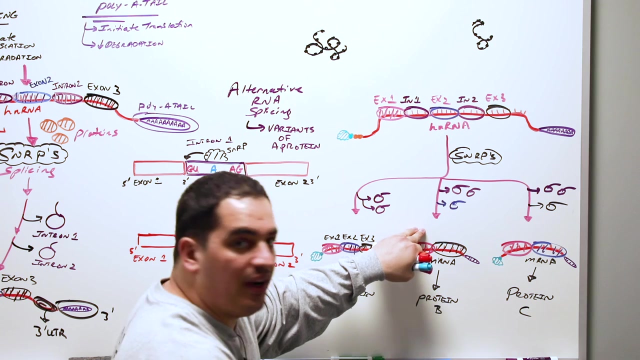 exon one and I'll be left with exon two. And what will this code for? This will code for this will give an mRNA that'll then do what Code for another protein, and let's call this protein C. From one hnRNA, we made three different mRNAs. 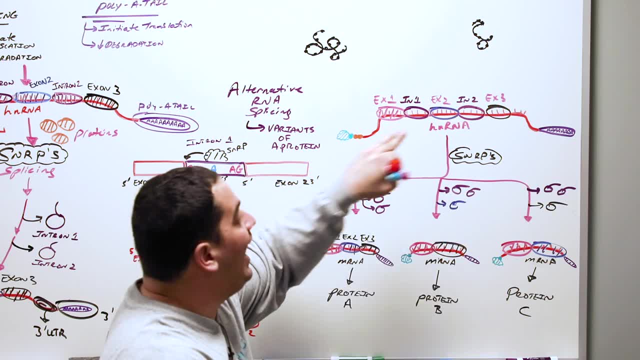 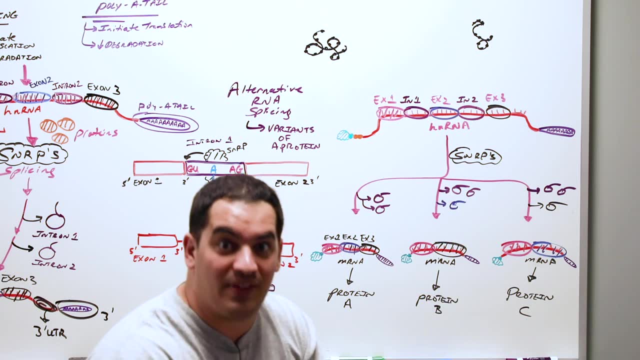 and made three proteins from the same hnRNA or from the same kind of gene, if you will. That means it's going to be the same protein if it's coming from the same gene, but it's a variant of that protein. You know what this is. examples of: 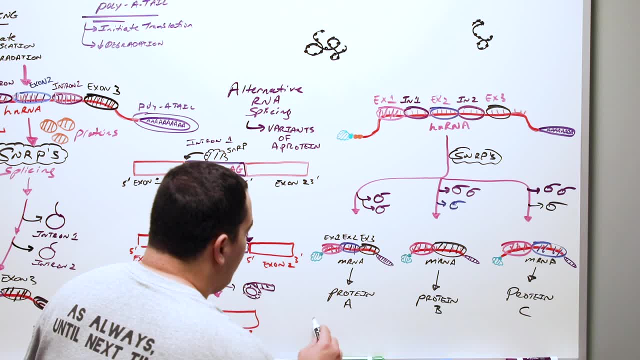 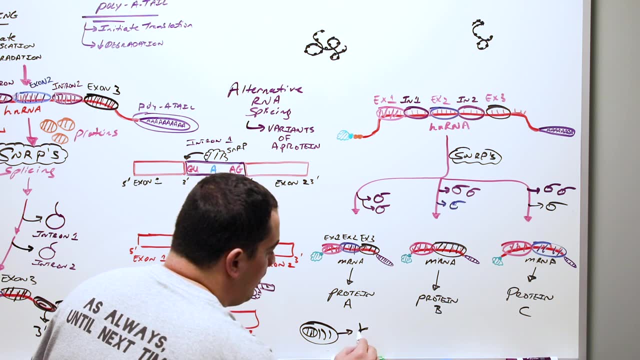 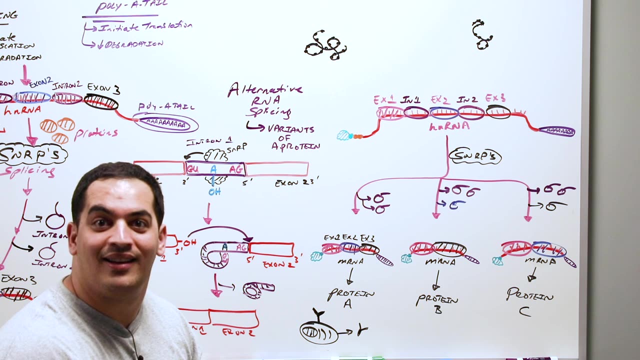 Think about it guys. Think about plasma cells, which make antibodies. When they make antibodies, you can have antibodies that can be secreted, or you can have antibodies that are different and they're expressed on the cell membrane. That could be one example. So antibodies- 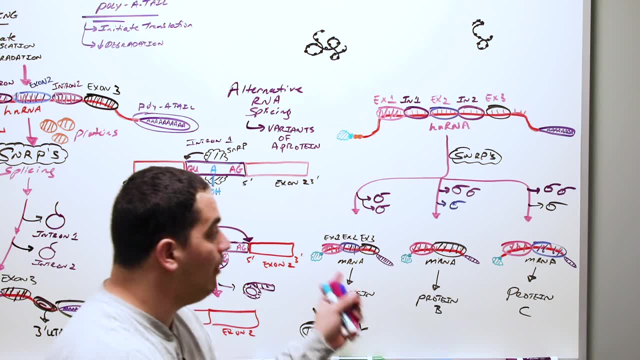 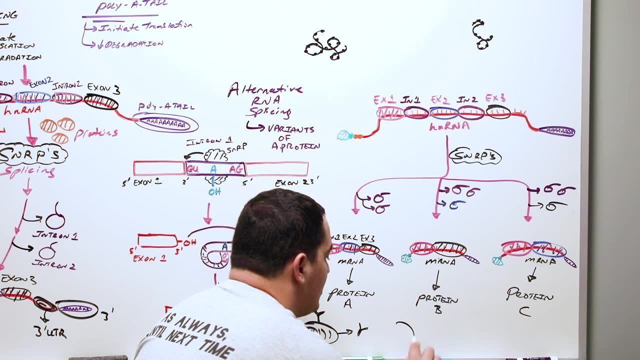 differences in antibodies would be an example of how that works from alternative RNA splicing, because I'm making one protein that'll bind to the membrane and one protein that can be secreted. Think about neurons. Let's say here's one neuron and this neuron. 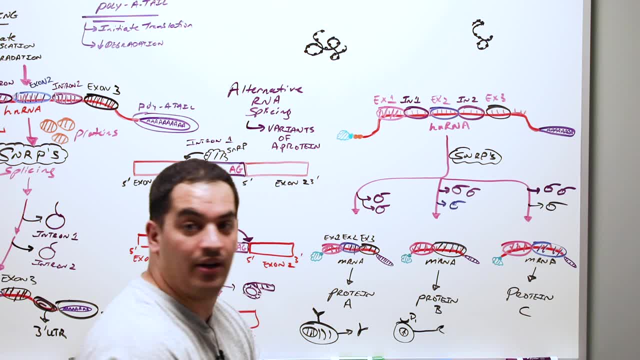 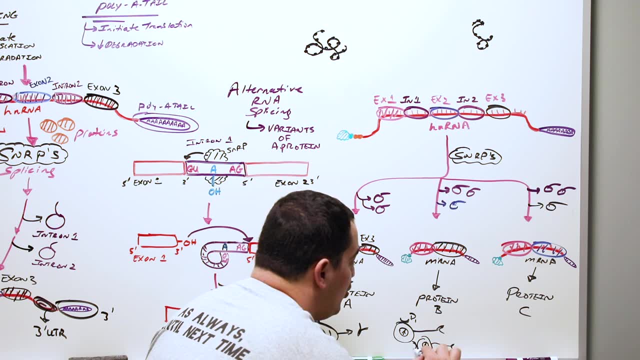 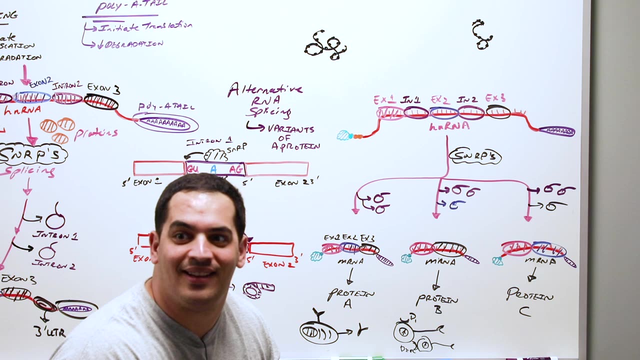 has a dopamine receptor. dopamine one receptor. But then you have another neuron and this has a dopamine two receptor. It's the same gene that's making these proteins, but just a variant of it. And then the last thing is: take an example of a muscle within the heart. 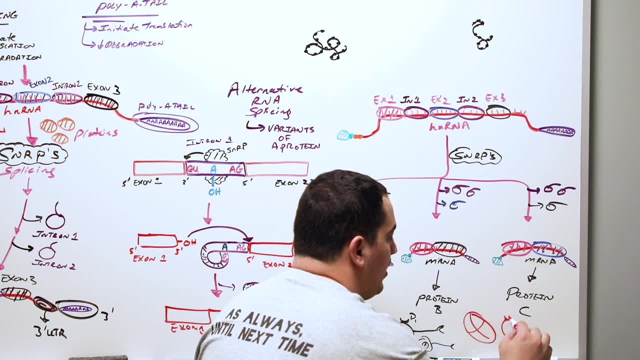 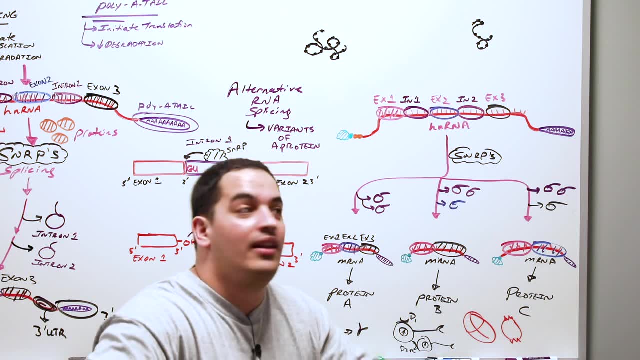 called tropomyosin, and the muscle within the skeletal muscle is tropomyosin. They're different. They're small changes or variants within the protein that are coming from the same gene. So one of the things that they'll love to ask on your exam questions. 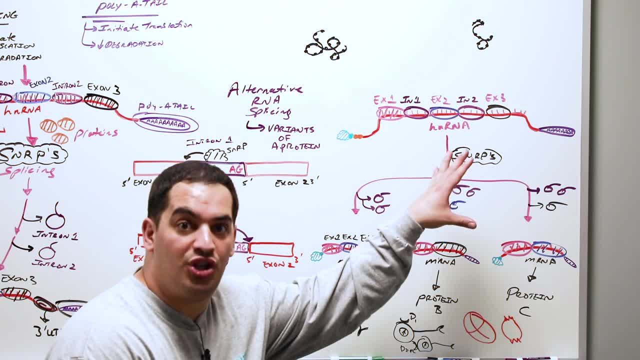 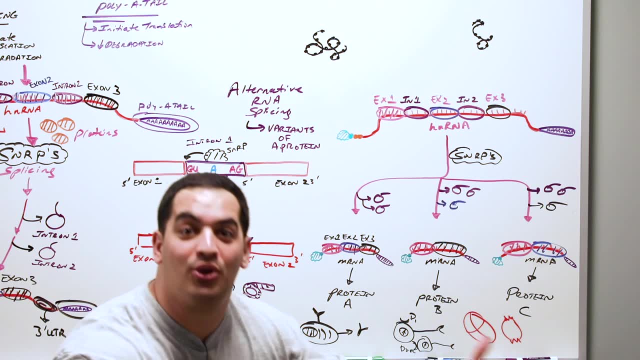 is alternative RNA splicing. It gives you takes one gene, one H in RNA, gives you multiple mRNAs in variants of the same protein. If you give examples, something like immunoglobulins, dopamine receptors of the brain or tropomyosin variant within cardiac and skeletal muscle. 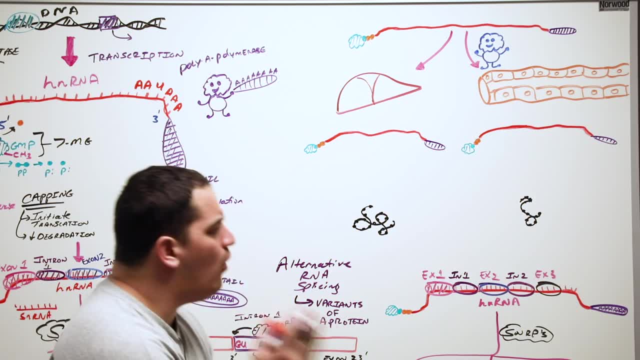 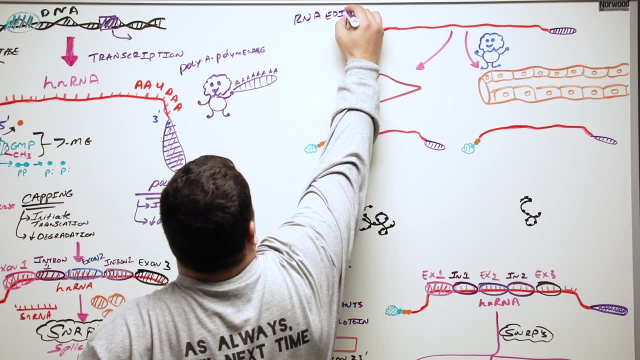 I promise. I'm so sorry for this being so long, but there's one last thing that I want us to talk about. The last thing that I want us to discuss is called RNA editing. This is also mentioned a lot in your exams, And the reason why is: 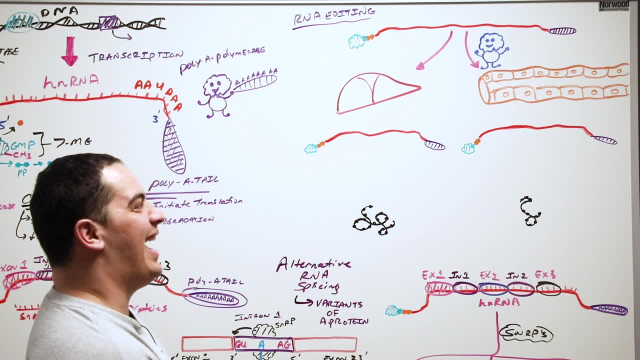 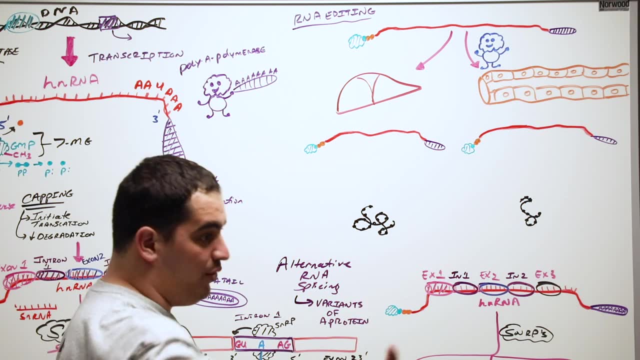 it's really interesting kind of how this happens. There's two different types of RNA editing. I only want to mention really one of them because it's the most relevant to your USMLEs and kind of a clinical setting. So let's say here: 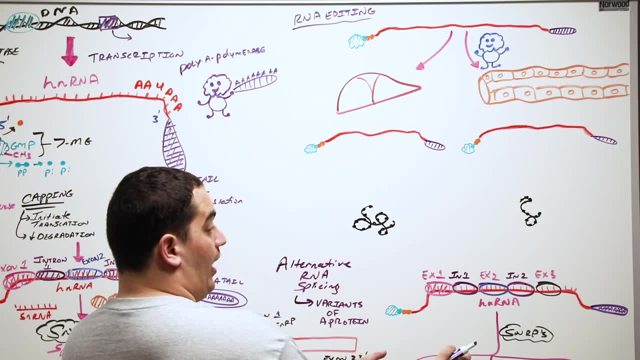 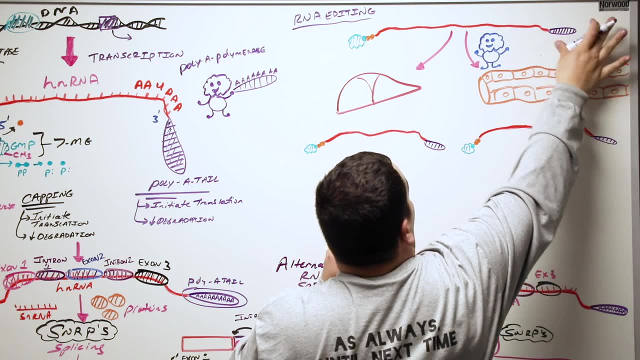 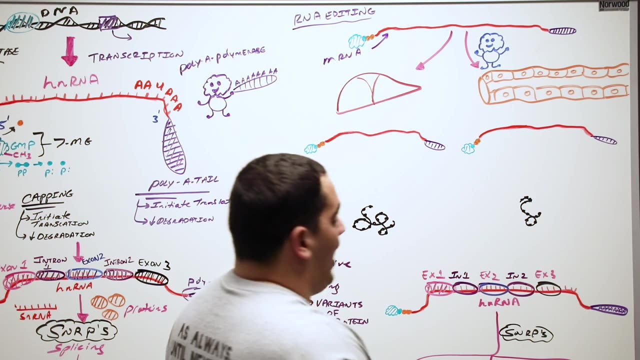 we have our mRNA. So this isn't an H in RNA. We've already, at this point in time for RNA editing, we've already formed our functional mRNA. So at this point in time, this structure here is a mRNA. Okay, This mRNA can have a particular nucleotide sequence. 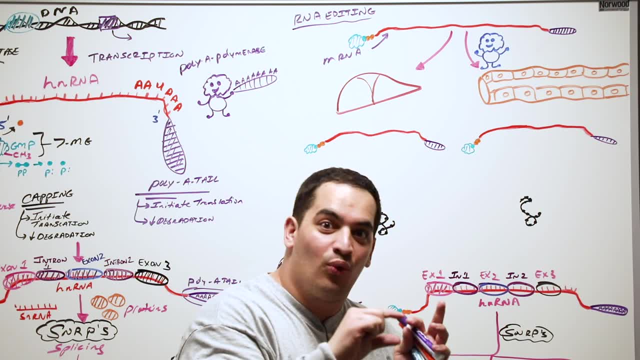 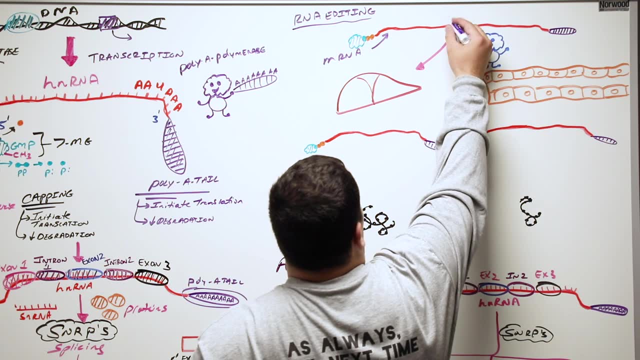 that a special enzyme can read and sometimes switch nucleotides with. What is that nucleotide sequence which can be seen in this mRNA which we really want to know? It's CAA, And we're going to be talking about apoproteins. 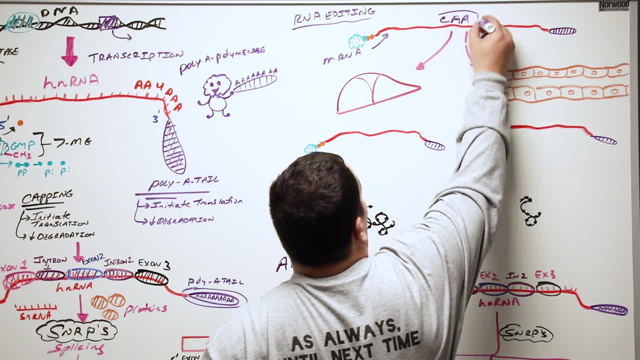 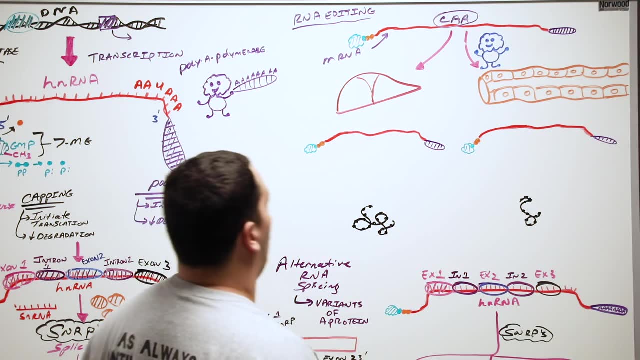 That's why I'm mentioning CAA. So this is our signal, which is really, really important within this mRNA Which is going to be making apoproteins, A particular protein called. let's say that this mRNA is going to code for a particular protein called. 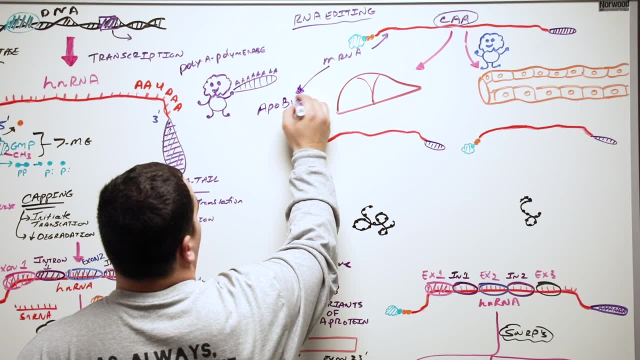 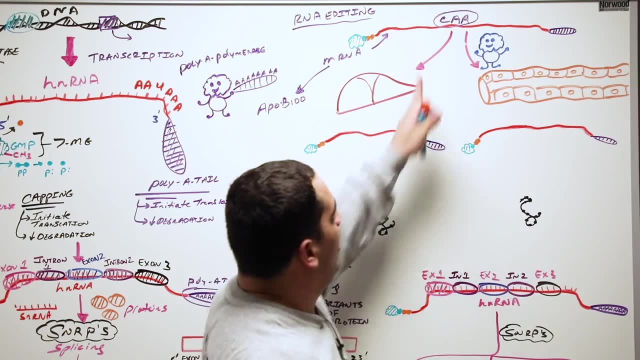 ApoB100.. If you guys watch our lipoprotein metabolism video, this will sound familiar, right? But ApoB100, this is going to be the mRNA that will code for that protein, And here's a particular nucleotide sequence that we're going to modify. 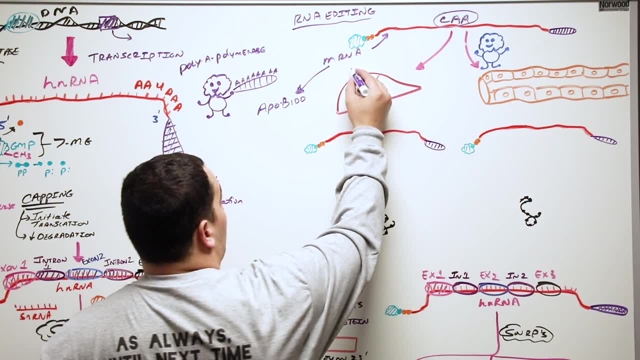 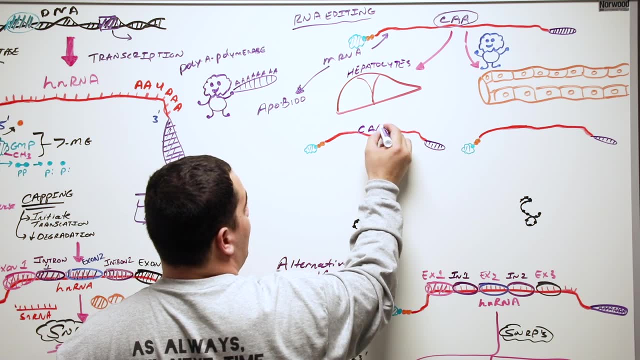 In the hepatocytes. this nucleotide sequence is not all about is not altered in any way. It's kept the same. So it's not going to be changed. It's still going to be CAA And whenever this mRNA is translated by ribosomes. 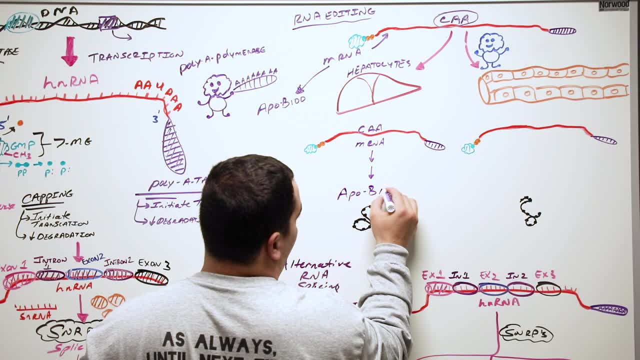 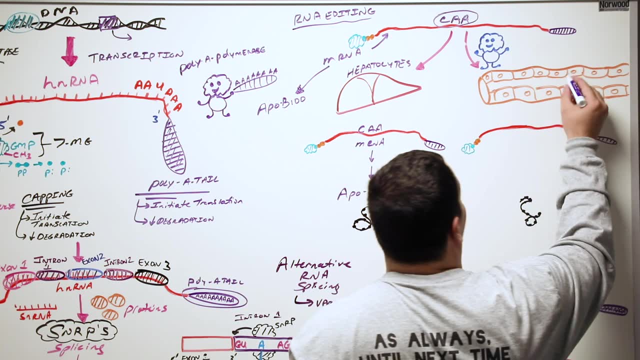 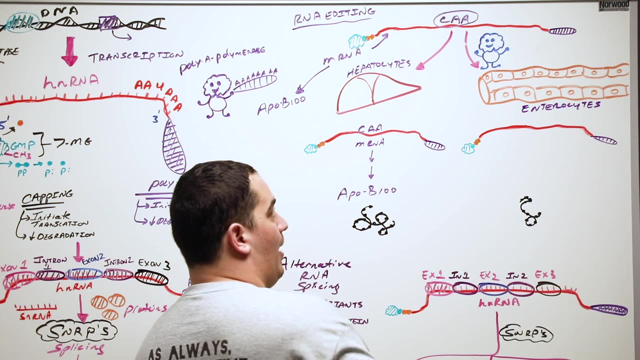 it makes a particular protein that we already talked about, called ApoB100. But in enterocytes- okay, your GI cells, what are these cells here called? These are called your enterocytes. They have a very special enzyme where they can modify the same gene. 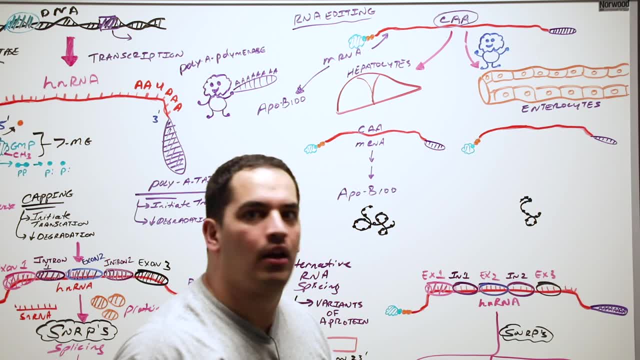 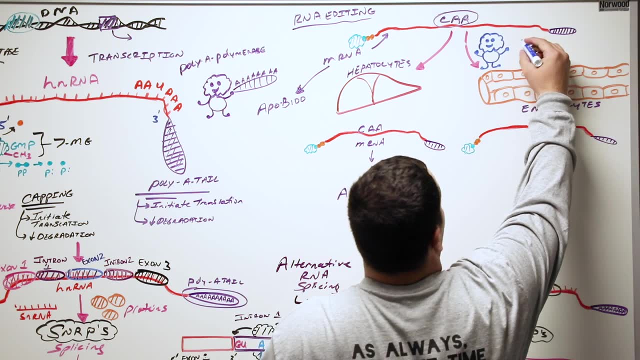 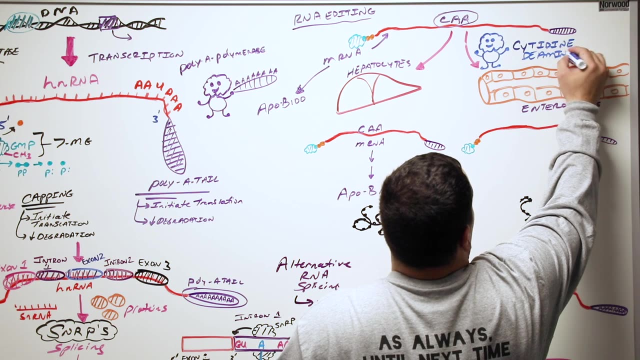 that makes ApoB100 but make a different protein. How the heck? How do they do that? Let me explain. There's this cute little blue enzyme in the enterocytes called cytidine deaminase, And what this cytidine deaminase does is 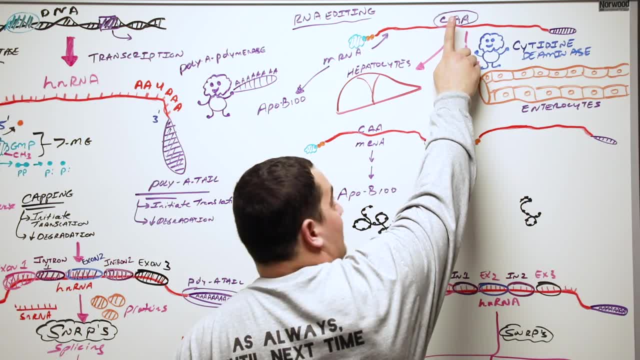 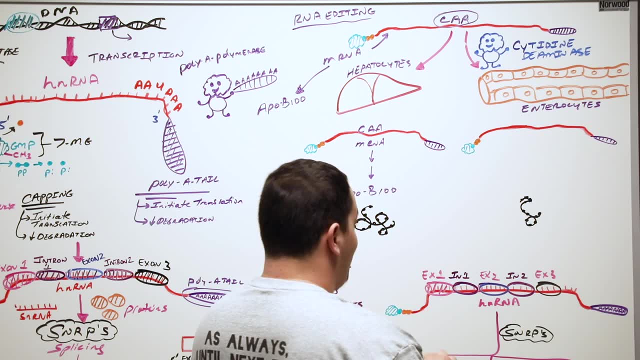 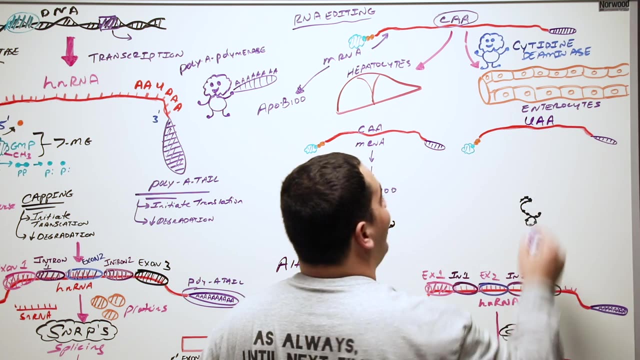 is. it deaminates the cytidine right here or the cytosine nitrogenous base And switches it with uracil. So now let's switch it here, where we're going to have this as switching C and putting UAA, If you guys know anything. 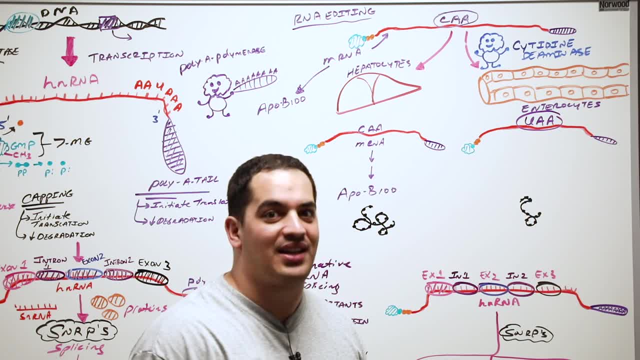 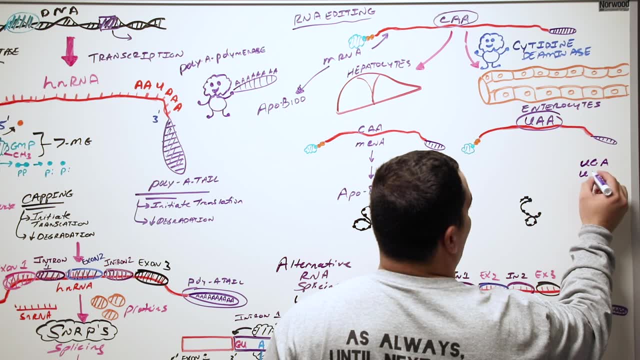 about your codons. there's a little trick to remember your stop codons. Do you guys remember the? the little way to remember them? You remember it by you go away. You are away, You are gone. These are the easy ways to remember your stop codons. 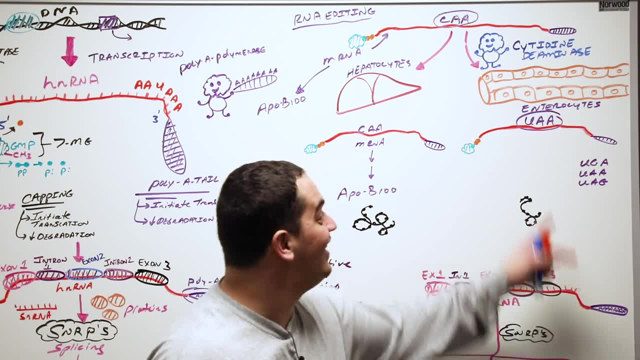 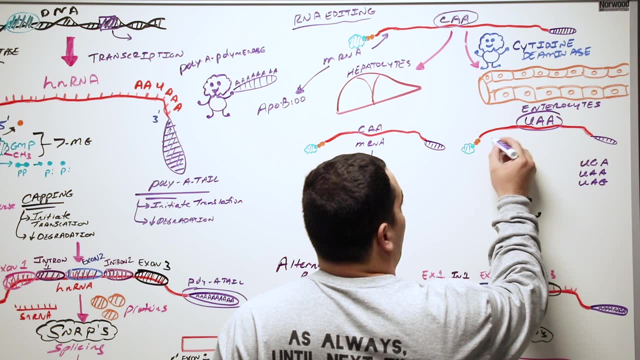 Does any of these look like a stop codon? Yes, UAA, UAA, that's a stop codon. So what's going to happen is when you have the ribosomes which will be reading this. let's say here, I kind of put 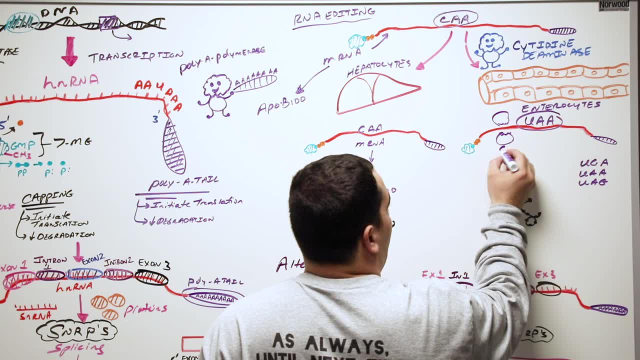 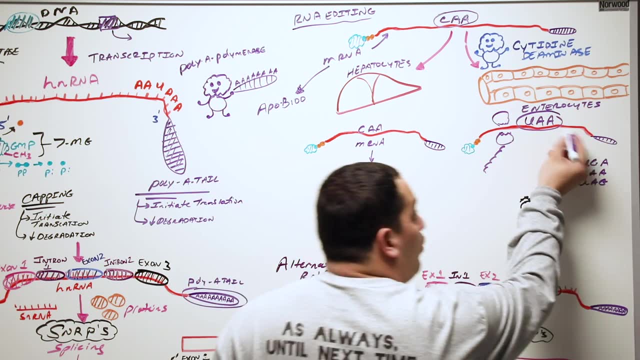 like a little ribosome. It's going to be reading this and making a particular protein As it gets to this point where it's going to translate it. that's a stop, codon. Will it then read the rest of the RNA and translate that into a long protein? 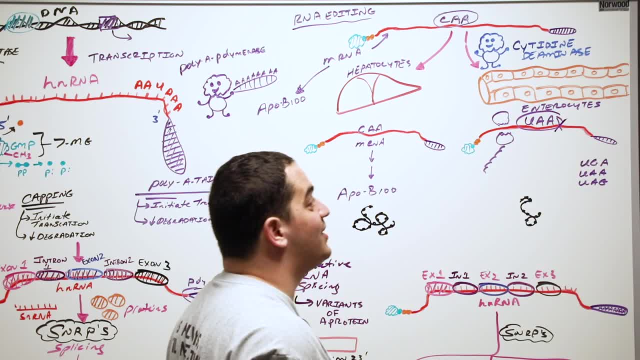 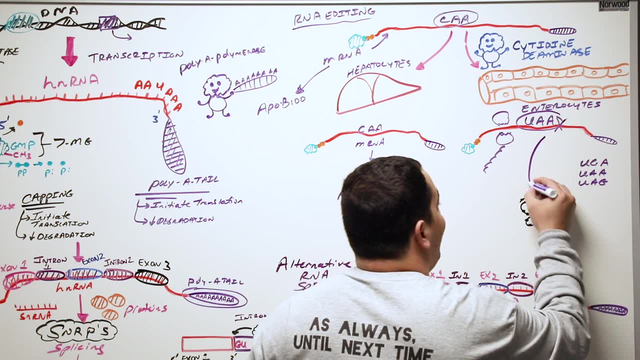 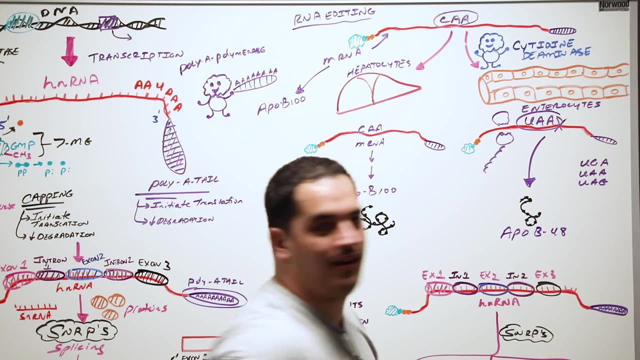 No, So at this point translation will stop. You won't read all the rest of the mRNA and make the full protein. Instead, you'll make a smaller protein, And this small protein is called APOB48.. This is something that they love. 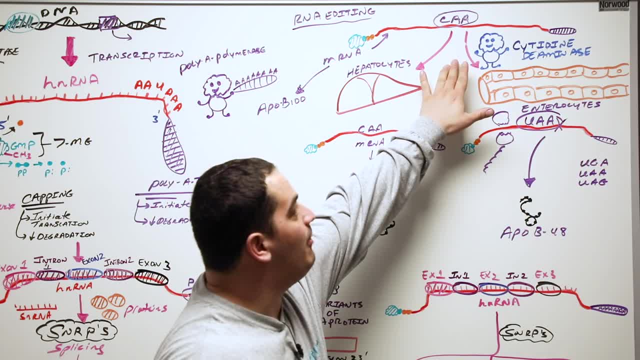 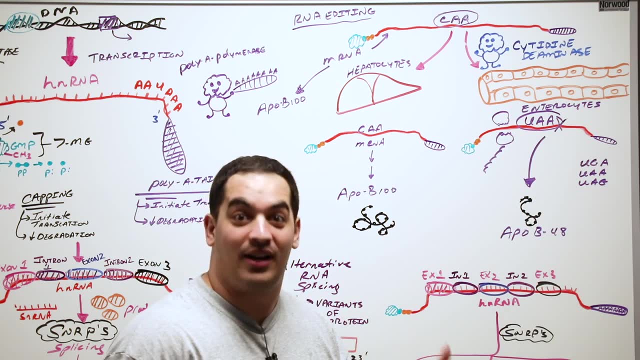 to ask on your exams because you're taking the same mRNA, just modifying it a little bit to produce a different protein That is a completely different size protein. So that's really cool. Definitely wanted you guys to know that, And that finishes our lecture.